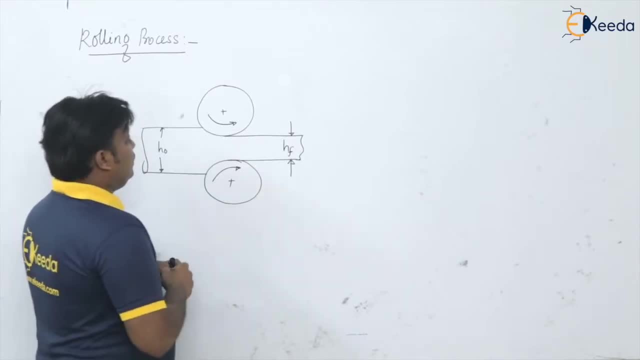 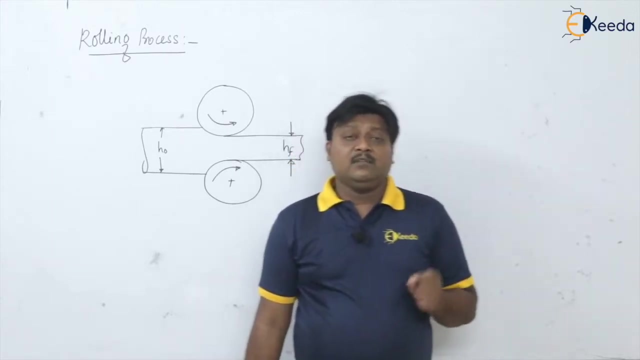 the constant velocity. okay, so these are the two rollers. so the metal is compressed, the material going to have the plastic deformation and it is, okay, in a lengthwise direction. okay, so this is actually rolling process. so rolling process is one of the oldest metal forming process, which is having a very high productivity with the low cost. that is why it is. 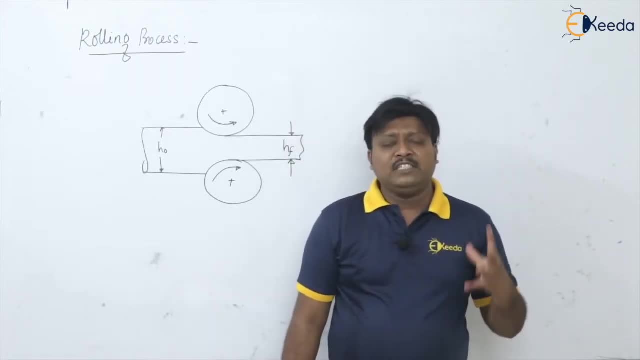 very important process so we can produce the different cross sections like t, l, okay, i and up to certain extent we can go for some complex shapes, so very complex shapes. we cannot get deformed in the rolling operation. so, as i told you, these are the simple shapes we 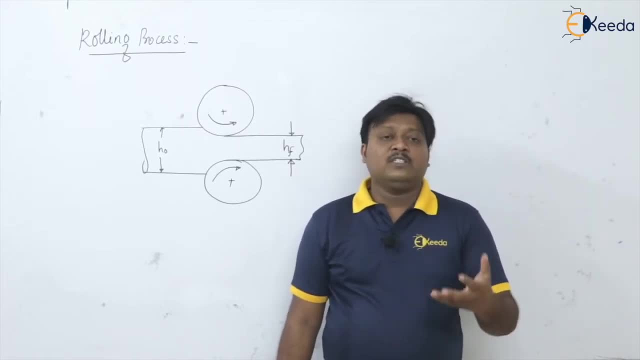 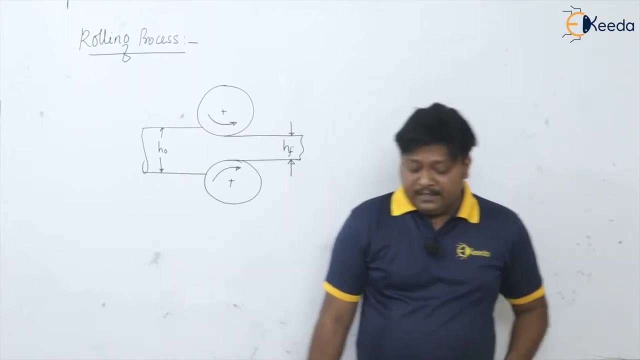 can able to produce. so if you go to the, say, the manufacturing of the railway wagon wheels, this can be produced. if you get it into single, single part that can be again able to produce by these rolling operation. okay, so this is simple definition and some introductory part about the. 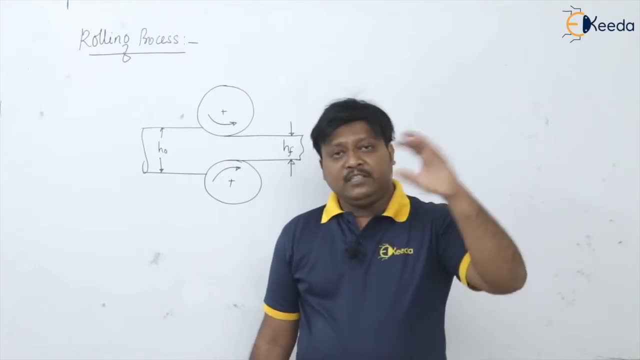 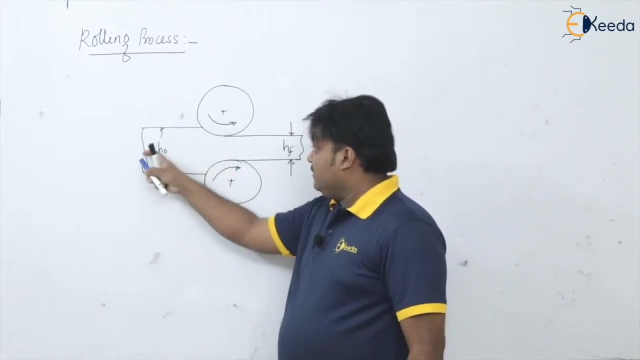 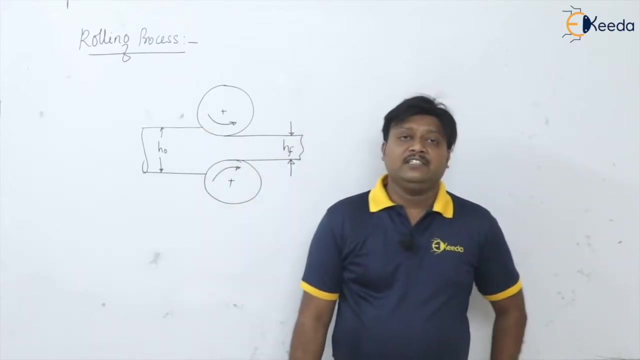 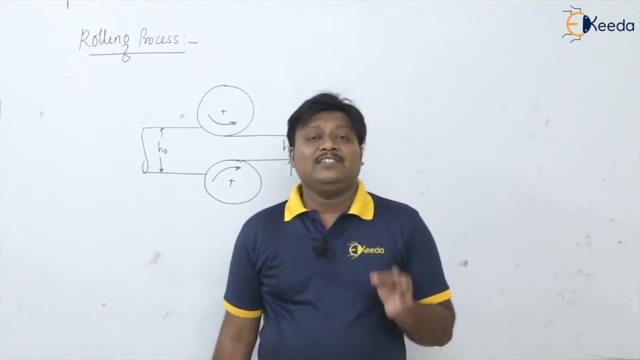 rolling rollers in that roller, these railers are rotating and we are supplying or giving the material between these two rollers so that, because of the deformation, you can get here the reduction in the thickness. okay, now, very importantly, make a note that this rolling process is always treated as 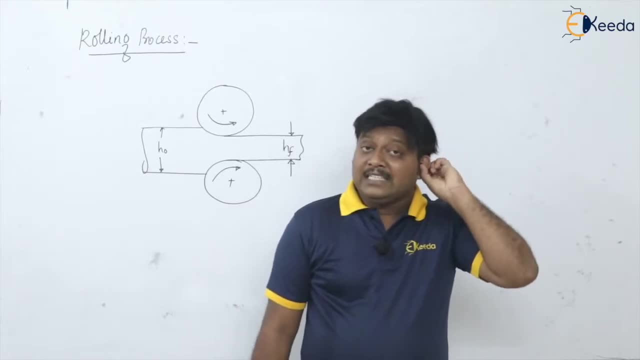 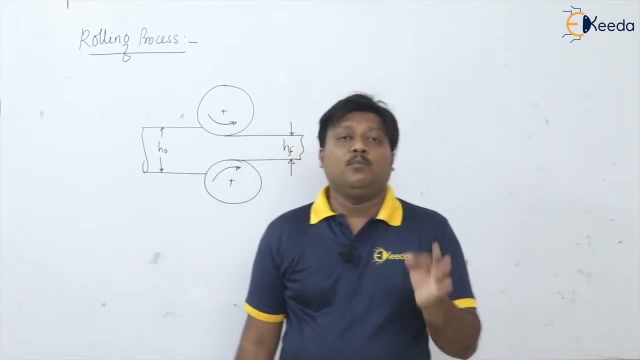 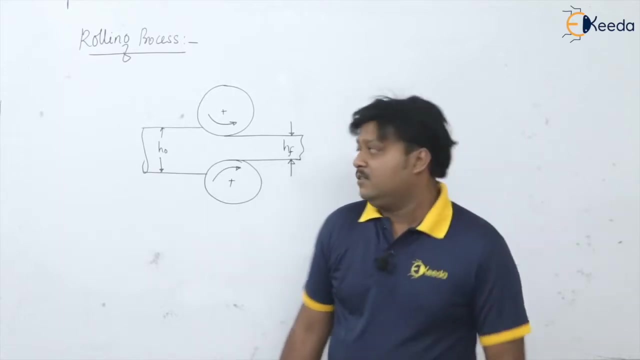 the hot rolling process. please remember, unless and otherwise stated, we always have to assume the given rolling operation as a hot rolling operation. okay, if there is a intentionally or there is a highlight there highlighted for the colder rolling process, then and then only we can assume that this is the cold rolling process. otherwise, please remember, the rolling is always. 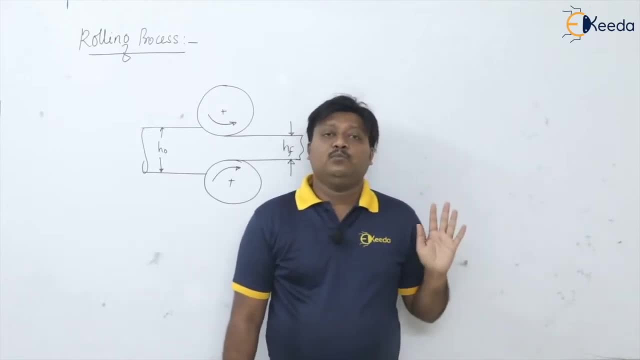 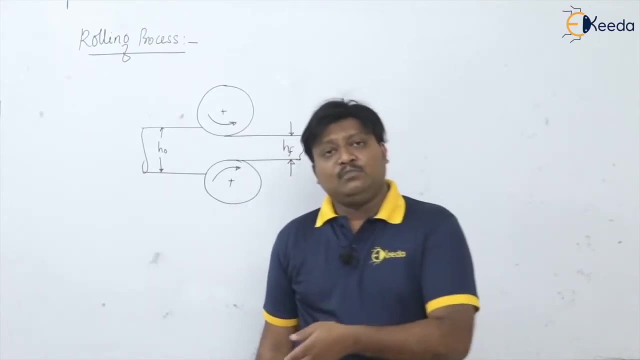 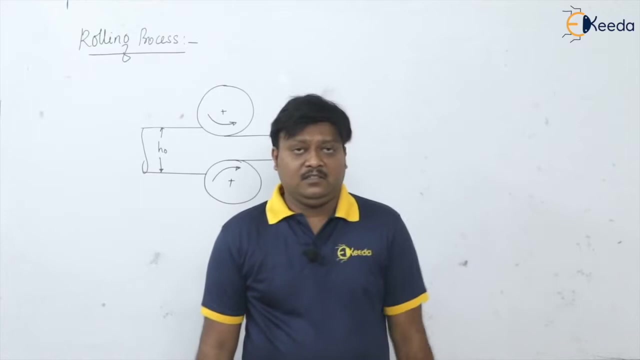 rolling is always treated as hot rolling process. okay, so before going into the detailed analysis or mechanics of the rolling, so let us have some assumptions in this process. so what are these assumptions? what are the assumptions we are going to do? first, we will take that and move forward. 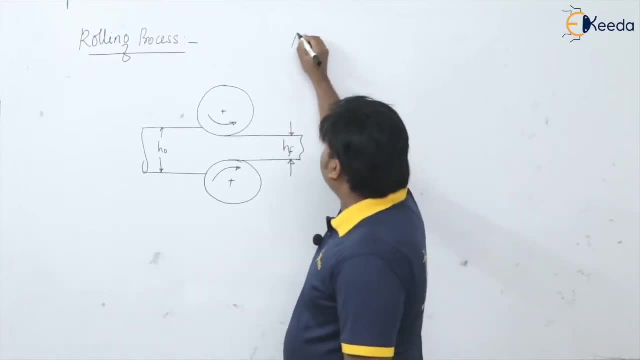 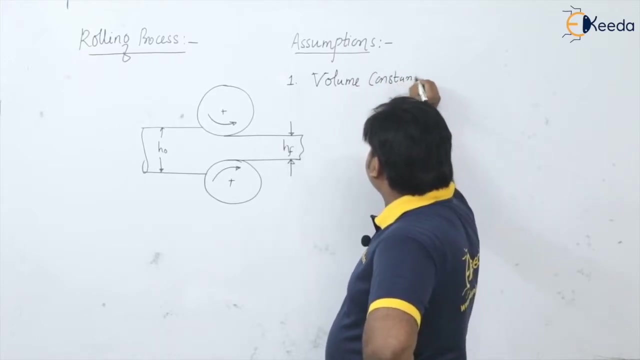 so the first assumption, so I will write here the assumptions now- why these assumptions are required: to analyze the process, to see the mechanics of rolling process. these are the assumptions are made. so the first assumption is that is very simple, because it's a forming process. so volume constancy is valid. so volume of the material before and after. 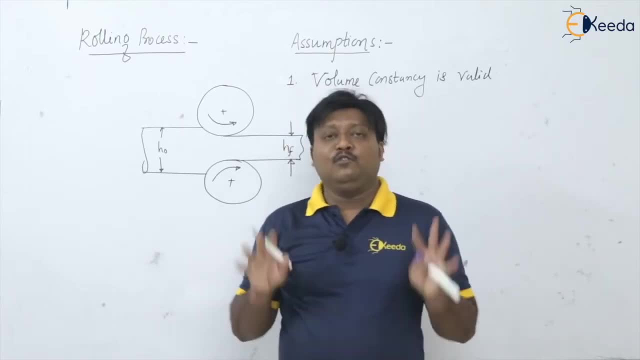 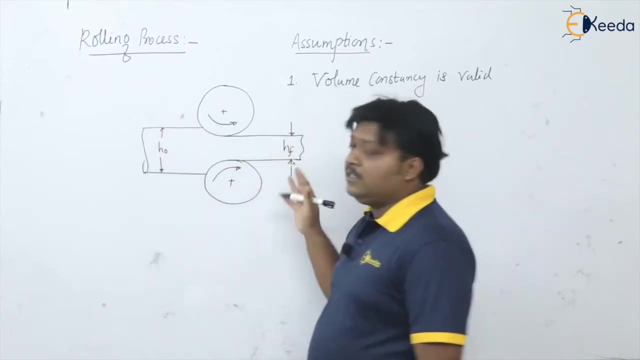 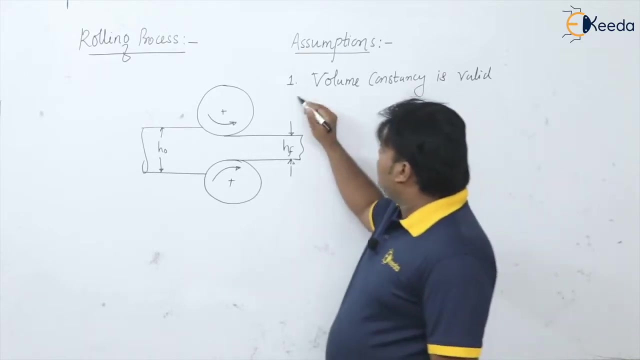 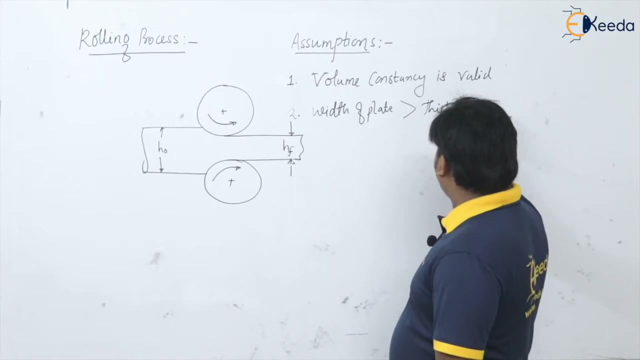 process is going to be same or the volume flow rate will be going to be same, So the initial volume will be at the last or at the exit. Okay, So volume constancy is valid. The second important thing is that the width of the plate is more or larger than the thickness of the plate. 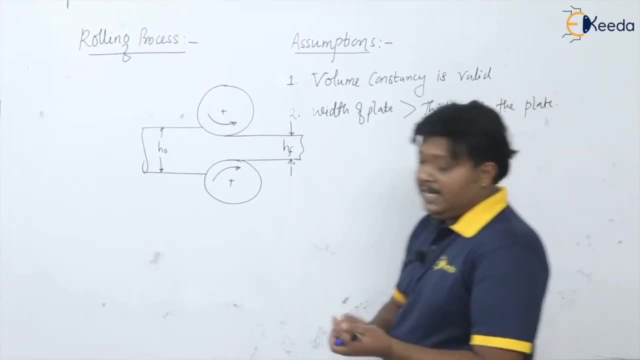 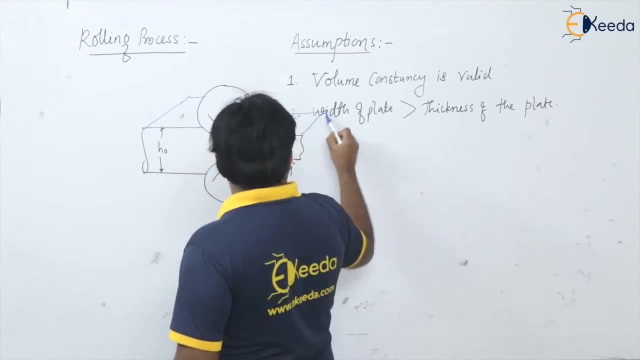 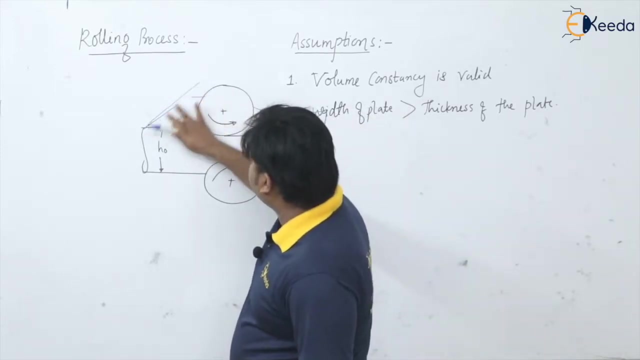 Please remember what we are considering, that Whatever say width of this plate is much more in size than the thickness of the plate. Okay, So I have to little bit more width. I have to show here. That is why what we can have assumption here: 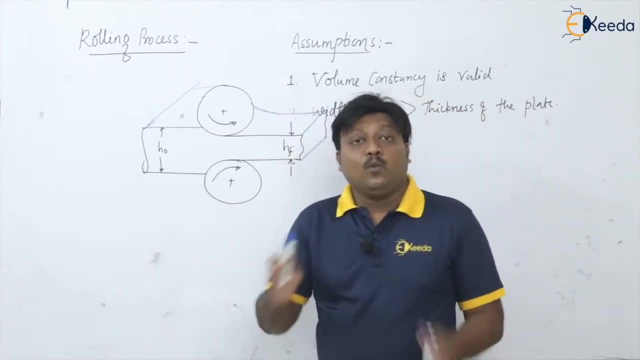 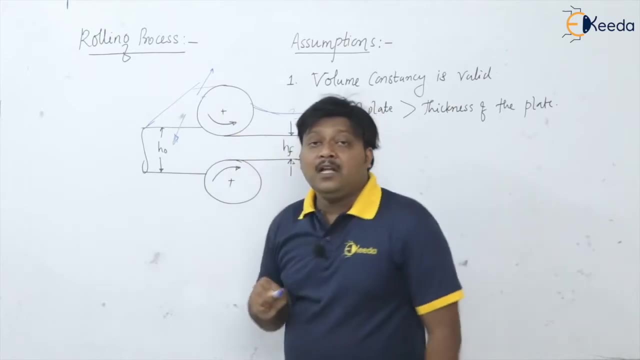 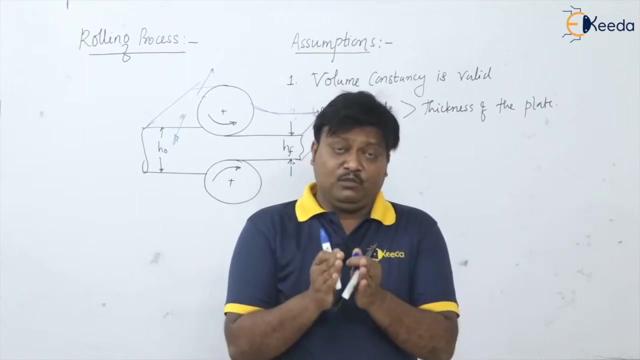 So there will not be any widening of the plate in the width direction. Please remember, Very important As we are, what we are assuming: that the width of the plate is larger than the thickness of the plate. That's why, during the deformation, there will not be any widening of this width. 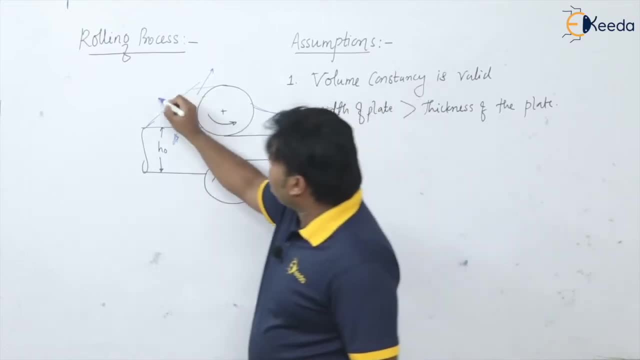 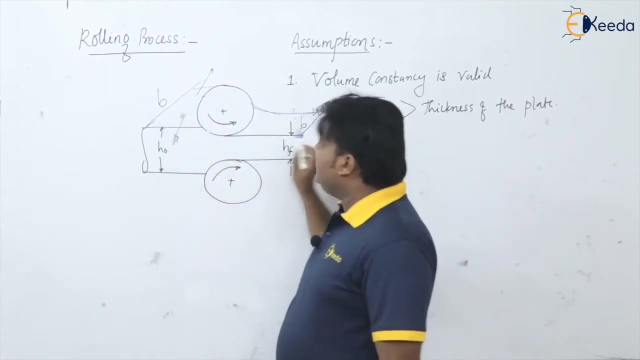 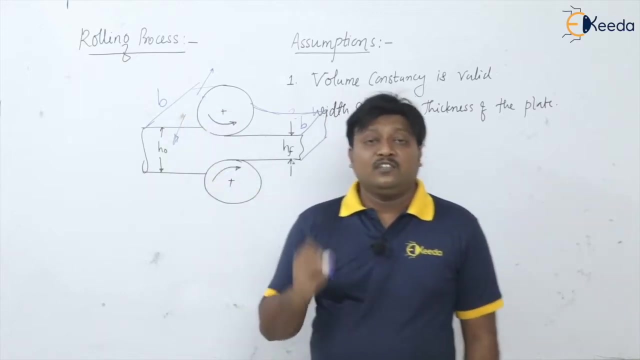 Okay, So that is means what this say. B is the width of the work, that sheet or plate. Okay, This width is going to be same before and after deformation, Please remember. So this B is going to be constant. width of the plate will remains unchanged. 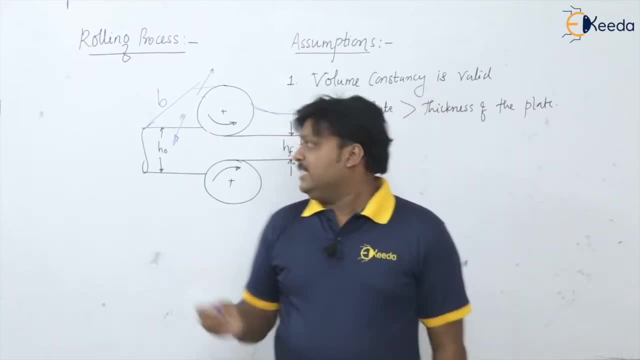 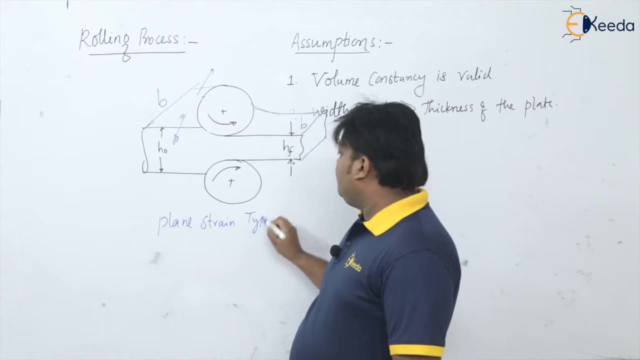 That is the assumption. So what is that actually? This is the operation of plane strain type, Isn't it? That is a plane strain. Plane strain condition is valid. Okay, That is the thing that is. width is going to be. 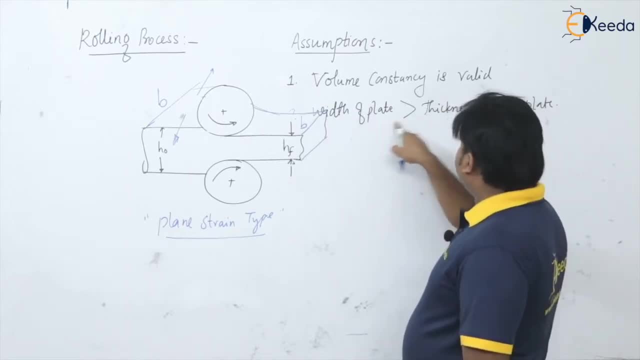 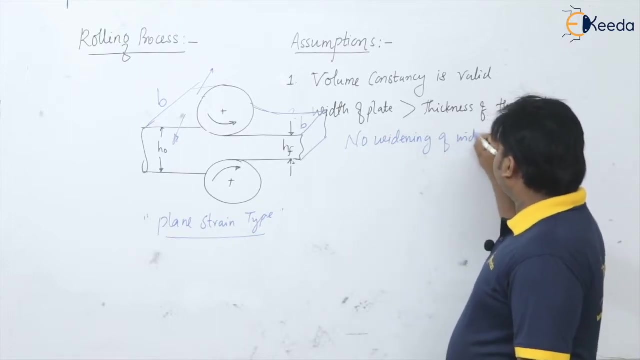 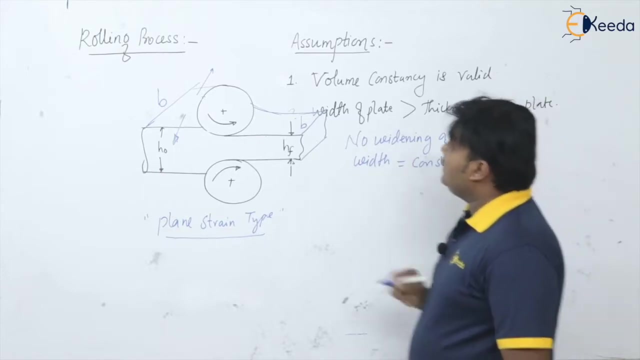 So, in other words, Width of the plate, Thickness of the plate is more than the thickness of the plates. Why the two or no widening? that means no widening of width. Okay, That is. width is going to be constant. That is the thing. 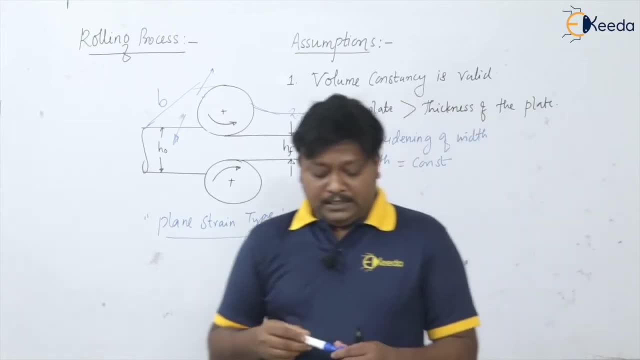 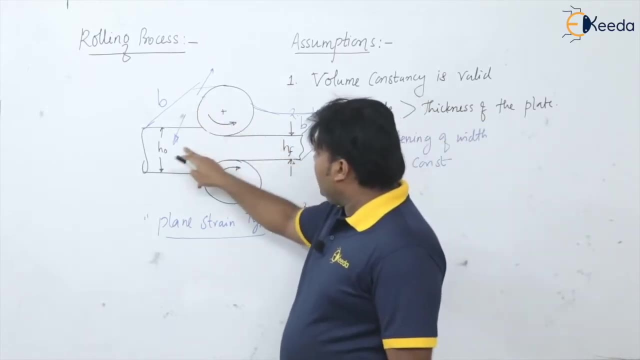 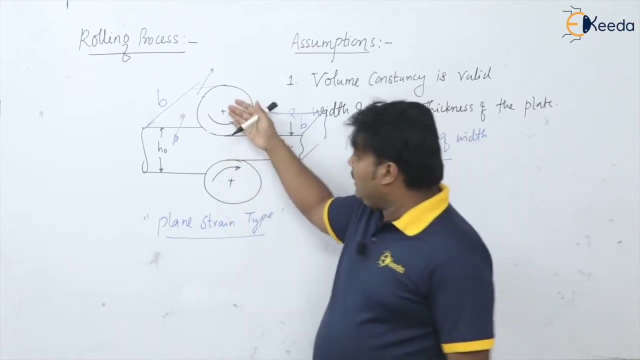 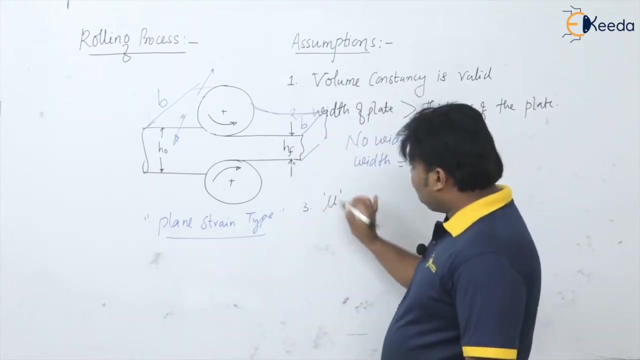 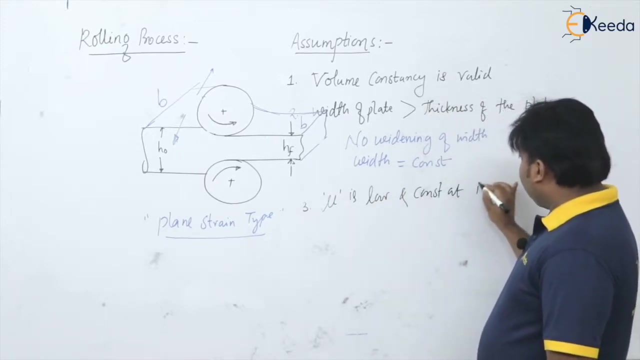 This is the second assumption. Okay, Now the third assumption. what we are saying? that the coefficient of friction between the, The roll surface and the plate surface, or the at the interface. okay, the coefficient of friction at the interface of roller and the plate is going to be low and it is constant. mu, that is coefficient of friction, is low and constant. at what or where? at interface of the roll and plate. 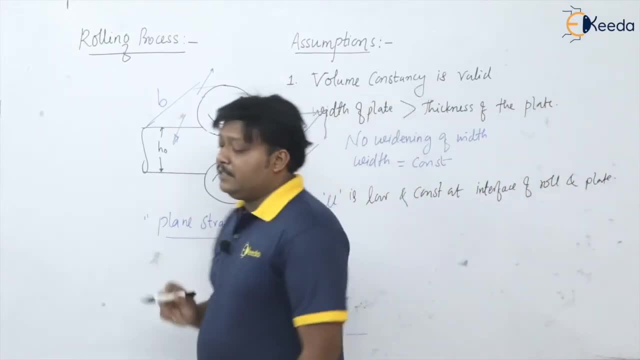 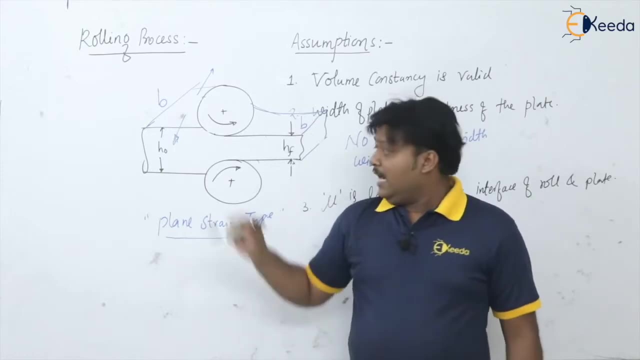 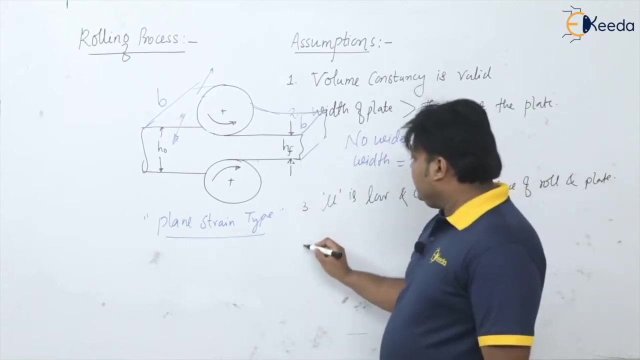 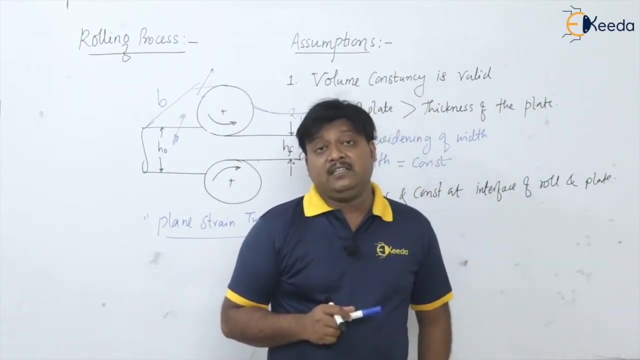 That is very important. That coefficient of friction. We are assuming that it will be a constant throughout the operation at the interface of roller and plate, and it is of course it is low. and the last assumption we can have here, What is the last assumption- says that is the yield strength of the material is again going to be constant throughout the process. 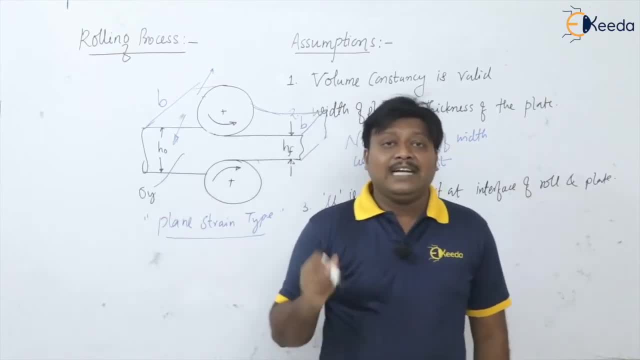 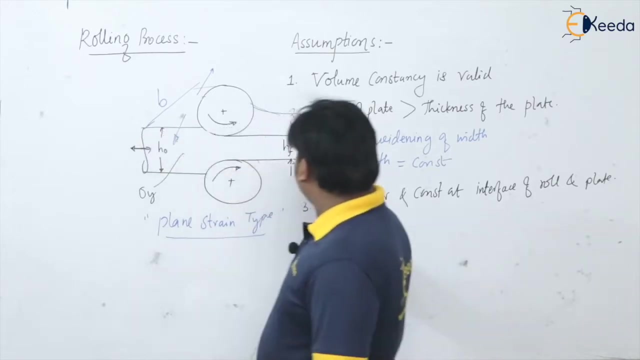 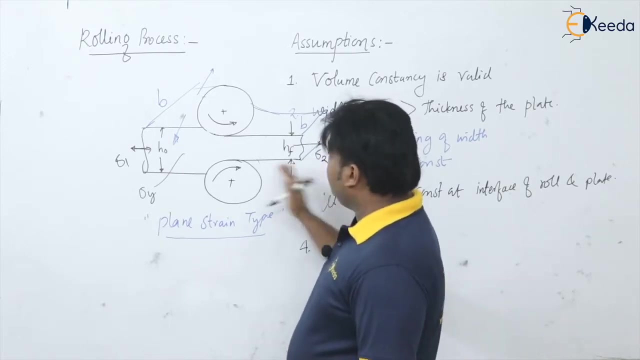 Say Sigma y is the yield strength of the material. That is going to be constant throughout the operation. So, beginning me Jitani thi wahi kya hogi, end me utni hogi, okay. and if we are provided with the front and back tension- say Sigma 1 and Sigma 2, okay. so this is a back tension and this is a front tension. 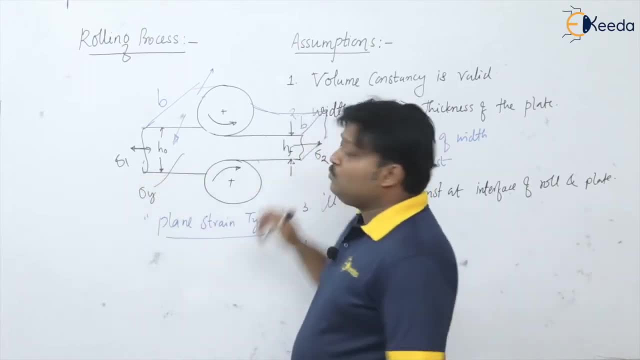 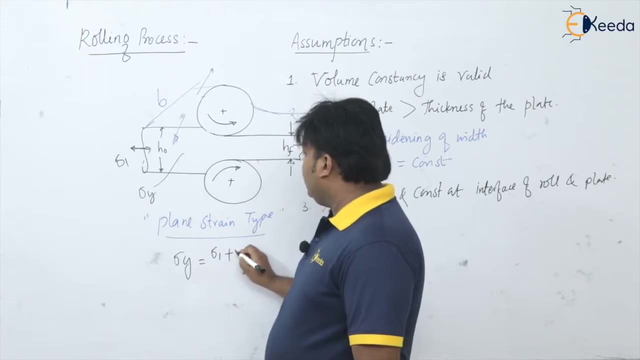 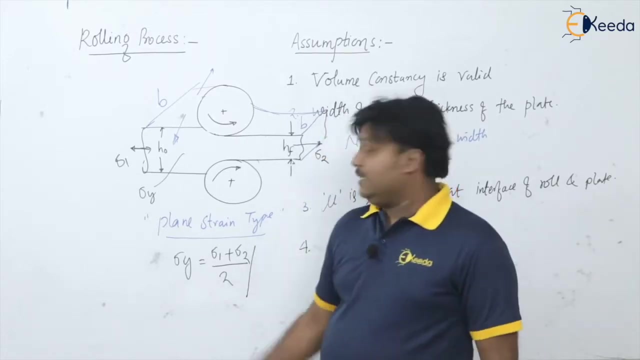 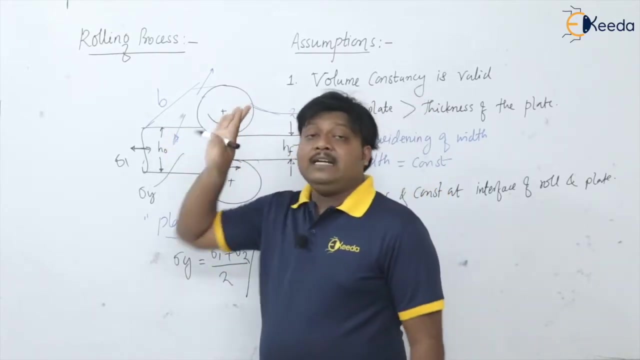 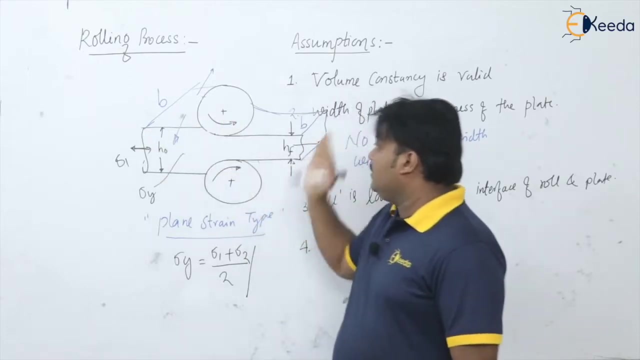 If this Sigma 1 or Sigma 2, these are given, then you can Take this Sigma y as the average of these tools, That is, Sigma 1 plus Sigma 2 by 2.. Please remember, if the condition is such that agar aisa hoga to, then when the front and back tensions are given, but Sigma y is going to be same constant throughout the operation. before the operation or before the deformation, after the formation at the front at this, 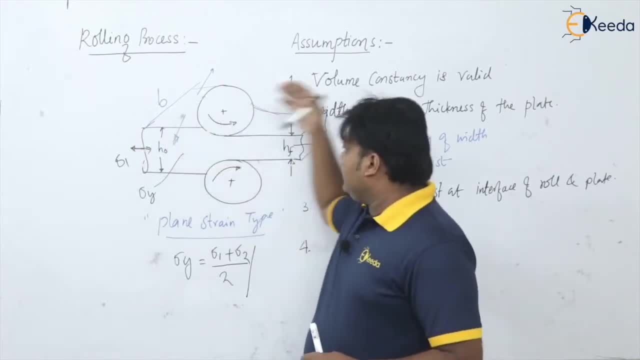 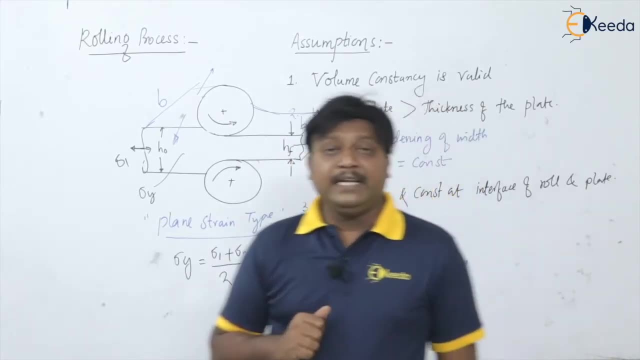 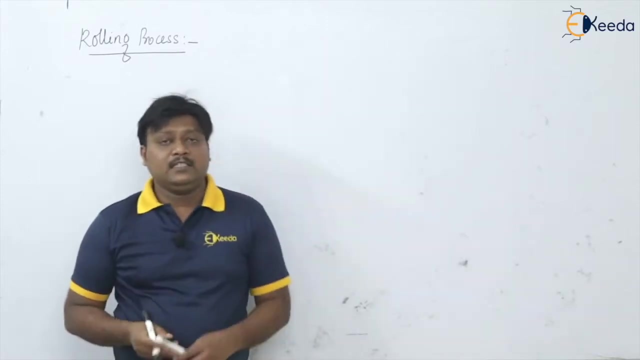 Sorry, at the front, Back, at the initial stage or at the final stage, It will be same. So these are the assumptions which we have to made before seeing the welding process in details. Okay, let's look at this now, students. Let us have the first assumption into consideration. 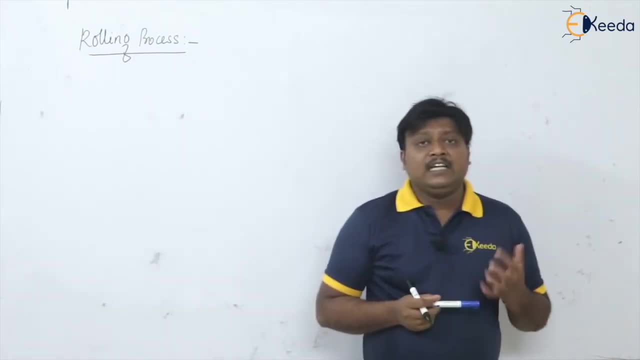 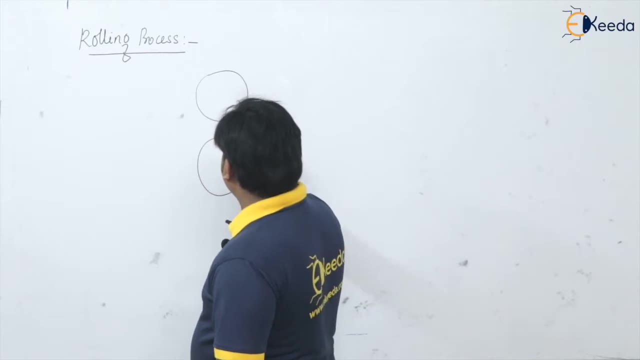 Kya hoga? when the volume constancy is valid. So when the volume constancy is valid. So these are again, I will draw. These are the two rollers. Of course, see, rollers are with the same diameters and they are moving with only the same velocities, which is constant throughout the operation. 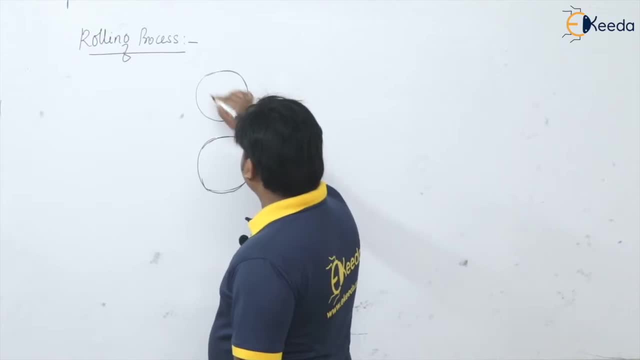 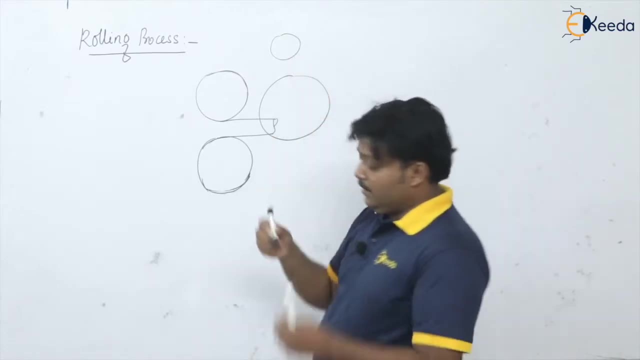 Please remember. it is not like that: one roller it and another roller it like this. What will happen if you are using this such a kind of rollers? then there will be the bending of the plate, No, any deformation. Okay, please Keep it in mind. 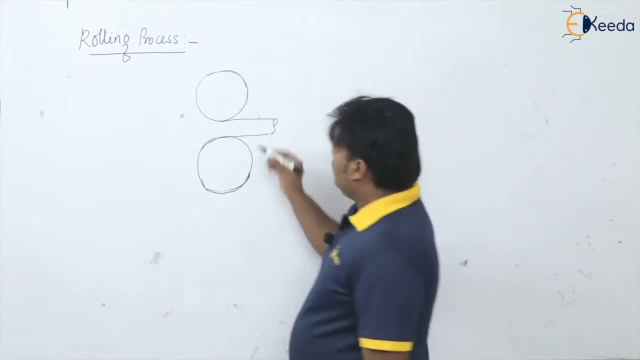 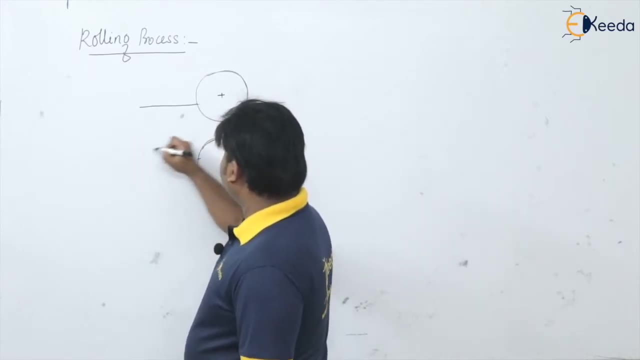 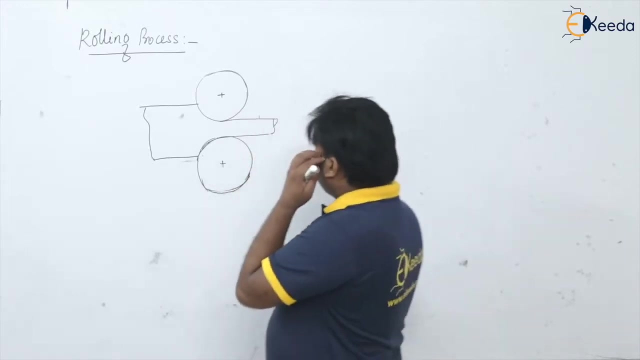 So again, they should have the same velocities also. Okay, so say, this is the material that is entering into the roller And this is at the exit. Okay, So now what I'm saying, that we have to say: take into consideration the first assumption. 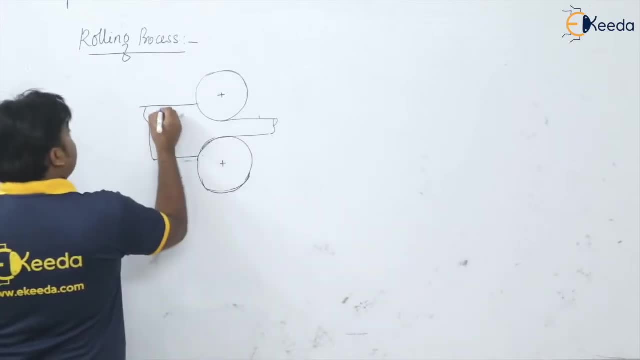 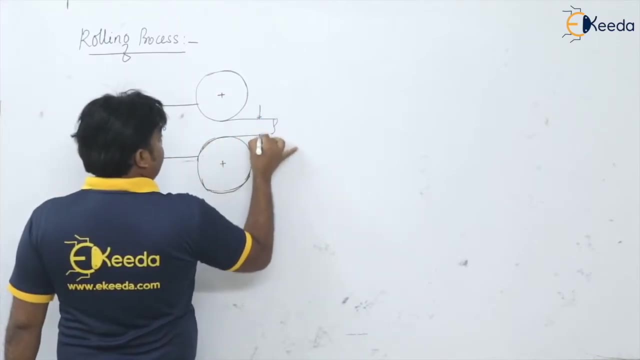 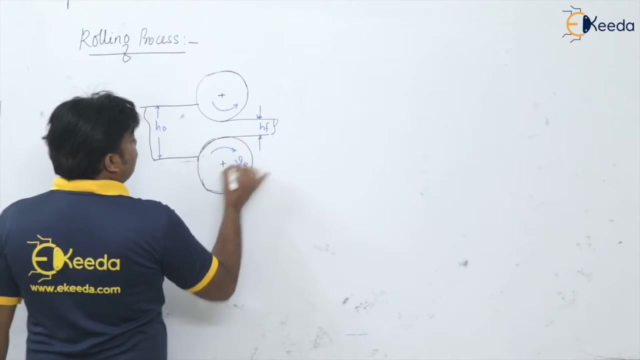 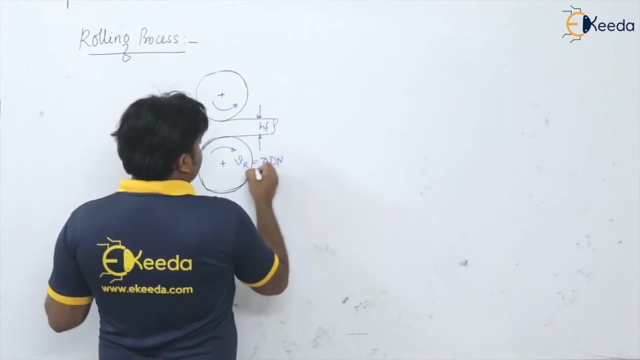 So let us have The initial plate thickness or height as H original and the final that you are going to get- say it is H final roller- is moving with the constant velocity. say VR is a roller velocity is a roller surface velocity. Okay, how to calculate? say pi d n by 60 in meter per second or pi d n by thousand in meter per minute. 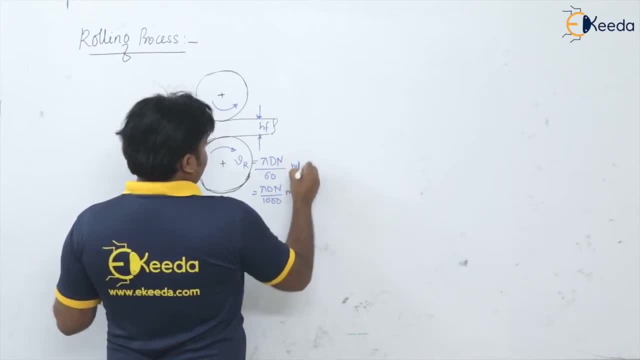 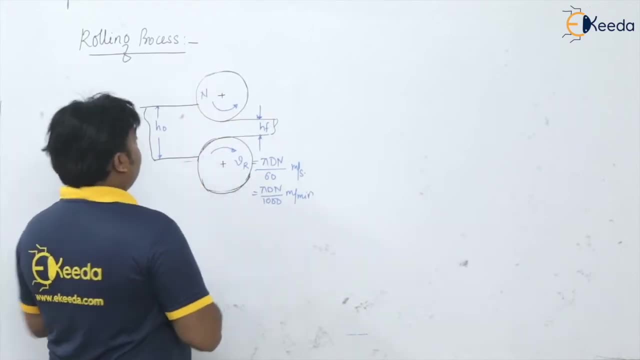 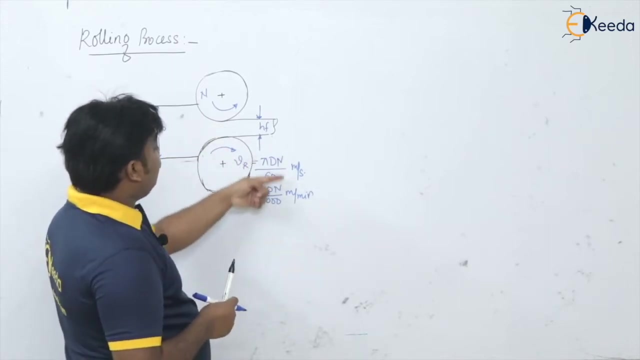 Okay, So see, capital N is the RPM for the roller. roller is rotating with the constant RPM and and to have the linear velocity of that, So we have to multiply with the. this pi d n by 60 watt is Omega. for that We have to multiply with the radius of the roller. 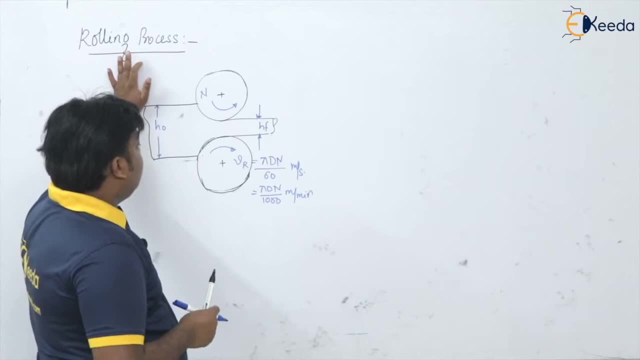 Okay, So we have to multiply with this pi d n by 60- watt is Omega for that. We have to multiply with the radius of the roller. Okay, So we have to multiply with the radius of the roller, isn't it so that we can get the linear velocity of the roller? 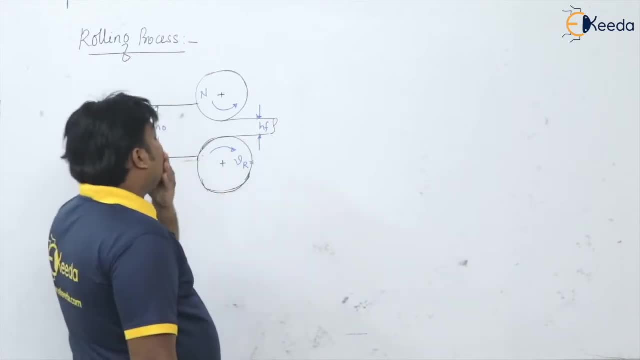 Okay, So see here. So what is the velocity of roller here? If it is moving with the RPM young, then it is say pi d n by 60, isn't it So pi d n by 60, that should be the velocity of the both the rollers. 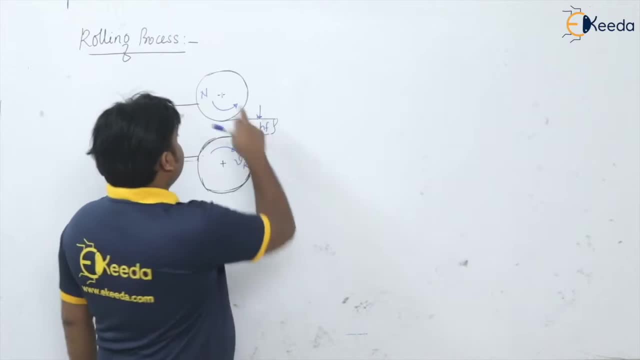 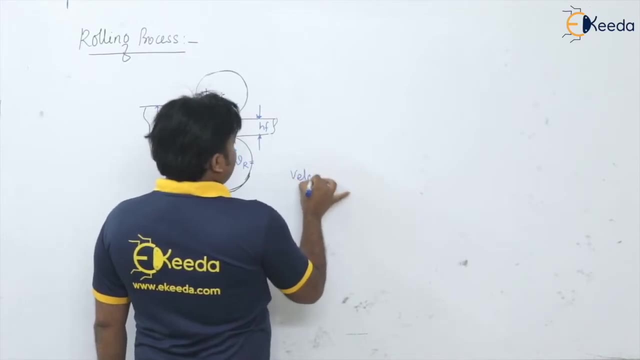 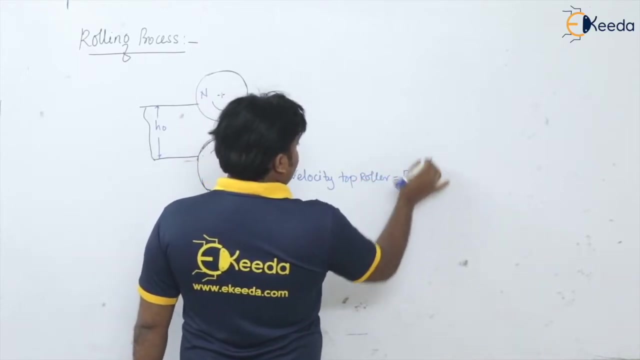 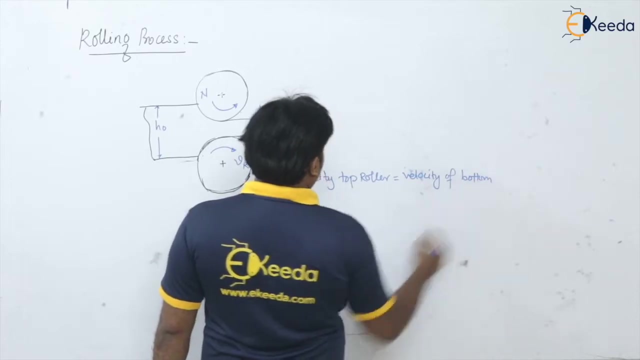 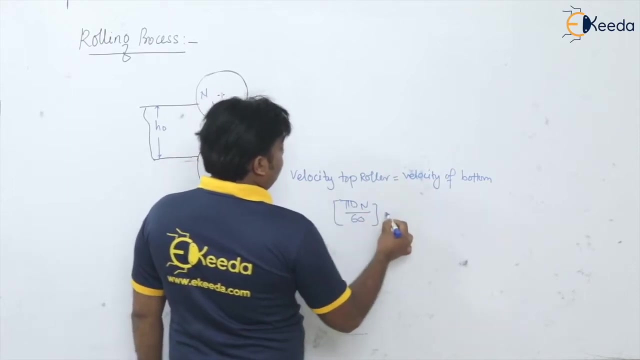 Okay, that is, if I write for, say this is top roller and this is bottom roller, The velocities are going to be same. the velocity of top roller should be equal to roller velocity of bottom roller. Okay, So if it's pi d n by 60 for top and having the same rotation, 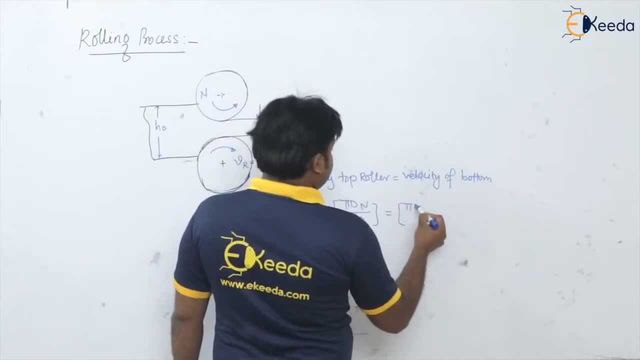 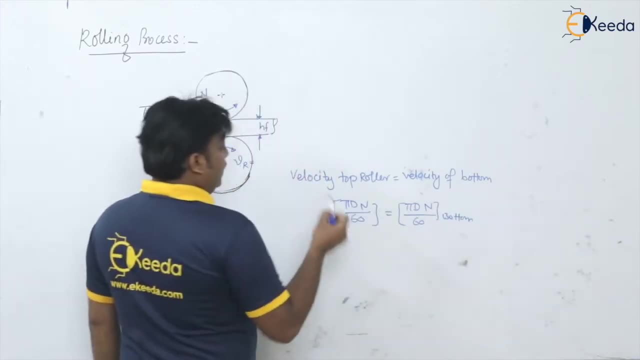 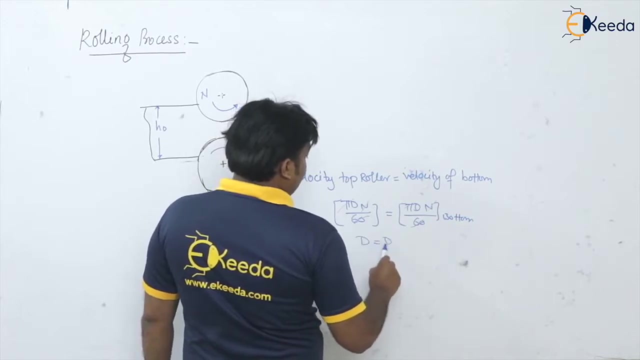 Then it is pi d n by 60.. Okay, Then it's pi d n by 60 for bottom. Okay, So both are rotating with same RPM only, and cancel these all get cancelled. So diameters of the roller or radius of the roller also should be same. 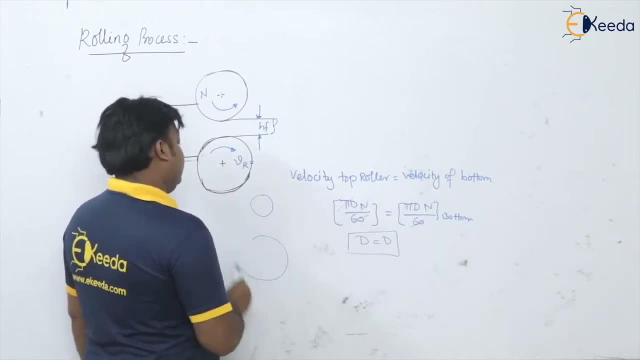 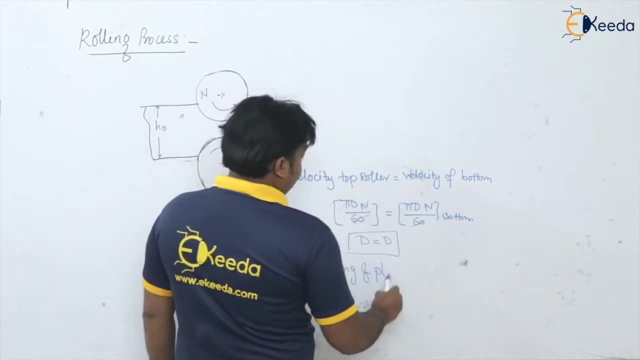 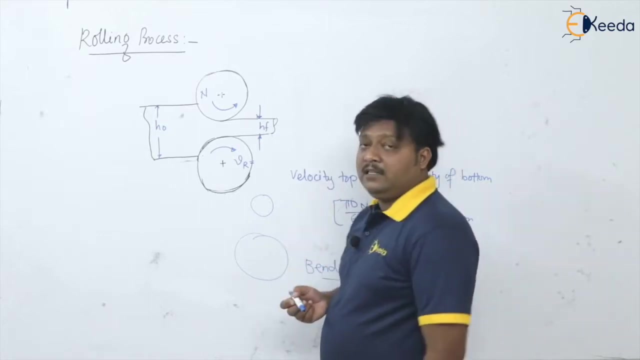 So it is not like that One needs small and another is bigger, Otherwise what will happen? bending off plate? that is going to happen for sure. okay, now what we are assuming here, actually the we are talking for the volume constants, you know. so say the plate is. 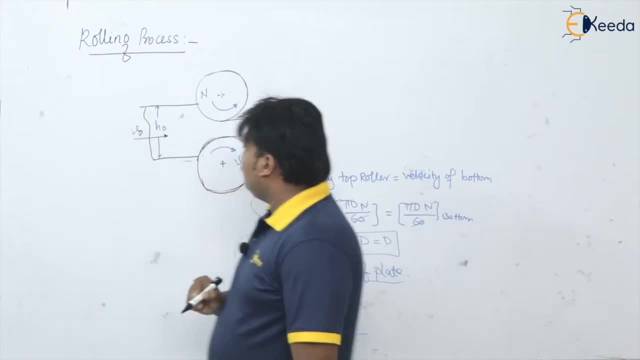 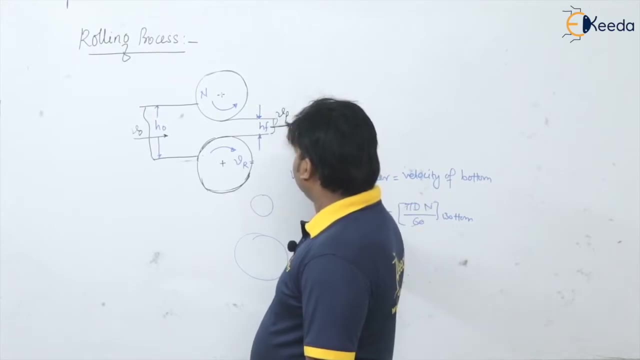 entering with initial velocity V, original, and at the exit it is now moving with the velocity V final. okay, and please remember: R is the roller radius or D is the roller diameter. this is the deformation zone. actually, this is the deformation zone in which the stresses that is induced in the material. 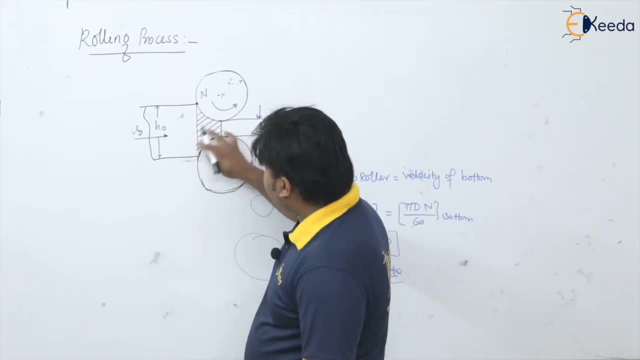 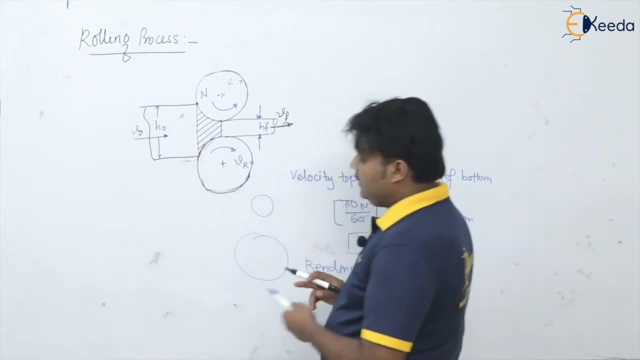 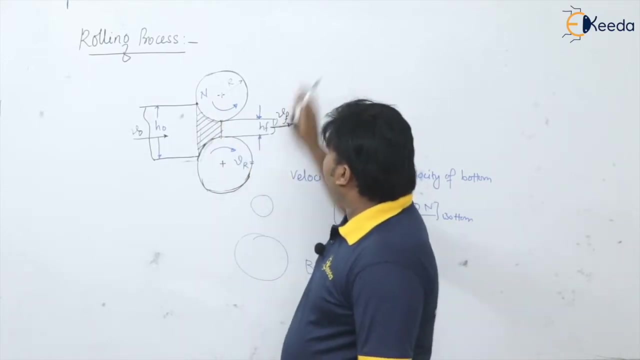 are greater than the yield stress but less than the fracture, isn't it? and of course, these are the huge comprehensive stresses here. that is, this is our deformation zone. now see here: if you apply the volume constancy principle, what is the initial volume flow rate entering into the roller? that is, V naught into B? see if width: initial width. 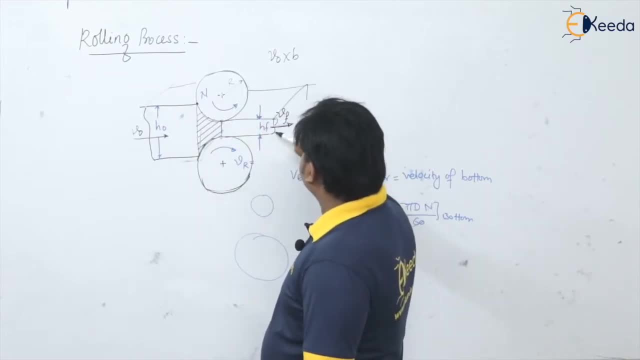 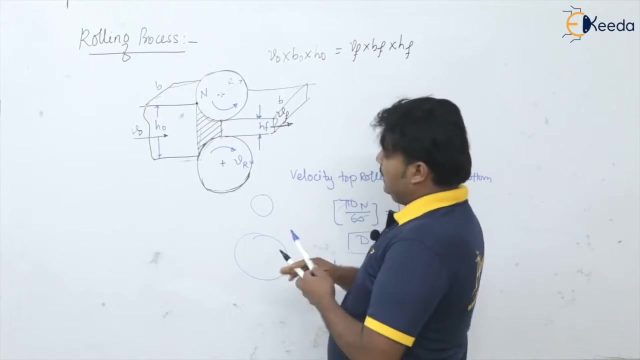 was say B and as the second assumption, that is B, is going to be constant, so b into B, naught into H naught should be equal to V final into B final into H Final, as you know that the end is not going to chain. this is plain sin. 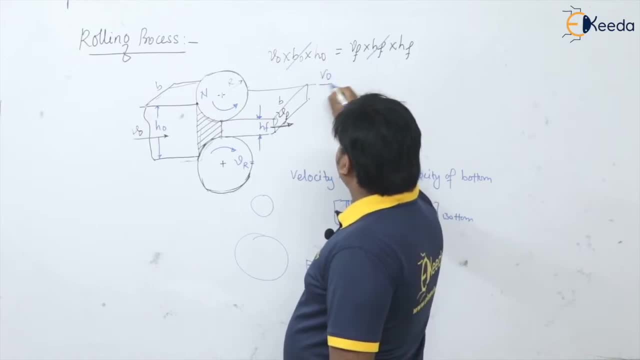 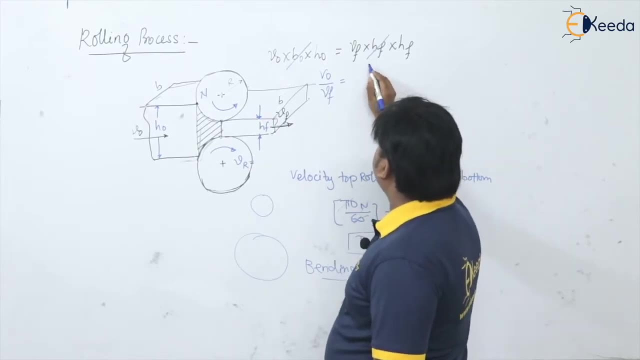 condition, that is, V naught by v final is equal to our ro lot of in a board by the final is equal to what V original divided by V final is equal to was being on this to that condition to reach, which is this: we to what h final divided by h original or v final divided by- sorry, v final divided by v original is. 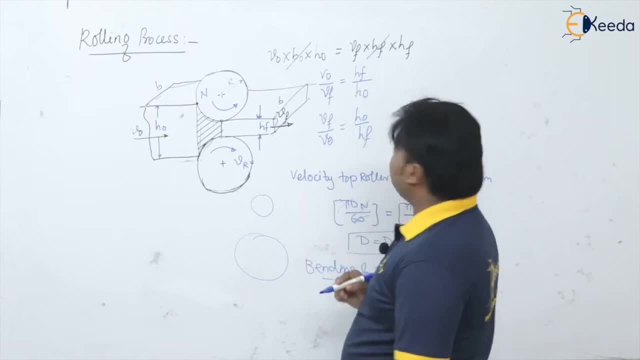 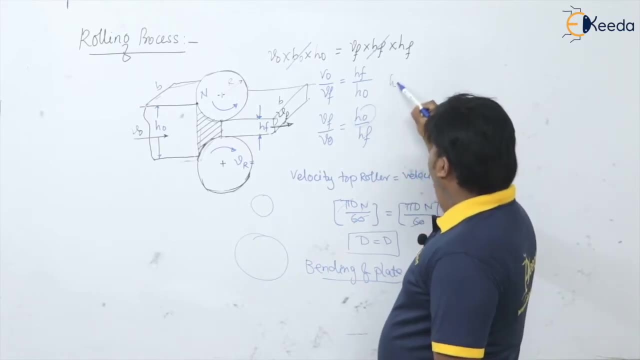 actually h original divided by h final, isn't it? and we know that in rolling operation always we have this: original thickness is greater than the final thickness, isn't it? so this is bigger than this, so of course this ratio will be more than one. so definitely what we can have here, the final. 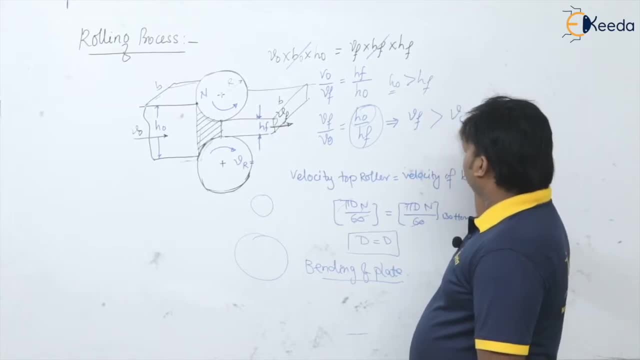 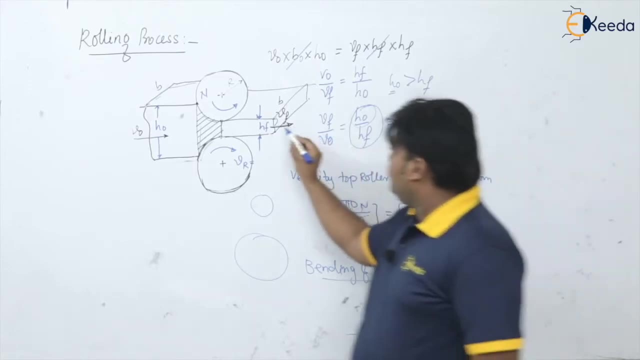 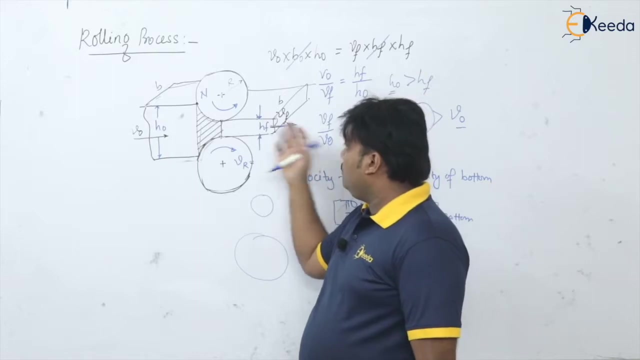 velocity is always greater than the initial velocity for the strip or for the plate. the final velocity of this plate here, that is plate- is coming with the very high velocity. once the it passes the deformation zone it is in, it will show the increase in the velocity, whereas 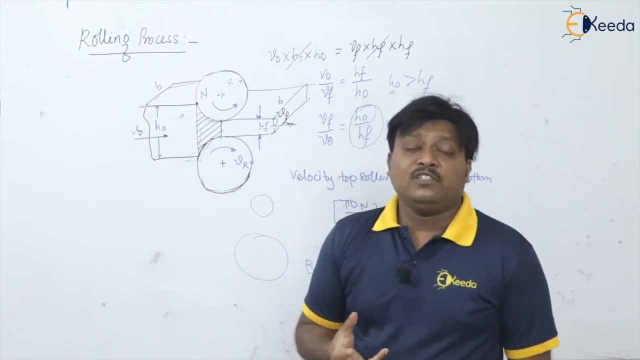 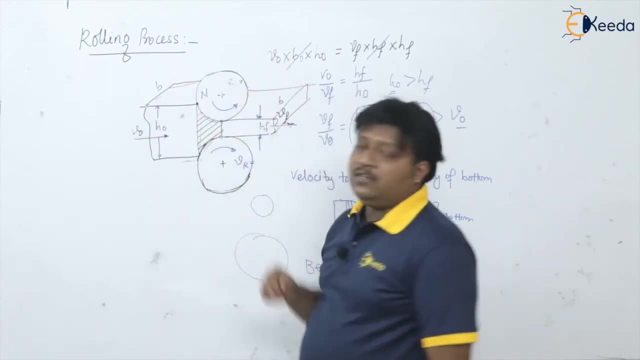 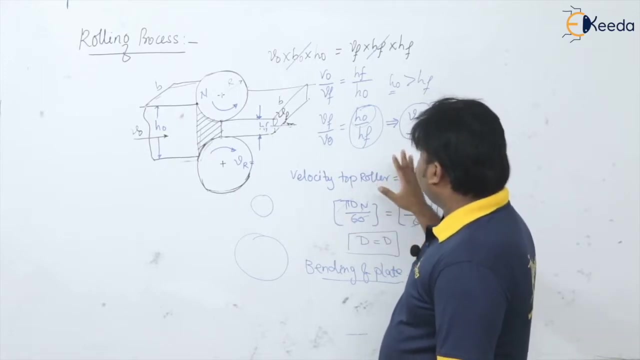 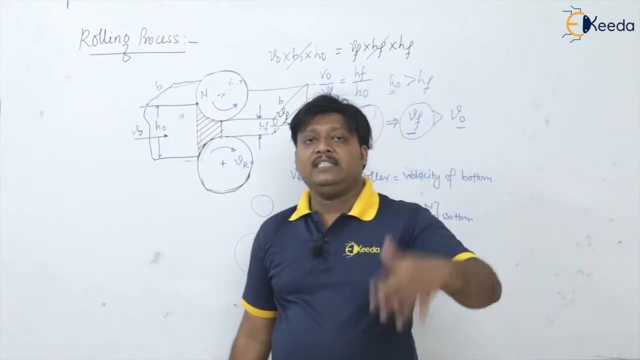 initial, initially the strip velocity was very less, but in entire operation the velocity of the roller was constant. Now, from this point, what we can have from this discussion? we can prove this mathematically: that velocity of the plate at the exit point is more than the velocity of the plate or strip at 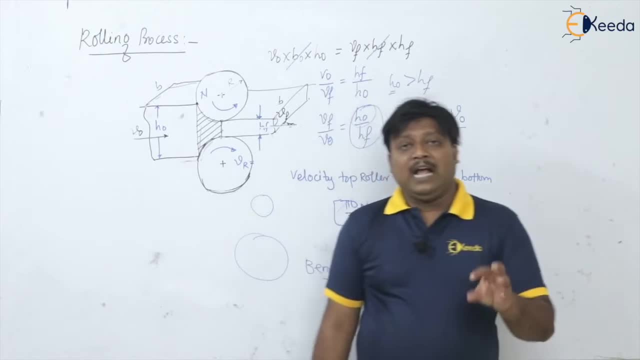 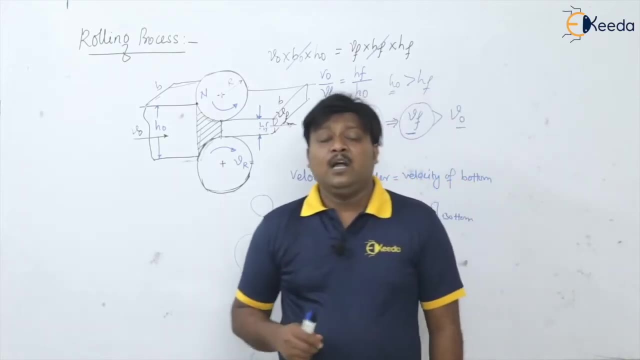 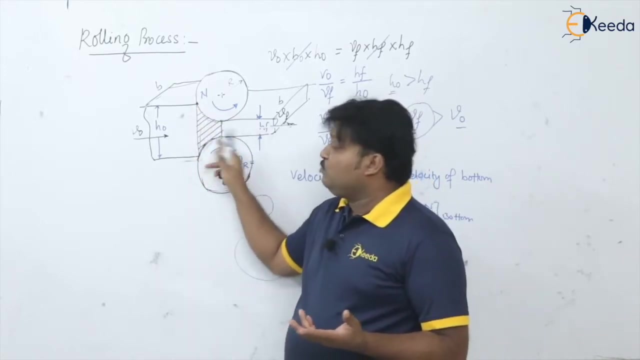 the entry point. we can say like this: but what actually happened physically is, that's why this material or that plate shown the increase in the velocity. what is the reason behind that? so the reason is very same: that because of this huge amount of compressive stresses, the pure flow. 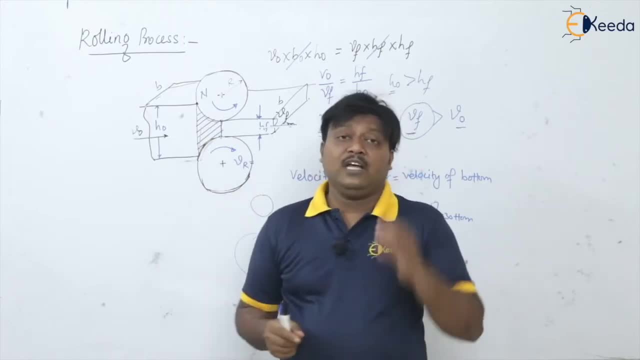 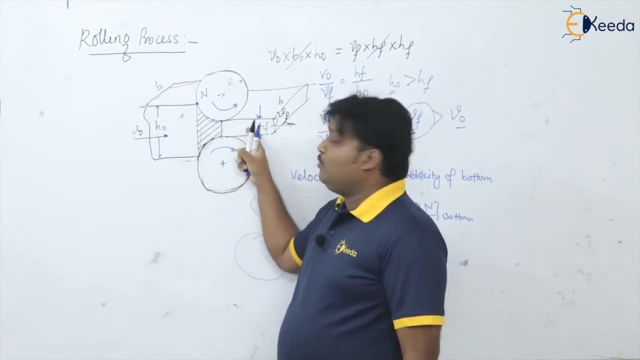 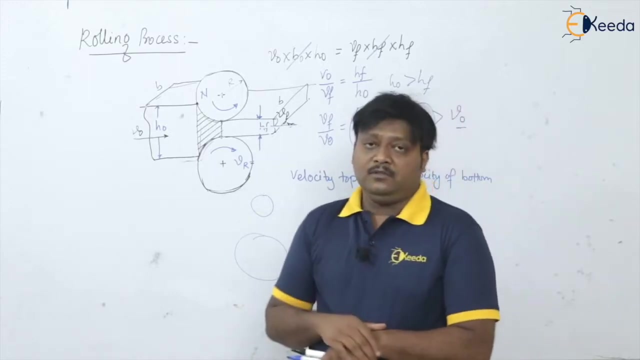 stress was get induced in the material and because that, because of that, the material now flowing like liquid. so after passing through this deformation, that's why it is- the plate is having the maximum velocity at the exit point than the entry point. okay, so, students, if we talk about the relationship between 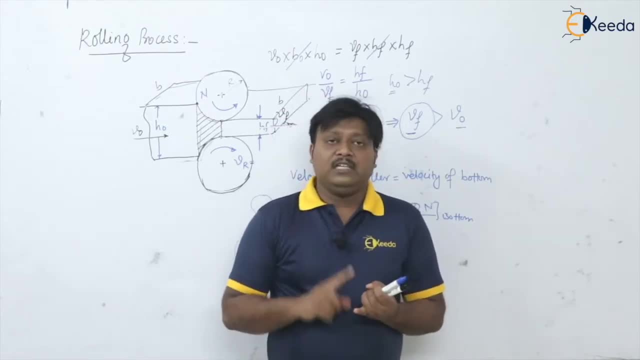 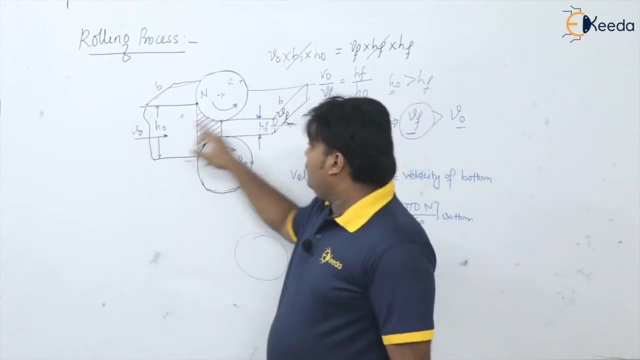 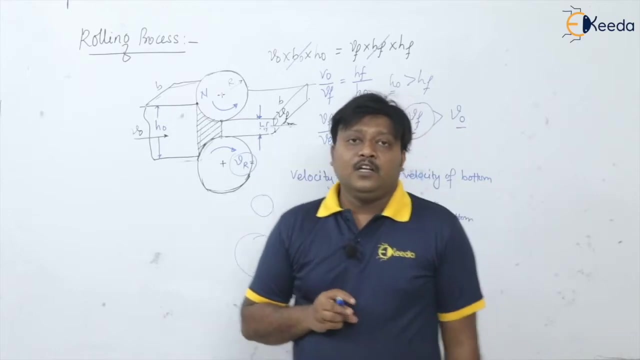 the linear velocities. if we talk about the relation for the linear velocities, that is, the velocity of the strip or plate at the entry point, the velocity of the plate at the exit point and the roller velocity vr and the roller velocity vr. so what can be the relation? so initially the 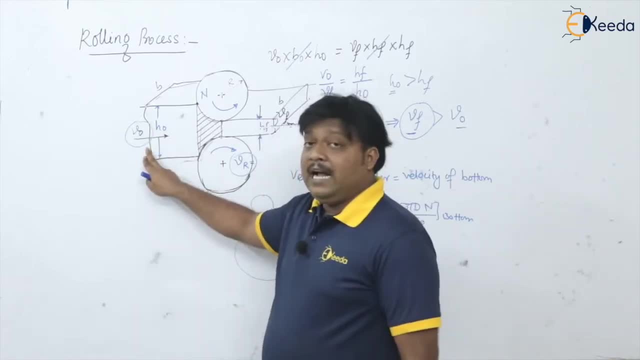 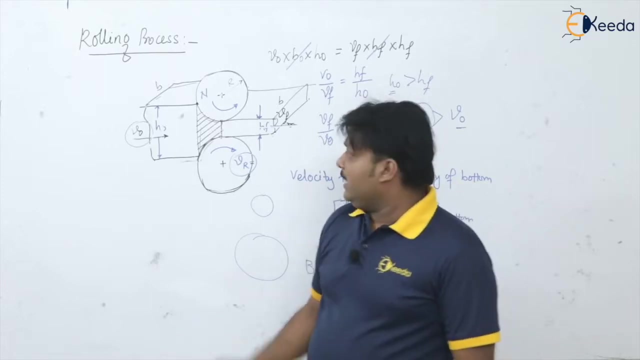 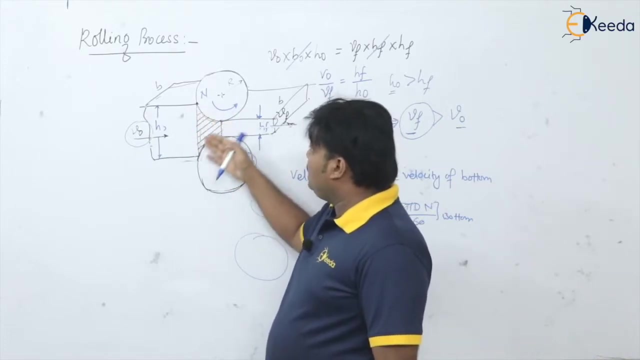 plate velocity was very less okay at the entry point. roller is rotating with its constant velocity, constant rpm, okay. so definitely, initially the velocity of the plate was less than the velocity of the roller. okay. now, as the material is going into the roller, as it is getting deformed between the two rollers, its velocity goes on increasing at the 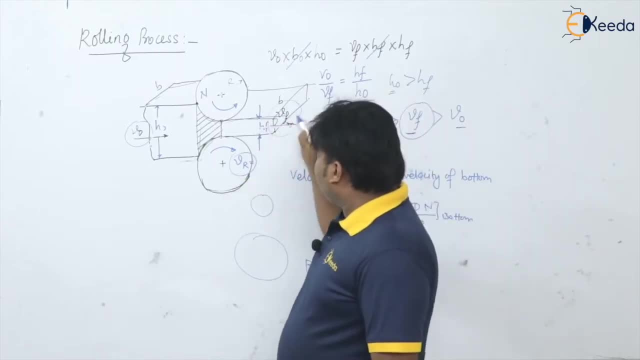 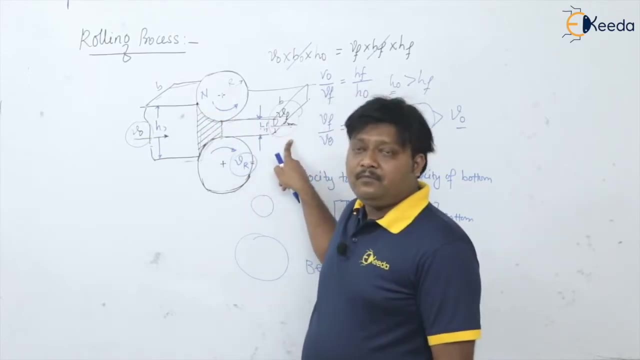 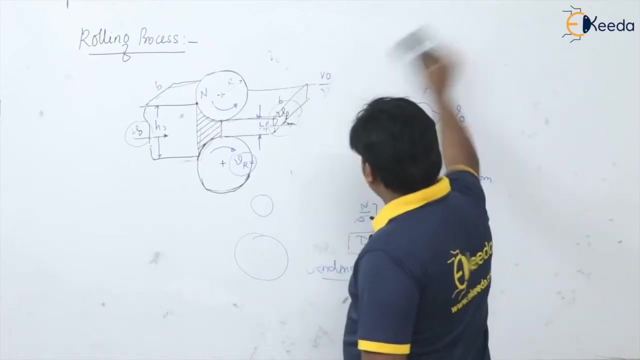 end point, isn't it where, at the exit point, this velocity of the strip is now again more than the velocity of roller. so if you write the relation for, if you write the relation for the velocities or the linear velocities, we can simply write the relation for the linear velocities. we can simply 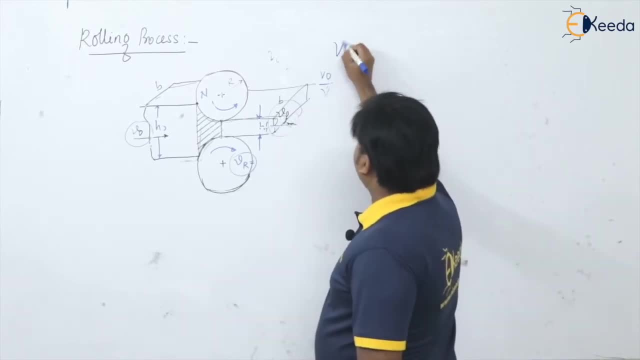 write that. so initial velocity of the plate is lesser than the roller velocity, which is again lesser than the final velocity of the strip. please remember, this is a very important thing we got here, isn't it? that is the relationship between the linear velocities. now, at the same time, if you 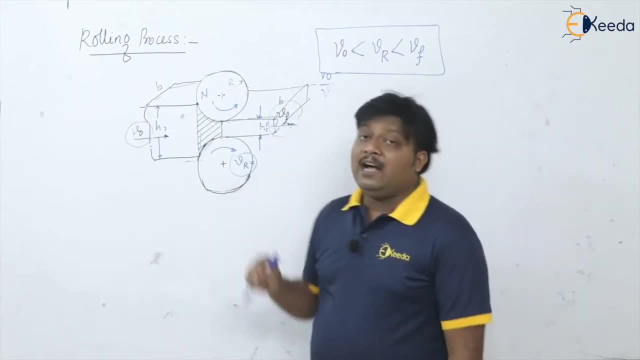 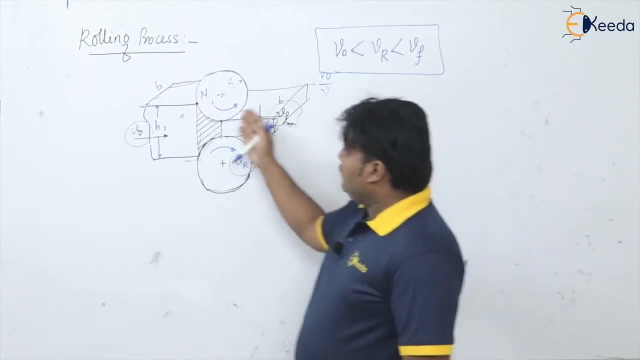 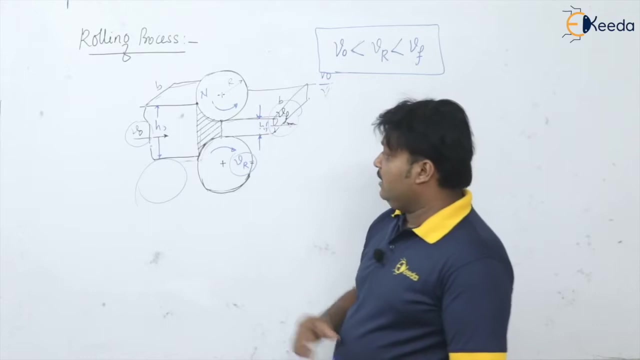 are having the relation for the linear velocities. you can write the relation for the linear velocities. then can we have the relationship between the relative velocities? okay, so of course, if I talk about this relative velocity at the beginning of the process. so again, there was a huge amount of 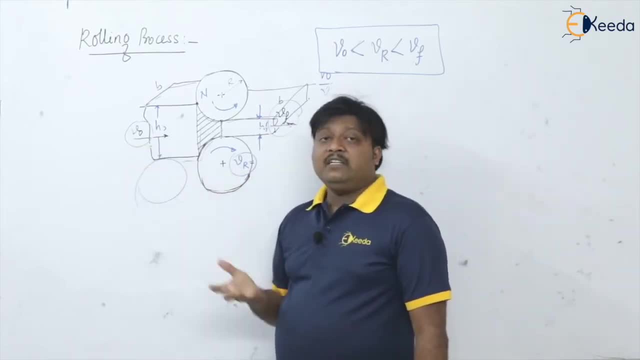 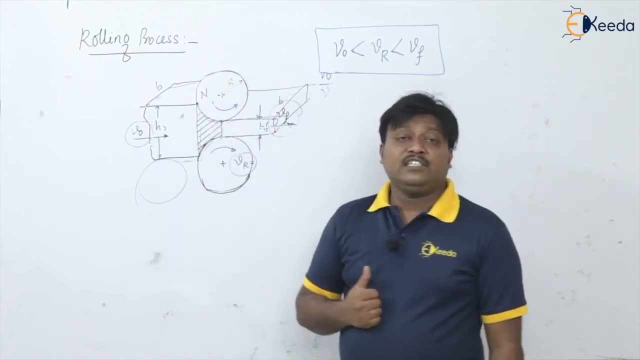 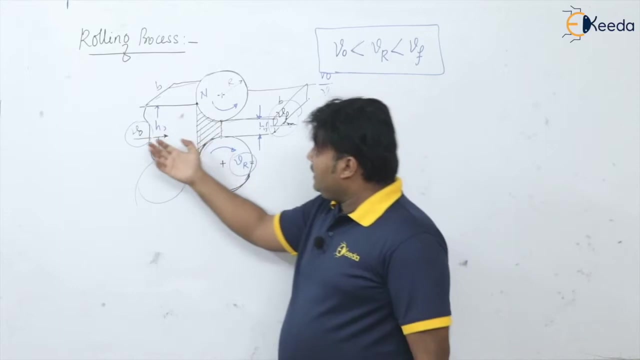 relative velocity because at the beginning strip was having very less velocity but rpm. sorry, but ruler was having much more velocity than this strip velocity. so definitely at the beginning of the process the there is existence of quite huge relative velocity, isn't it now? what will happen when this strip is now coming into the ruler? definitely when it is coming into. 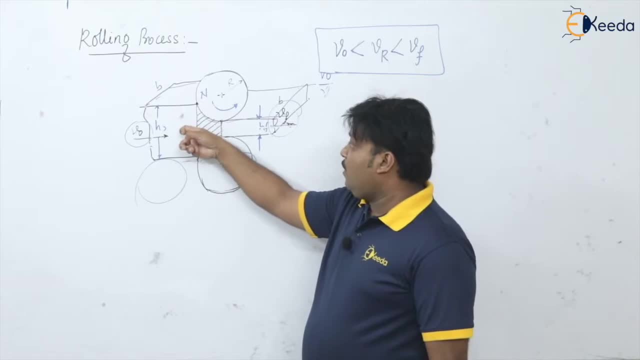 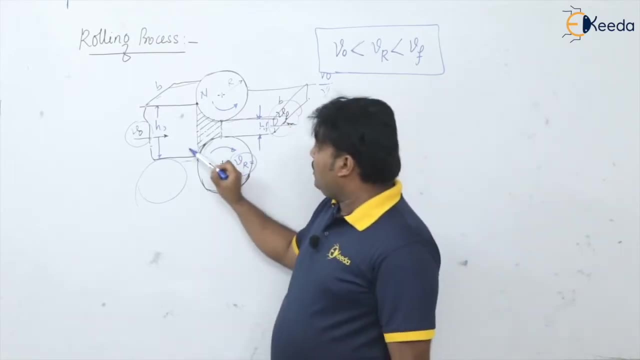 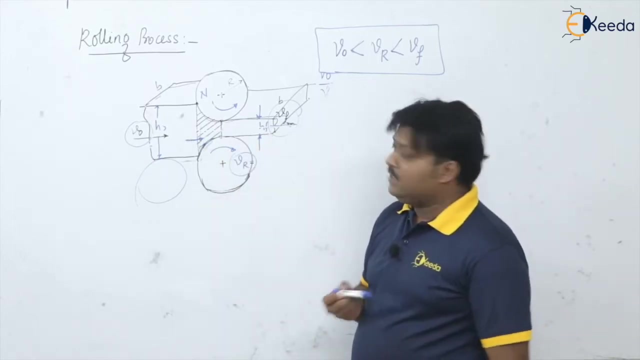 the roller. now the velocity of the plate is decreasing. now the velocity is decreasing, you or strip is going to increase, okay, so now it is gone, increasing into the deformation zone, isn't it? and at particular point, same case in linear velocity also, but here I am saying that at particular point. what happened? the 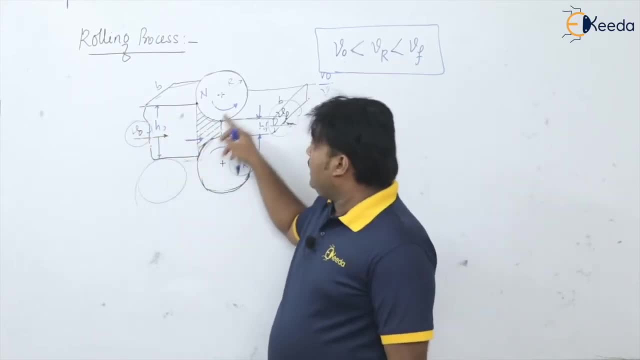 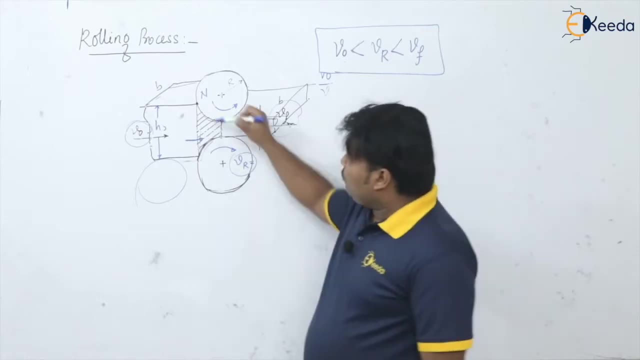 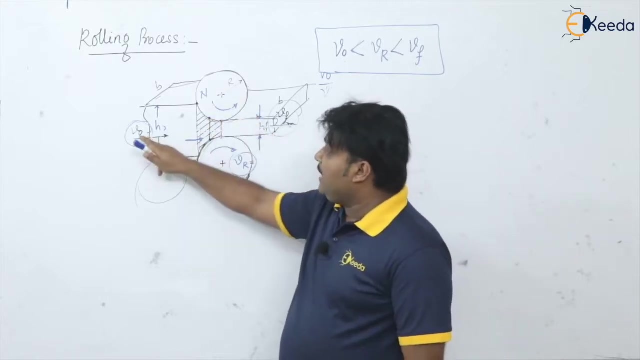 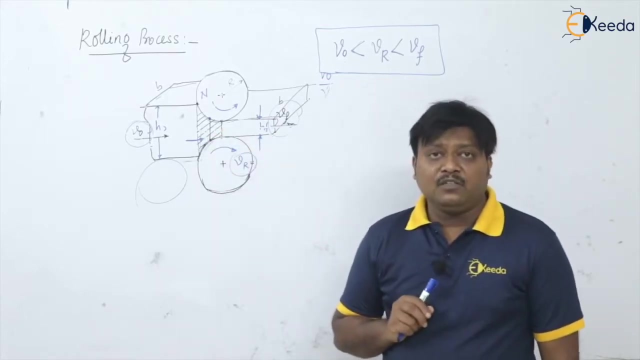 velocity of the strip and the velocity of the roller get matched with each other, get equal. okay, so at that point, what will happen? say this: is that point where the roller velocity get match with the velocity of that strip, that at that point, what is the relative velocity? both velocities are same, so definitely what? 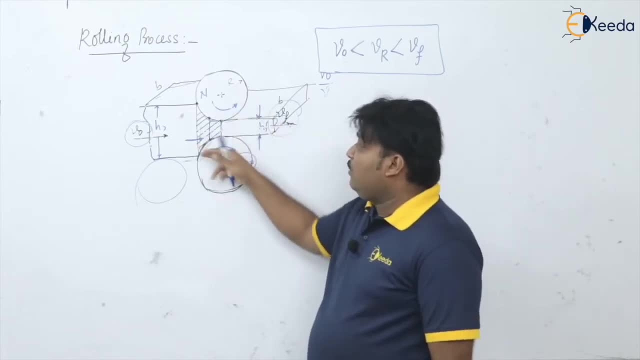 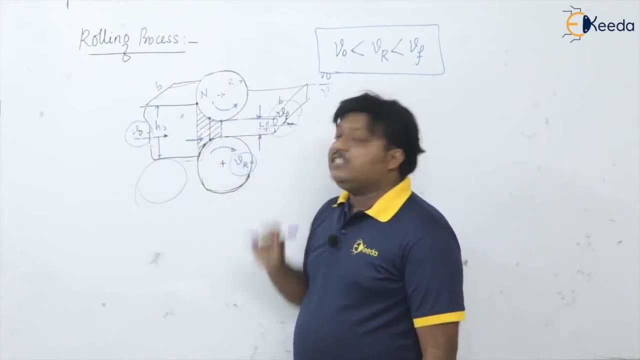 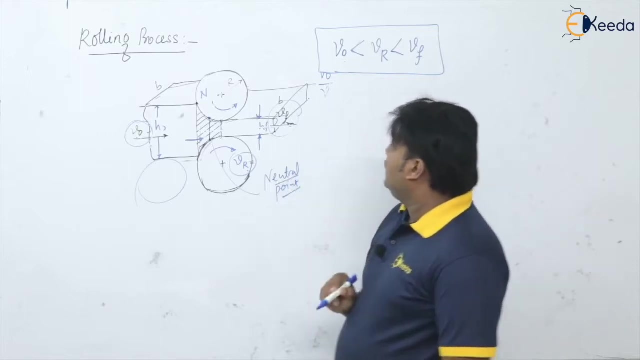 happened there. there will be the zero velocity. okay, at that particular point, where a vo is equal to vr, the velocity will match with the velocity of the อยetty. velocity at that point got zero and that point in the deformation zone in the rolling process is known as the neutral point. as the neutral point okay. 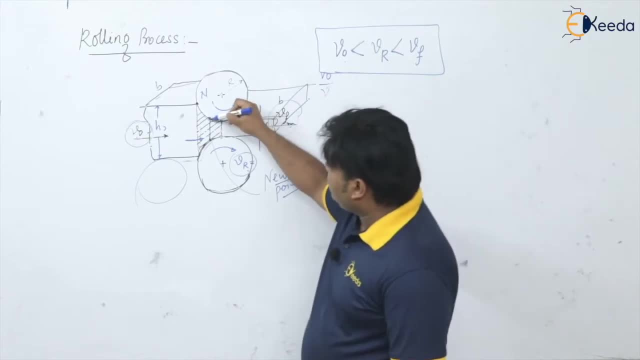 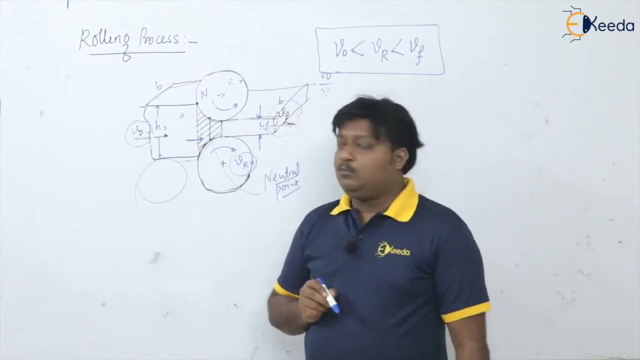 so here also at some moment in linear velocities also, the linear velocity of plate get matched with the linear velocity of ruler. that point was a neutral point here with the relative velocity where the lower rate of deflection z is that point. so that is what this Geminies over here got��. 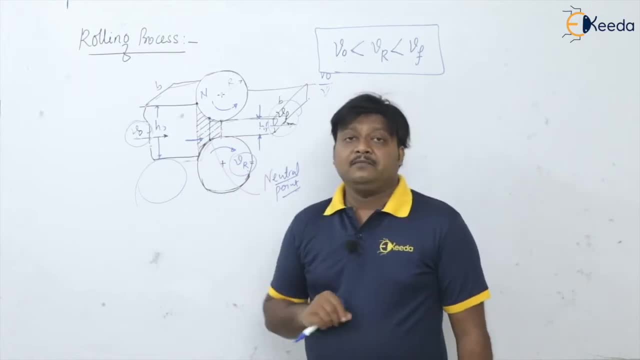 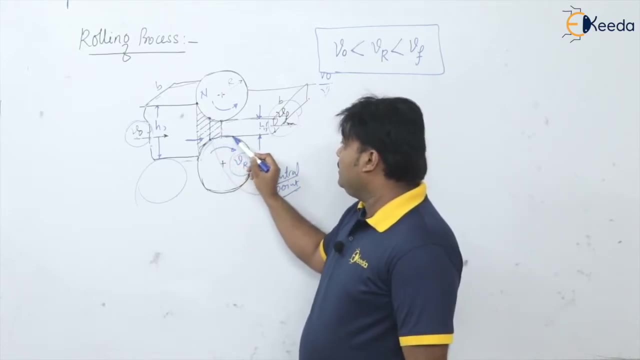 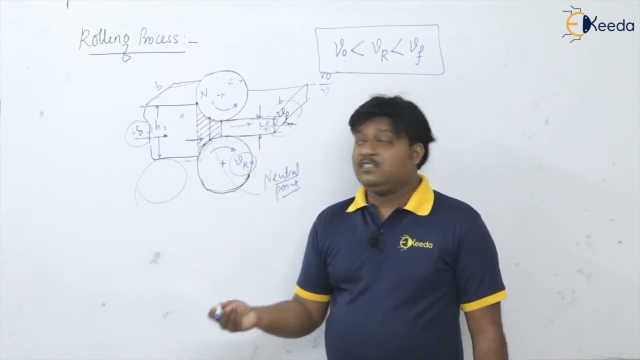 the relative velocity is zero. that is the neutral point. okay, now, once the neutral point get passed by the strip, again what happened? as we know that, because of the flow stresses, it is moving with quite larger velocity than the roller, isn't it? and it will get the maximum at the end, so definitely. 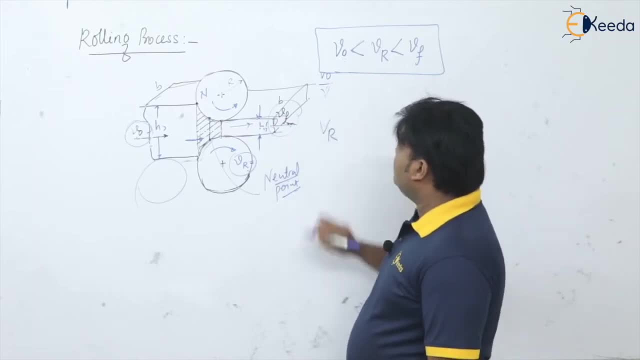 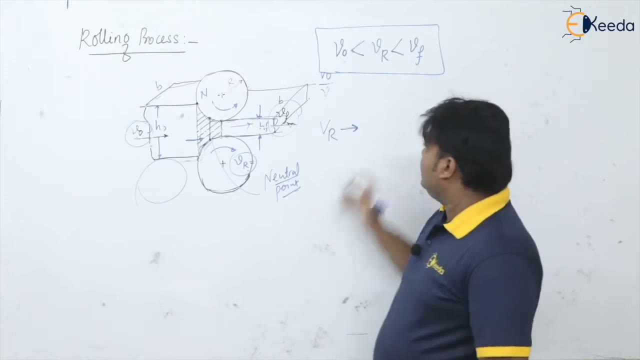 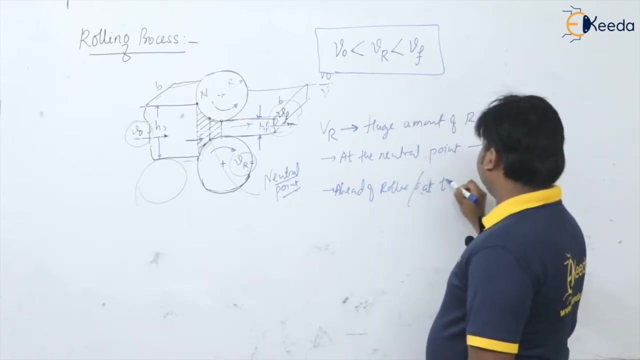 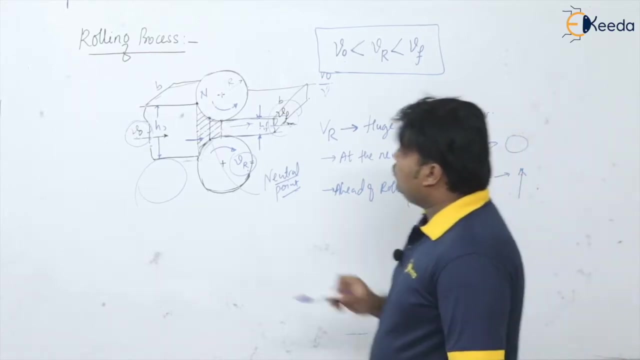 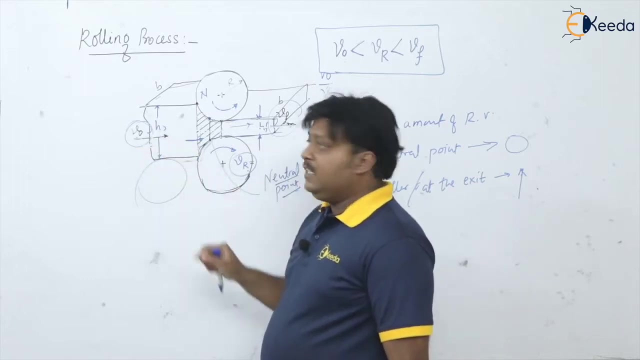 now the relative velocity was again initially. huge amount of relative velocity at the beginning, huge amount of relative velocity, but at the neutral point it is get the zero and ahead of roller, ahead of roller, or at the exit. at the exit it again goes on increasing. okay, so initially said, if we take this velocity of roller with respect to the plate, then there is a 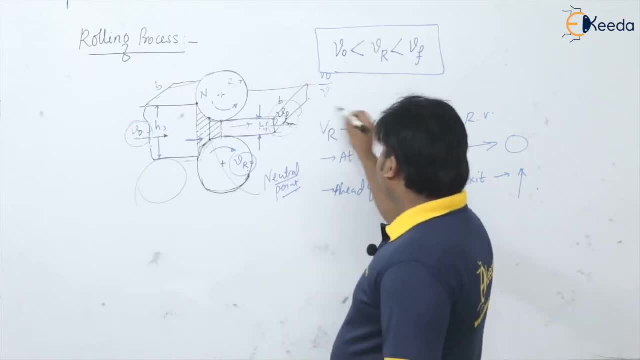 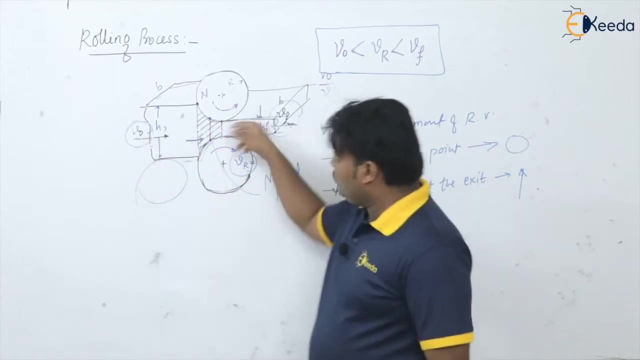 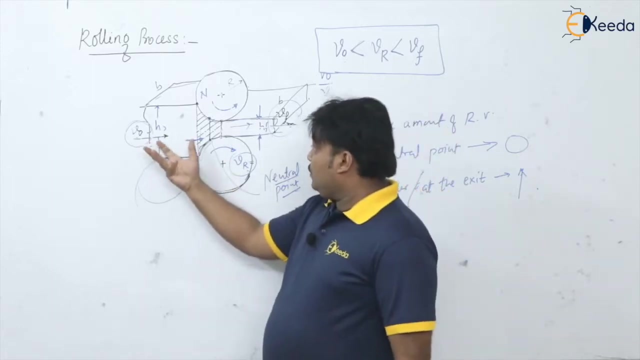 initially you can have the large positive relative velocity, isn't it? because roller velocity- i am taking roller with respect to plate, because roller is moving with the high speed than this uh strip velocity- then, definitely so at the beginning, we can have the huge amount of positive relative velocity. okay, so it was positive. now it is coming down, down, down at. 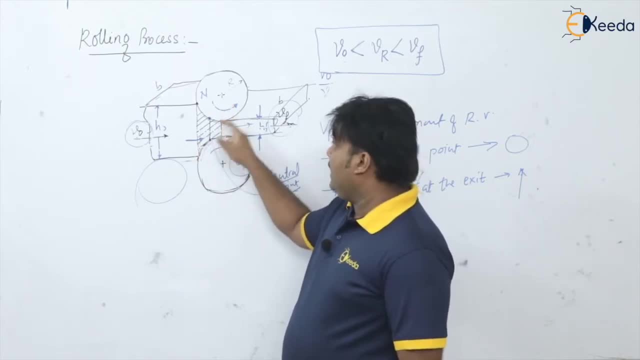 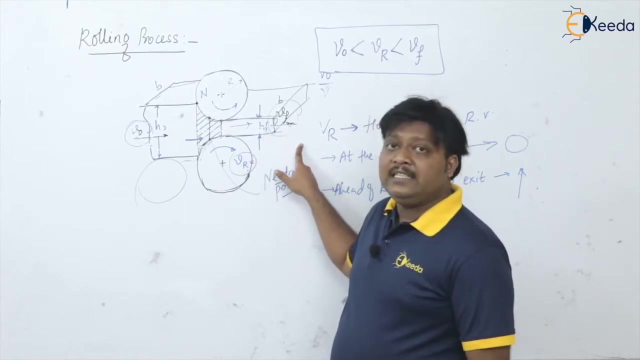 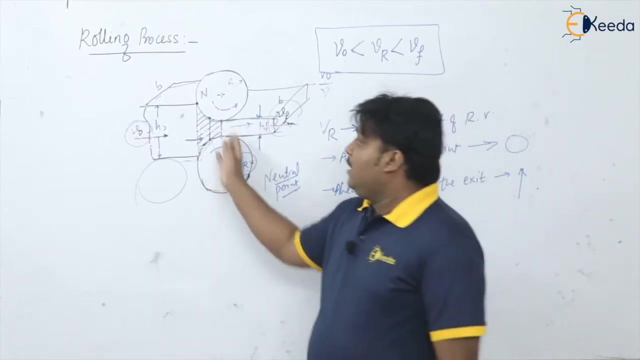 neutral point becomes zero. and now, ahead of roller, at the exit zone, what happened? plate is moving with high speed. so, with respect to roller, the relative velocity of roller, with respect to now the plate at the exit, is what? this large amount of what negative relative velocity will exist, please remember, or we can have the velocity, relative velocity plate with respect to: 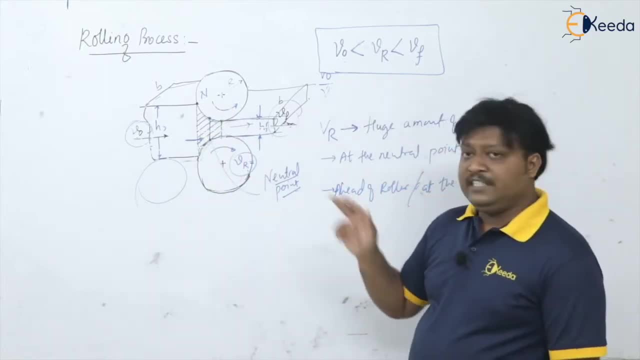 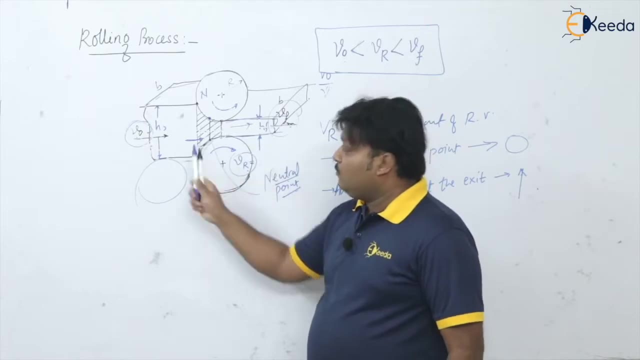 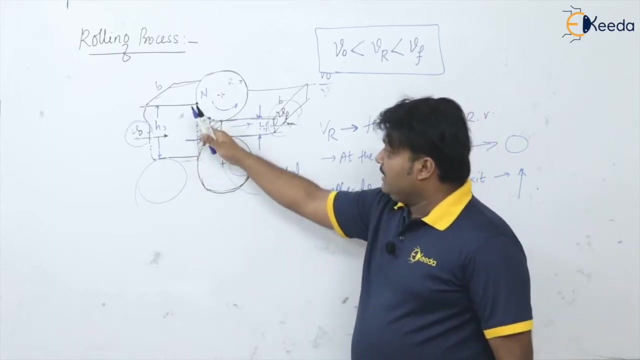 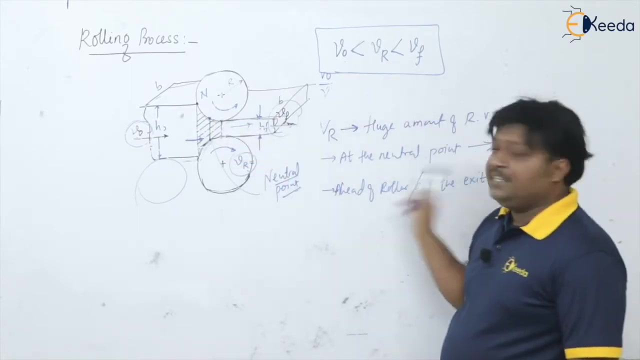 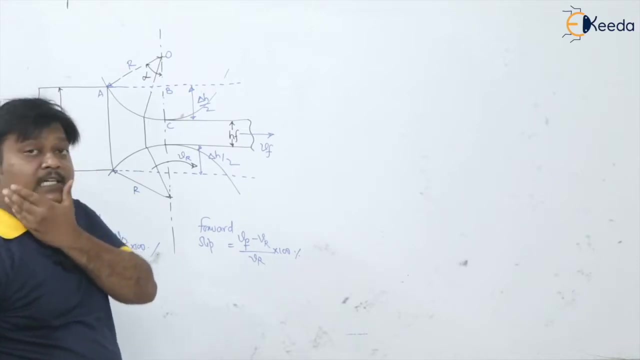 roller. then also, initially it is negative. at the exit you will get it is positive. okay, anyhow, we can uh have the statements for the relative velocity. okay, so please remember, relative velocity goes on increasing, at the beginning at zero, neutral point with zero, and again okay, okay, fine, now, uh, i have drawn the little bit detailed diagram of this rolling 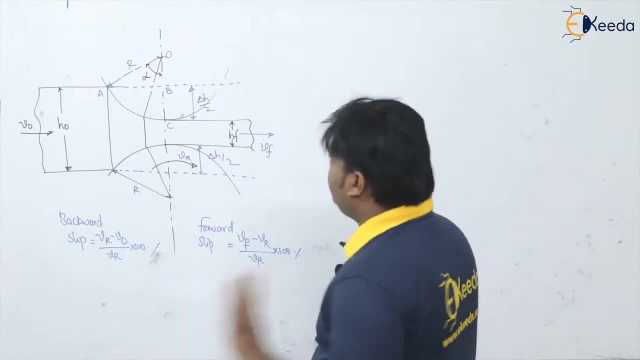 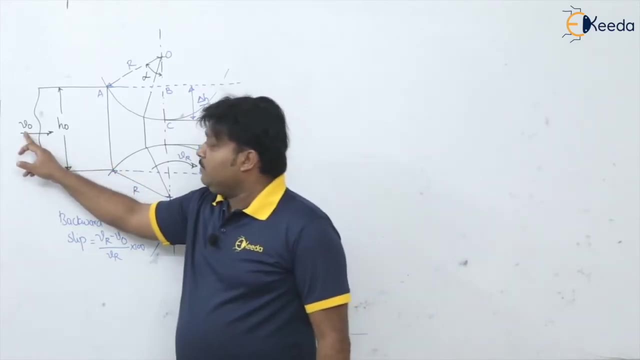 operation. so see here the same thing. that are not. i'm going to- uh, i will not write actually. so what is v? we will stand for velocity, h will stand for the thickness. okay, o, that is the v o, h. o. these are the initial parameters, or the beginning. 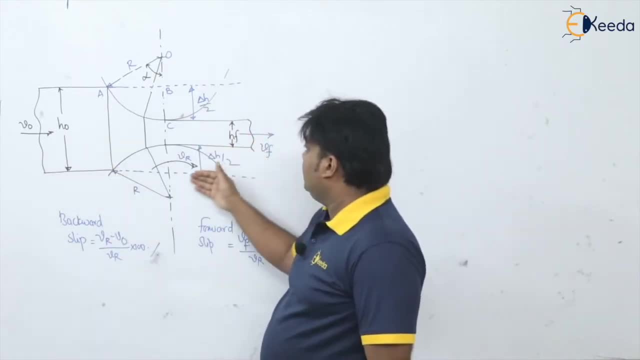 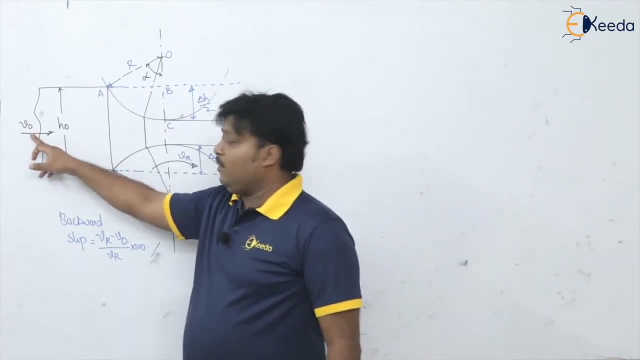 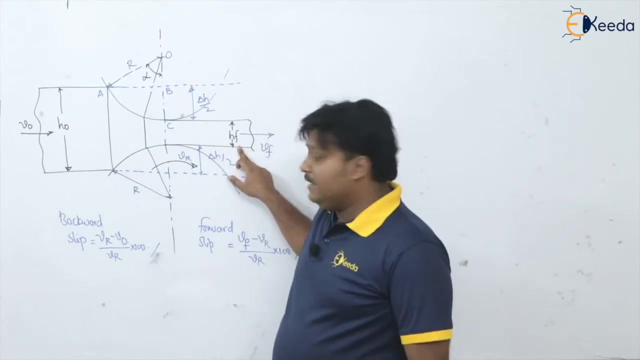 parameters. okay, and f will be the at the final or at the end or at the exit. so v? o is the initial parameter, h? o is the original height of the strip or original thickness of the strip, h? f is the final thickness of the strip and final velocity of the strip is v? f. v? r is going to be the roll. 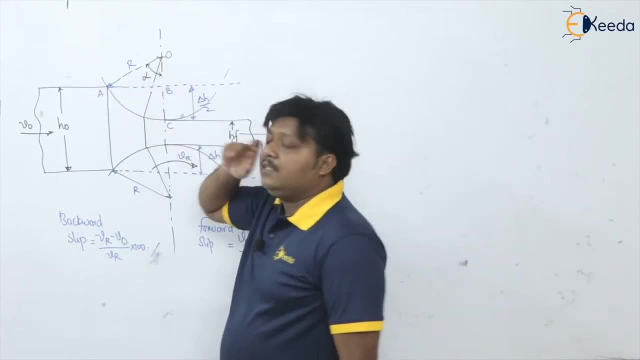 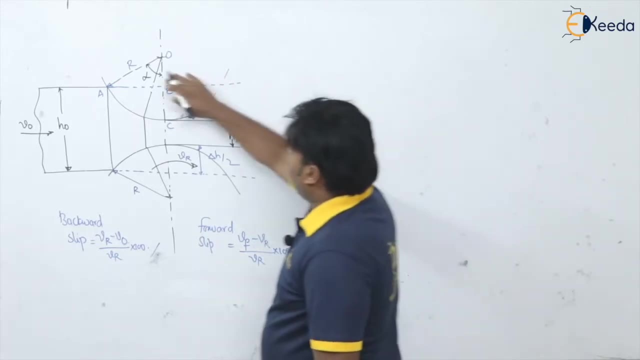 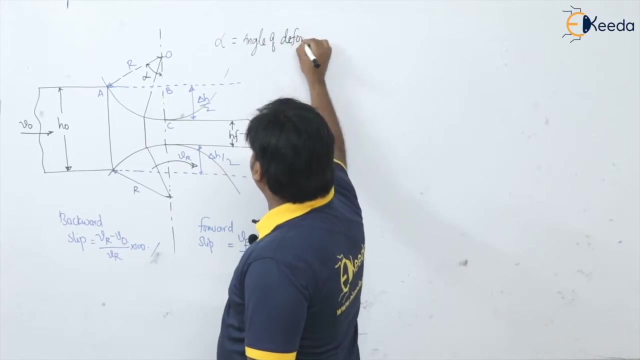 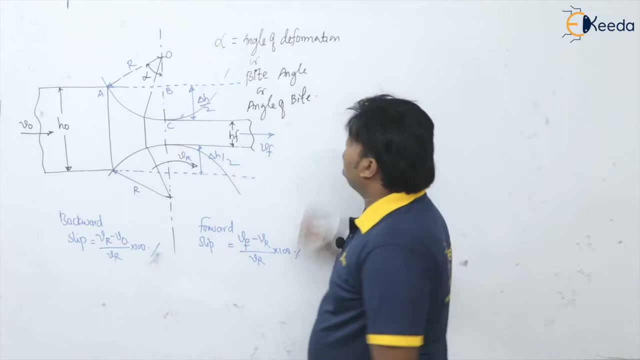 velocity and r is what the radius of the roll. okay, so see here again. i want to write here alpha. alpha is what. alpha is known as the angle of deformation, angle of deformation, or it is also known as the bite angle or angle of bite, angle of bite. please note this. okay now. 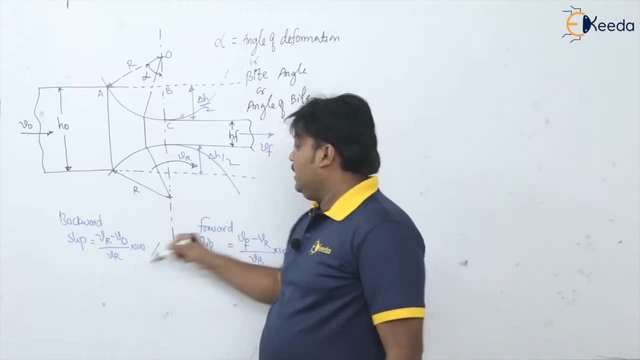 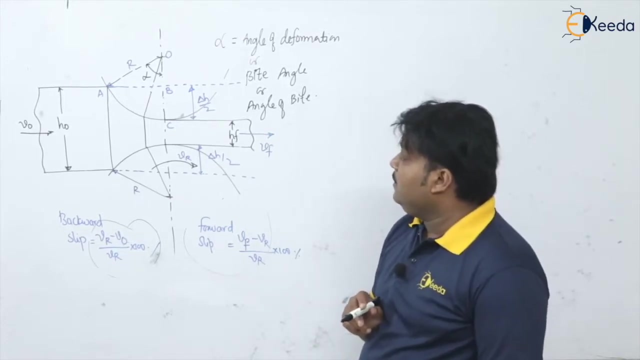 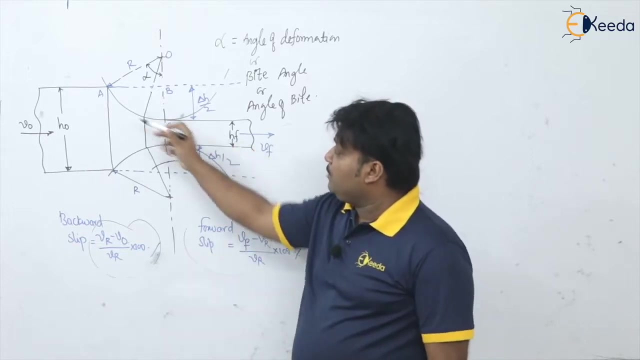 you can have the, the forward slip and the backward slip. we can calculate with these formulas. okay, one thing definitely we'll discuss about: the slip and pressure are inversely proportional and the plate is going to have the self-entry because of the friction present at the plate surface and the roller surface. 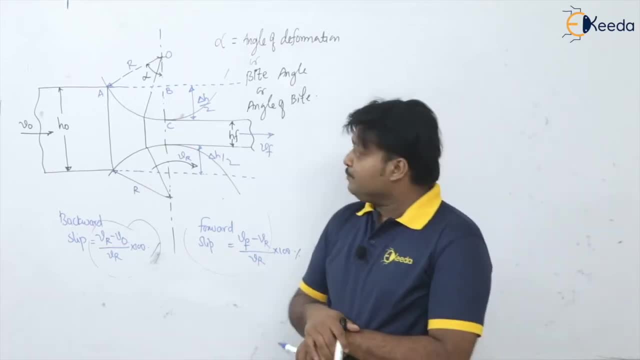 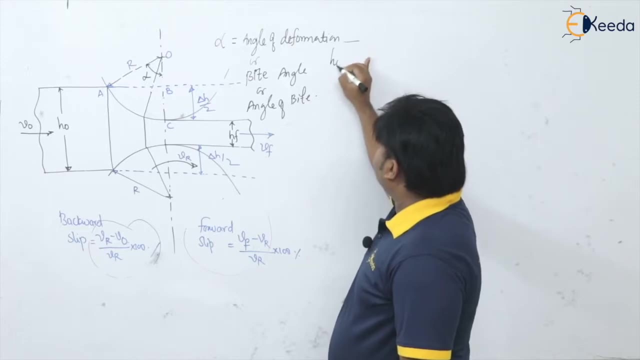 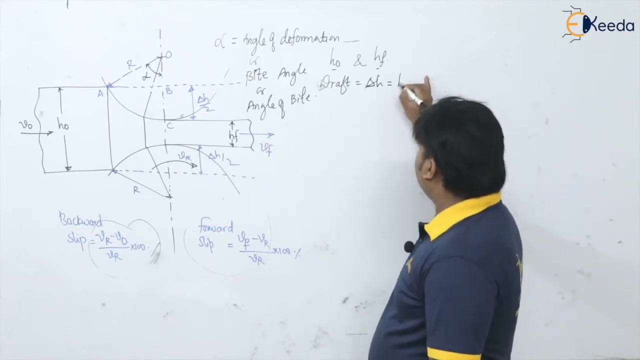 So plate is going to have the self-entry. Now you can see here: initial thickness HO and the final thickness HF. okay, So the difference between these two thicknesses is called it as a draft, the draft that is given as the delta H. okay, which is equal to HO original minus H final. 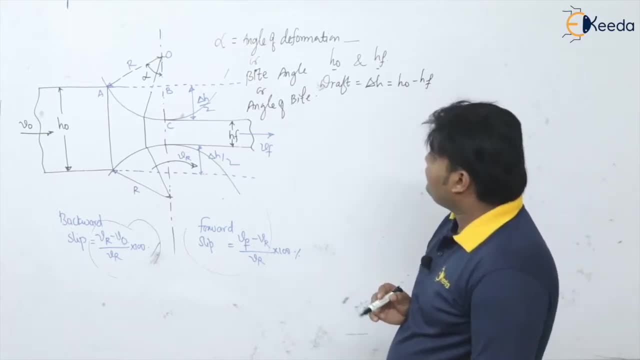 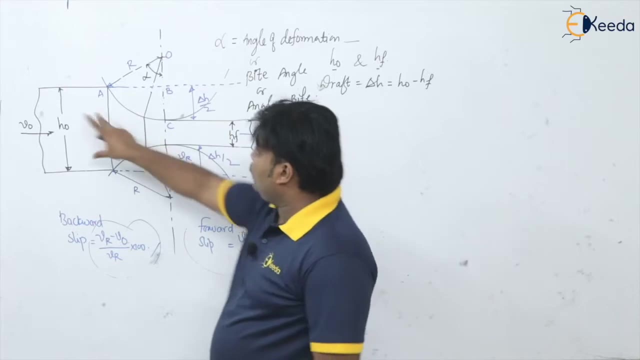 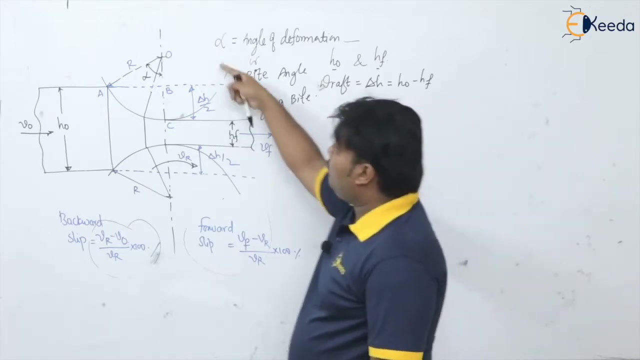 Okay, now you can see here from the diagram. this is the draft we are getting here. original height may say final height, minus ho gayi. So jo delta H mila. wo top roller ke liye kaha hai: kitna hai yaha pi mila, jo ditna mila. 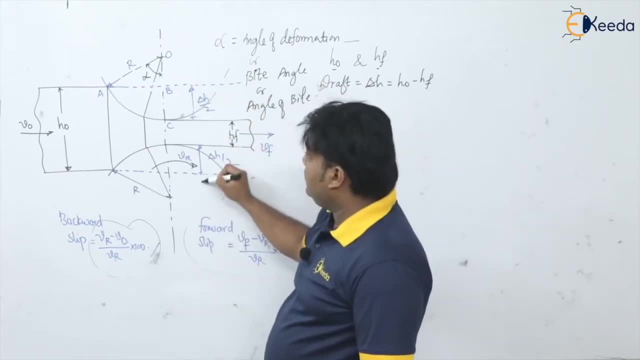 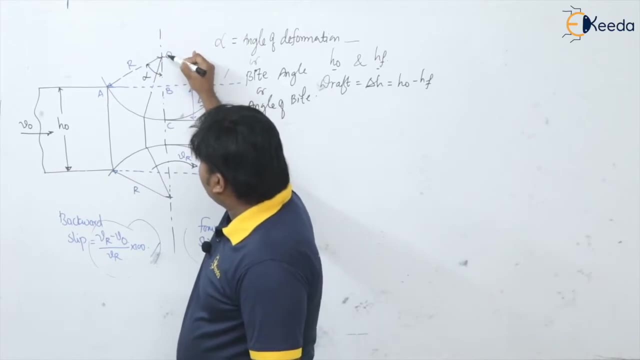 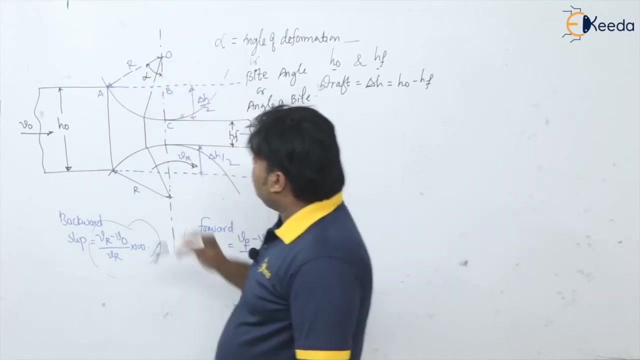 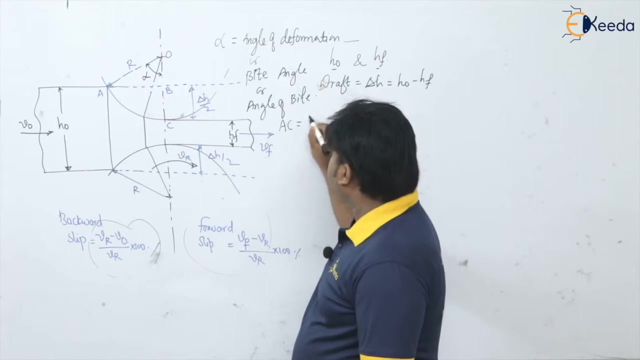 uska aa ghaan. so that is delta H by 2 and this distance is delta H by 2, okay, And see, here You can have this OAB. this is a right angle triangle, isn't it? And this AC, this AC, very important. this AC is known as the arc of deformation, very 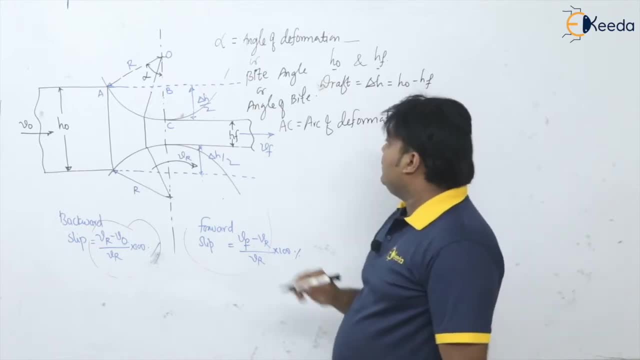 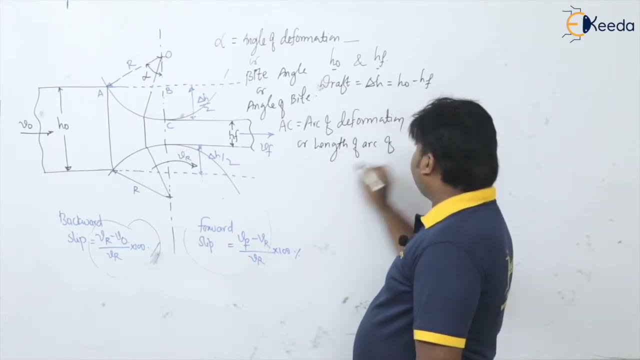 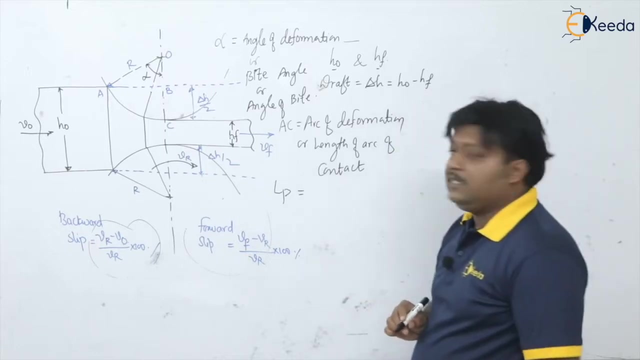 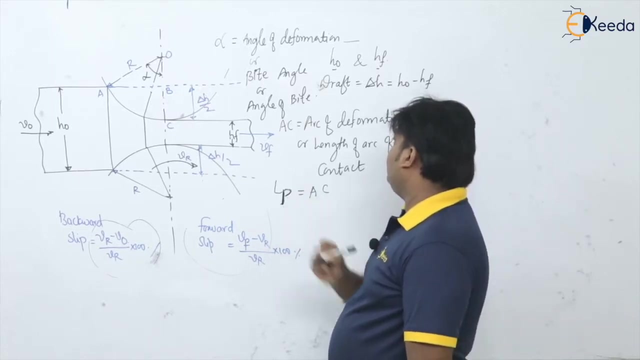 important, many times question asked: or length of arc of contour. Kya bolte isko AC ko, which is generally represented by LP, which is represented by LP, is nothing but our AC length of arc of contact or length of deformation. 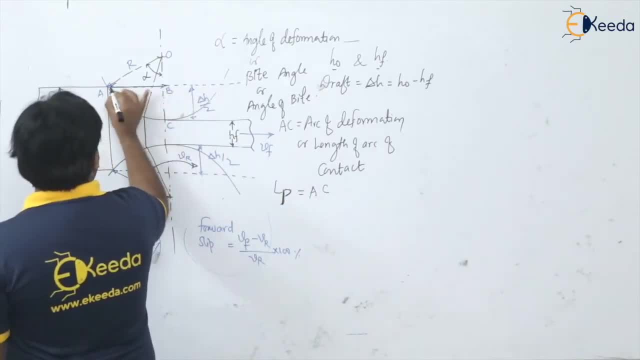 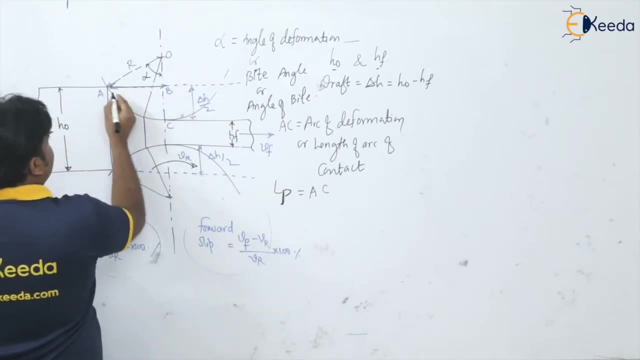 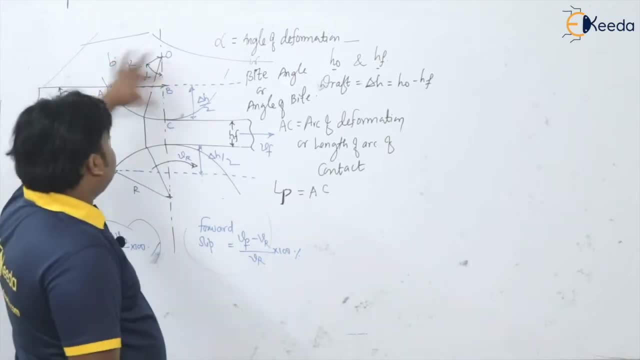 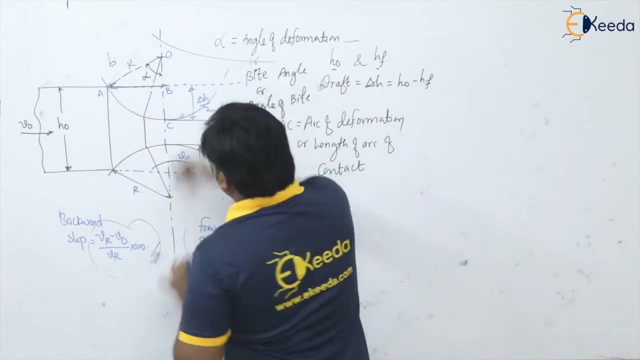 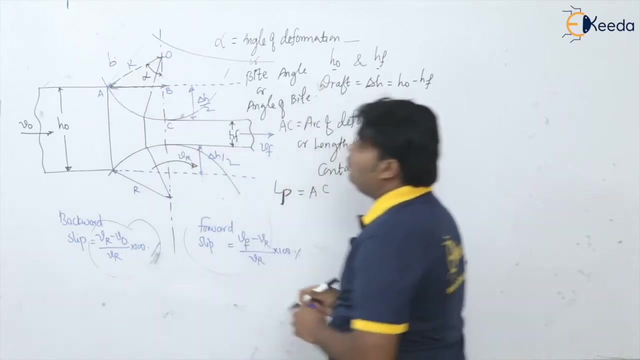 Okay, Okay, We'll get the projected area or contact area to find out the pressure actually. Okay, So let us see in this diagram. see again: OC is again what R. OC is nothing but the radius of roller. OA is again the radius of roller. 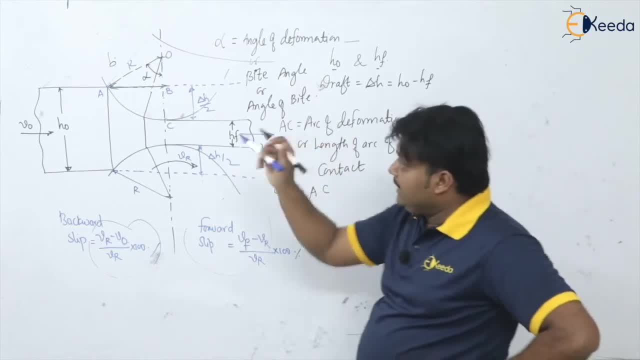 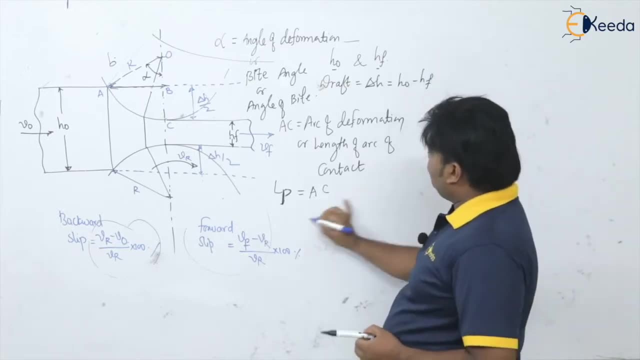 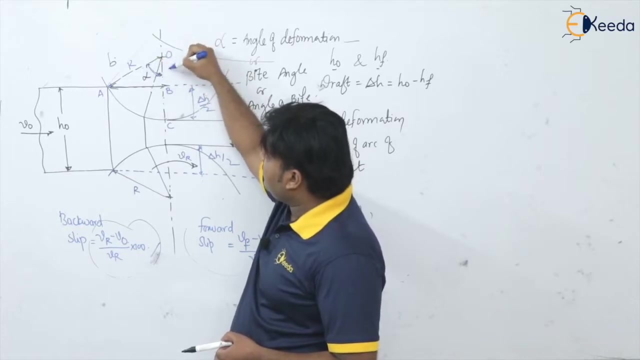 So in right angle triangle OA, OBC. in right angle triangle, OBC, tell me what is the cos alpha. So in triangle OBA, ABO, may please tell me what is cos alpha is equal to? for this is the bitangle. okay, cos alpha, adjacent side divided by hypotenuse. so OB divided by: 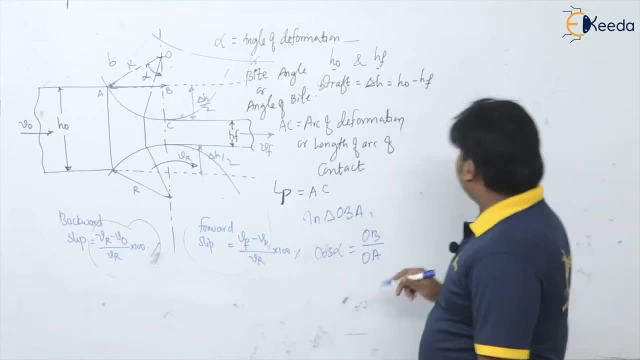 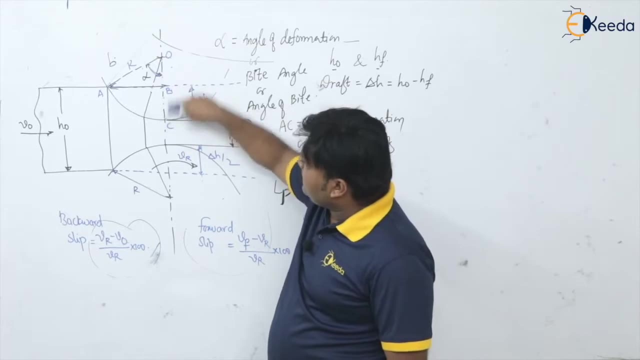 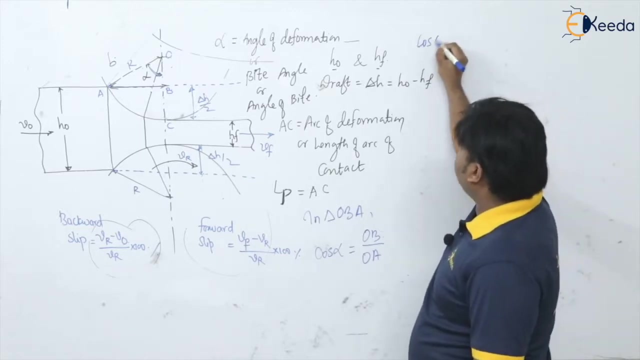 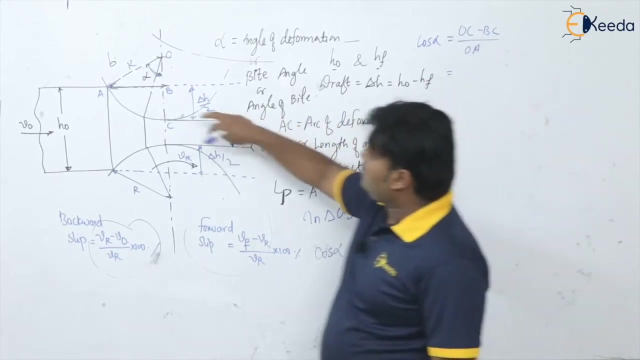 OA, isn't it? so what we can write for OB, OB, how we can get OB, if you minus BC from the OC, OC may say other BC, Nika, the other camera, OBA. so cos alpha, we can write it as OC minus BC divided by OA, and you know that OC is what OC is. 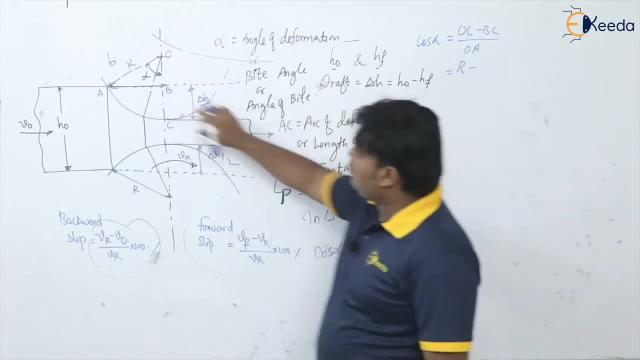 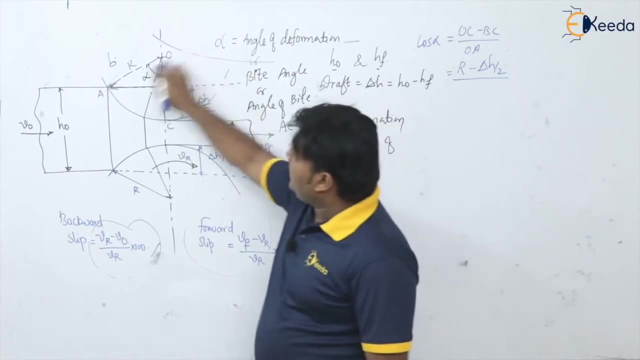 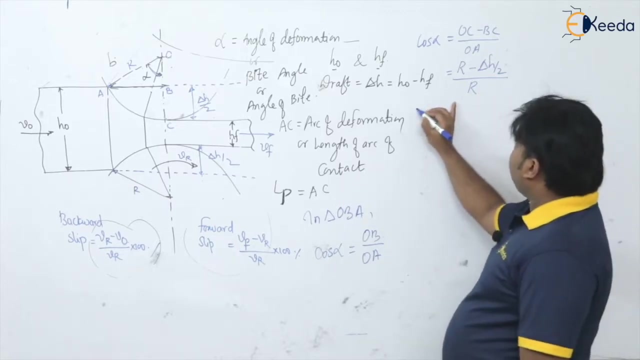 nothing but the roller radius. R minus BC. is what BC? is this half the draft value Delta H by 2 divided by OA. again what it is. please, students, see here very carefully, so tell me. I can write: R cos alpha is equal to R minus Delta H by 2 or Delta H by 2. I can write it as R minus R cos alpha, isn't it, or I? 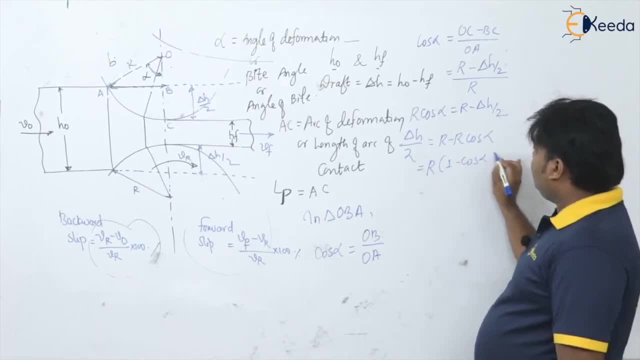 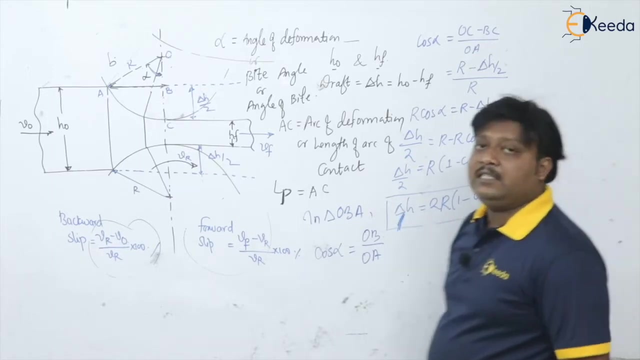 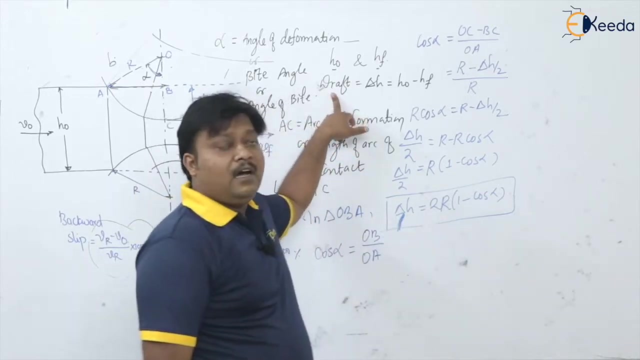 can have this R into bracket 1 minus cos alpha. Delta H by 2. or I can have this: Delta H is equal to 2 R into bracket 1 minus cos alpha. very good, important. you get the formula for the draft in the rolling operation. what you got, this Delta, is nothing but what. this is the draft in the rolling. 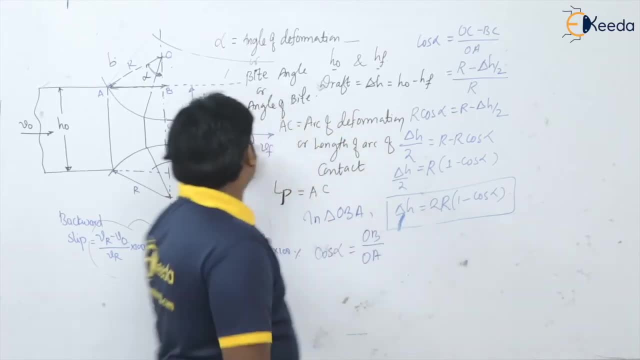 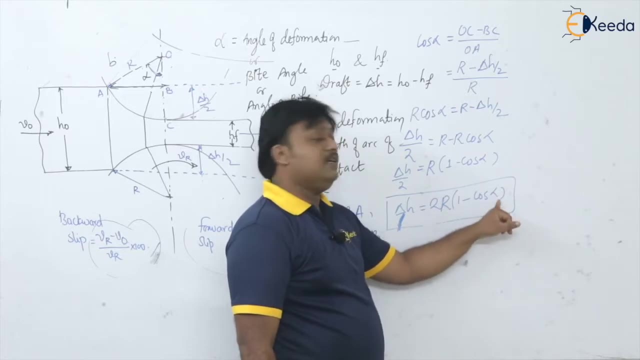 operation, which is 2 R. 2 R is nothing, but what diameter of the roller. you can also write here diameter of roller into bracket 1 minus cos of alpha. okay, so from this relation generally, Delta H is known to us, H original is there, H final. 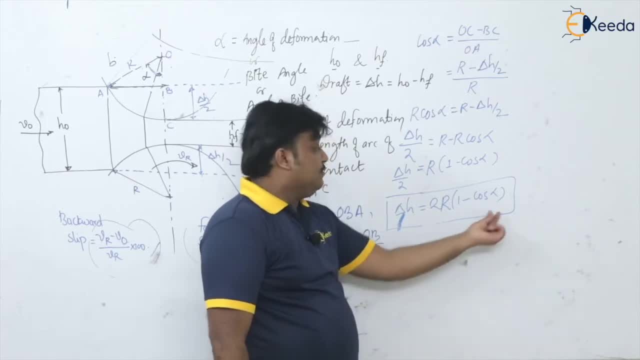 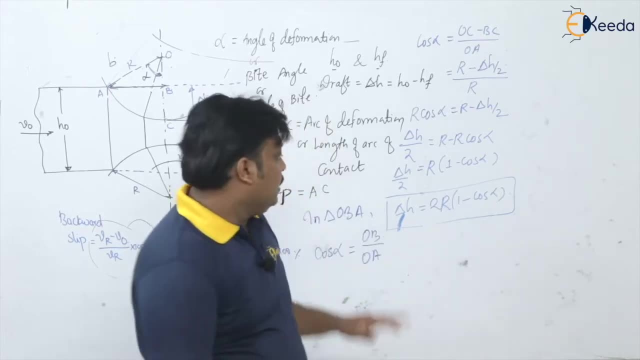 given into the numericals, and then we get the formula for the rolling operation. we are interested to find this alpha value that is, angle of deformation, or the angle of bite we are interested in, isn't it so, from this formula. please see this formula. this formula is for the calculation of the angle of bite, this alpha value. okay, 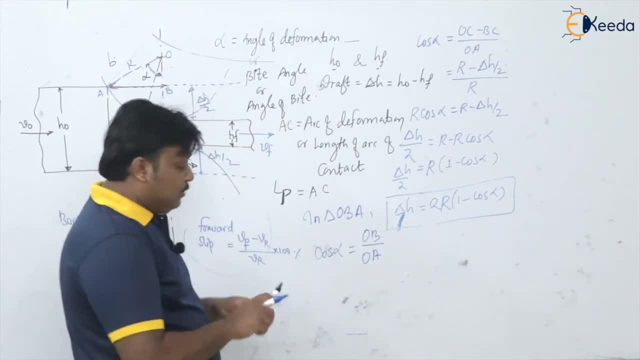 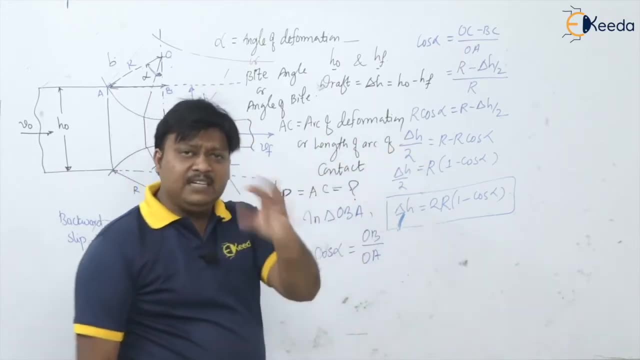 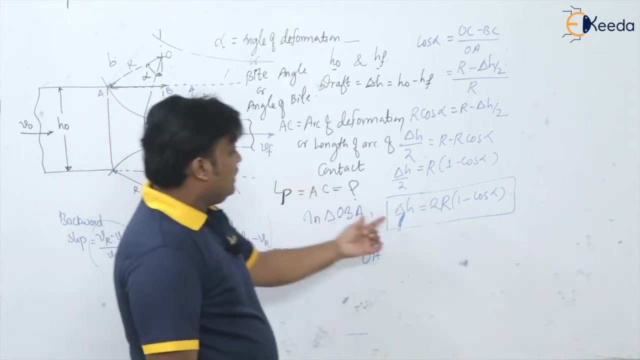 now the next thing that we are going to determine the AC, because again, many times 2, 2 mass is question. many times in the gaze or es paper you can find this question on these formulas okay. so delta h is equal to 2r into bracket 1 minus square alpha. from that alpha can be determined. 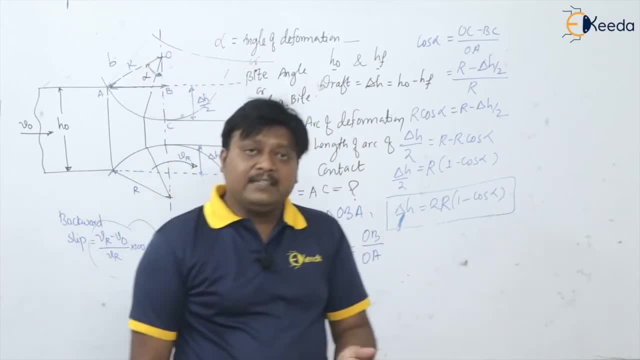 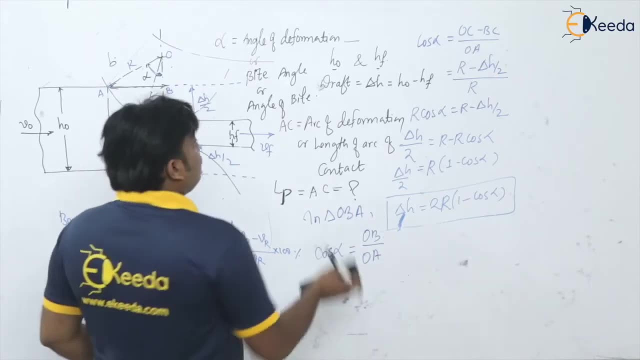 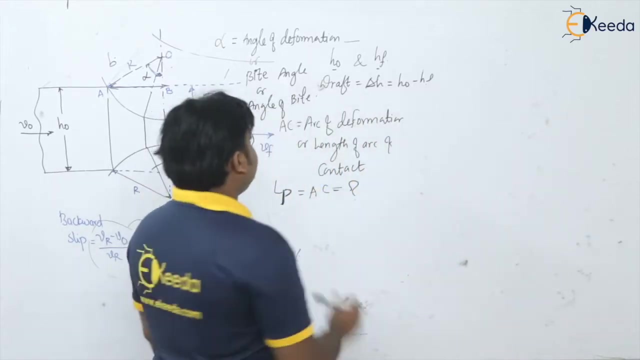 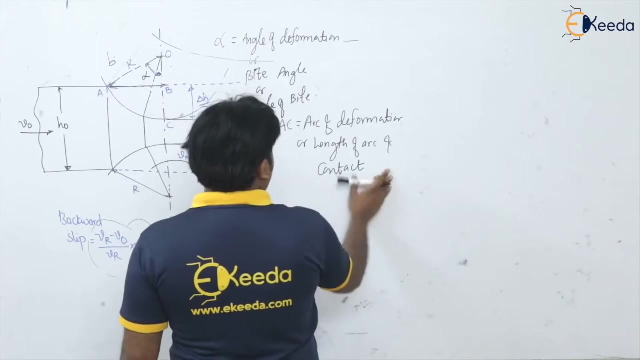 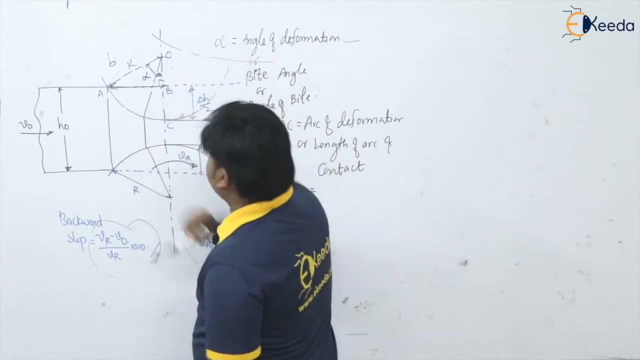 now they are asking to determine the length of arc of contact or length of deformation zone is nothing but how much. a, b, okay, so if it is over i will rub it. so tell me now we are doing work for this lp. so again from c, right angle triangle, o, b, a, what is? 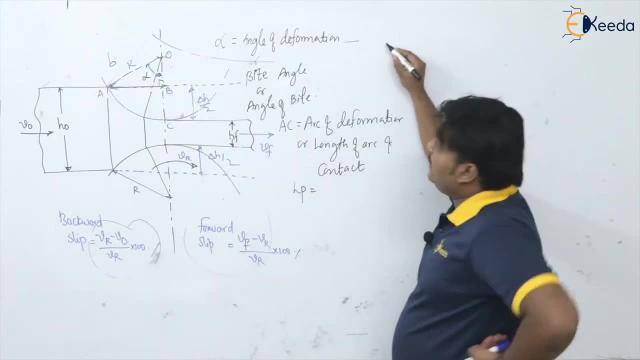 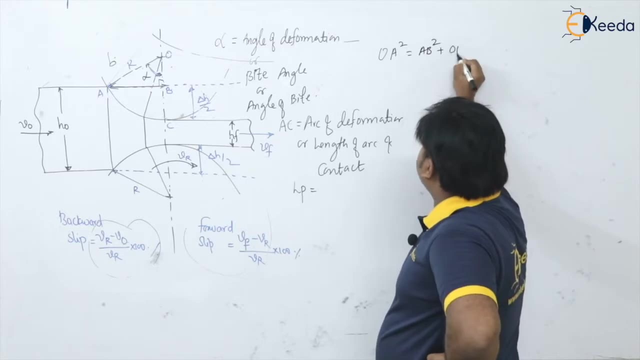 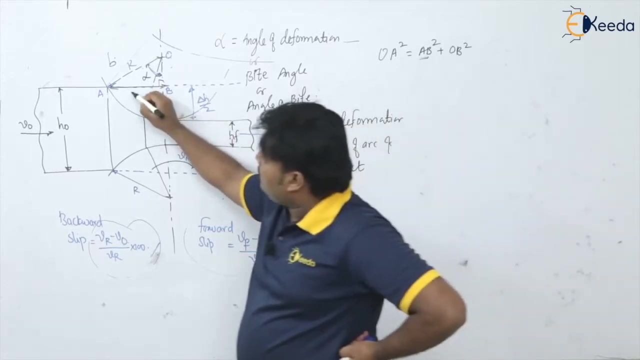 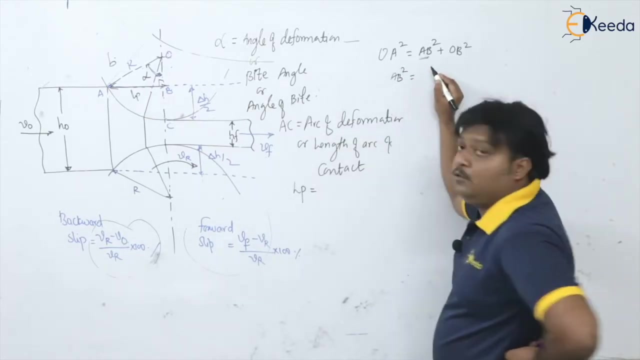 if you apply the pythagoras theorem, simple pythagoras, what you can write this: o a square is equal to a b square plus o b square, isn't it? so from that we want a b is nothing but our length of arc of contact. that is represented by lp. so a b square will be what? do it fast, but show. 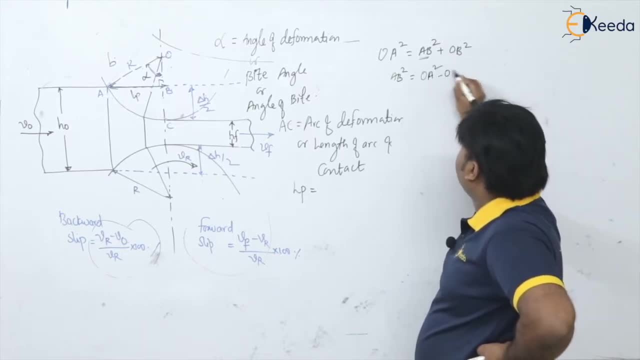 this o a square minus o b square, isn't it? o a square may say o b square square or a b will be what under root of o a square minus o b square. now put the real values for this. what is o a is nothing but the. 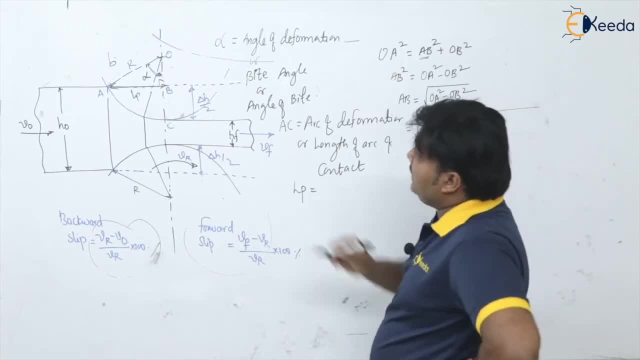 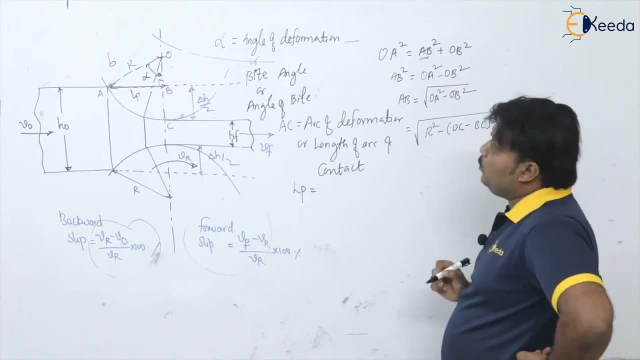 radius of roller: r square minus o b, again o b, guess, any call. okay, o c may say b c nickel. yeah, o c may say b c nickel. gaya ob uska square. but again in that, again go for simplification. r square minus o c is what again? radius of roller. 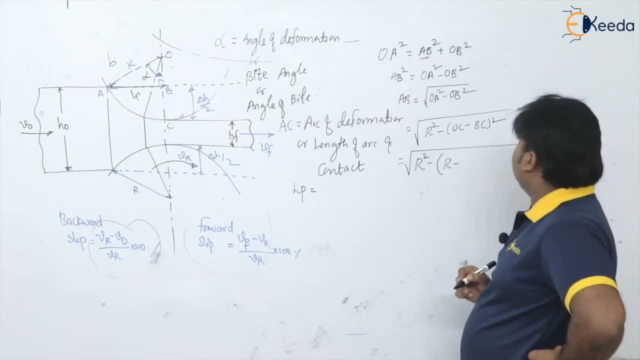 r minus b c is delta h by 2, isn't it delta h by 2 whole square. now solve for bracket a minus b whole square, that is r square into bracket calicum: a minus b whole square, that is a square minus 2 a b. 2 a b means 2, 2, 1 minus r times delta h plus b square, delta h square by 4.. 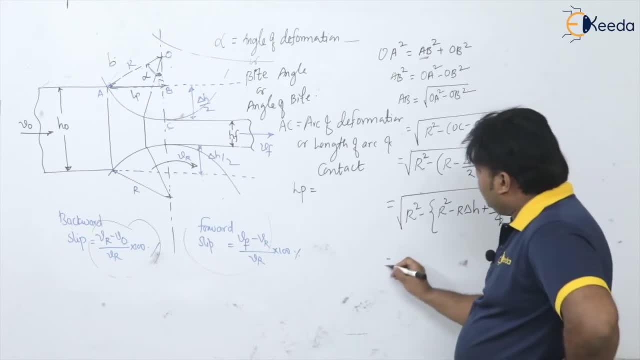 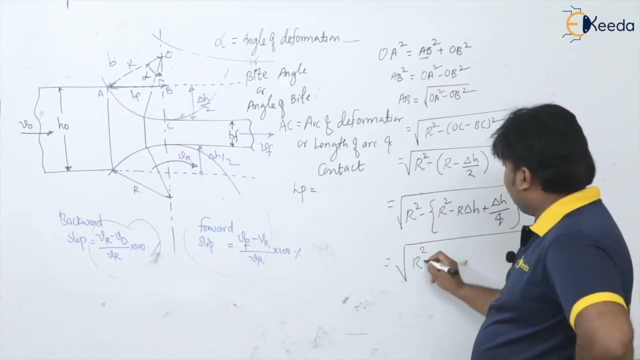 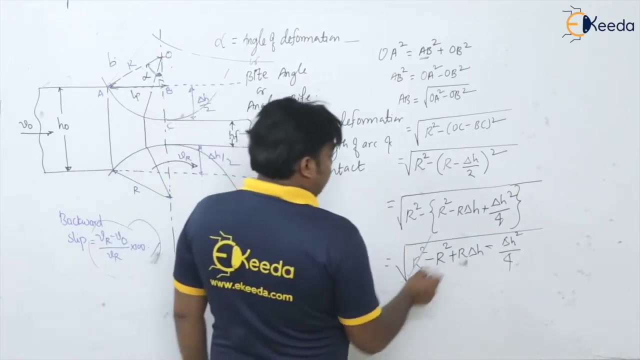 bracket complete. go for again simplification. so r square. it has a minus sign, so multiply and get the minus r square plus r times. delta h heute devide by 4. i hope it is clear to you. so you look at this, this already, this delta. 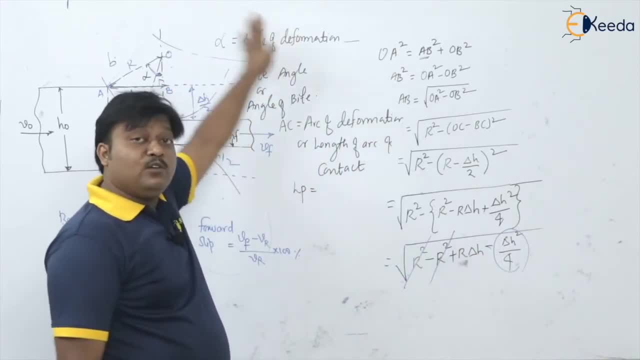 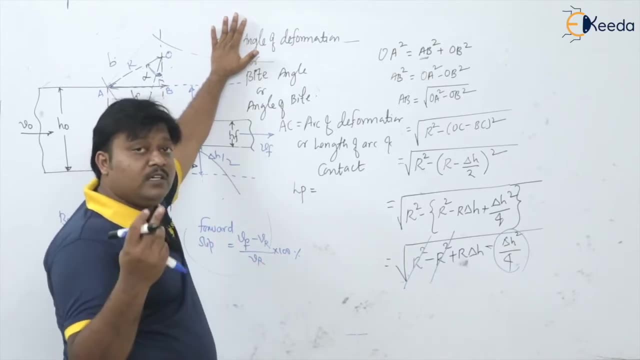 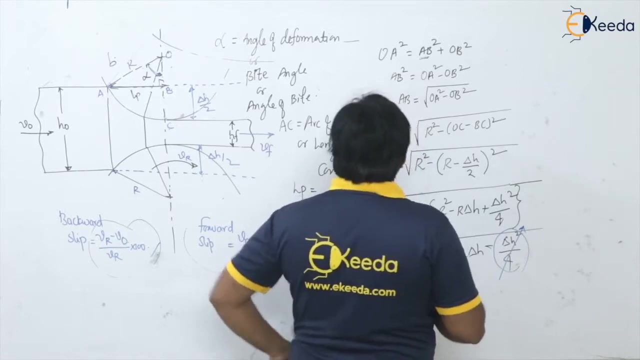 delta H by 2 is very small term. square it again, divide by 4, and R into delta H. we have to minus it because the roller radius is much bigger than the plate thickness, isn't it? or whatever the reduction we are getting as a draft. delta H. so it is very small term. you can not have any kind of impact on the relation. 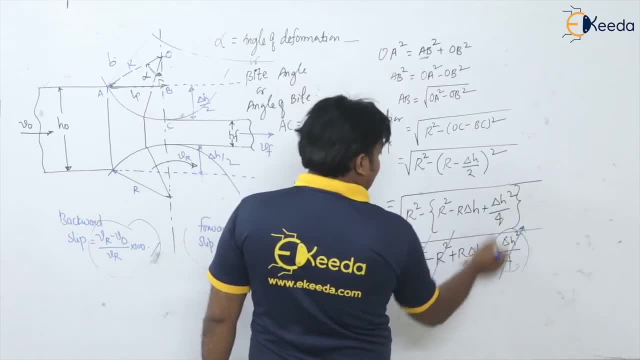 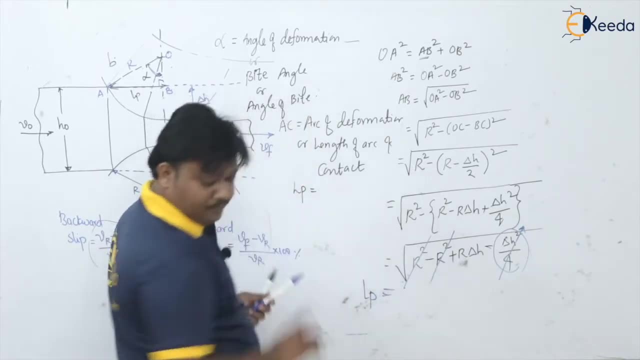 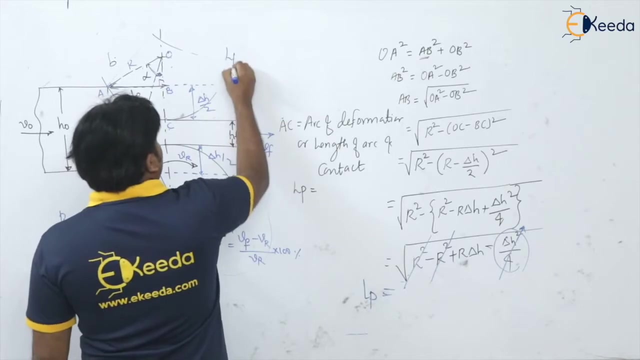 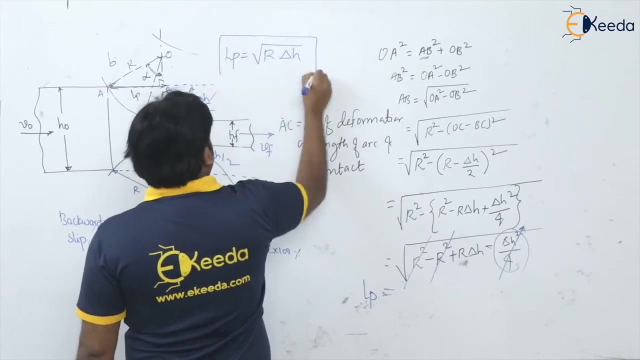 so say I am neglecting this term because no need there. so what I can write for LP, I will write it here on the top. so what I can write, this LP is equal to: under root of R times delta H. R times delta H. 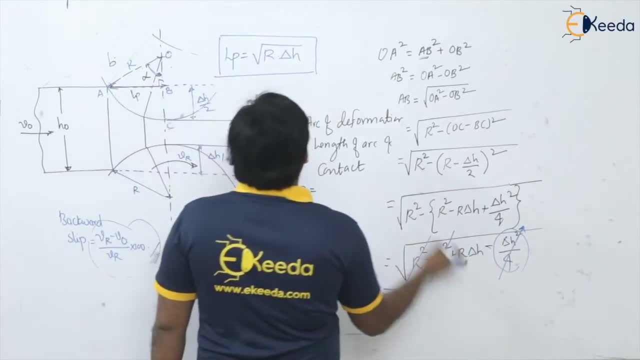 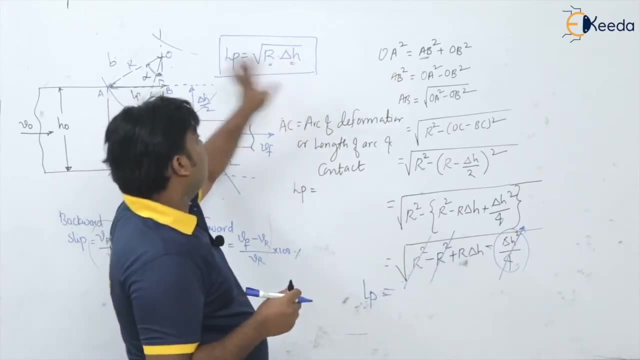 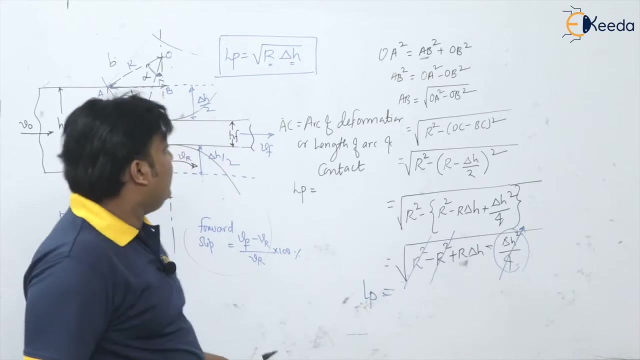 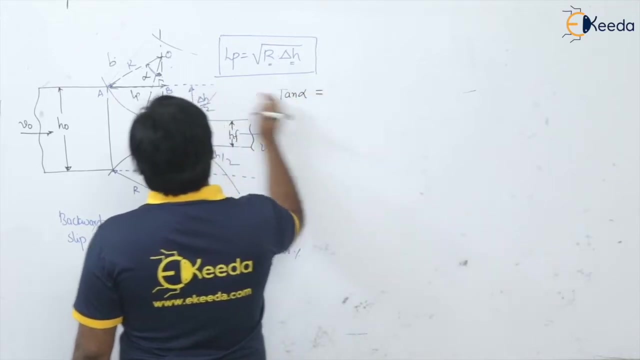 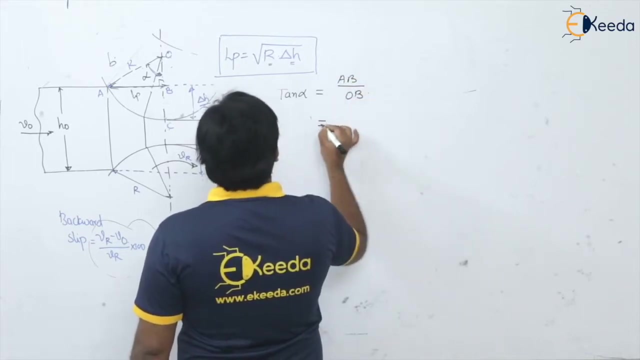 please remember R times delta H, where R is roller radius and delta is the draft H original minus H final. this is your delta H. okay, now tell me the value for tan of angle alpha. tan of angle alpha: what is tan alpha? that is AB divided by OB. what is AB? this is LP. 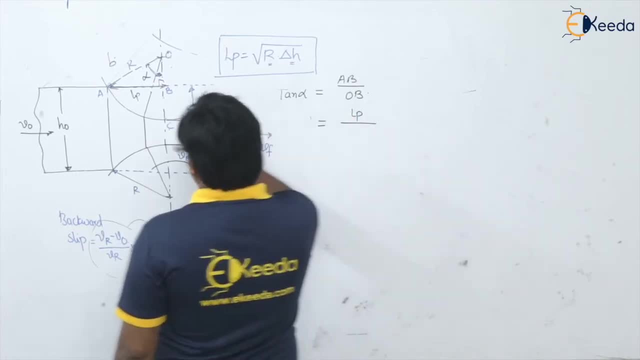 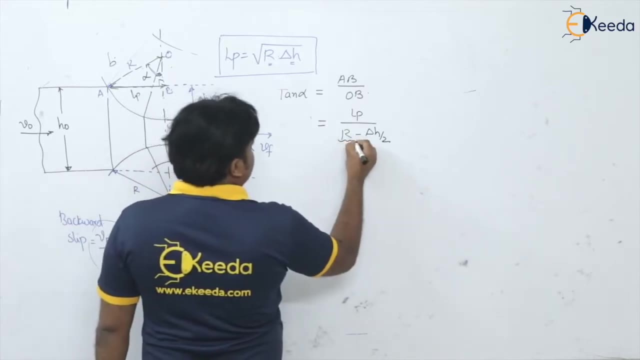 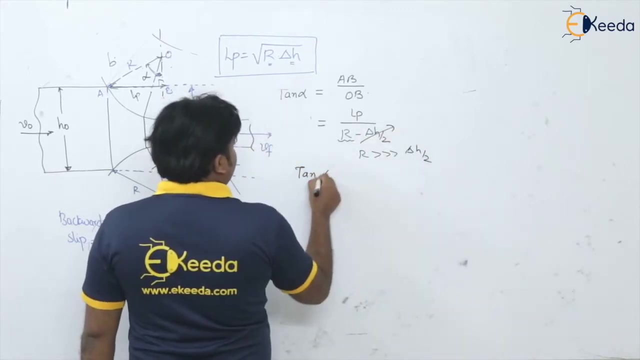 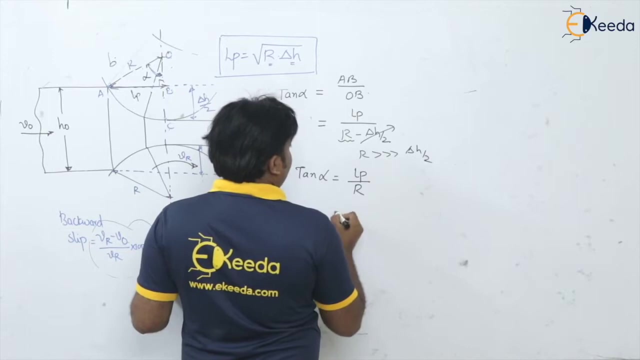 that is R, length of arc of length of arc of contact and OB. is what this R minus delta H by 2,? I will write directly: okay, now, R is very much bigger than this delta H by 2, so neglect this term. so what is tan alpha, which is equal to what this LP divided by R? what is LP under root of R, delta H divided by R? 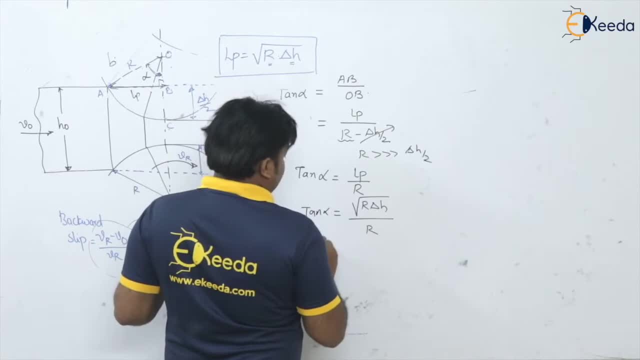 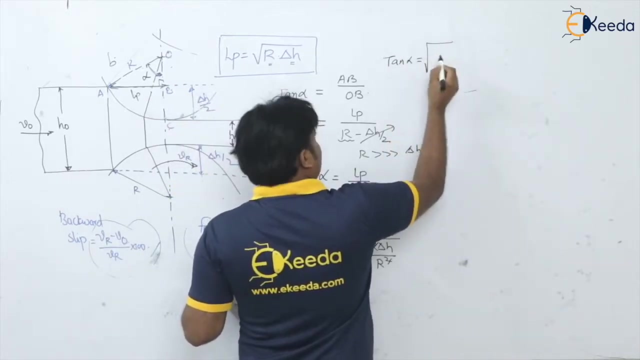 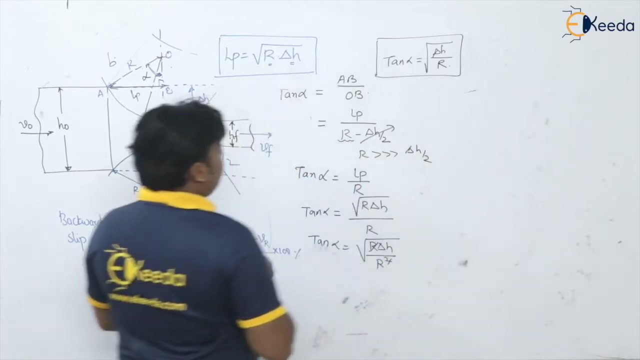 so tan alpha. tan alpha is equal to what? take this R into this under root. so R, delta H divided by R square R, R get cancelled. so what is tan alpha? tan alpha is equal to under root of delta H by R and as the by classical friction theorem, this tan of angle alpha is what is nothing but the coefficient of friction. 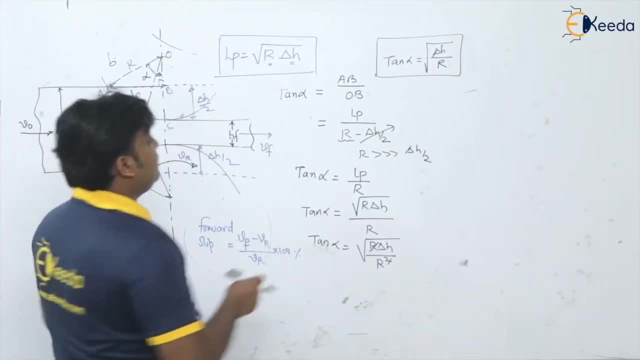 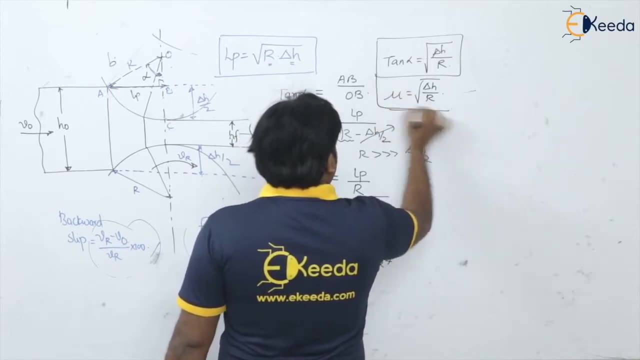 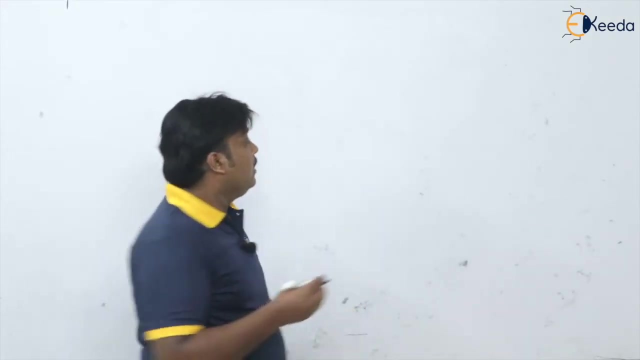 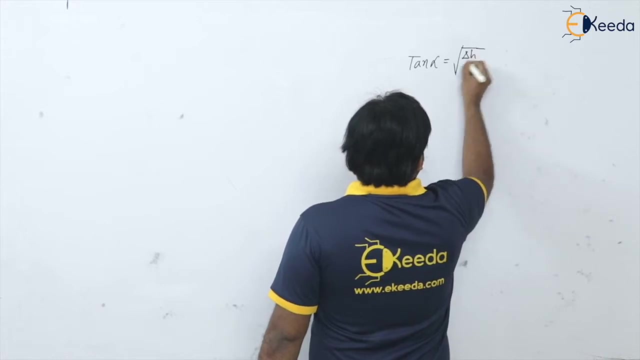 so tan alpha is equal to what is nothing but the coefficient of friction. so we can write, for mu is equal to tan. alpha is nothing, but mu is equal to delta H by R, R, R. see here, dear student, now what we have seen, that about the tan of angle, alpha is equal to under root of delta H divided by R. 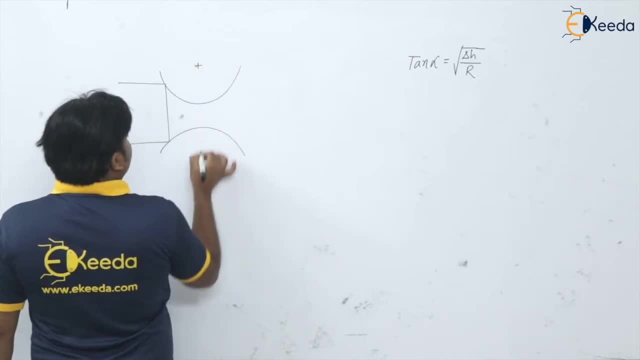 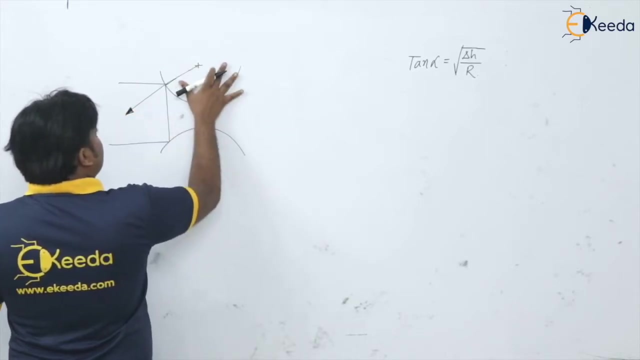 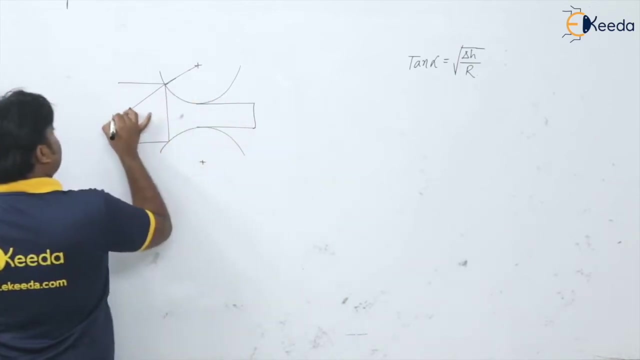 okay, so resolution of pressure. so see, so here will be the pressure acting by this roller onto the strip is say Px, okay. and at the same time, when the strip is moving, 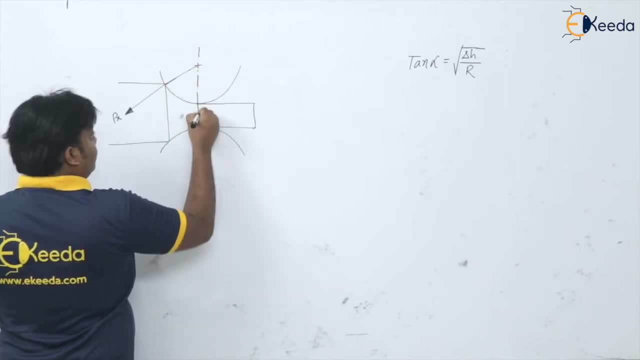 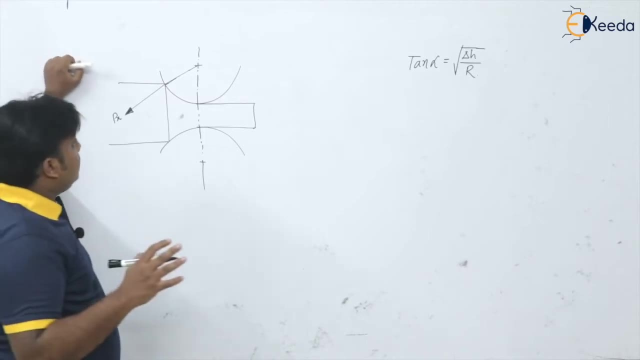 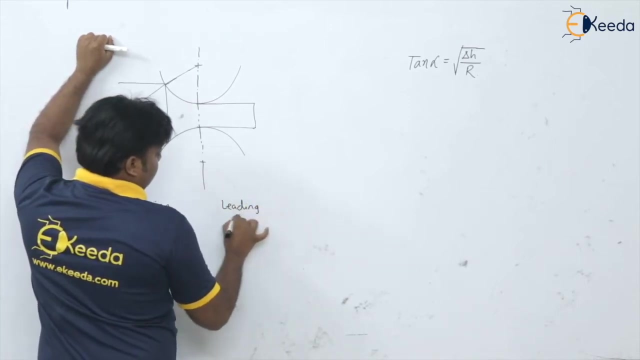 to the deformation zone. please remember that in the rolling operation the add the, the, the lagging zones. see, there are two zones basically in the rolling operation: lagging zone and leading zone. so lagging zone. 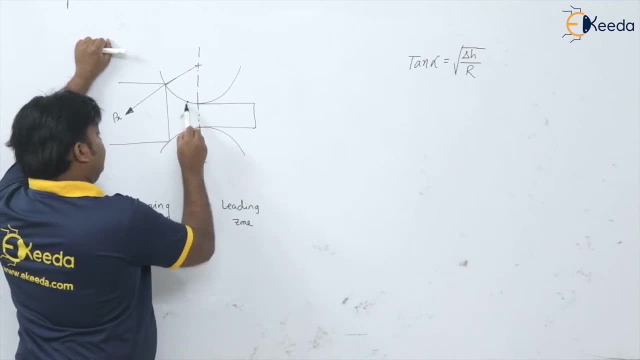 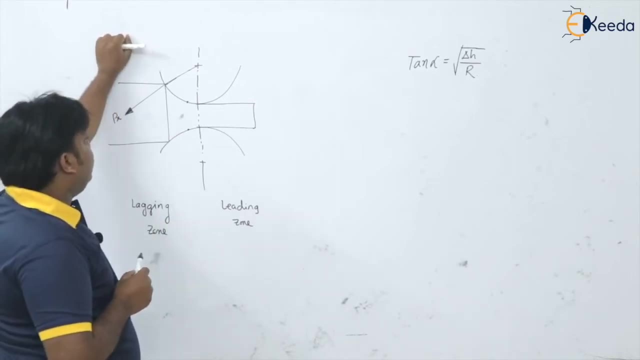 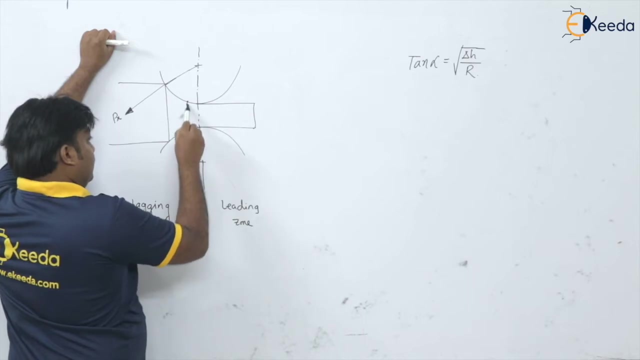 Qa' phe hai. so we have discussed about the neutral point, isn't it? where the relative velocity 0, where the linear velocities are same. okay, now, in the zone left to this neutral plane, where the strip is lagging behind this neutral point, isn't it? and if you see, 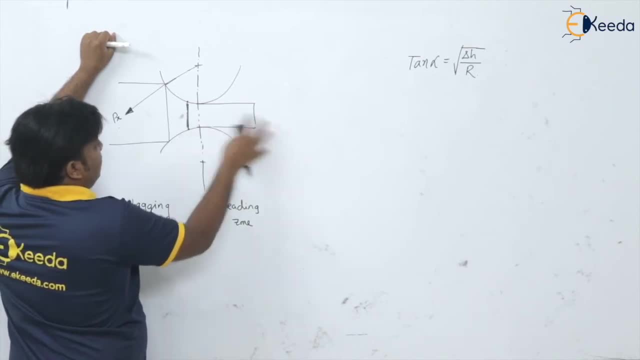 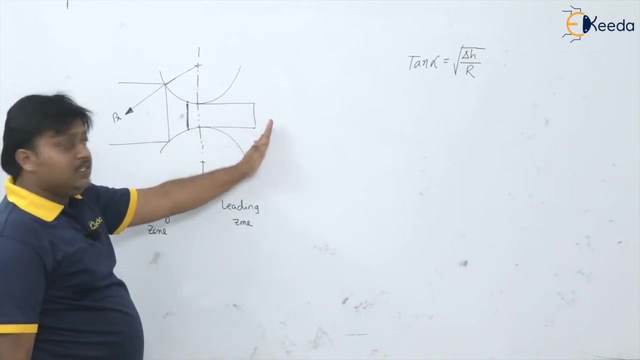 this exit point. now, strip is leading ahead of this neutral point. that's why we are getting here two zones. one is at the left of this neutral plane that is lagging because strip is lagging here, and at the right of this neutral plane, if the strip is leading, isn't it so that's why it's a leading zone now, if 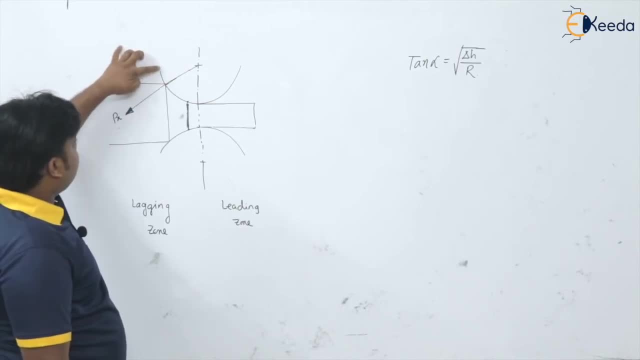 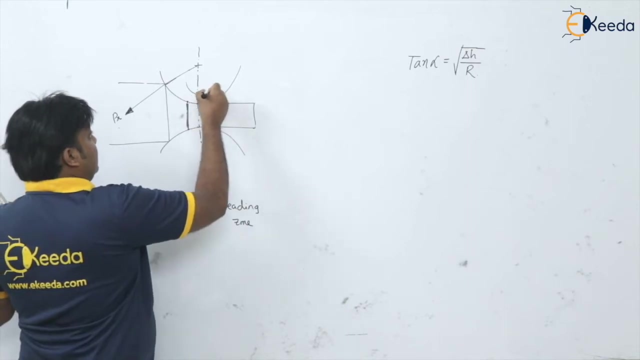 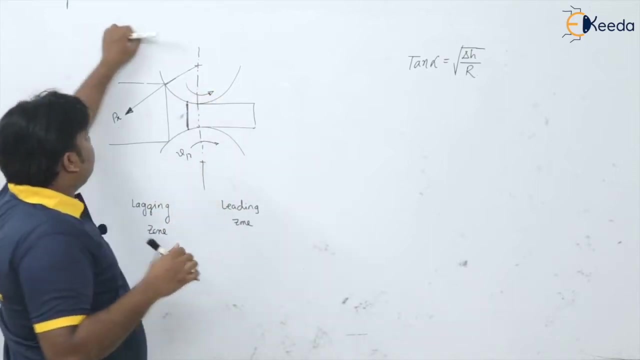 you have say, this is the contact point, where the contact point of roller and the strip, we are having the pressure acting as px now at the same time when in the lagging zone the roller is having the velocity rolling, a roller velocity. we are in this direction, so initially from the in the leading zone, from the 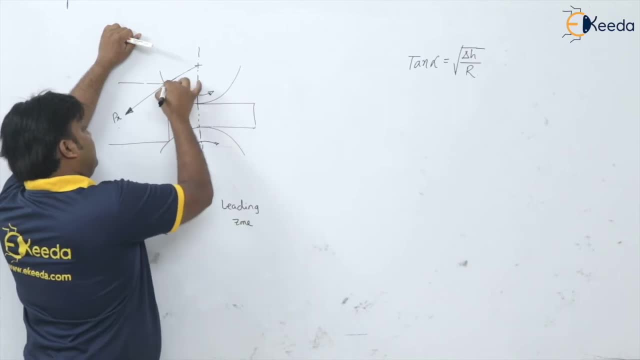 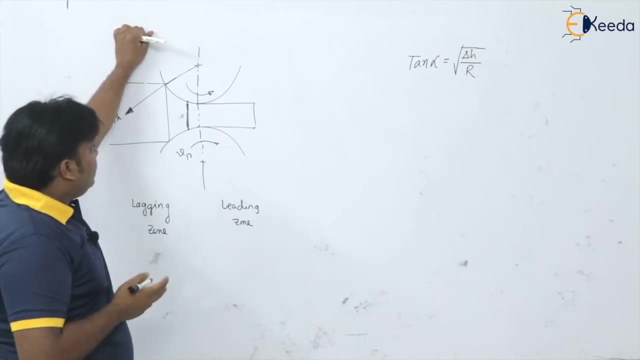 starting point up to the neutral point. please remember that the component of frictional force or frictional force is always acting in the direction of the velocity of the roller. please remember the frictional component of this pressure px, that is nothing but mu times px, which, in acting here tangentially to 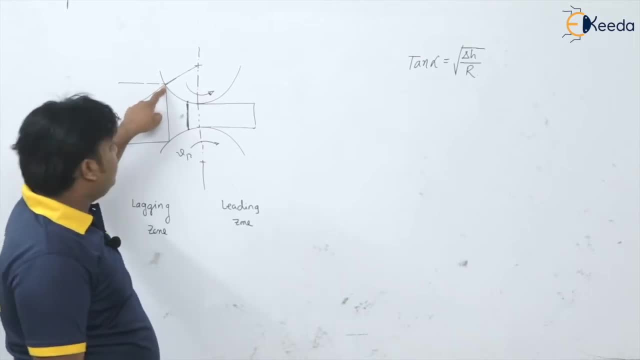 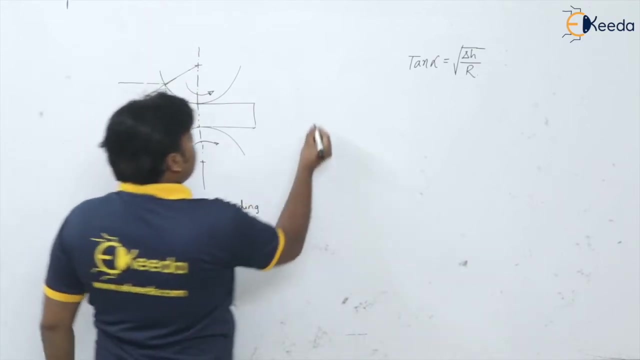 this is having the same direction as the direction in which the roller is moving up and down until the point where the flow is rotating. please remember, up to neutral point. but when the neutral strip passes the neutral point, now the friction is acting in opposite direction. please remember, say in: this is the pressure px. 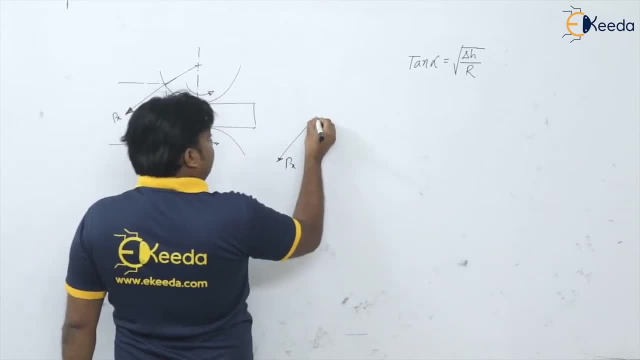 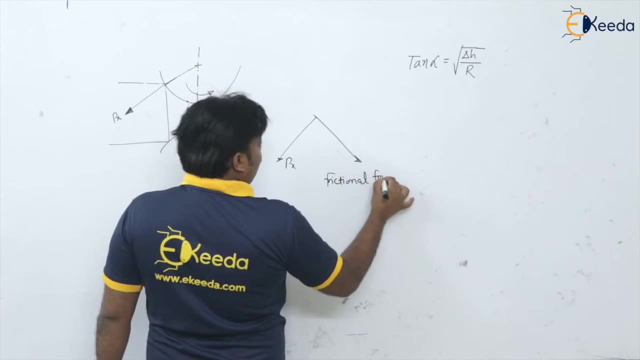 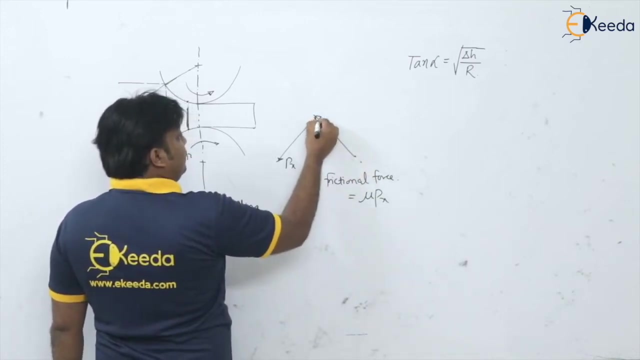 okay, now to that, we are having this component of frictional force. frictional force, what should be, it is that is mu times px. so in fact, this is the pressure px, so in px, isn't it? but it is not acting in the opposite direction, otherwise a friction. 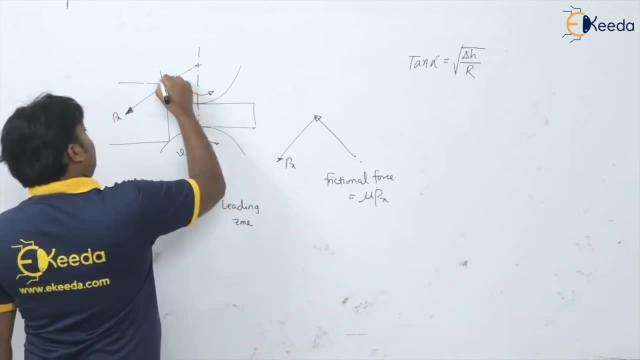 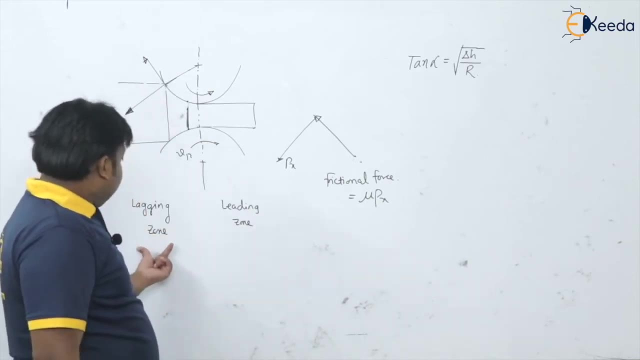 will it? opposite map, but coregay definitely pressure our work. frictional force, a Bologna sir, a salary, but please remember that at they are in the lagging zone. the component of frictional force is along the direction of the rotation of roller. once it passes the neutral point, then the frictional 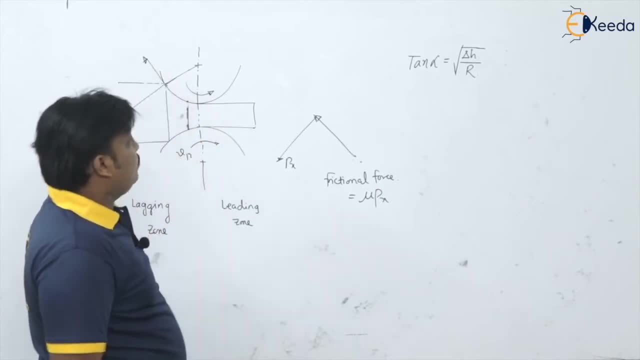 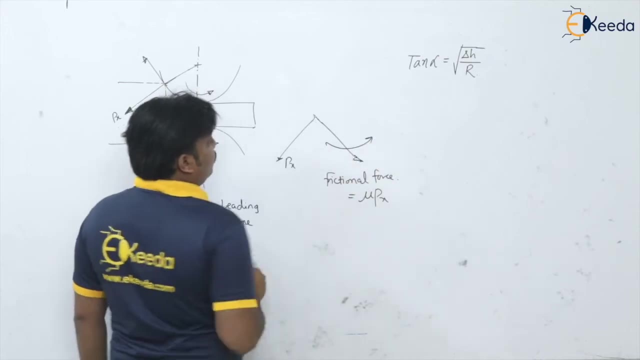 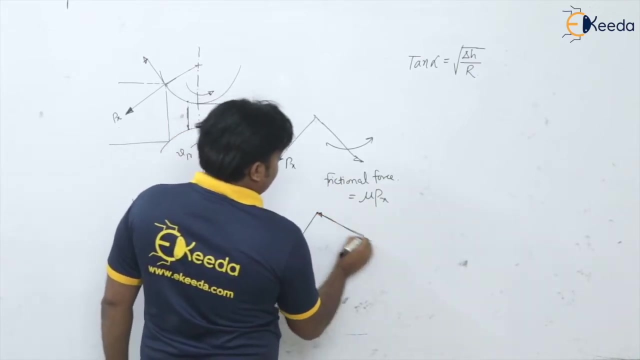 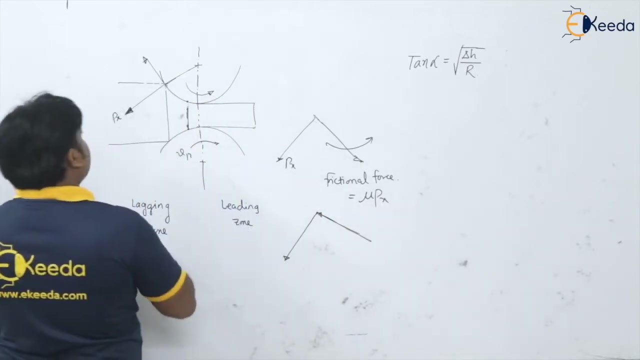 force is now started acting in opposite direction. please remember, like this: but here, at the lagging zone, it will be in the direction of rotation of the roller, and in the leading zone it will be opposite to that of direction of the roller. okay, so here, if you have this component, I will show. this is the. 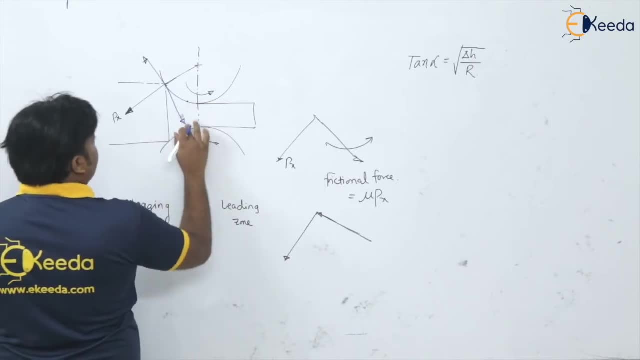 frictional component of this PX, which is nothing but what mu times PX, which is a frictional component. this is mu times PX. so mu is what the coefficient of friction at the interface of roller and the strip now tell me. if this angle- we know this angle- is how? 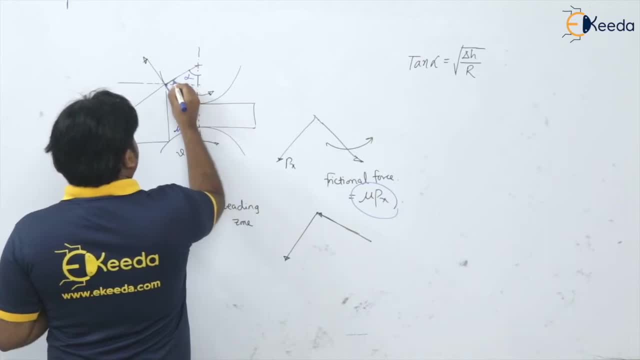 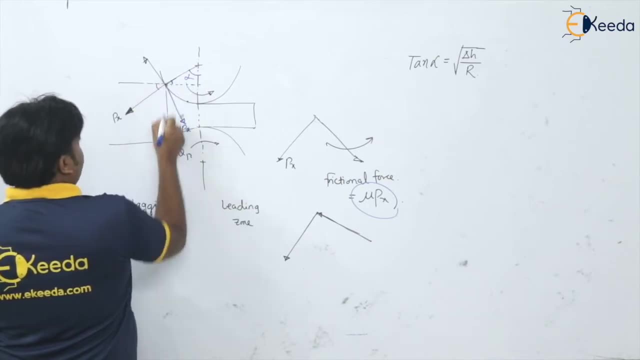 much alpha, isn't it? so this angle will be what 90 minus alpha, so this angle will be what 90 minus alpha- opposite angles. so from this right angle, 90 minus this 90 minus alpha, you will get this angle as alpha, isn't it? and at 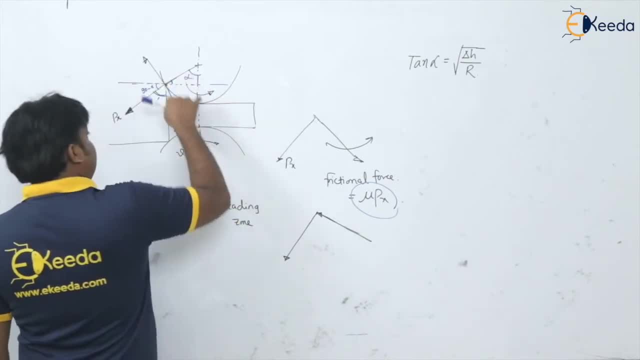 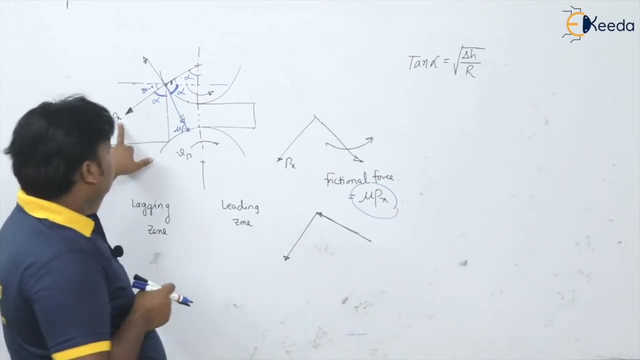 the same time. see here, this is tangent shield to this PX. so this angle is 90 degree, isn't it? but in that 90 degree this is angle 90 minus alpha. so if you look at this angle, this is again alpha. please see it carefully. and now you can easily resolve this component PX, that is, pressure force, and 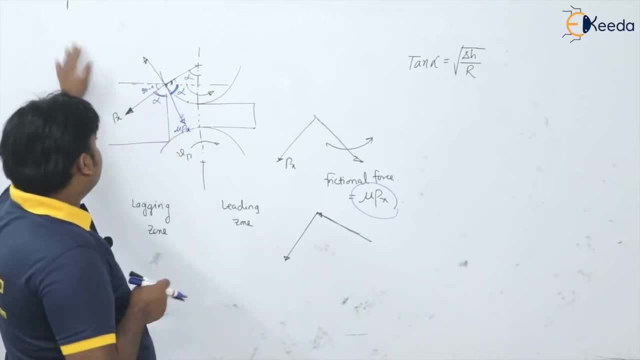 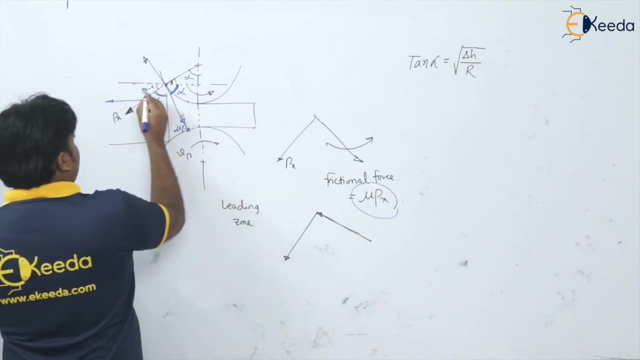 the frictional force very easily. how see: if this is alpha, then horizontal component of this will be: this is the horizontal component of PX, will be PX cos alpha and this will be PX, what they can component, PX, sin alpha. now this is the mu PX and this is the horizontal line, this is alpha. so with the horizontal, 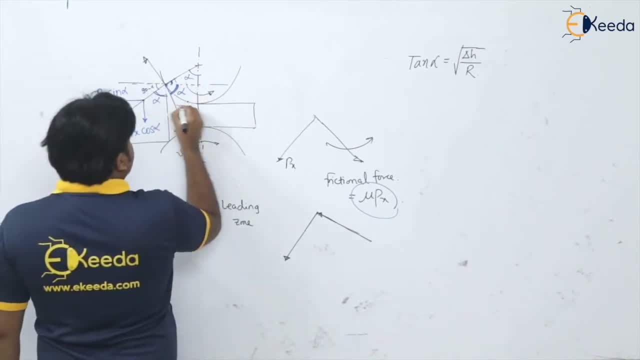 line. it will be the angle. horizontal component will be mu times PX, cos, alpha, isn't it? and this vertical component will be plus alpha. now, here, when we have alpha got, this is the equation. now, what is the frictional component on PX? so nge will be. 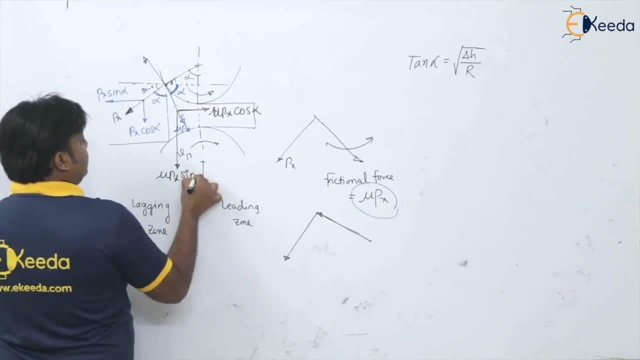 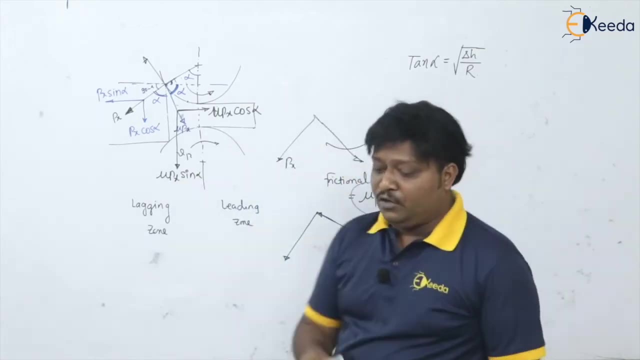 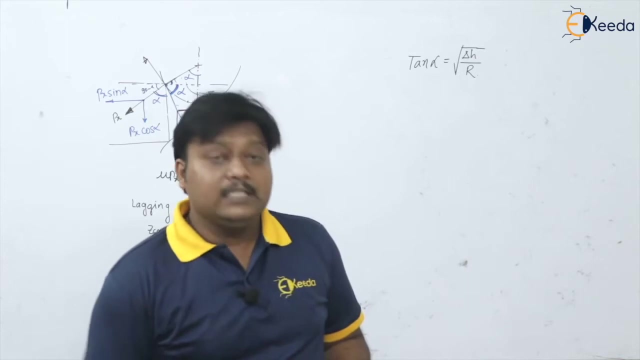 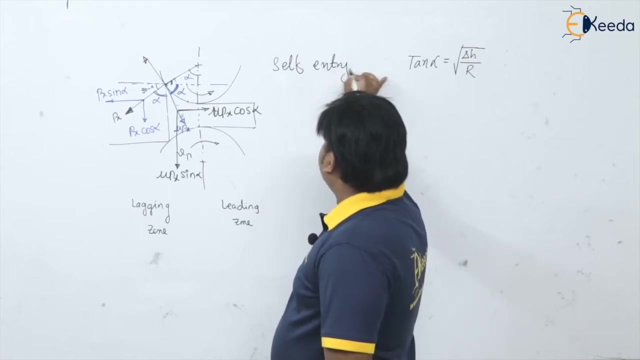 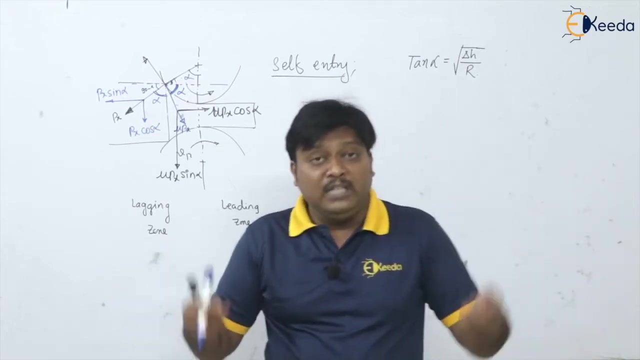 be mu px sine alpha. Now I hope it is clear Now, after having these components of forces, now we need a very important condition, that is, the condition for the self-entry. the self-entry that the plate or the strip without any back or without any pulling action, 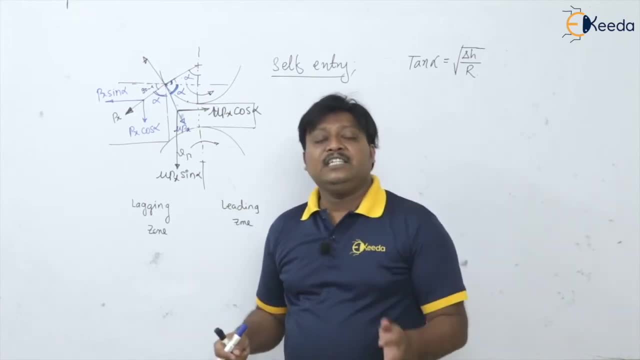 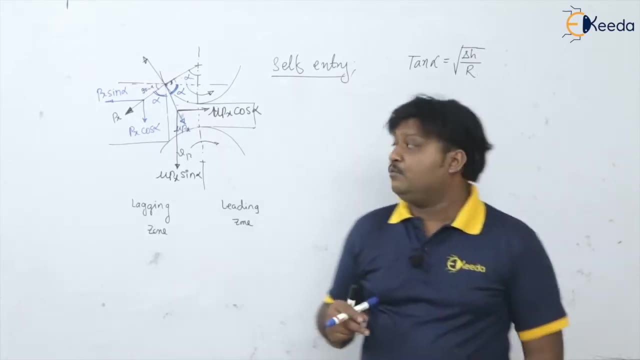 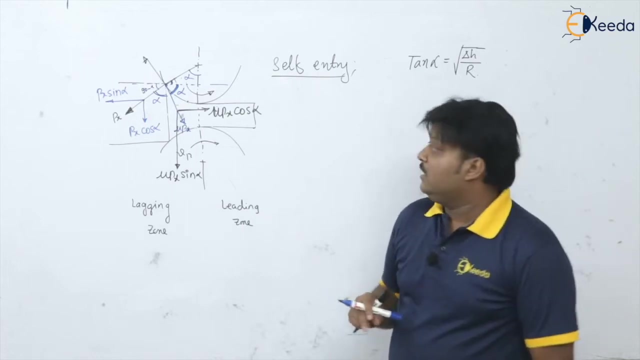 it will enter into the roller. that is the condition for self-entry and this is we know very well. this is because of the, this is because of the frictional force, this is because of the friction which is present at the surfaces of plate and the roller. So, of course, 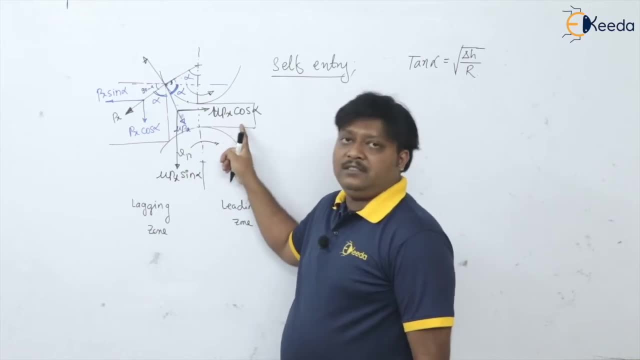 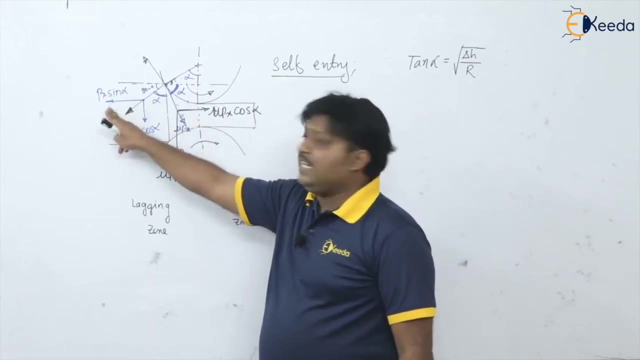 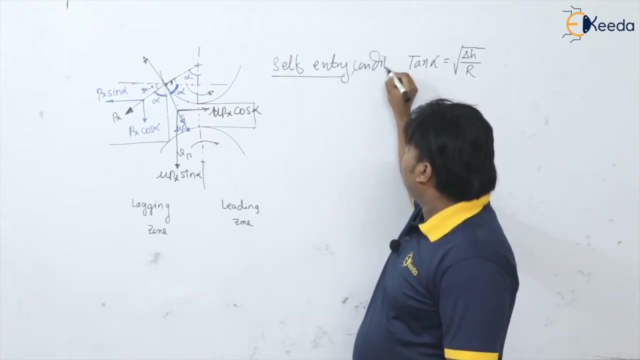 the self-entry will enter into the roller. and the self-entry will enter into the roller here, this frictional component in horizontal, that is, mu, px, cos alpha. that is what I am writing for, the self-entry condition, when the self-entry can happen, when this mu px cos alpha should be greater than or equal to what this px. 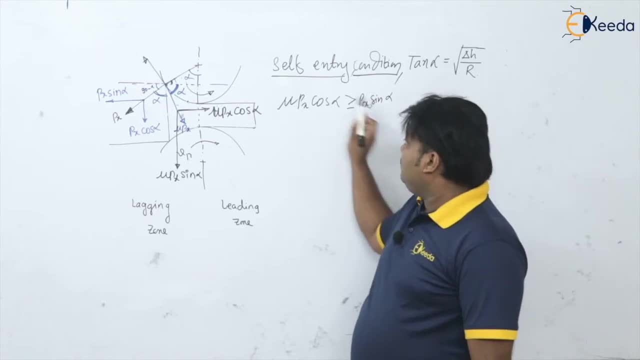 sin alpha. It means that this mu px cos alpha should be at least how much? at least px sin alpha should be equal to. If you do like that, then, and if you have like that actually, then, and then only the plate, which is the strip which will enter into the roller. 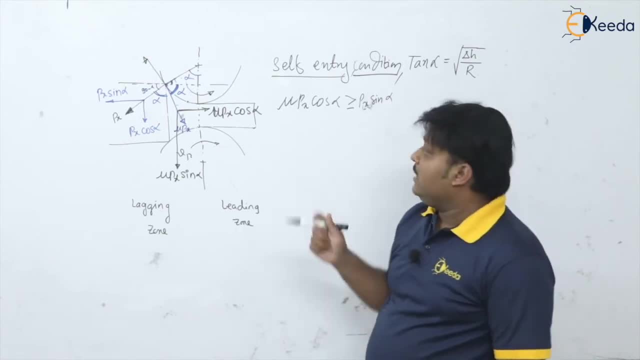 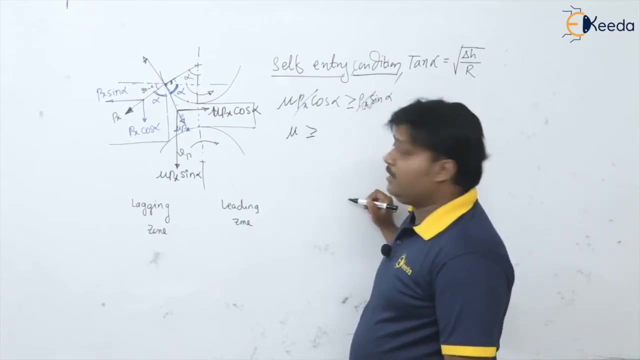 will enter into the roller. Okay, So here see px- px get cancels. So mu px cos alpha will enter into the roller. So here see px- px get cancels. So mu px cos alpha. mu should be greater than or equal to what this sin alpha divided by this cos alpha. 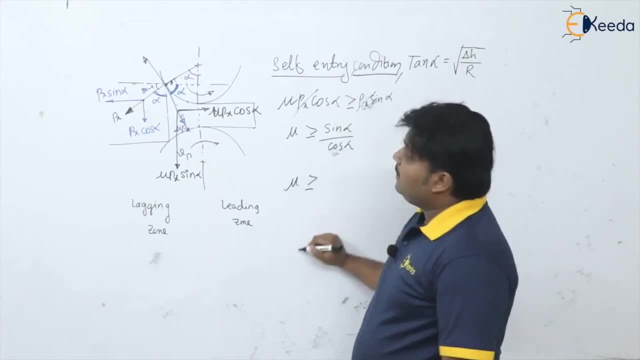 We know that mu should be, so coefficient of friction in the rolling operation should be greater than or equal to angle tan of angle alpha. That is the condition and what we have get. so mu should be greater than equal to what is tan alpha we got here. 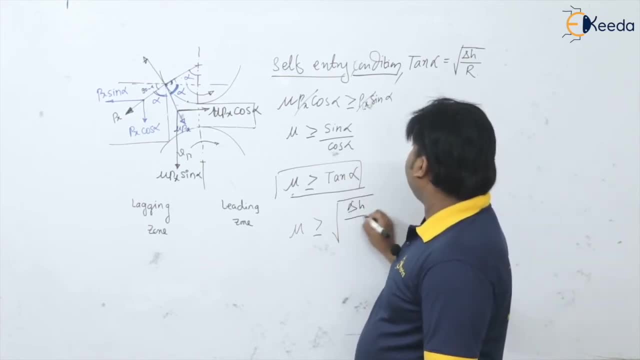 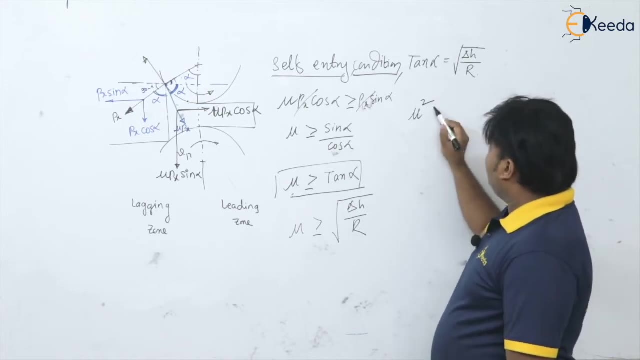 That is root of delta h by r, Isn't it? That is, if I squaring both side, what I can write. mu square should be greater than or equal to delta h times r, Isn't it So r? that is mu square. r should be greater than or equal to h, Isn't it Or? 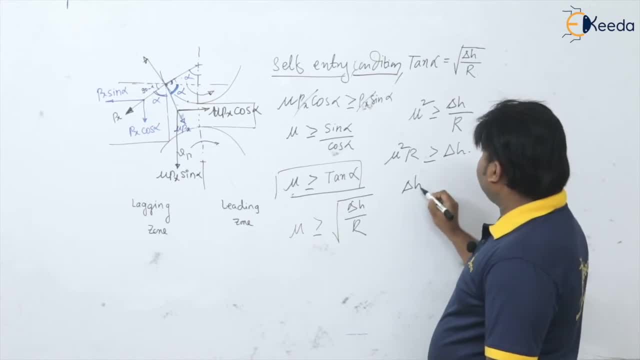 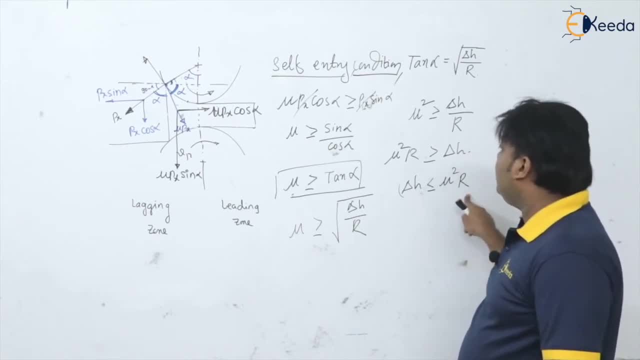 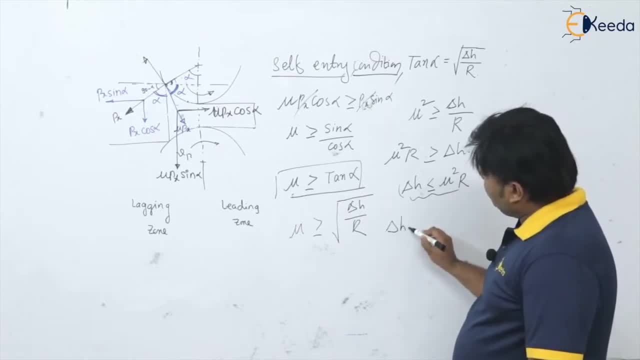 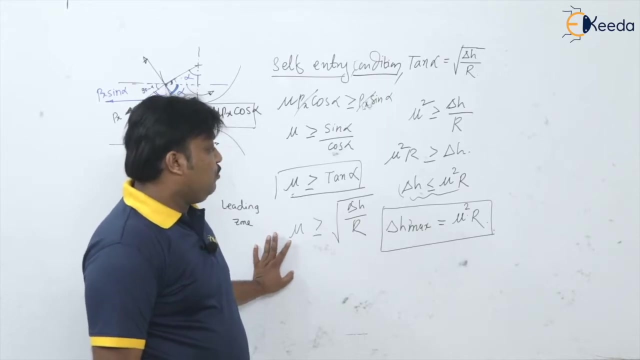 this less than or equal to sign. that is the maximum possible draft, maximum possible draft in the rolling operation. what we are getting, that is equal to what mu square times are very important, very, very important. please remember many times, many times- there are there are the questions many times asked in the gate- or is based upon this, this maximum? 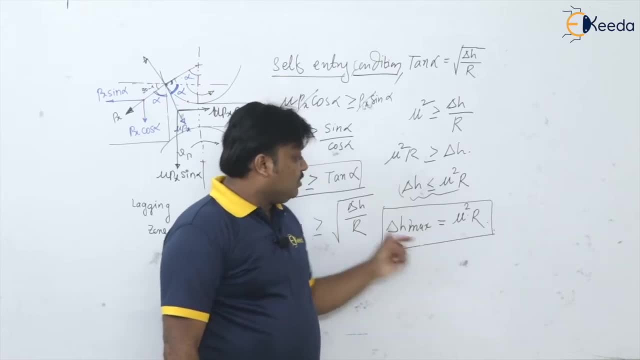 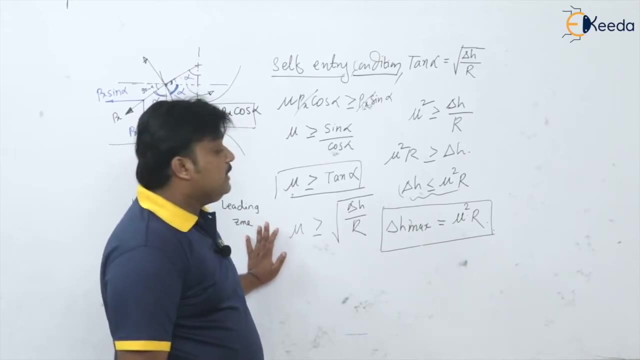 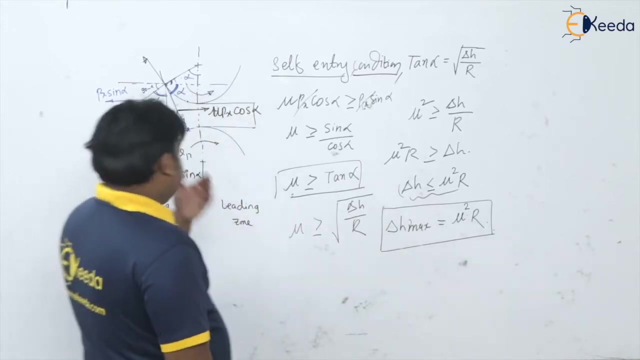 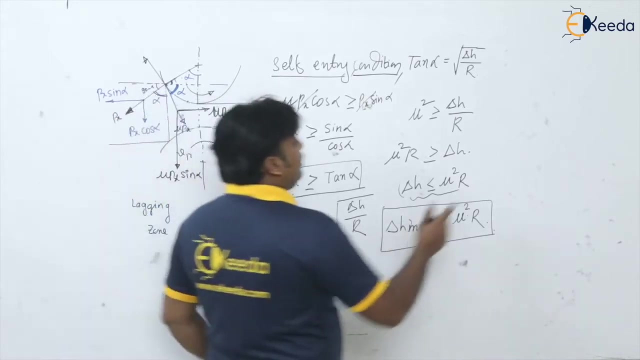 possible draft in the rolling operation now, the maximum possible draft rolling operation may. it is equal to mu square. mu is the coefficient of friction. square into the roller radius. into the roller radius. please remember this now from here they are also asking one more question type. is there that is they are asking: calculate the number of passes. 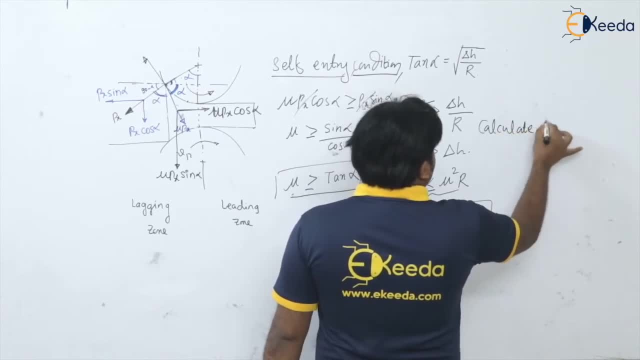 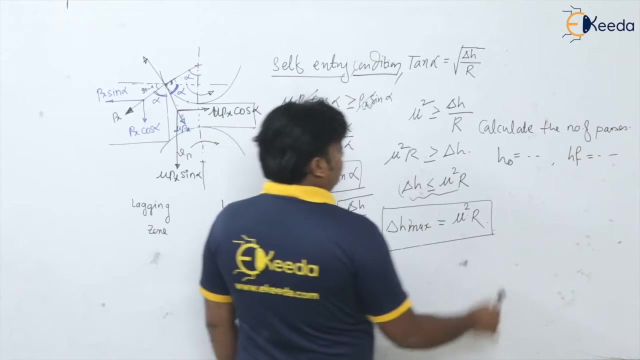 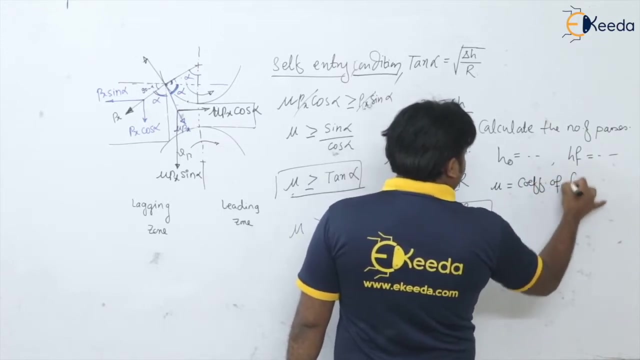 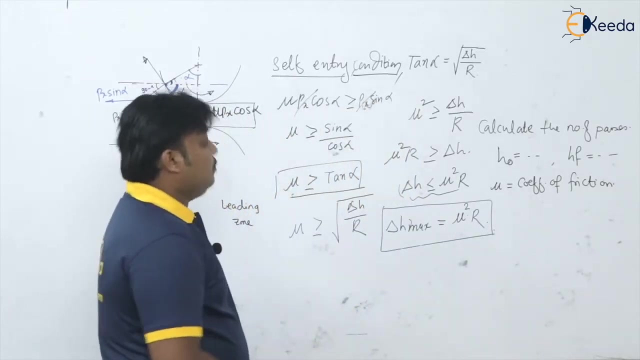 calculate the number of passes in the rolling operation. that is, h initial to give is given to you, then h final is given to you. okay, This is given term. and the mu, that is, coefficient of friction, is also given to you. coefficient of friction, Now how to calculate the number of passes or number of drawers in. 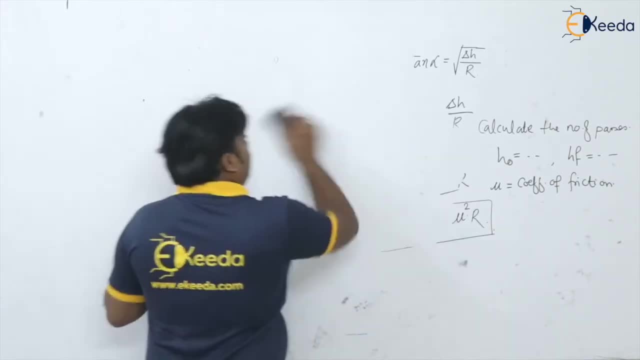 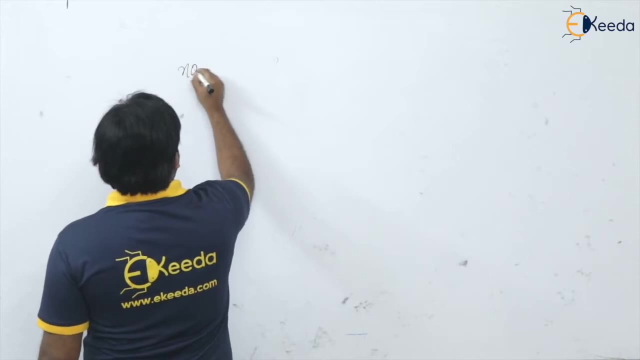 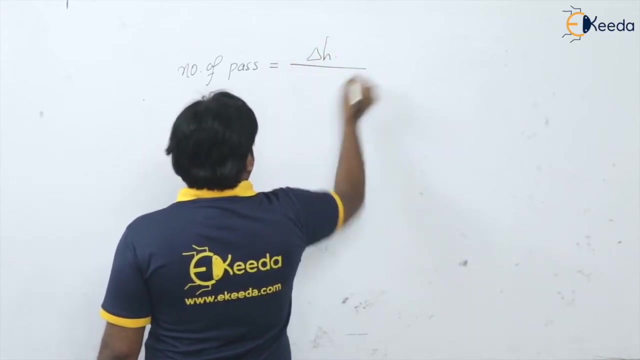 the operation of rolling how many number of passes. so the number of passes, the number of peach иса, the number of peach passes and the number of pens are the number of pieces pass in the rolling operation can be calculated as this delta h. that is the draft divided by 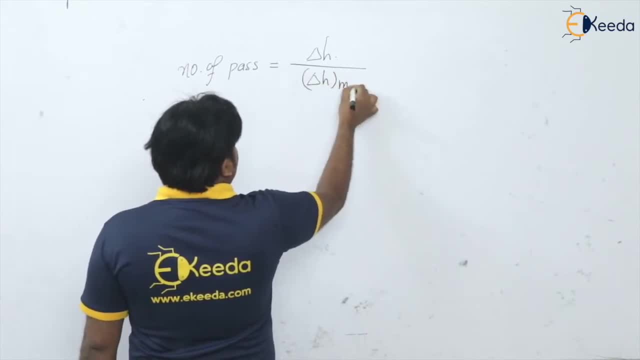 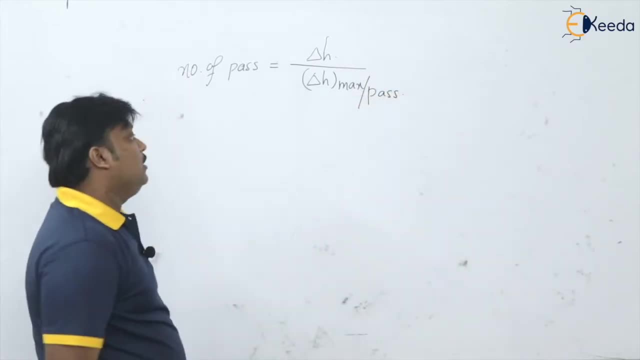 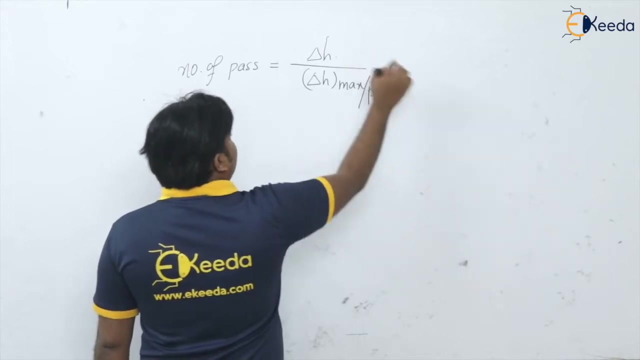 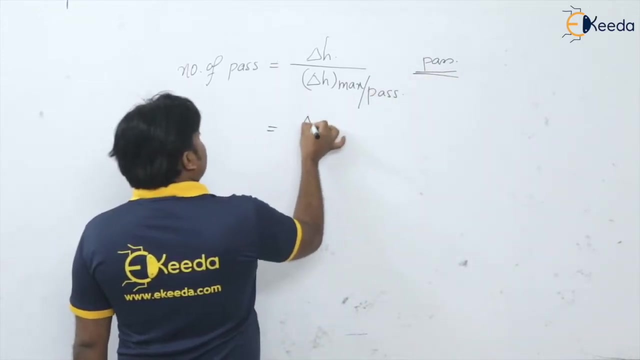 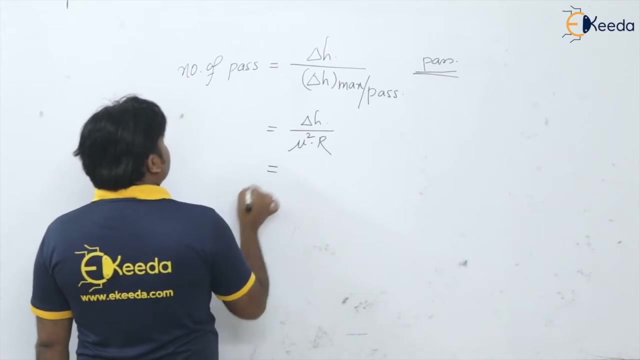 this maximum possible draft per pass, isn't it yes or no? so this delta h in millimeter, this max, is also millimeter. this pass will come here, so we'll get number of pass here. okay, so what you can write here. so delta h divided by mu square into r is nothing but the number of. 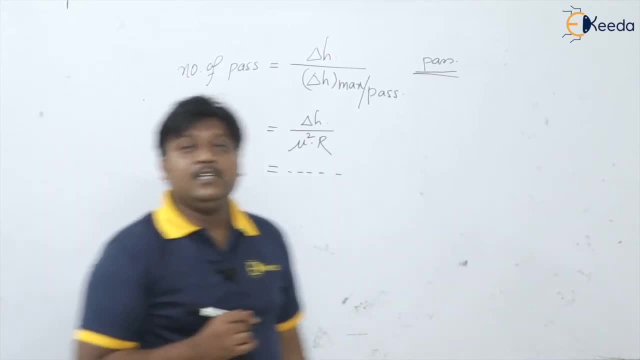 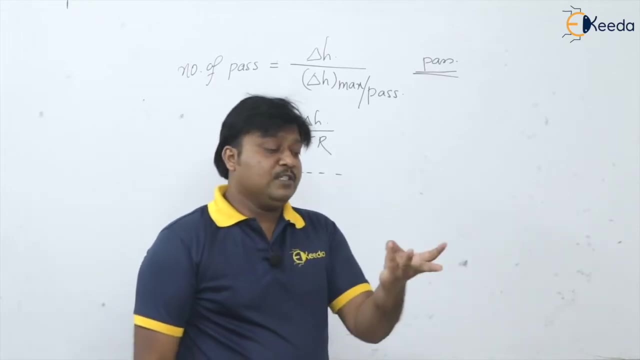 passes or number of pass in the rolling operation. this is how you can able to calculate the number of pass. please remember, irrespective of the two high, three high, four high, cluster planetary, irrespective of the rolling mill. okay, the answer should be there, otherwise, what happens sometimes? what students are doing? 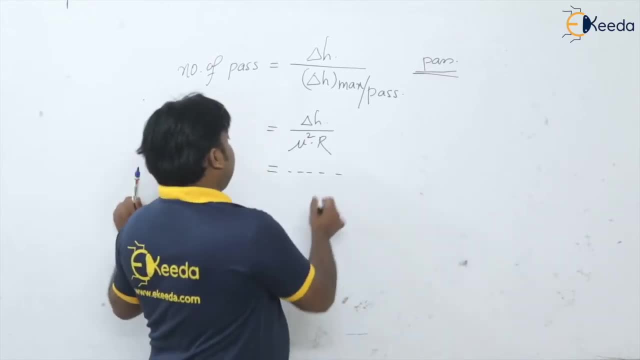 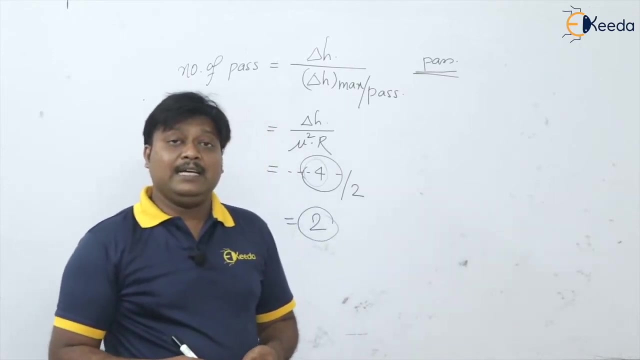 suppose if i say the two high reversible mill, then again, whatever the answer is coming here, suppose four passes, they will divide it by two and the answer will: they will write it as two. that is wrong. so whatever the answer is getting here is, irrespective of the uh rolling stand arrangement or rolling mill, you, you will get the number of passes here, okay. 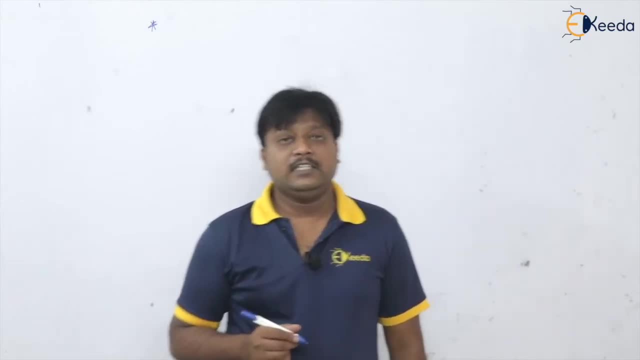 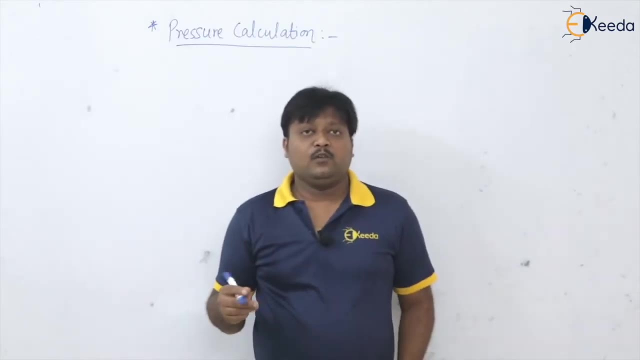 now we are going to see the pressure calculation in the rolling operation pressure. so in the rolling process we can have the pressure in the lagging zone, we can have the pressure in the leading zone and we know that the maximum pressure that is going to be at the neutral point. so in these three regions we can 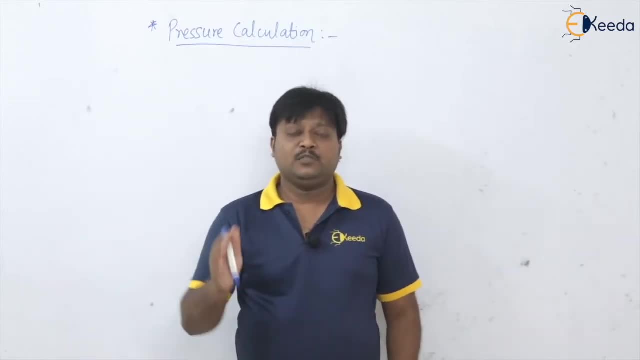 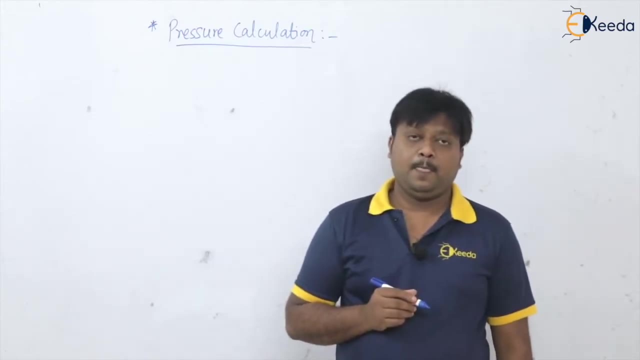 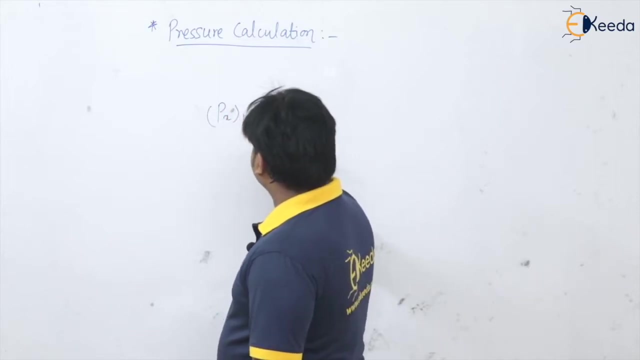 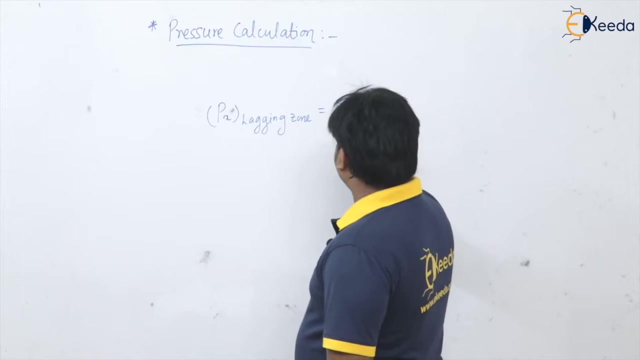 able to find out the uh pressure with respect to the uh thickness in the lagging zone, thickness in the leading zone and at the stationary pressure neutral point. so if you have the pressure px in the lagging zone, so it is given as the sigma y upon n into bracket. 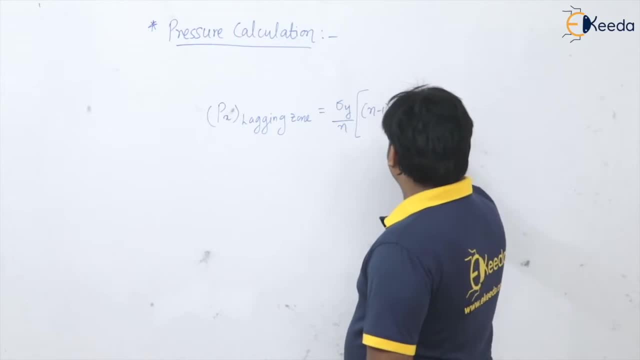 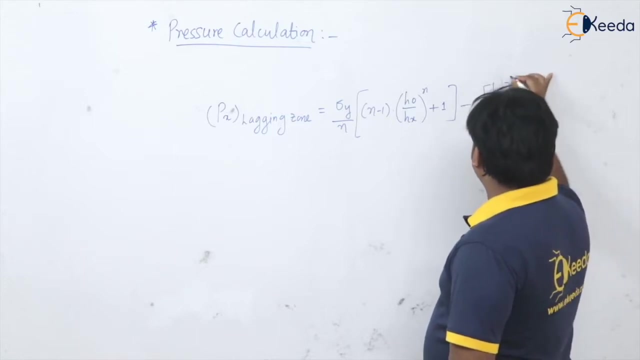 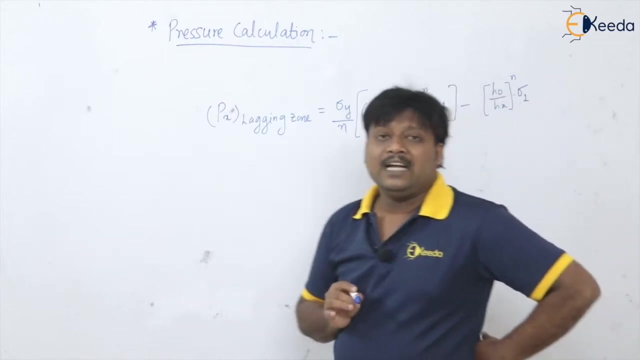 n minus 1 into H original, divided by H at X to the power n plus 1, minus this HO by H, X to the power n into, say, Sigma 1. so here Sigma 1 and Sigma 2 I am taking as the front and back tension, okay, so 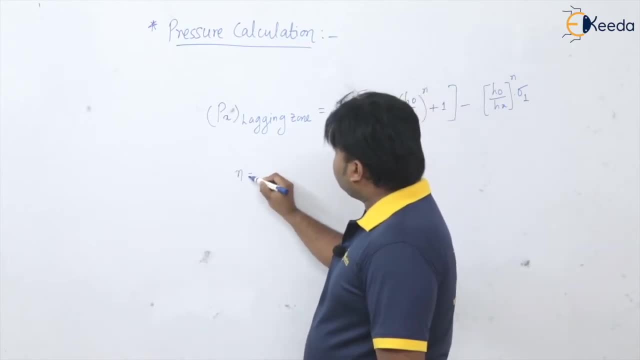 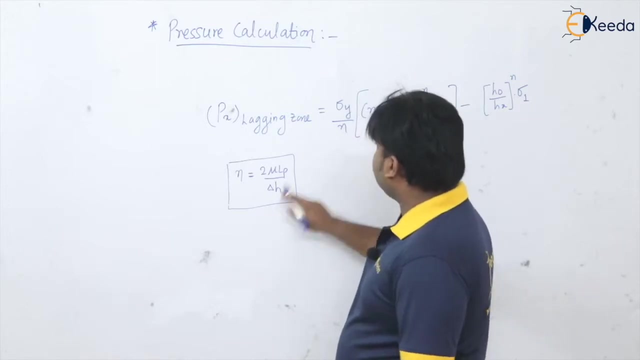 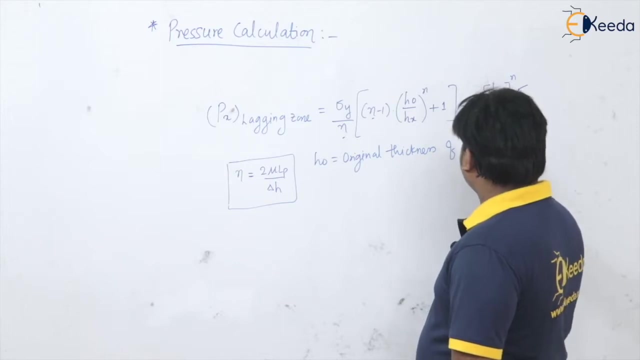 here this n that constant. I am taking as 2 mu LP divided by Delta H, that we will first calculate. we take this value, okay, and then we will you utilize this n value here. so H original is what our original thickness of the plate or strip and H X. 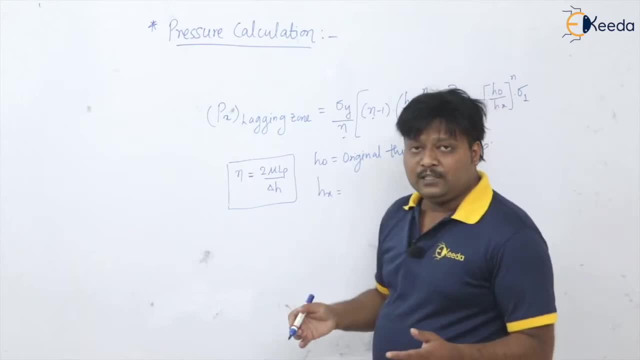 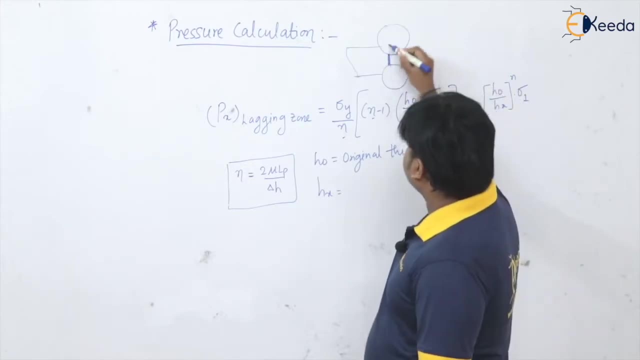 that. add in the lagging zone. you are getting this pressure at this particular thickness. say this is a neutral plane and if you go back to the neutral plane, the strip is lagging yes or no behind this neutral point. so it is a lagging zone. so H X will be from. say 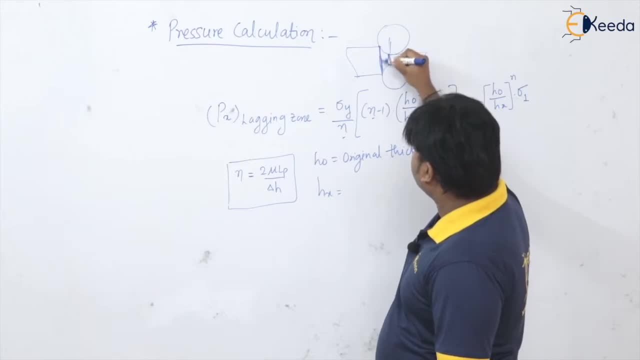 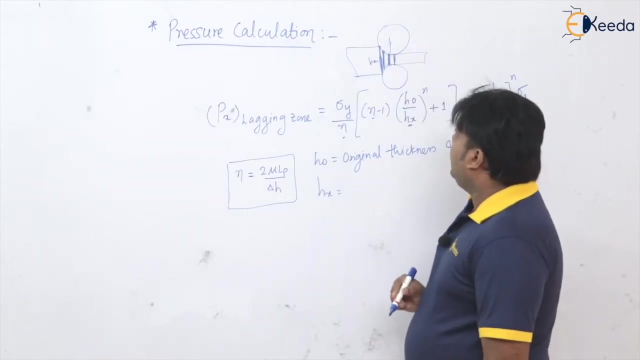 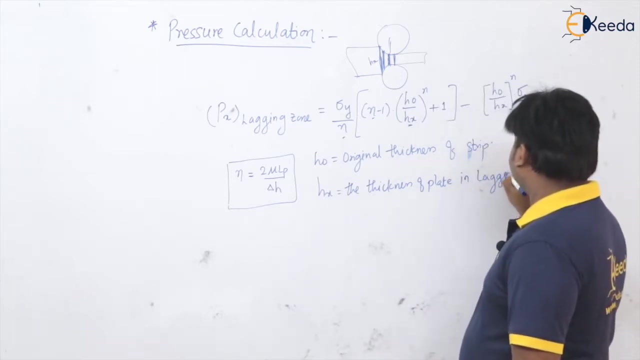 here to here this is the lagging zone and from here to here it is a leading zone. okay, so anywhere in this position we will have this value: H X- okay, so H X the thickness of plate in lagging zone, like that. now, if you calculate the pressure, 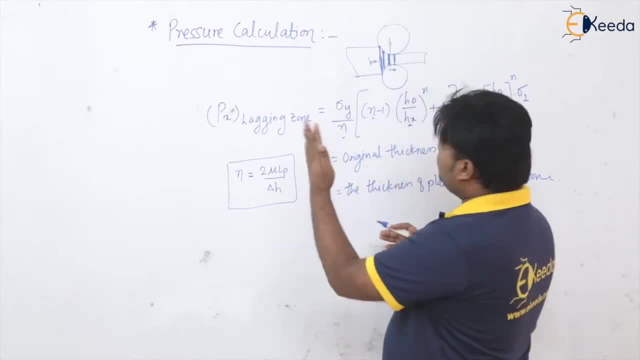 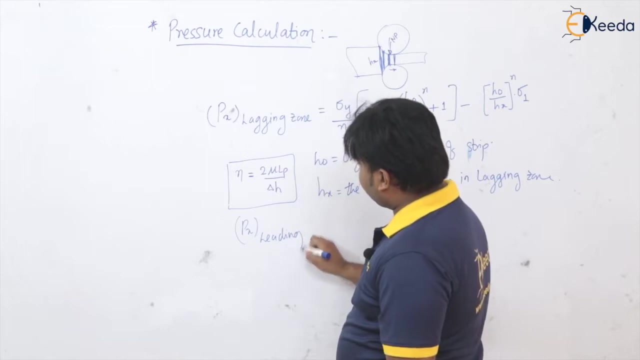 in the leading zone, that is, strip, is now leading ahead of this neutral point. so this is what our neutral point. so anywhere in this leading zone we can calculate the P X in the leading zone as equal to the Sigma y upon n into bracket n plus 1 into H X. 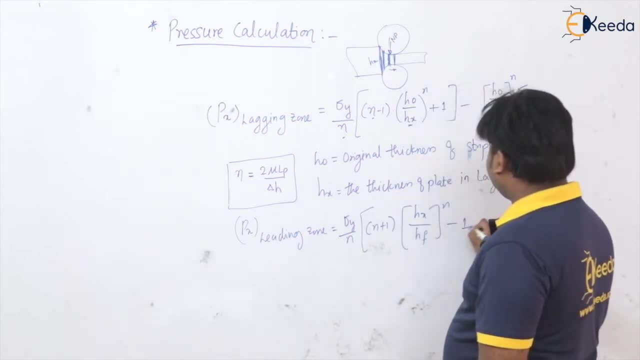 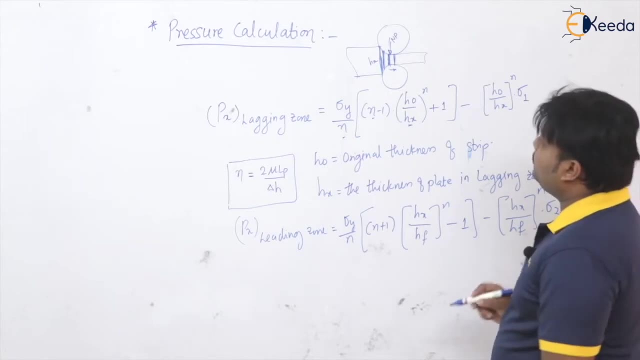 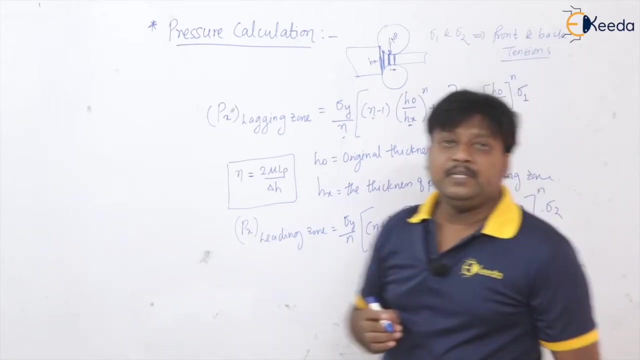 divided by H final to the power n minus 1 minus H X, by H F to the power n into Sigma, where Sigma 1 and Sigma 2 are what. these are the front and back tensions and we know why the reason behind these provision of front and back tension to 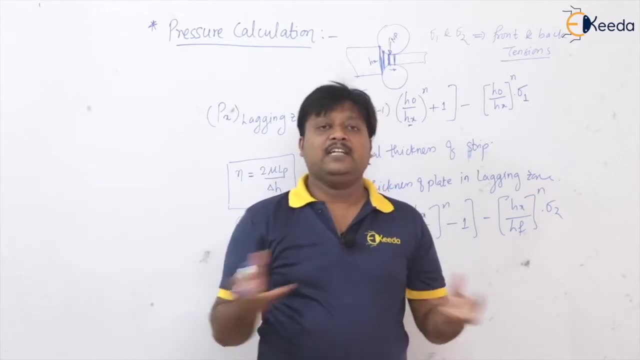 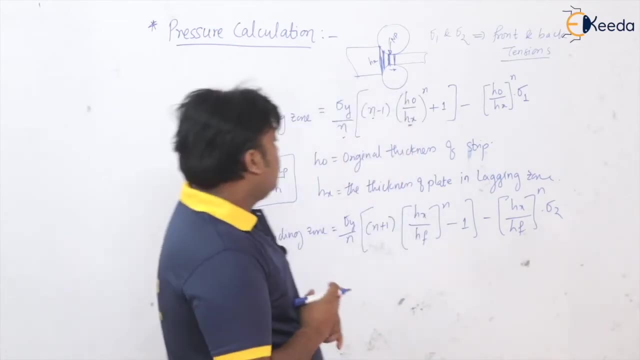 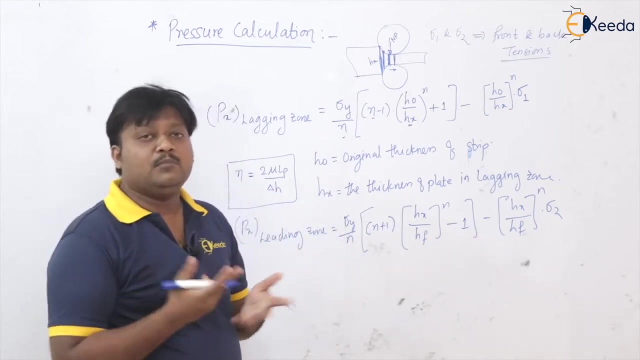 get the Poisson's effect so that we can reduce the role separating force. actually, We will see what is this force, role separating force. so if you have this pressure in the lagging zone pressure, what does? it? means we can able to calculate the pressure in the anywhere. 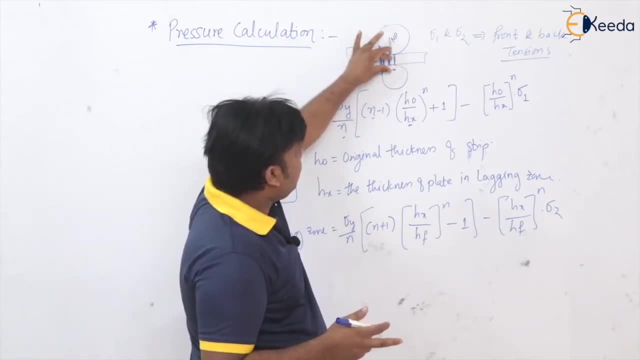 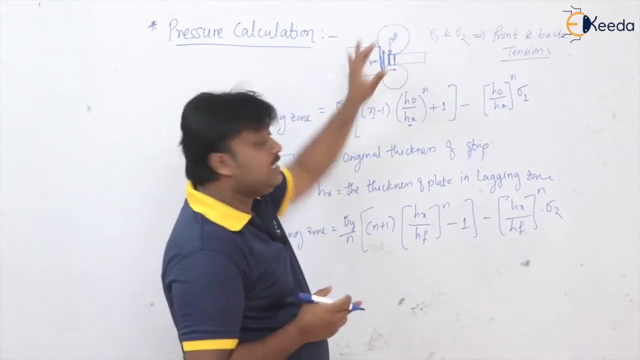 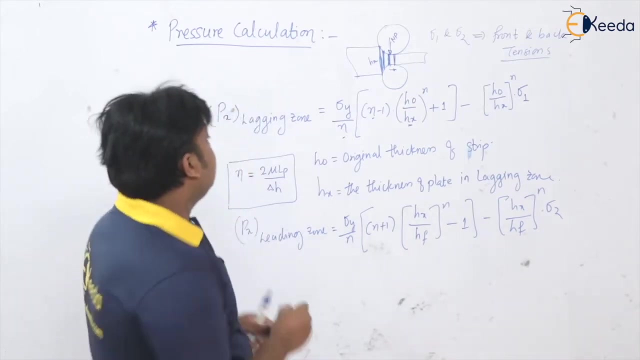 in this deformation. so either in leading zone, lagging zone and at the neutral point. so if you want to calculate the pressure at the neutral point, which is the maximum pressure, we know that what we can do, so there the thing will happen is that this H X will be now what this H X will. 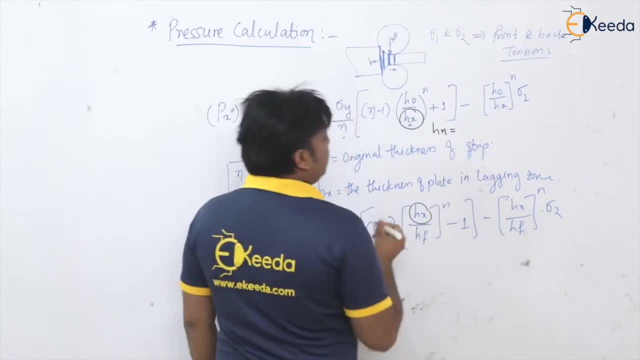 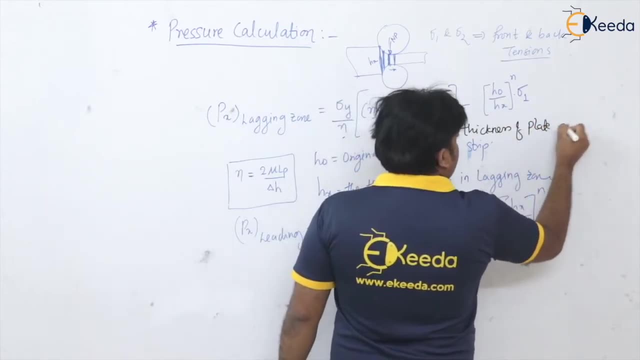 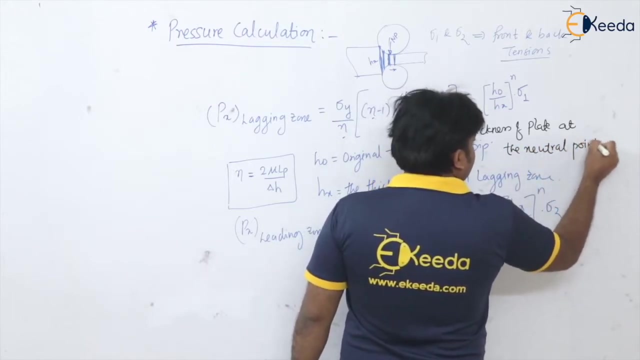 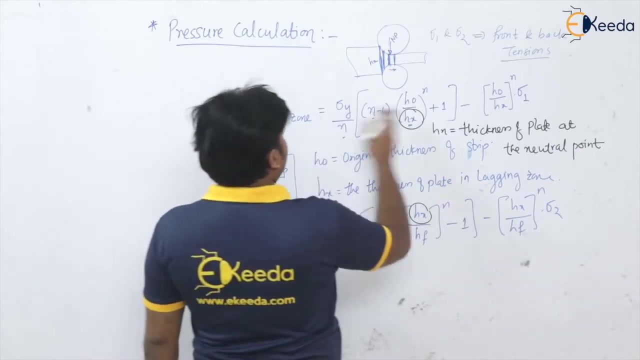 be what, the thickness of the plate or strip at the neutral point? the thickness of plate or strip at the neutral point, isn't it? and the pressure will be what maximum? so if this pressure at the leading and lagging zone your tenha equate at this neutral points, then what? 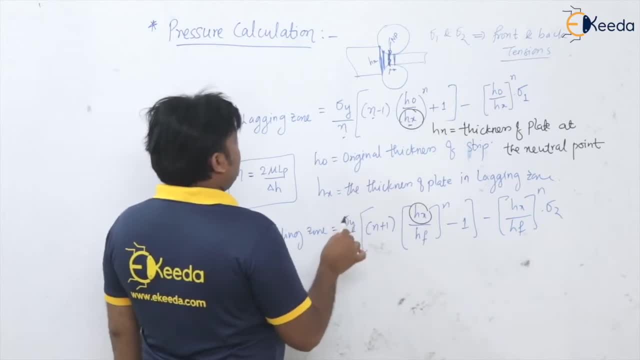 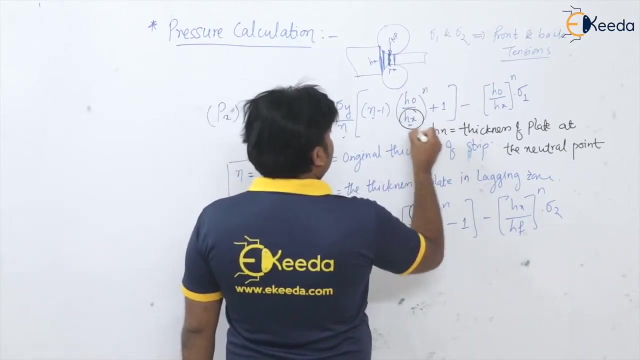 will happen. you will get the maximum pressure and from that what we can, we can going to equate this pressure. so both the pressures are same here. so at that point, what we can have, if you have the value of neutral point, thickness of the plate, you can easily 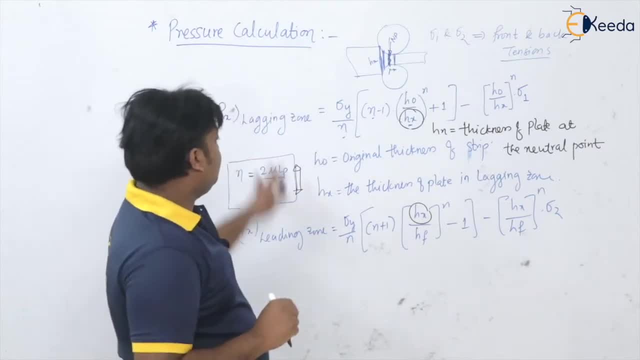 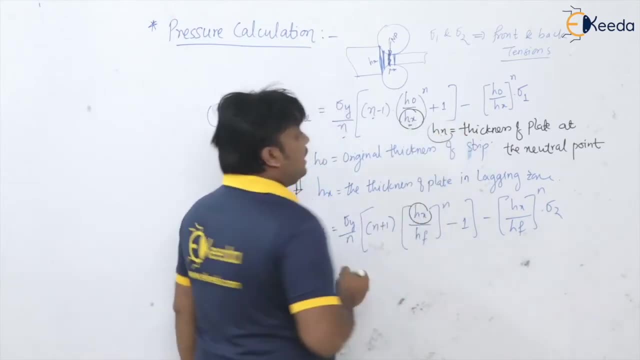 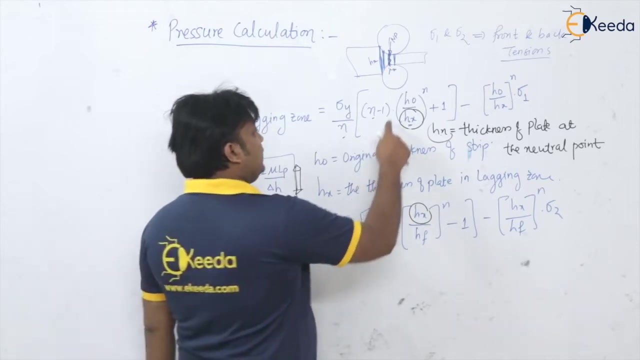 get the value for the maximum pressure pressure either put in lagging zone or in the leading zone. you put the value of hn, okay, then you can easily calculate the maximum pressure. or suppose, if you want to find out, anybody ask you to find out- this thickness of the strip at the neutral point, what we can do. so simply what we can do, we 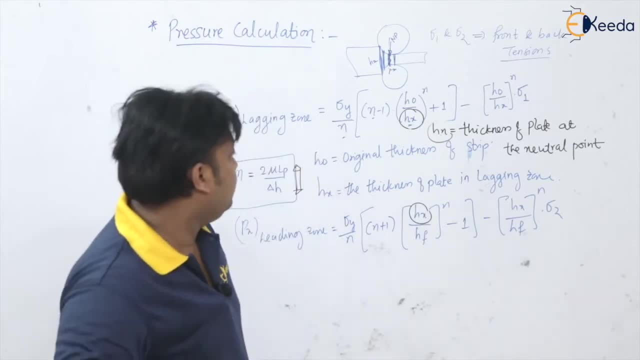 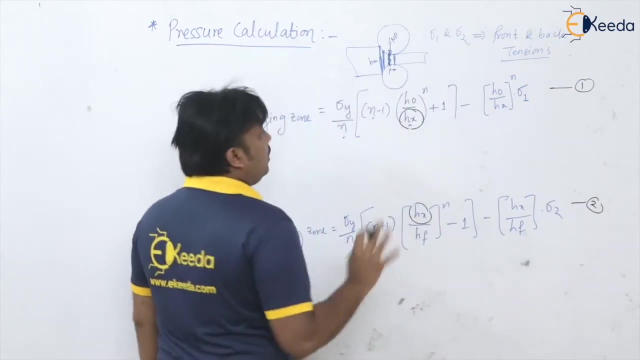 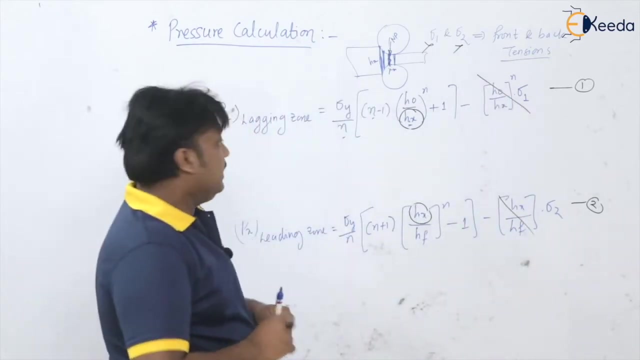 will equate these two equations. so what we'll get? so equate this, say, equation number one and equation number two. but the thing is that let us now for the simplicity. i am saying we are not applying the front and back tension, so these terms will get eliminated. so what we'll get? also this: 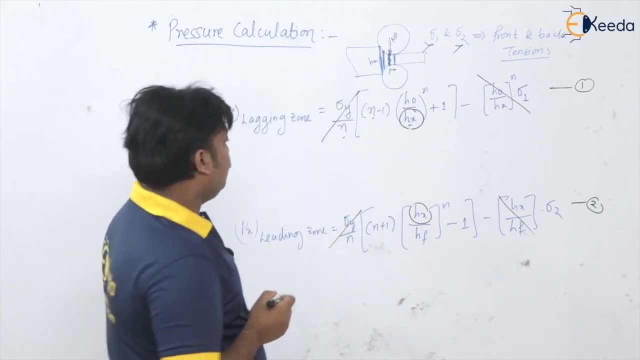 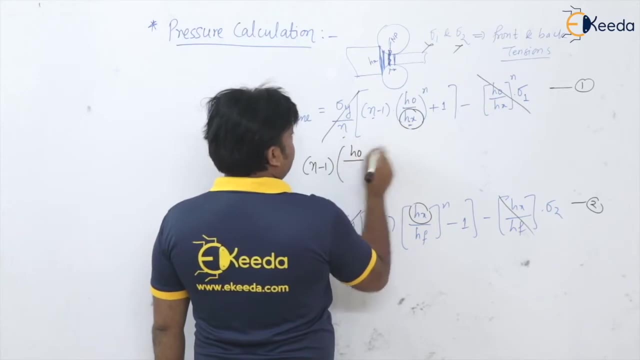 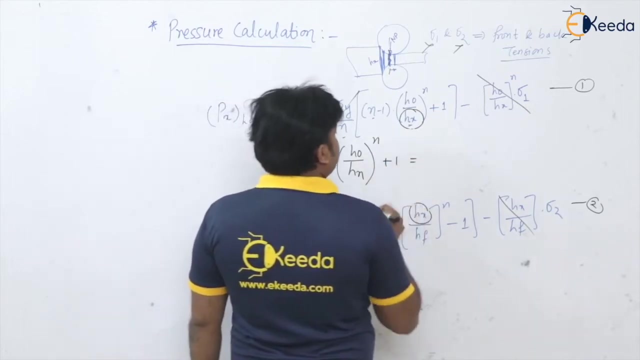 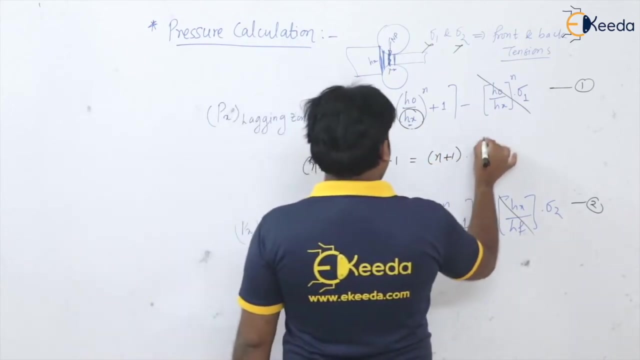 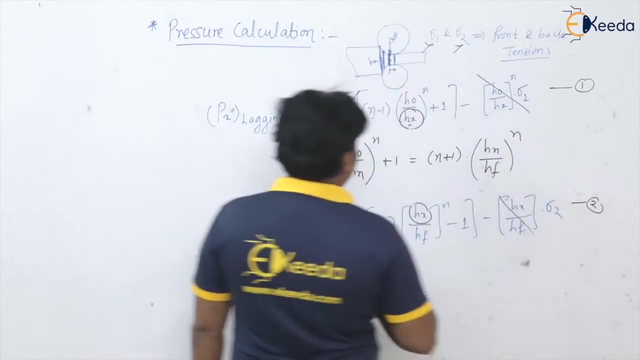 sigma y by n, sigma y by n get cancelled, so what we'll get that n minus one into h original, divided by this hx will not now be hn. thickness at the neutral point to the power n plus one is equal to this n plus one into h. n divided by hf to the power n. so from this equation by the 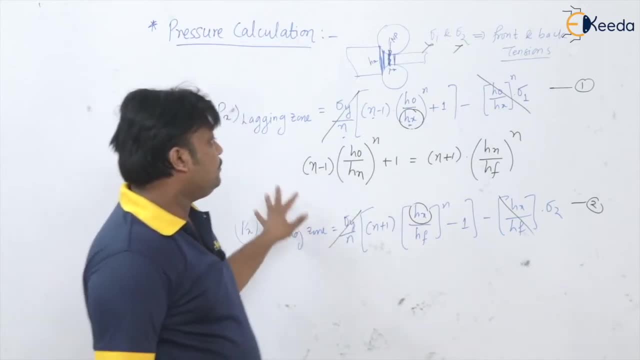 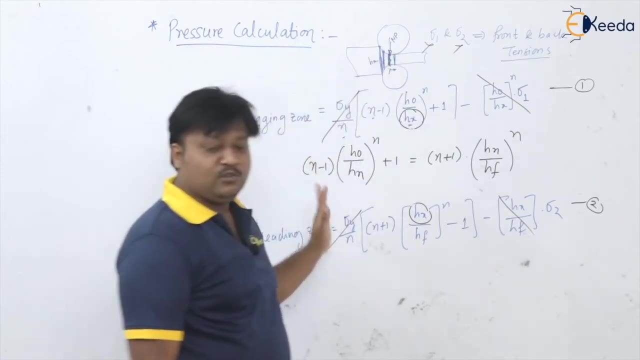 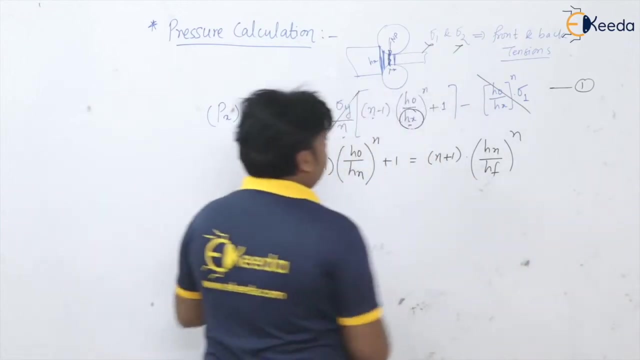 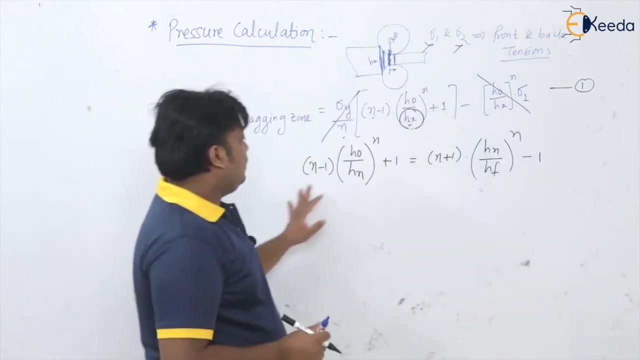 trial and error method, we can able to find out the thickness of the plate at the neutral point here. but see, this is time consuming. actually, trial and error, you will get the answer, but it is quite time consuming, okay. so here it is minus one. no, it is minus one. so for the n, as we know, 2 mu l by mu l, p by delta h, this is the value of n. 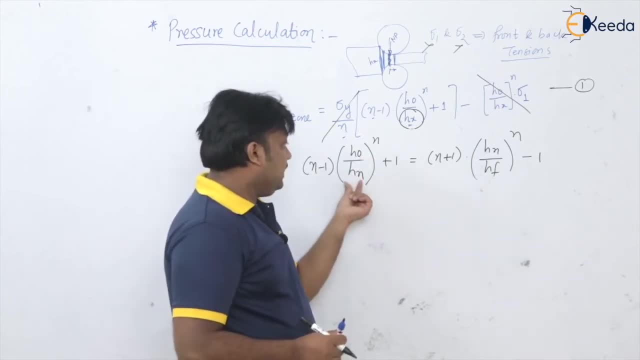 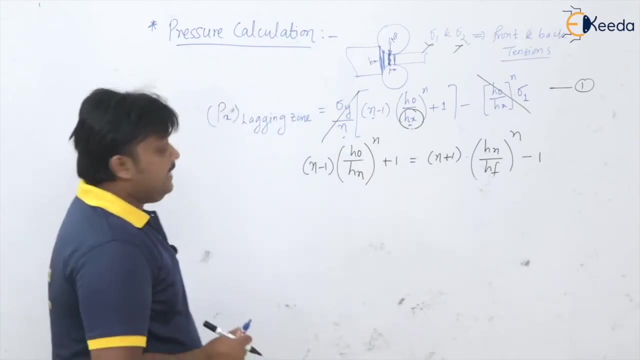 h? o is the original thickness, hf is the final thickness and hn. you can get the value for the thickness of the plate at neutral point. okay, so this is ringing ting to reach n into one minus first, one into h, in거야 u. so this is for pressure calculation. 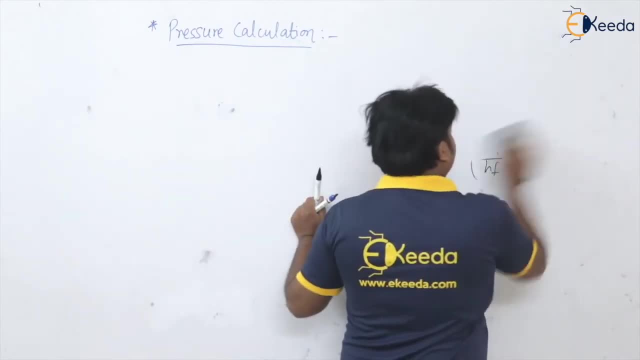 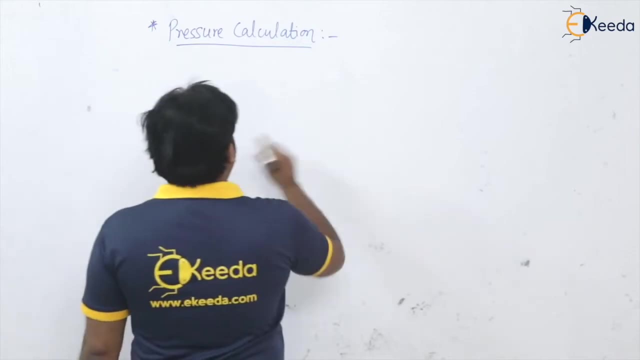 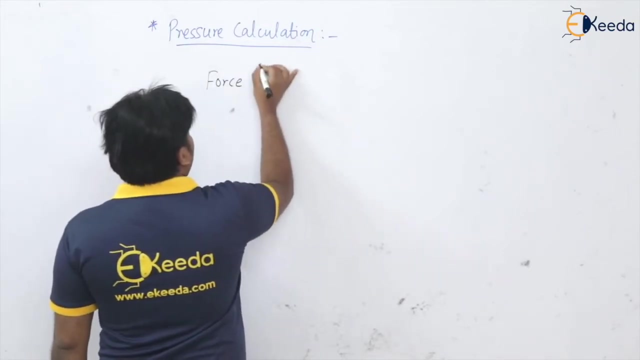 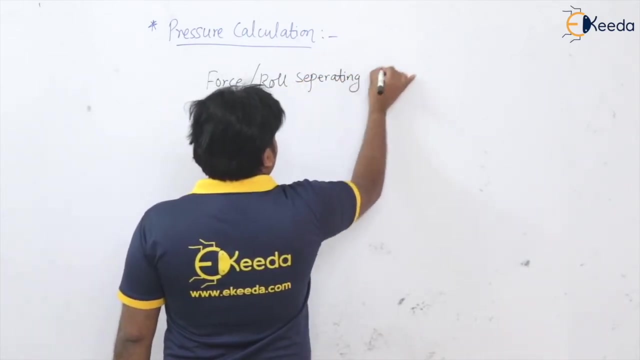 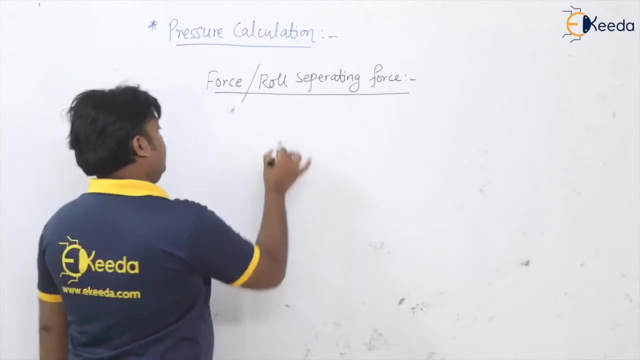 Now, once you get the pressure. once you get the pressure is meant to be force in the loading operation, rolling operation. okay, force, or this is also called as roll separating force, not more than an ordered twenty percent force force. so in the rolling operation, these rollers are compressing this plate, isn't it? and they are. 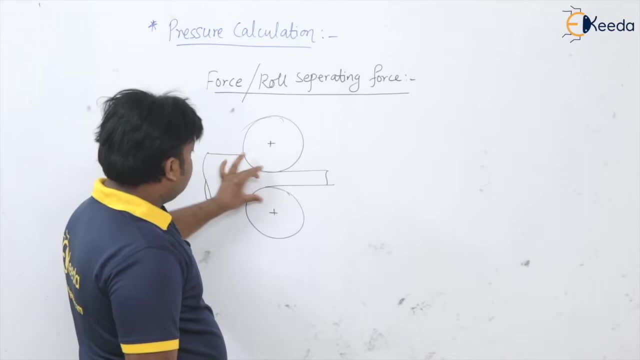 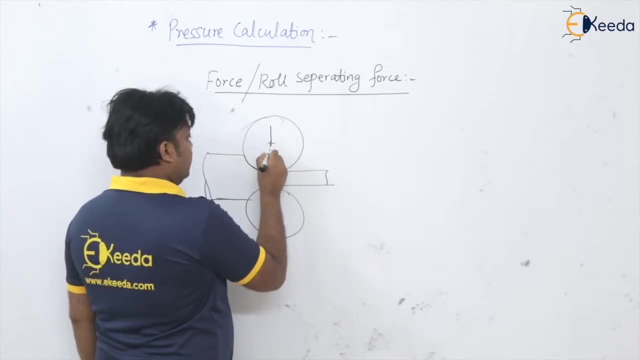 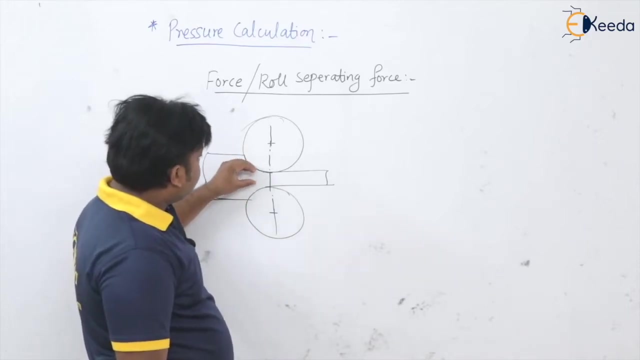 giving the, the huge amount of force on to this strip, so streety strip is also giving, as we know, the reaction, isn't it? so, because of this reaction in opposite direction, these roles are trying to get separate, isn't it? and that is the name why this force is also called as the role separating. 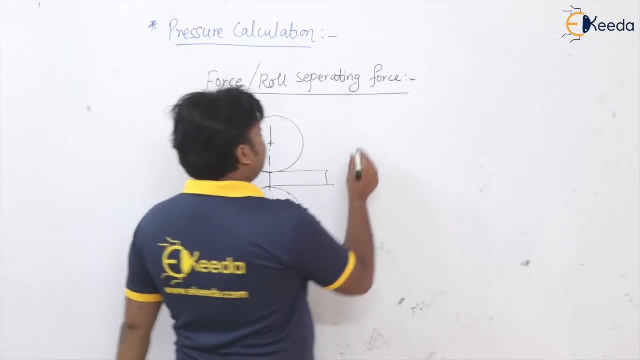 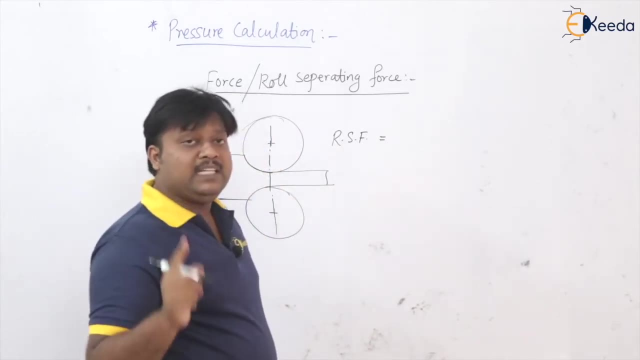 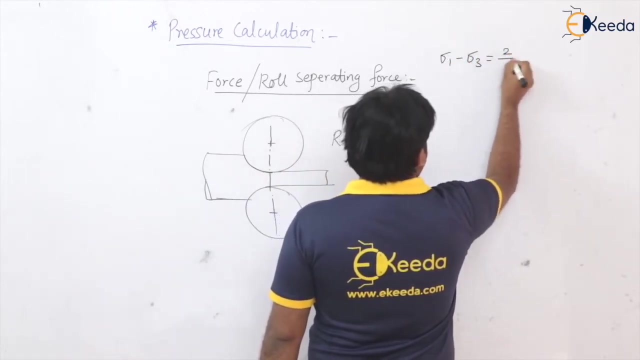 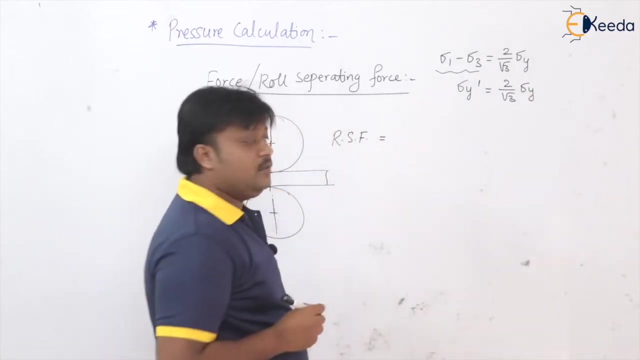 force. okay, so this role separating force, rule separating force, okay, by considering the plane strain condition, that is, you know that this sigma 1 minus sigma 3 is equal to 2 by root 3 times sigma yield strength. okay, this is nothing but say sigma y dash is equal to 2 by root 3 times sigma y. we know this okay from because 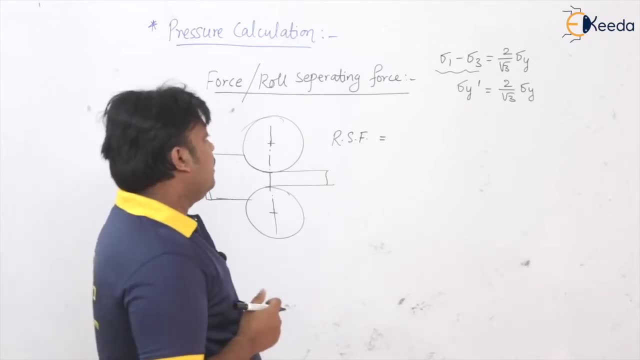 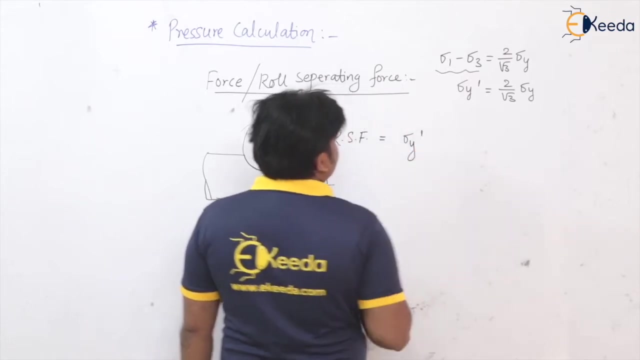 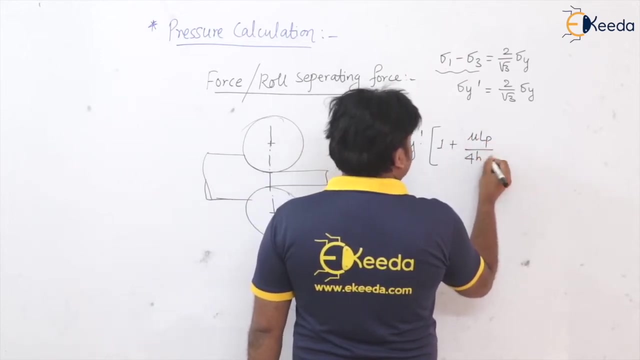 we are assuming that the rolling is the plane strain. where plane strain is valid, plane strain condition is valid in the rolling process. so there is no widening of the width, only along lengthwise direction material is going to deform. okay, so this role, separating force, so it is equal to this sigma y dash into 1 plus mu lp divided by 4 h average. 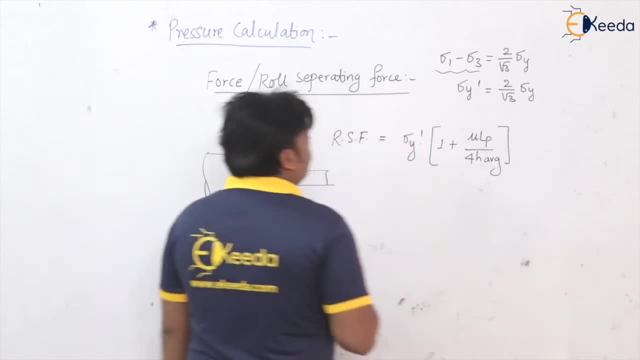 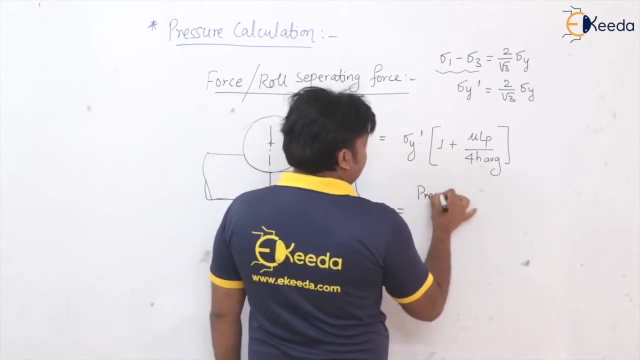 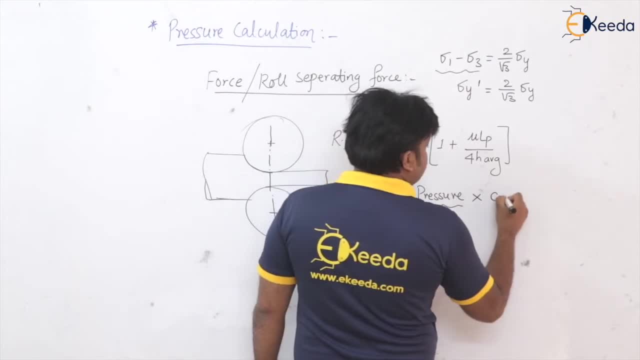 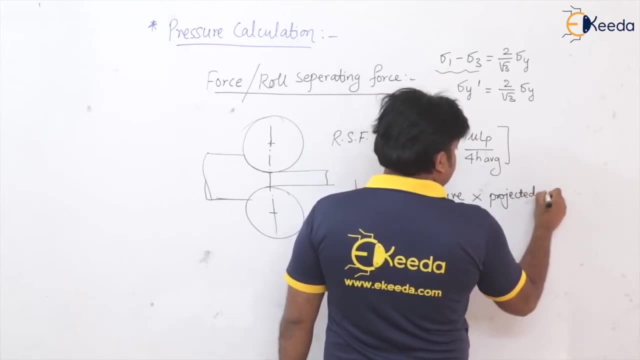 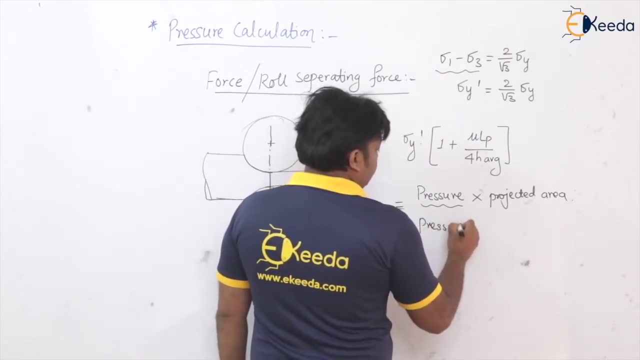 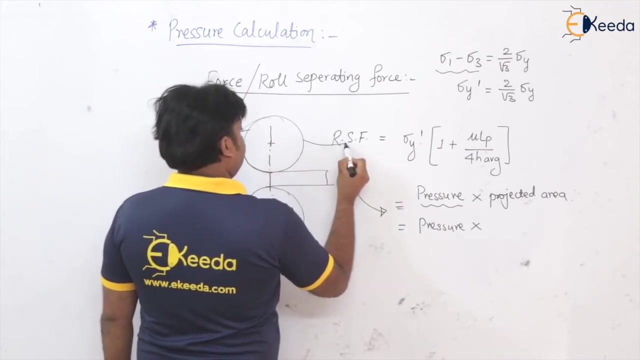 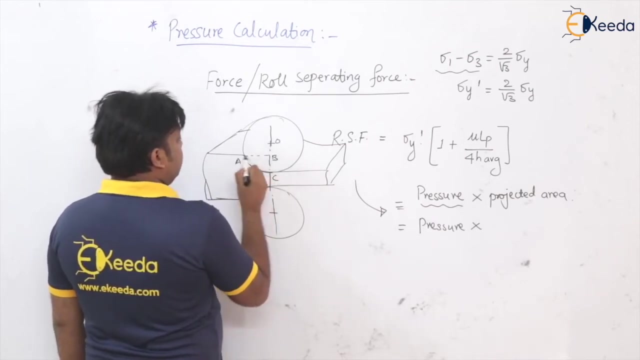 this pressure value by this contact area, or you can say this projected area, actually this projected area, what we can get this pressure into. what is projected area? see here, we already discussed about this. so this, this value, o, a, b and this is c, this a, b, our what length of arc of contact? so this length? 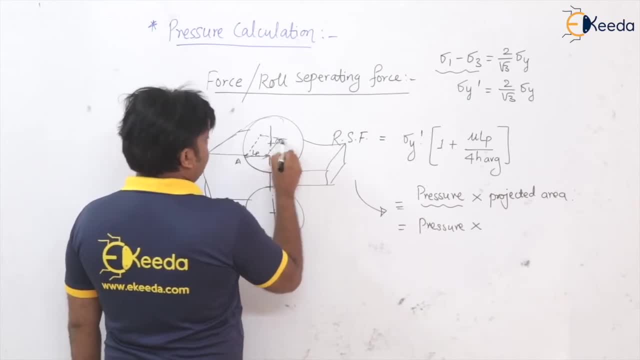 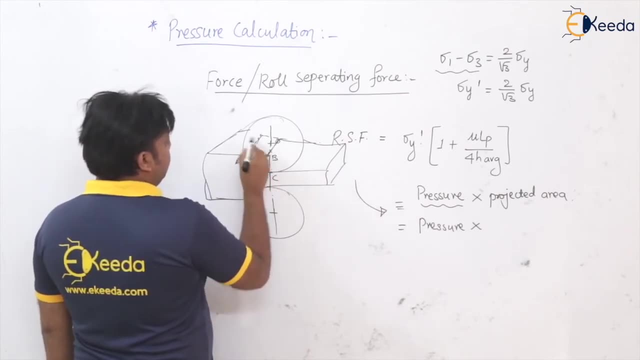 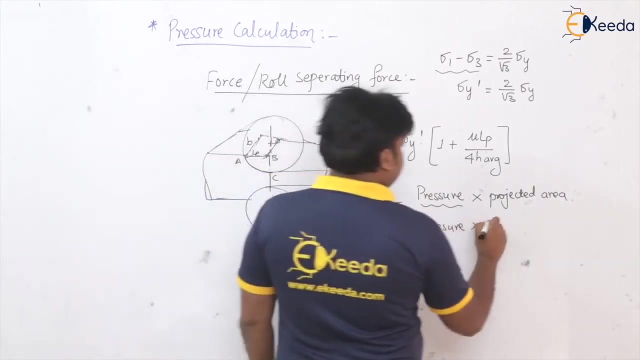 of arc of contact into this width of the strip and width is going to be same throughout the operation. this l? p, this length of arc of contact into this width b- this is our projected area. okay, so pressure into this projected area. what? this width of the plate into this length of arc? 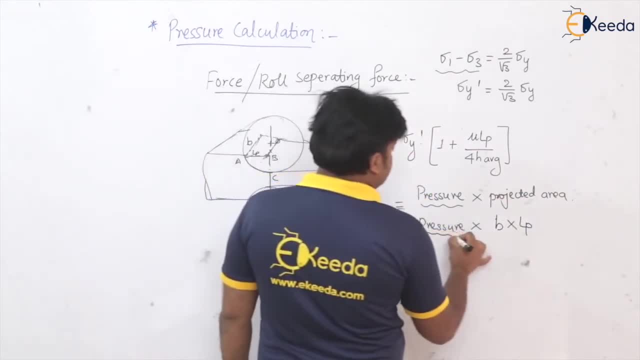 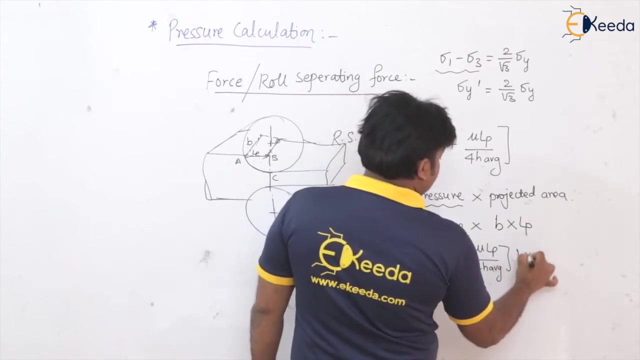 of contact. so here pressure. in simple fashion we can have this sigma y dash into bracket 1, plus mu l p by sigma y dash into bracket 1, plus mu l p by sigma y dash into bracket 1, plus mu l p by 4 h average into b into l p. okay now, what is the sigma y by plane strain condition? 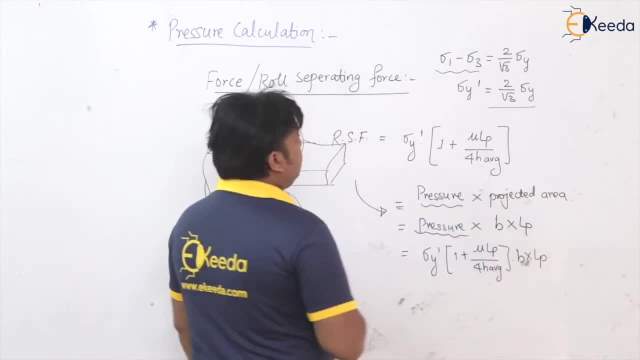 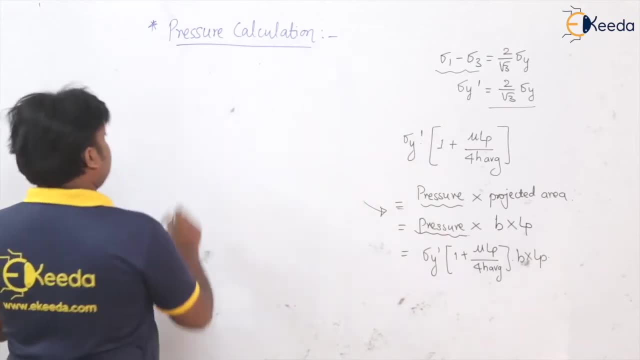 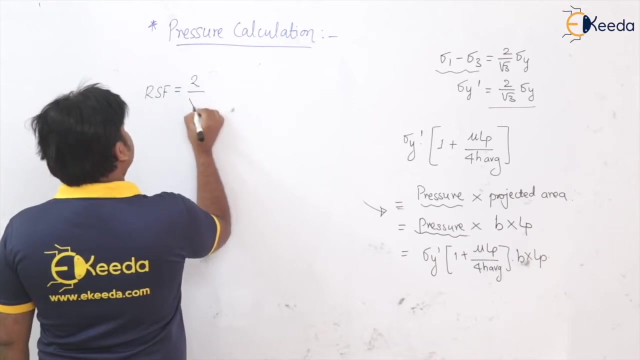 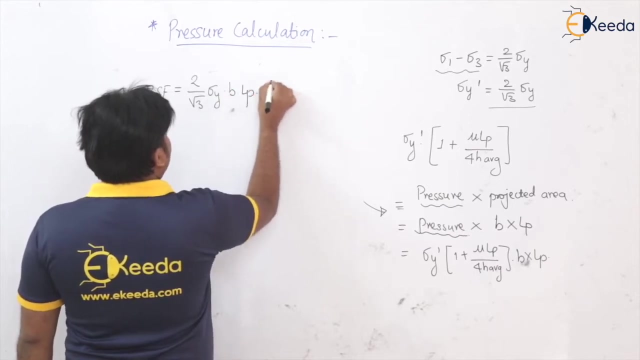 it is 2 by root, 3 sigma y, isn't it? so we will again write in simple fashion the role separating force as this: rsf, as what? sigma y dash is 2 by root, 3 times sigma y. sigma y dash is 2 by root, 3 times sigma y, into b, into l p, into bracket 1, plus mu l p divided by. 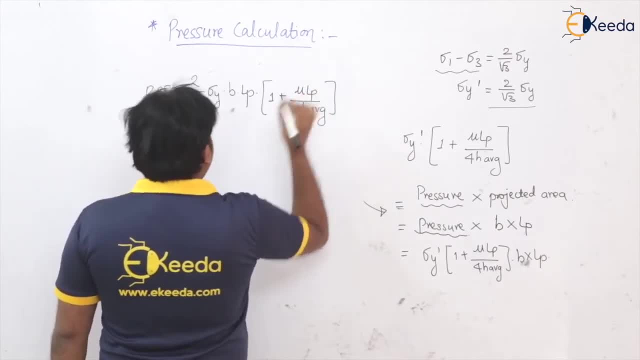 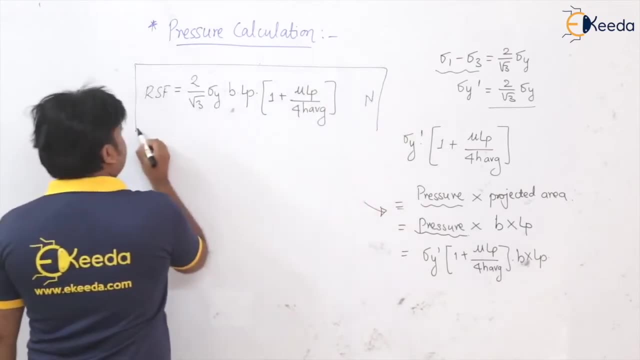 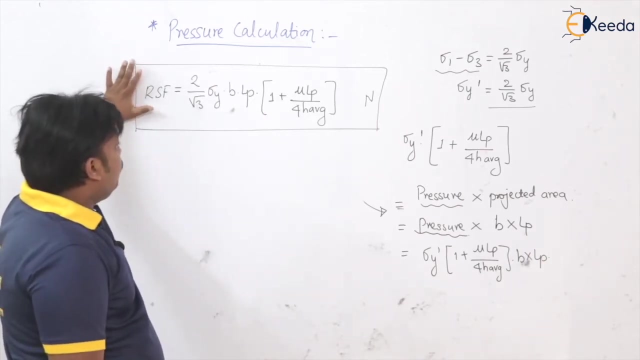 4 h average. so this is our role: separating force in newton, very, very important. dear students, you have to keep this formula in your mind. okay, always 2 by root, 3 times sigma y is the width strength of the material: b l p into bracket 1, plus mu l p by 4 h average. you know what, how to. 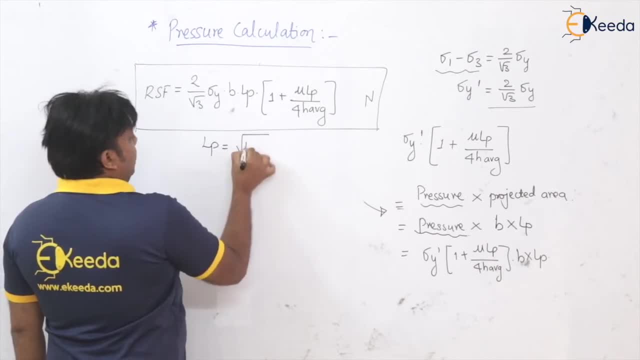 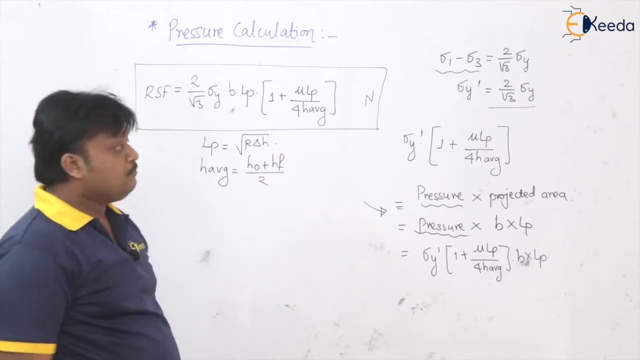 calculate l p under root r times. delta h b is given. it's a width and h average you can calculate as original thickness plus final thickness divided by 2. okay, so this is the role separating force, please remember, okay. okay, so this is the role separating force, please remember. okay, so this is the role separating force. 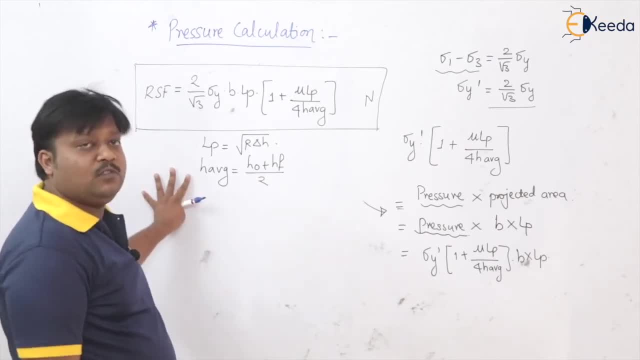 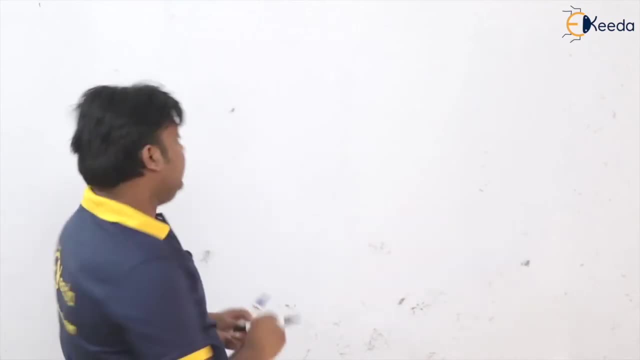 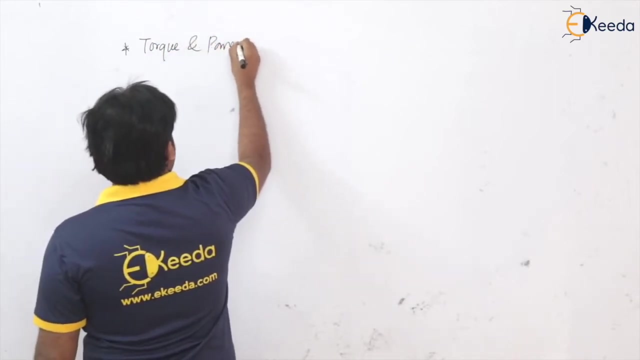 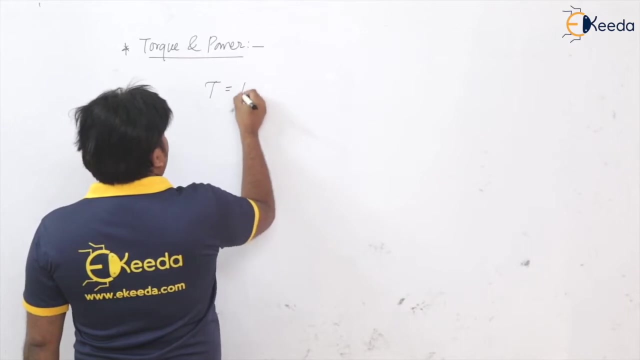 now, once you get this role separating force, now it is very easy to calculate the torque and power in the rolling operation. let us see now what we are going to see: the torque and power. so please remember that torque is what actually- this role separating force multiplied by distance. 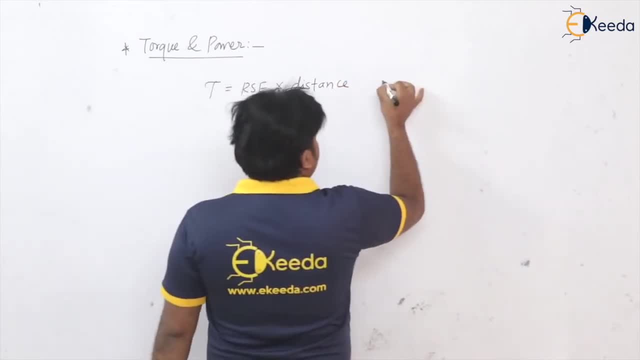 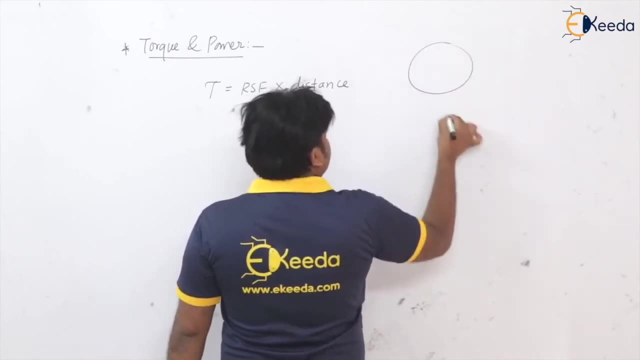 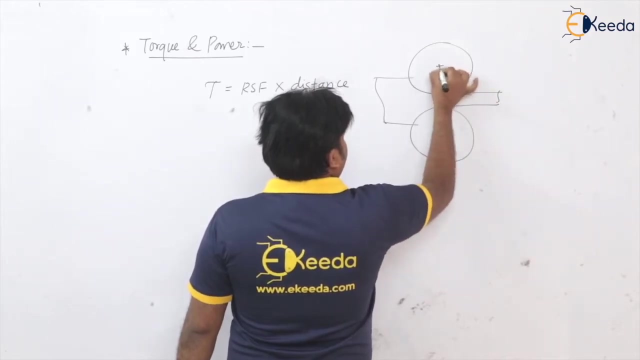 so your distance, actually the entire force is applied along this length of arc of contact. please remember, in the rolling process, if this is the rolling operation, so this is the center of the rollers. so this distance, please remember, we know that this is what the length of arc of contact, or length of 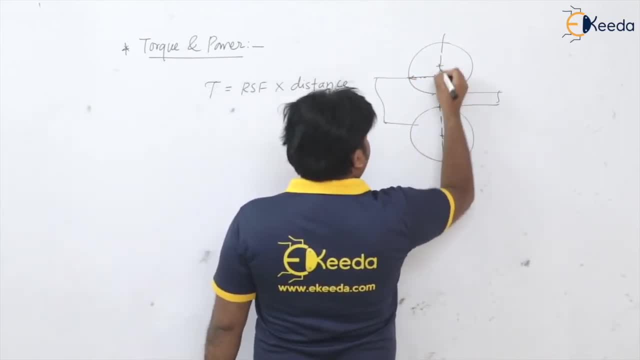 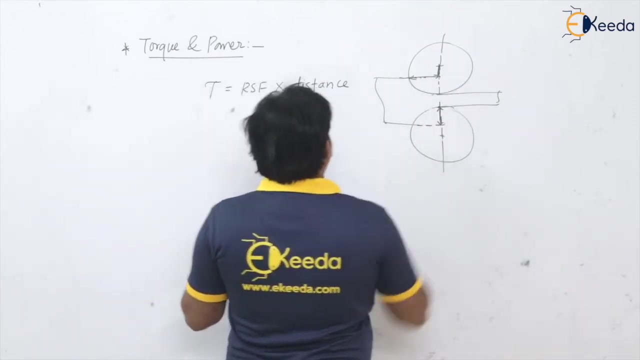 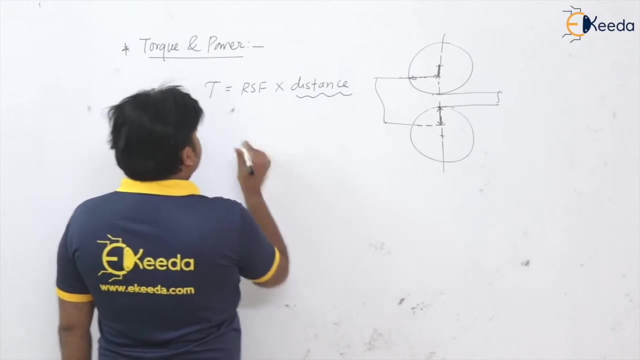 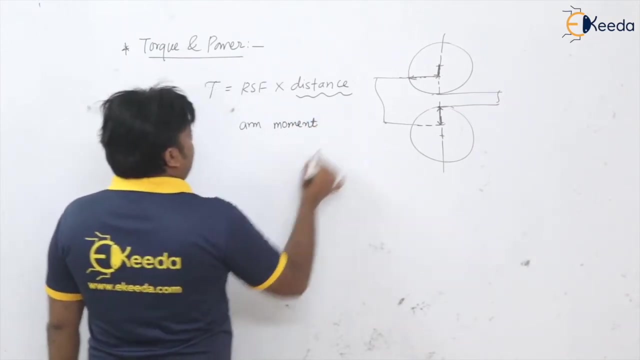 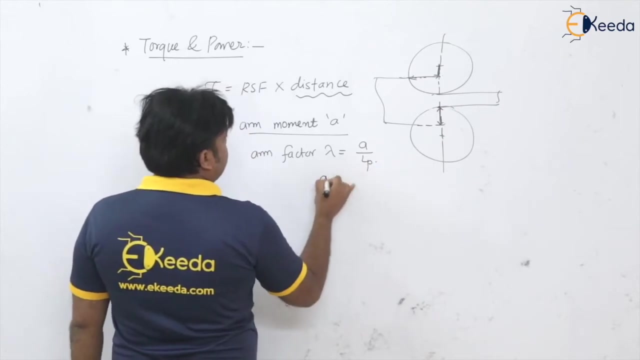 deformation. so from the center of the roller, okay, to this distance, okay. so whatever the forces are acting are along this length of arc of contact. so this distance we are taking as the arm, the arm movement, the arm movement, learned arm movement, as a, okay, okay, and there is a relation, for the arm factor, which is lambda, is equal to a upon lp. so we get they. 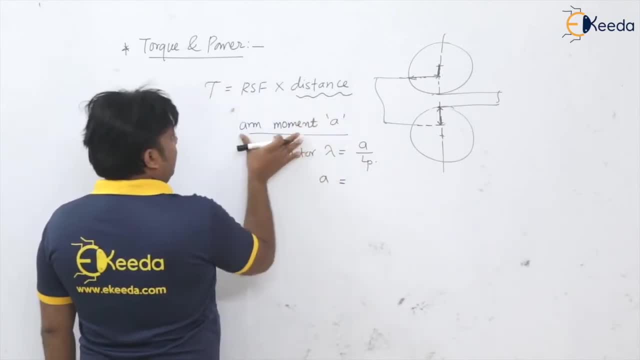 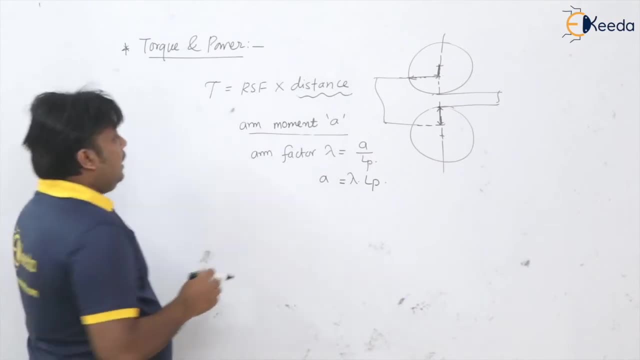 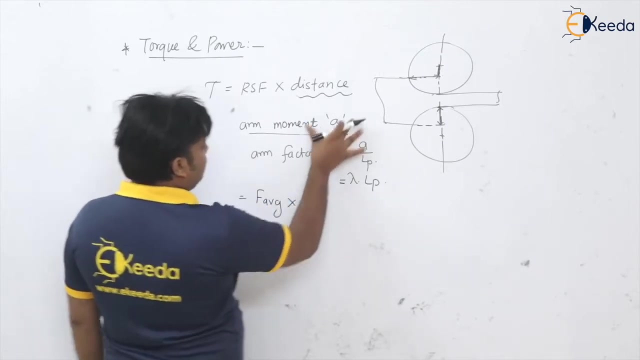 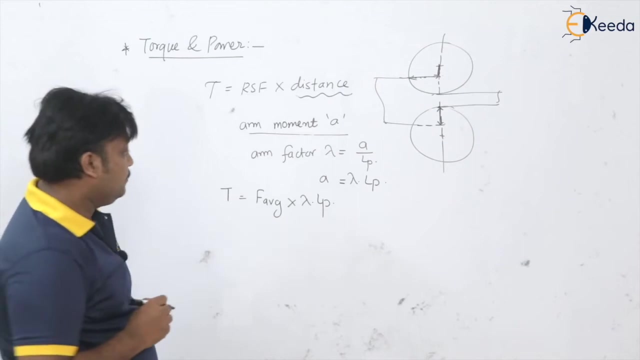 get this a as arm, arm movement, which is nothing but the distance as lambda times lp. okay, and you know this say role. separating force is, say f, average force into distance is what this lambda times lp. so this is our torque, please remember. and this lambda value is basically taken. 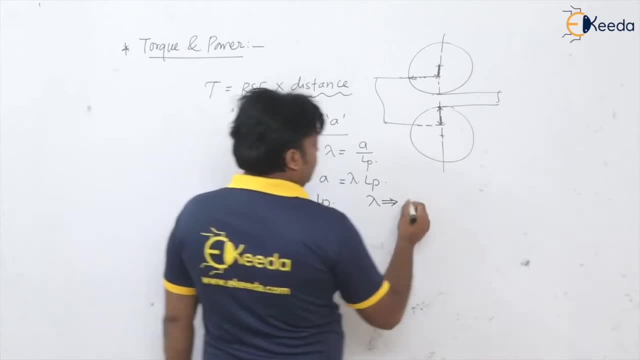 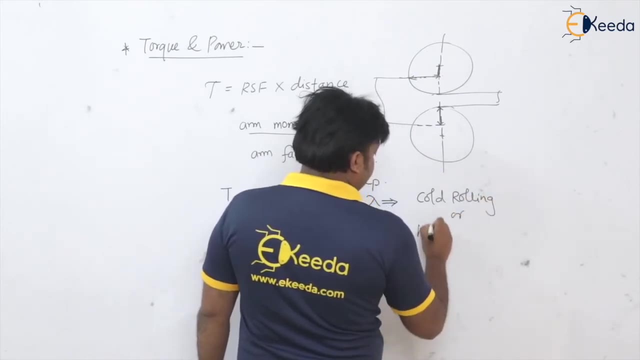 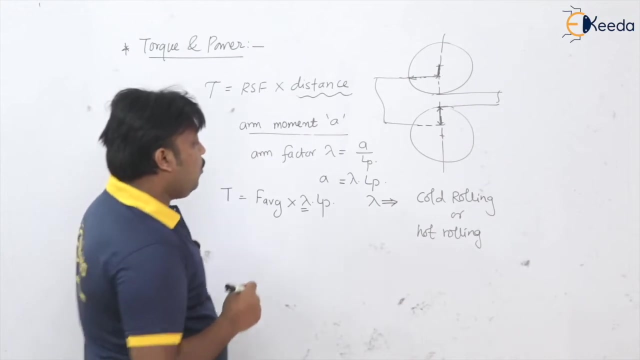 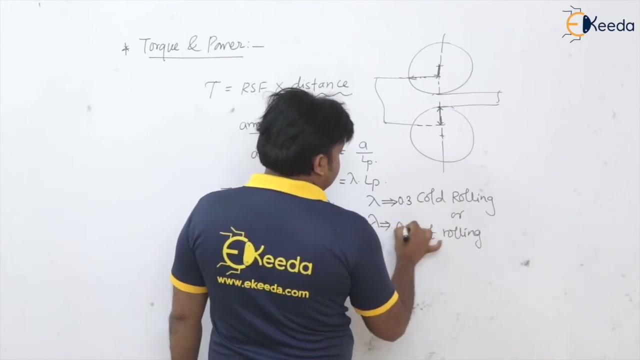 on the whether the rolling is cold rolling or hot rolling, and we know that the, unless otherwise stated, rolling is what it is: the hot rolling. so, lambda for cold rolling, it is taken as 0.3 and lambda for hot rolling, it is taken as 0.4. please remember. 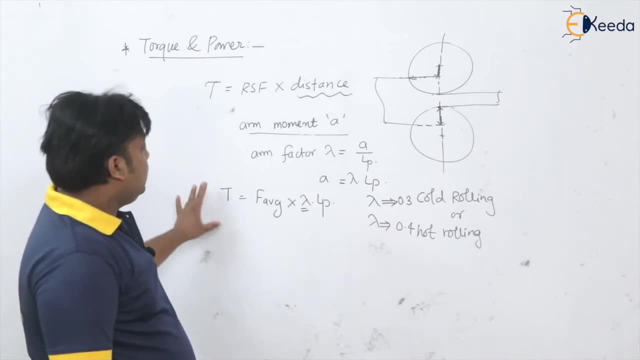 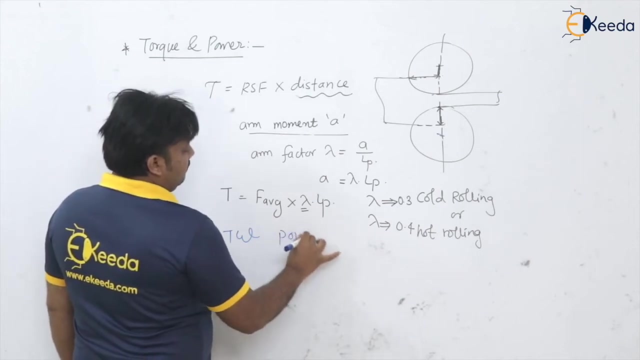 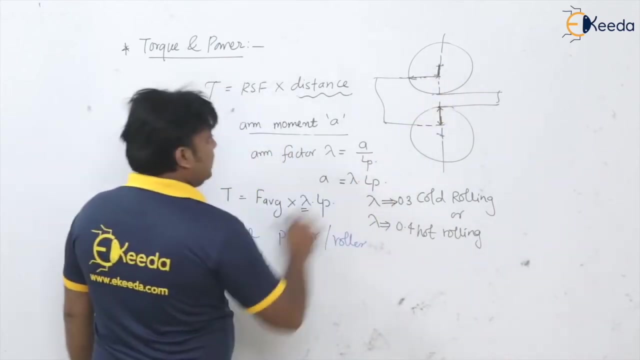 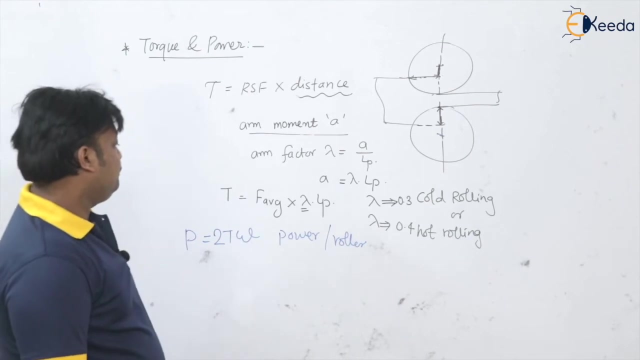 so you get this torque, isn't it? now, what is power? you know that power is equal to what? t times omega? okay, and here there are of course how many rollers? so this is the power in watts: power per roll per roller. okay, so total power is equal to 2 times T into omega. okay, 2 times T into omega. so let us elaborate. 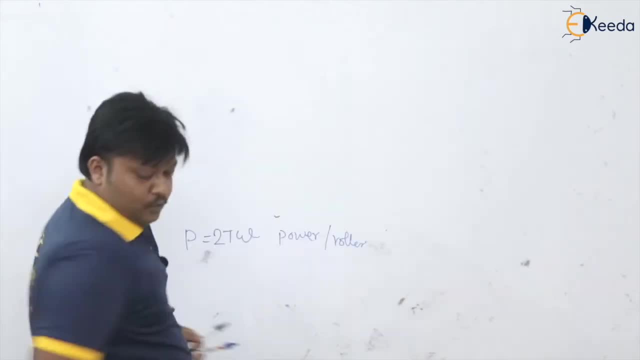 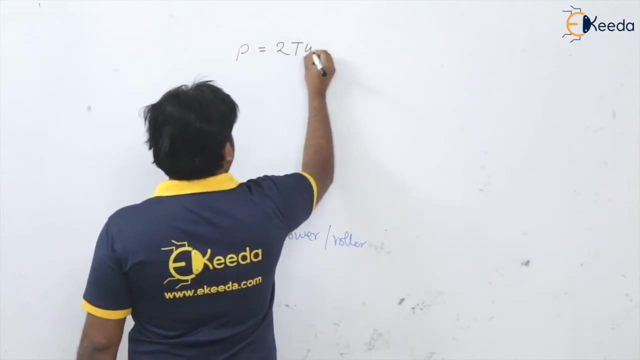 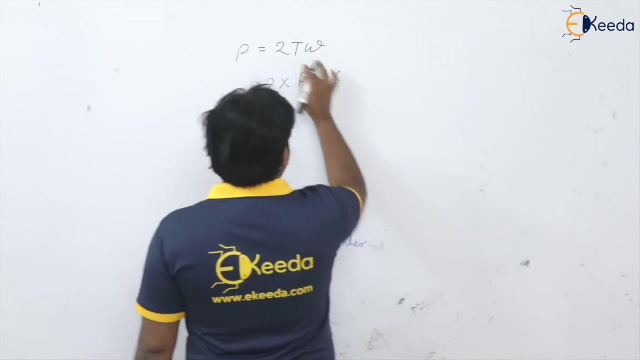 the formula here. so you got the torque. now the power is equal to what this 2 times t, omega. now put the values of all the things 2 times power- torque is what- into this force. average, into what this arm factor into lp, that is your arm movement. 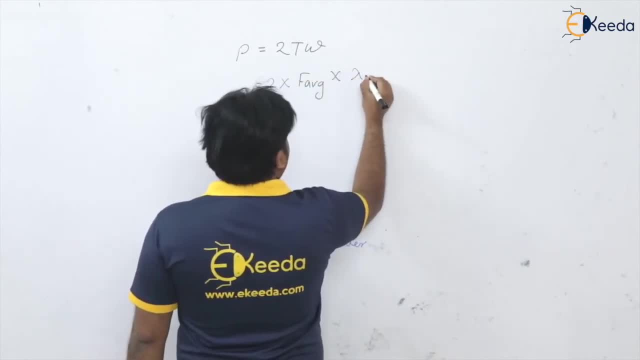 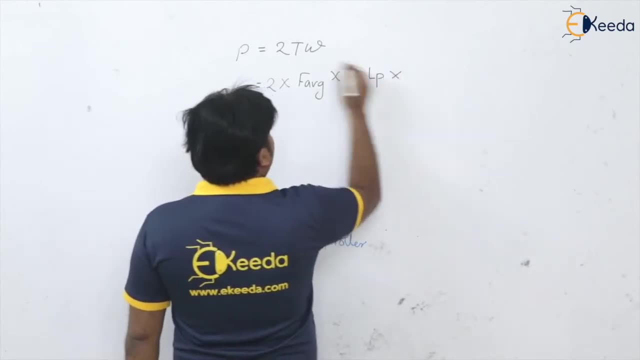 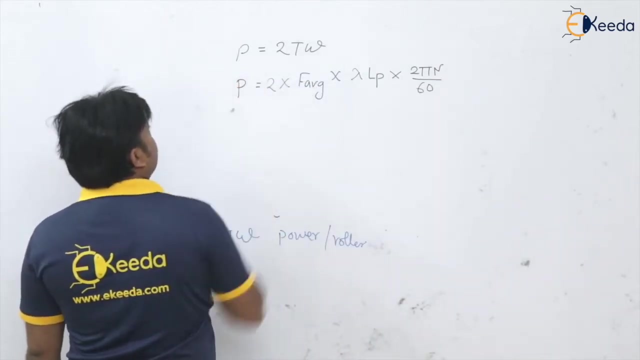 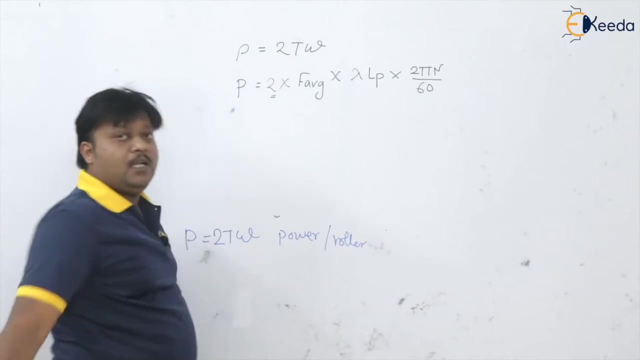 into lambda times, lp. okay, so force into distance, torque over here into omega is what 2 pi n divided by 60. very good, so you get the power here, total power, because i have multiplied here c with the 2. if not, it will be the power per roller. so you know what is. 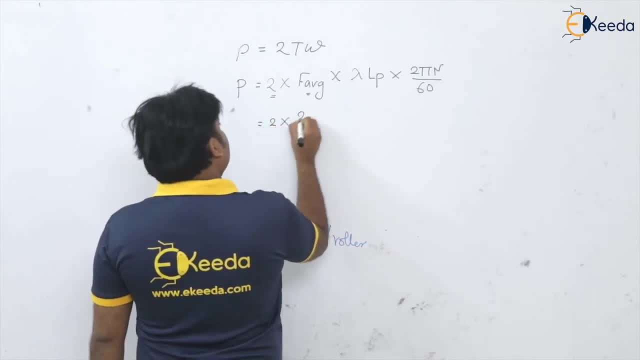 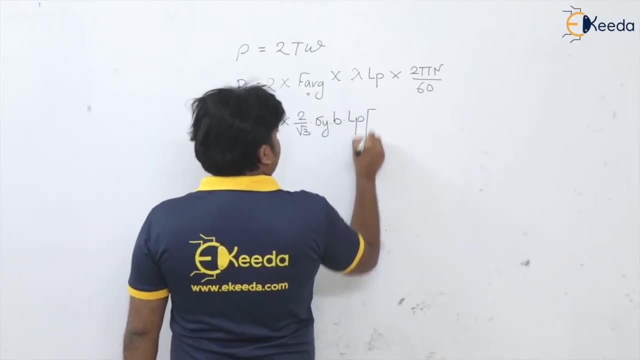 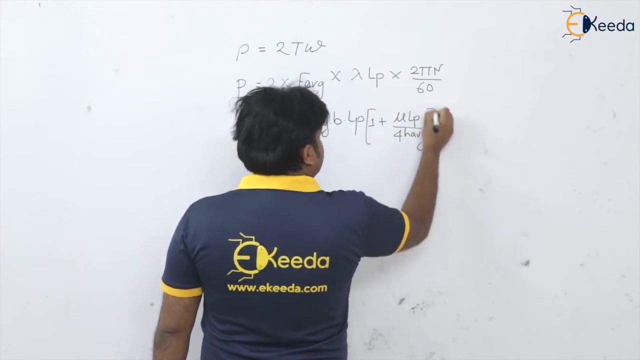 f average of role separating force. so 2 into 2 by root, 3 times sigma, y times b times lp, into bracket 1 plus mu times lp divided by 4 h average. please see these are: this is a empirical formula we have chosen here. okay. 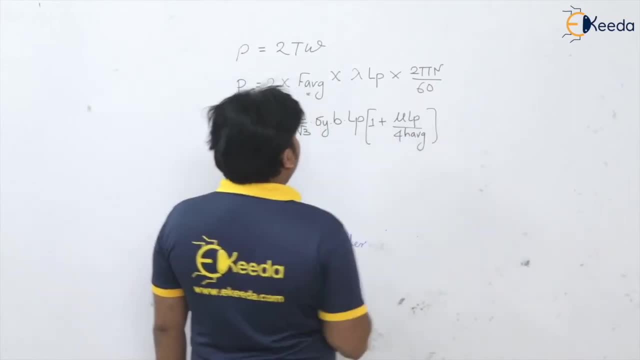 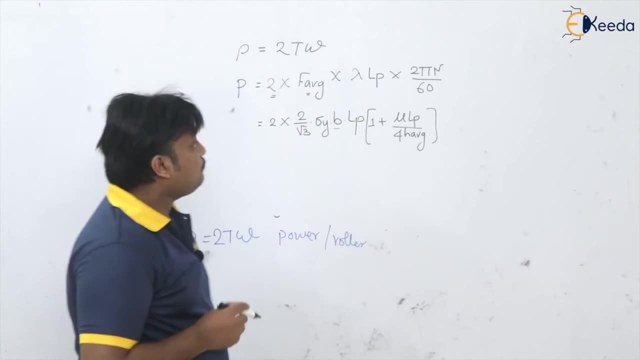 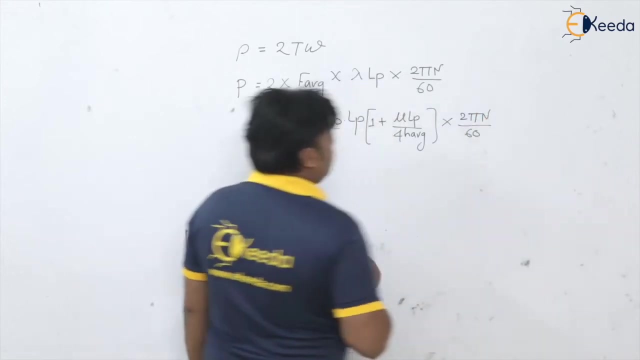 this sigma y into 1 plus mu lp by 4 average for the pressure. please remember, otherwise this area will be this: b times lp is the projected area and omega is what 2 pi n divided by 60 n is what the revolution per minute for the roller. so if you put this: 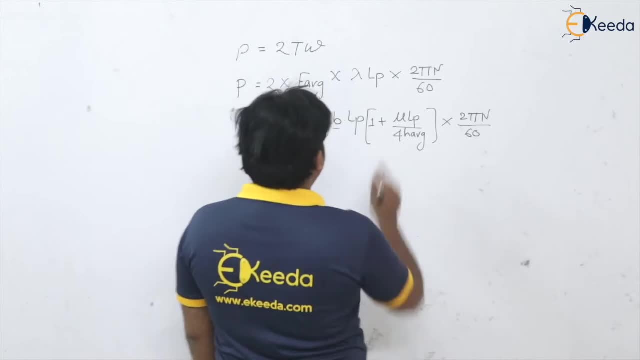 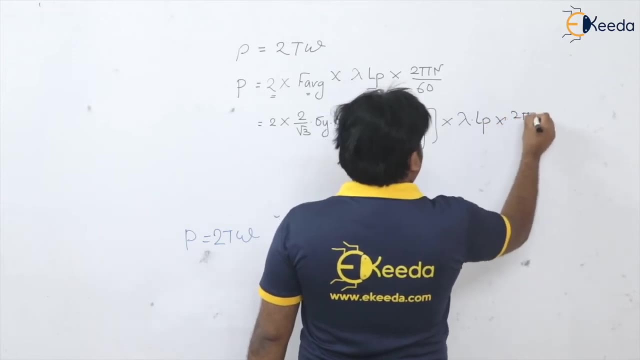 all the values here. so lambda p is left here. so here i will write plus lambda times lp. this is the problème, that this is the problem about this. anchor LP into 2 pi n divided by 60. so this is the power in watt you will get the power. 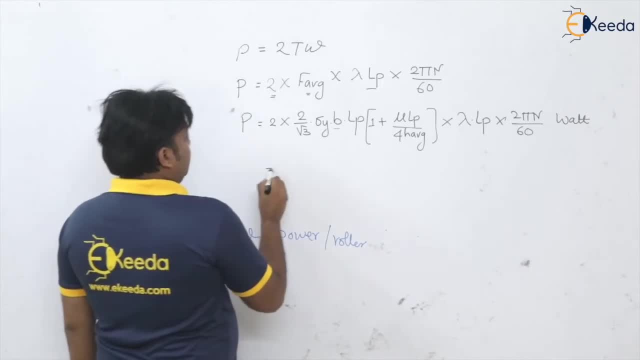 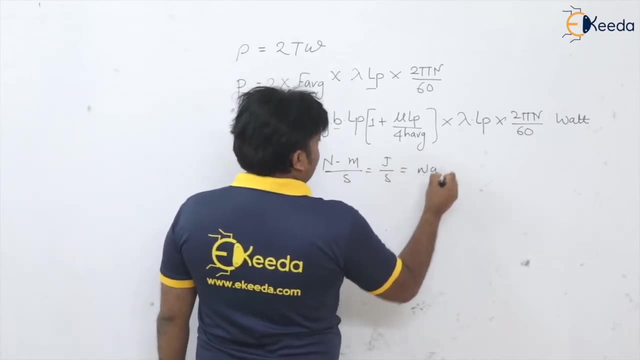 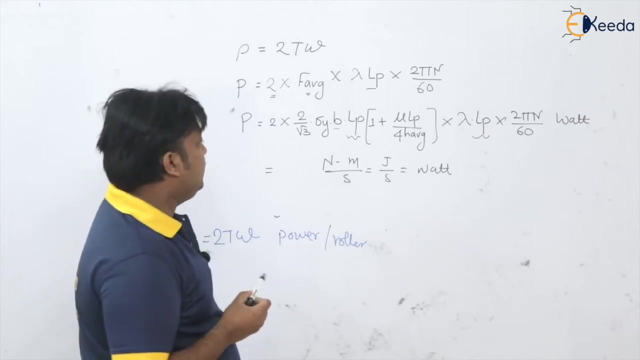 in watt and please remember that power is what it is. Newton meter per second, that is joule per second. that is watt. so whenever you take this value for LP here, try to get it in meter, not in millimeter, okay, so that you will get the power in watt. 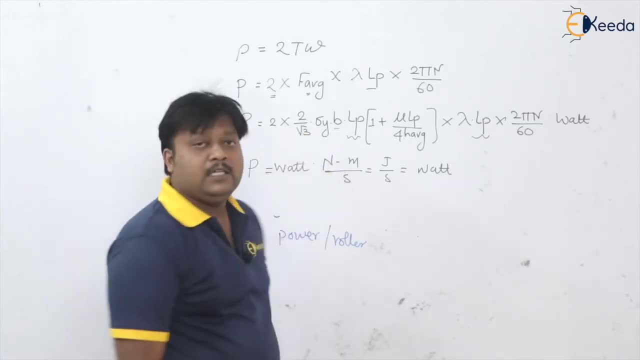 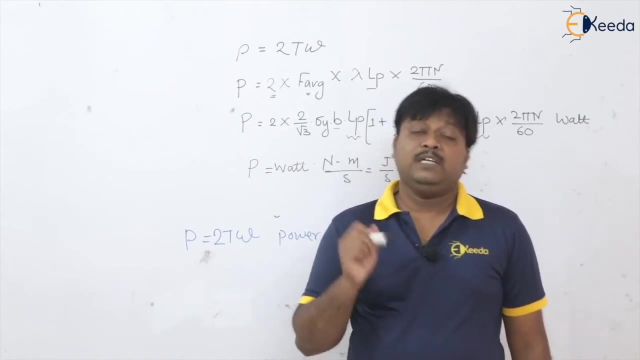 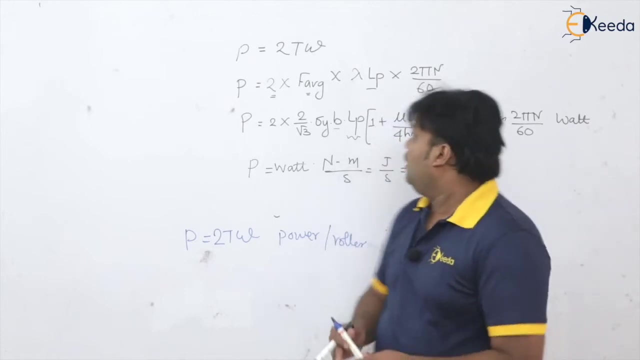 so this is the power in the rolling operation. try to use this formula only because we have assumed the plane strain condition. of course there are other formulas where plane strain condition is not assumed directly. you can get the pressure as the sigma y into sigma y into sigma y into. 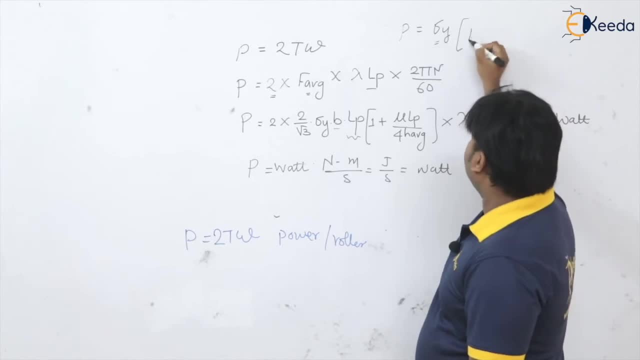 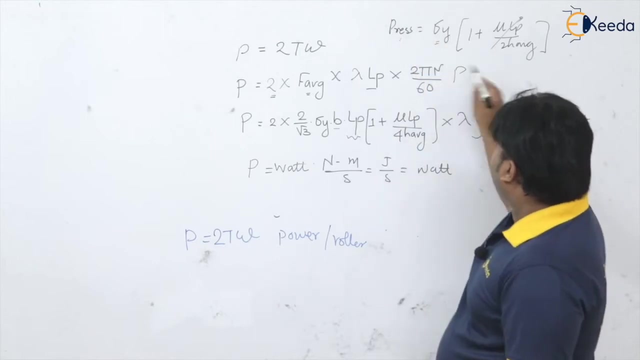 see directly sigma y. i am writing 1 plus mu LP by 2h average okay, and coefficient of friction not given. you can neglect this term directly. the sigma y is nothing but the pressure and you can directly have the power. this is, this is i am talking about the pressure. so power and force. 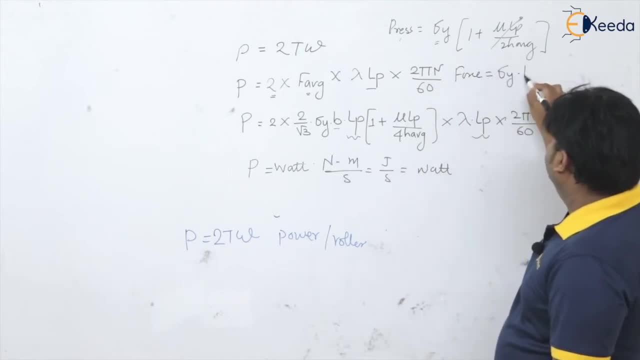 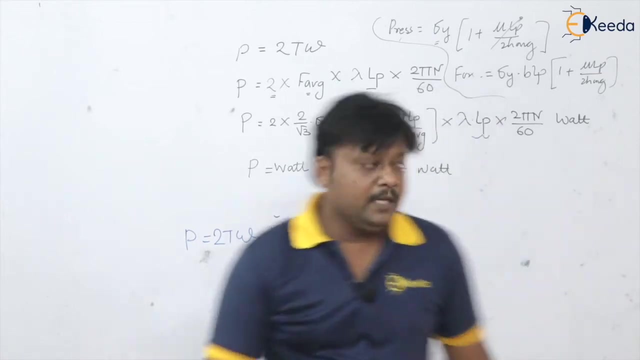 will be directly. the sigma y is nothing but the pressure and you can directly have the power into blp, into bracket 1 plus mu lp by 2 h average. see, this is the another method i'm talking about. from here i am telling another method, very simple, but see the nearness to the reality. 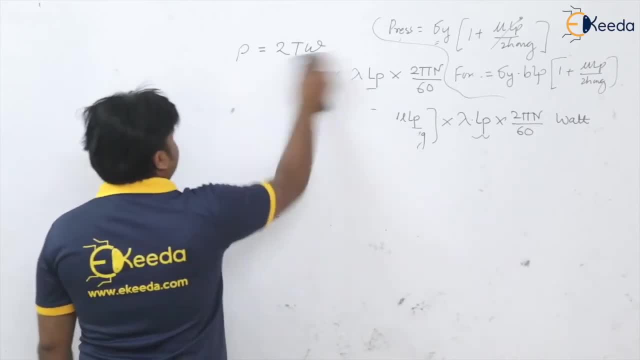 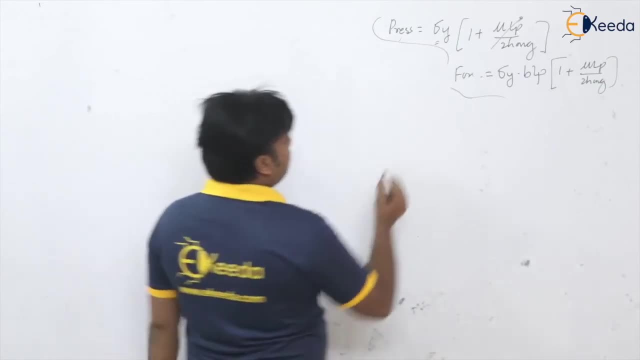 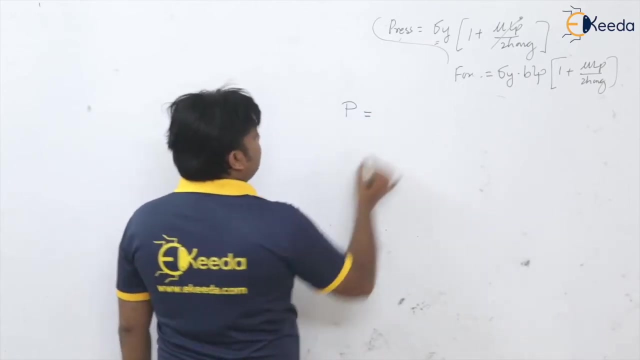 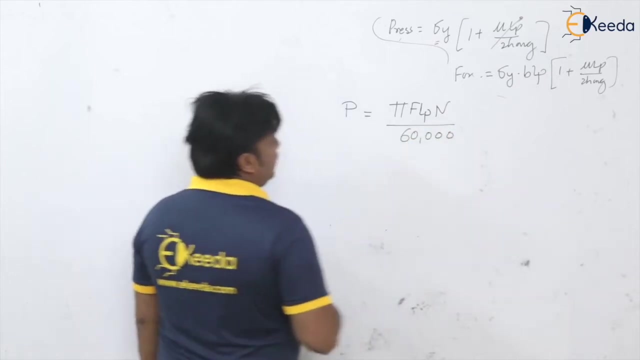 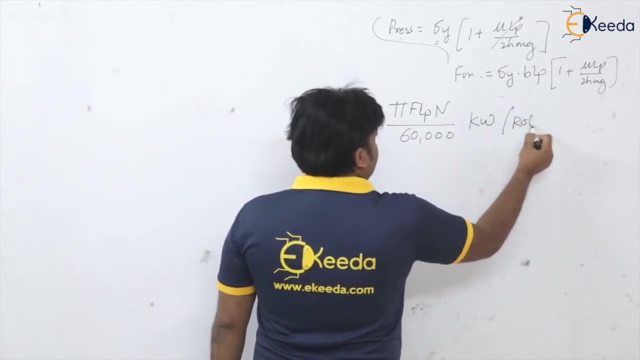 is only possible with this, this formula, okay, so here, by once you get this force, you directly get power. is equal to pi f, lp n divided by 60, 000. this is also way to calculate the rolling power. okay, and this is the power per directly, in kilowatt per roller. you want the maximum power, then you want the maximum power. 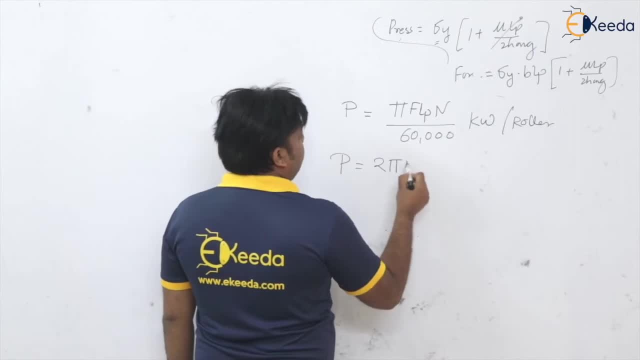 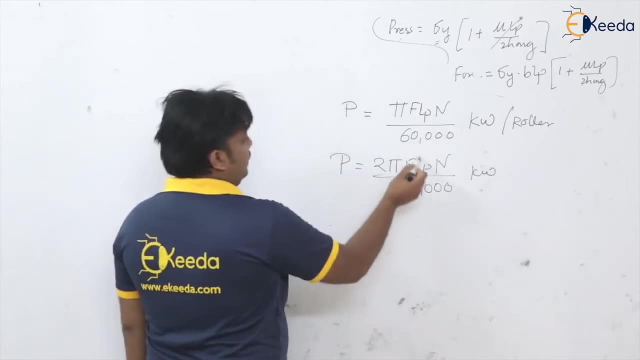 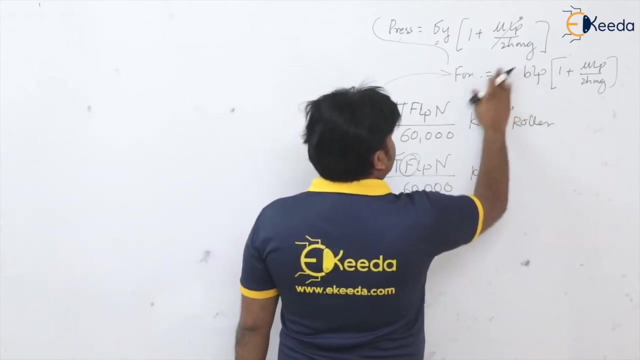 you want the maximum power, then you want the maximum power, then you want the maximum power. go for multiplying this 2 by f, lp n divided by 60,000 kilowatt, so your f will be calculated as with this formula, okay, where we have not consider the plane strain condition, if plane strain 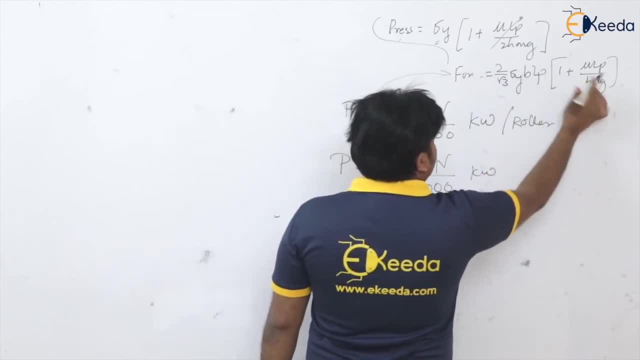 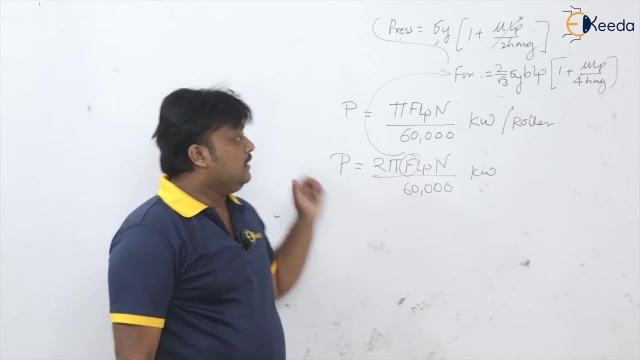 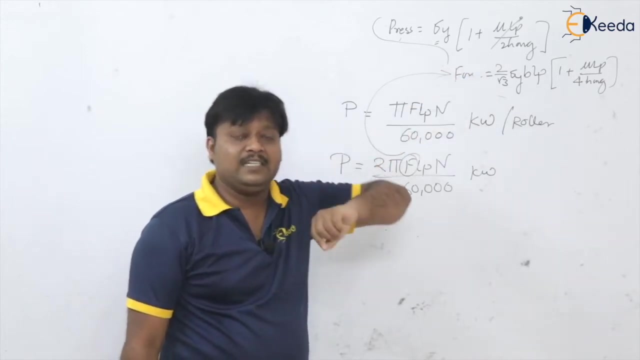 condition 2 by root 3 times sigma y, and instead of 2 here 4 will come. that is the difference. so anyhow, we will solve the question on this power. so next the question I will solve with this equation, that is, plane strain condition 2 by root 3 times sigma y, say solve kurunga power. 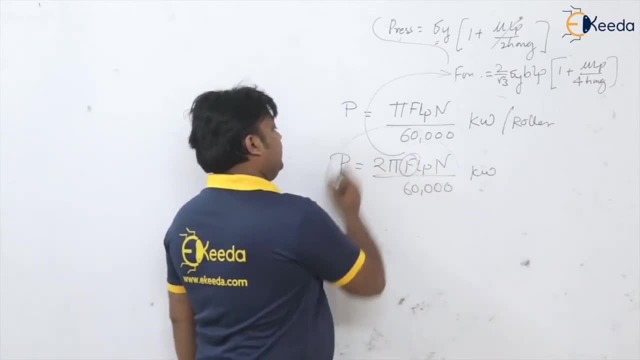 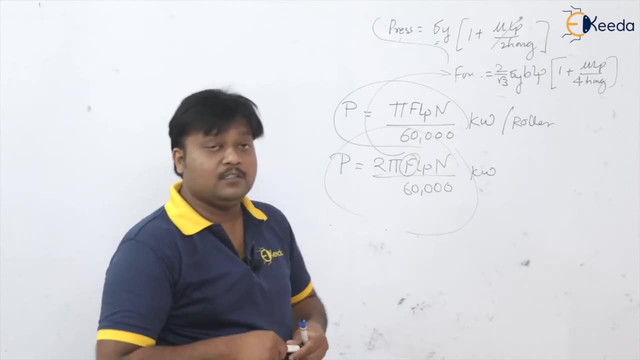 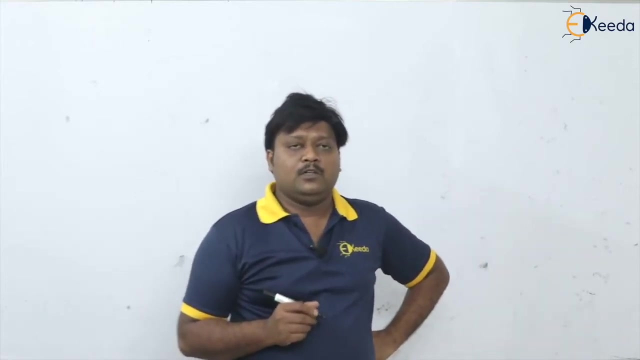 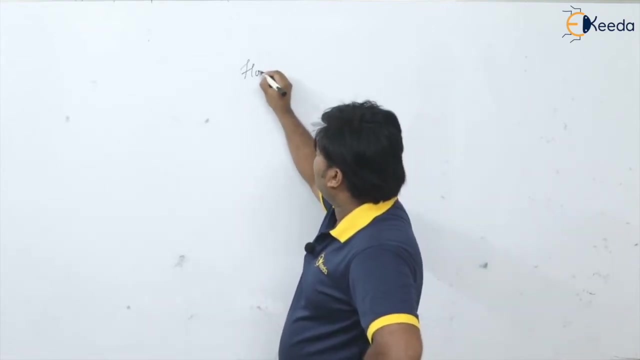 you can go and solve for with this formula. okay, just now, whatever I discuss, and just check the answers. okay, now let us solve one question. so, students, before going into that power calculation, you question, so let us see how we can able to reduce the role separating force, how to reduce this. 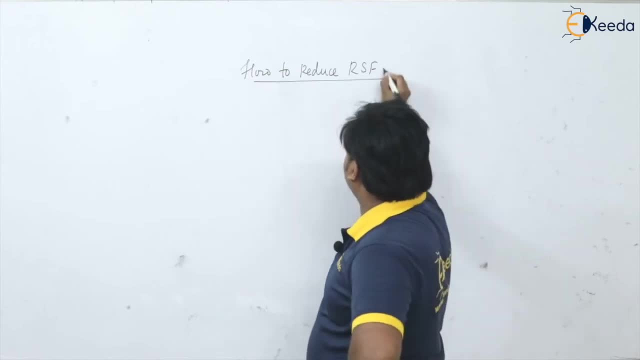 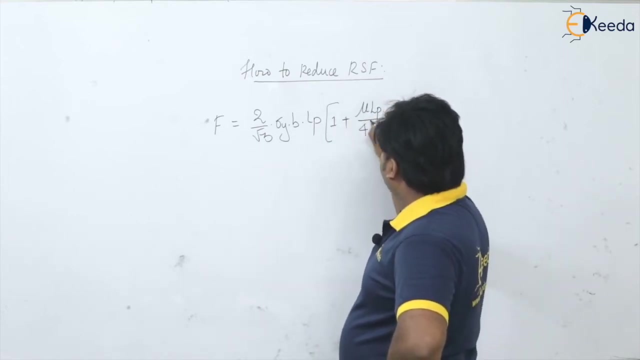 role, separating force or simply the force in the rolling operation. what is formula? f is equal to 2 by root, 3 into sigma y, into b times lp, into 1, plus this mu times lp divided by 4 h average. okay, so this is the formula. so let us see, because many times this is. 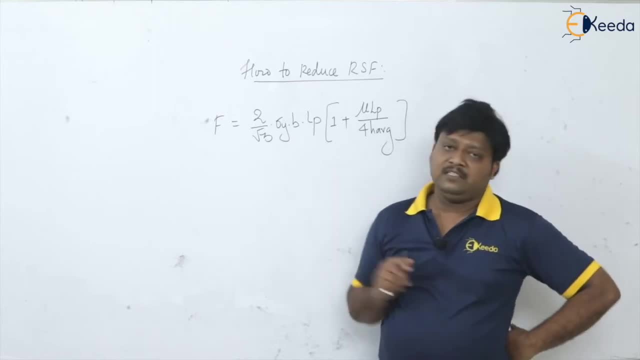 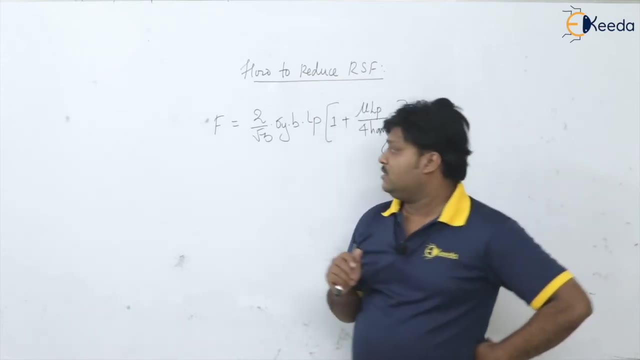 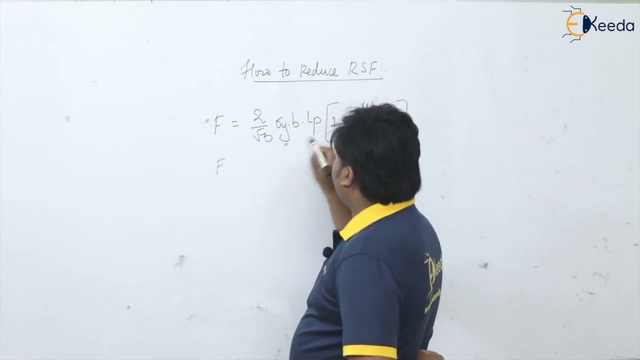 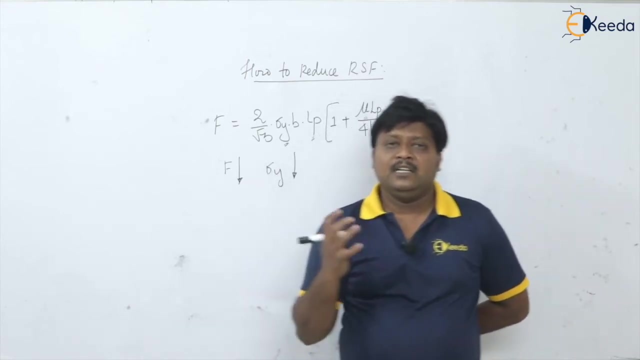 ah, ask in the exam that: how to minimize the rsf, that is, role separating force in the rolling operation, and this is a liner question for two marks. so see here, force c: it is directly proportional to the sigma y, lp and coefficient of friction And, of course, the application of front and back tension. Okay, So basically, see here, the force can be reduced by reducing the sigma. why isn't it? Yes, how to minimize the yield strength of the material. So go and heat the material above its recrystallization temperature. definitely the material becomes soft, its yield strength going to come down. 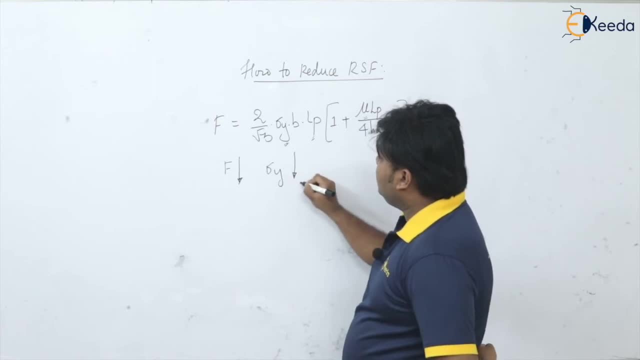 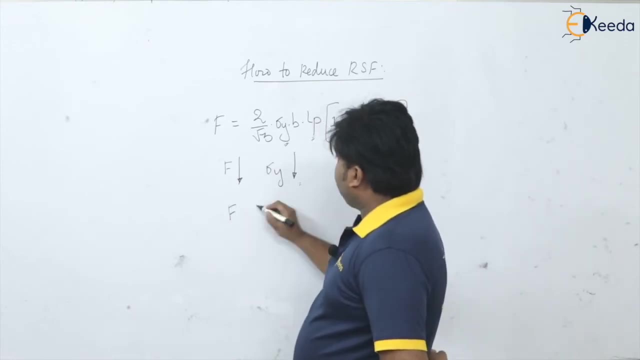 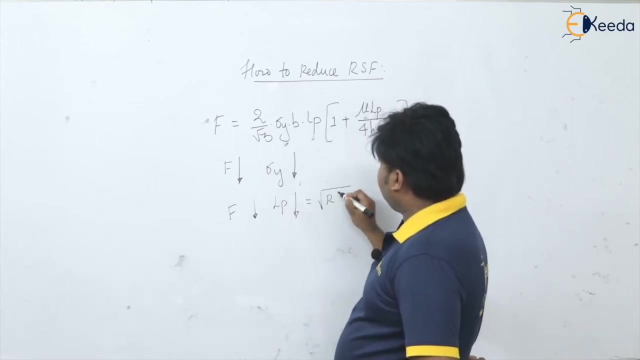 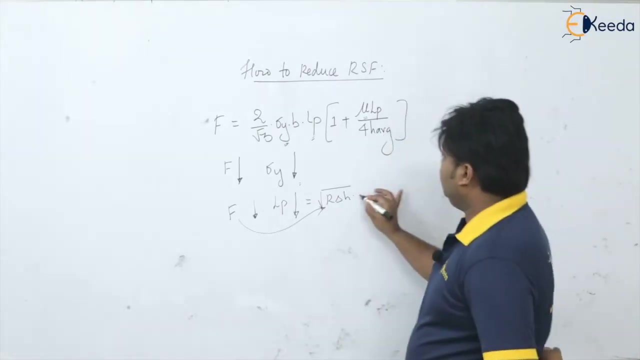 So the first thing is that you have to minimize the yield strength of the material. Okay, to minimize the force Again. second thing: what we can do, we can minimize this LP, isn't it? We can minimize this LP, But you know, LP is what is equal to under root of R. delta H means the force can also be reduced by the reducing roller radius or diameter. Yes or no? 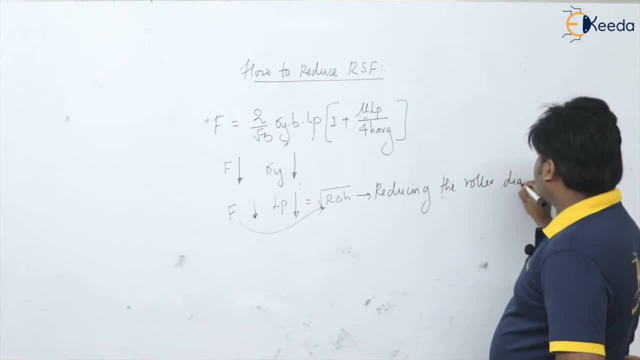 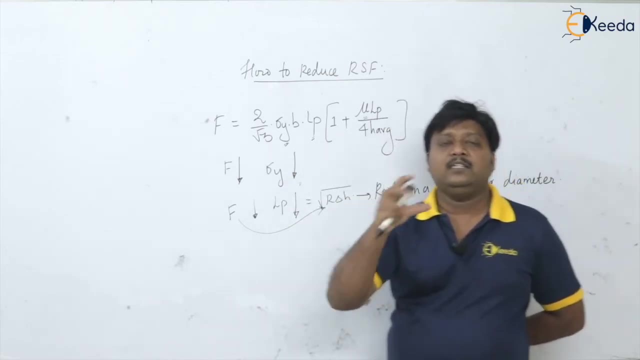 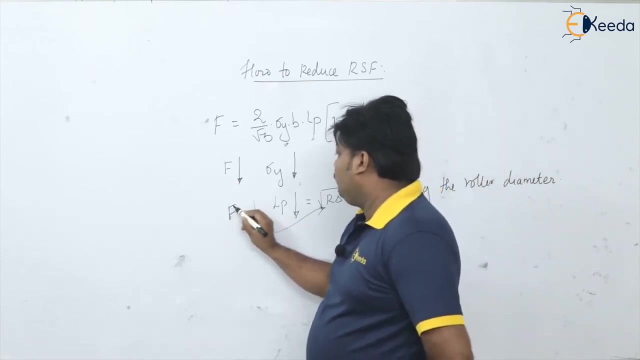 Reducing the roller diameter Okay, But when you go on reducing the roller diameters, you have to provide the backup rolls to maintain the rigidity, isn't it? So no issue Again, you can reduce the force by reducing the roller radius or diameter. 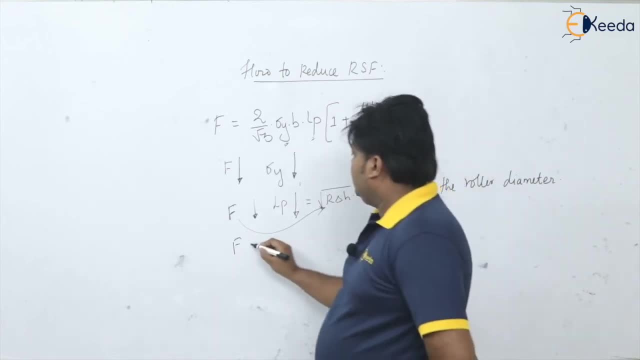 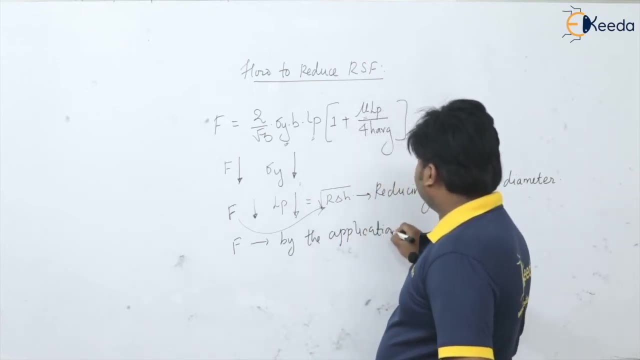 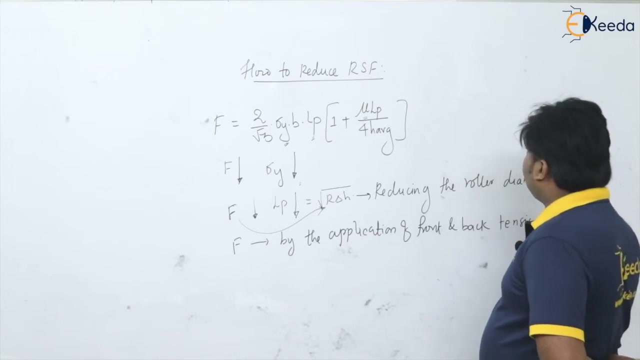 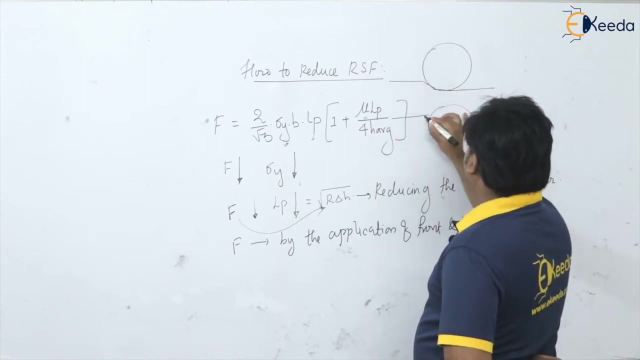 And the third thing, very important, that by the application of, by the application of the front and back tension- the front and back tension, of course, see when the strip is going to pass through the roller, it is undergoing the deformation. And if you apply the front and back tension like this, so what is going to happen there? they're going to be the effect called it, as see, poison effect is going to happen. 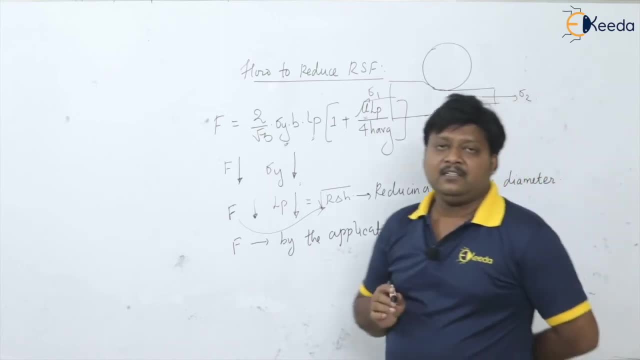 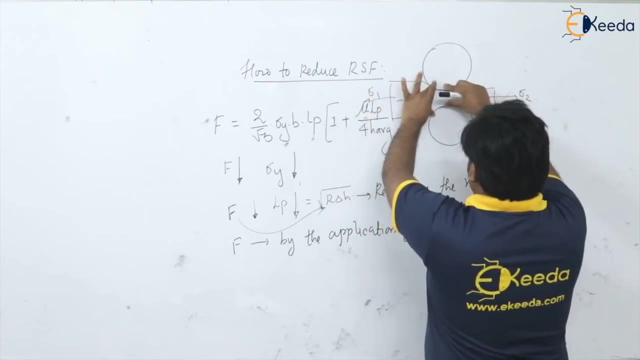 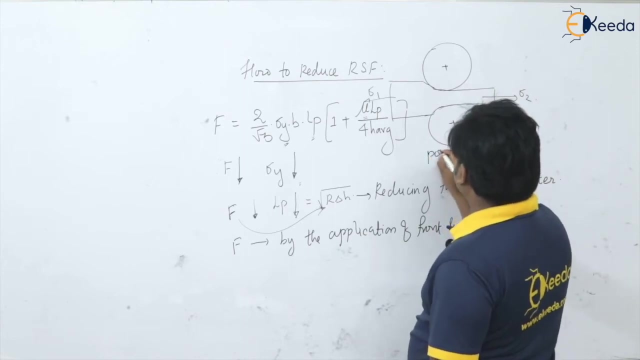 And back, And back And back. So generate, that is, in lateral direction. we are minimizing the thickness, isn't it? so we are getting here the poisons effect, the poisons effect, okay. so of course, this stress is going to minimize this thickness along the lens direction, so it 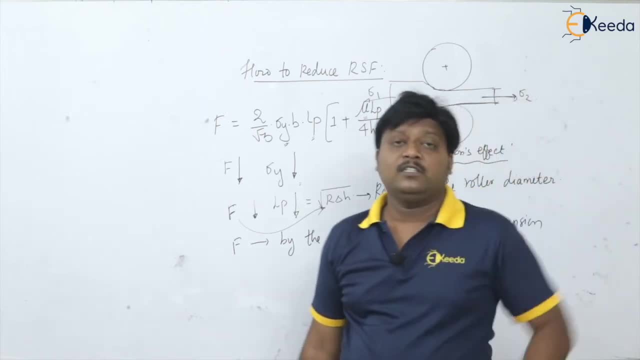 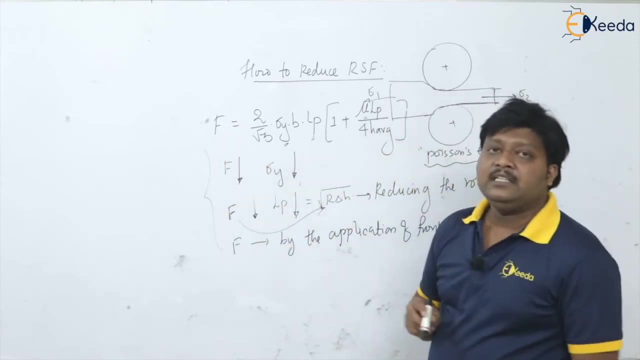 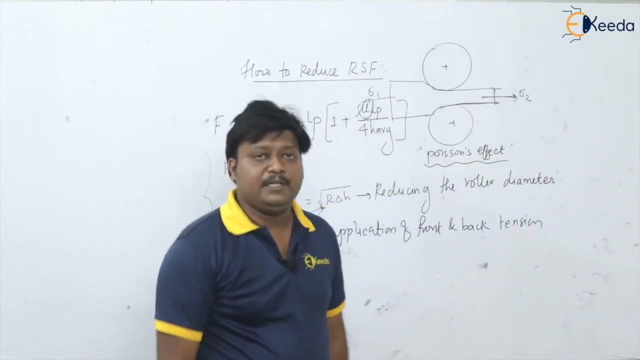 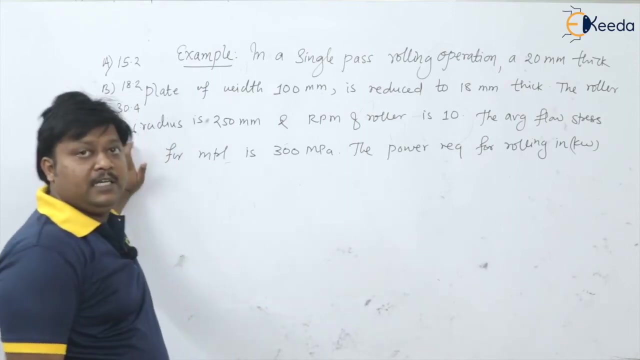 is going to help for reducing the force in the rolling operation. please remember so. in this way we can able to minimize the force. of course the mu also. if less, then also you can reduce the role separating force. okay, now let us see the question. so students see the question: what is given here in a single pass? 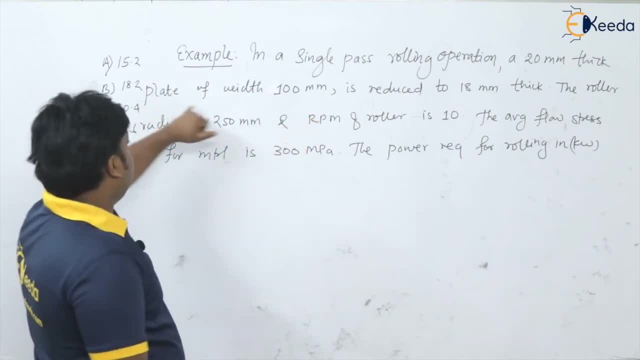 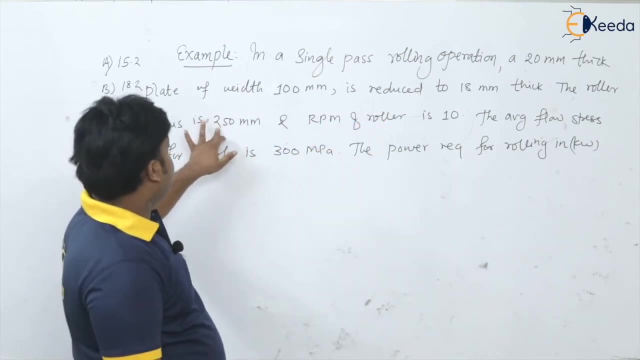 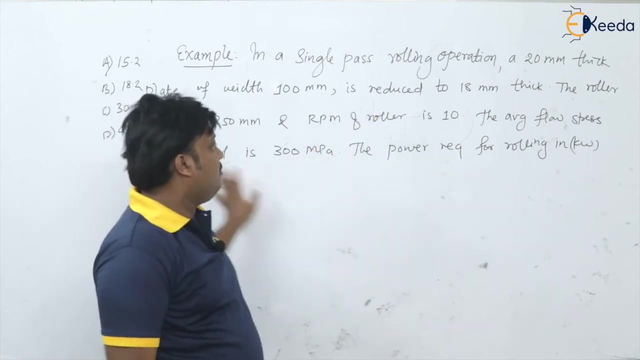 rolling operation. 20 millimeter thick plate of width 100 millimeter is reduced to 18 mm thick. the roller is radius is the roller. radius is 250 millimeter and the revolution of roller. how much then rpm is given? the average flow stress of the material is 300 and 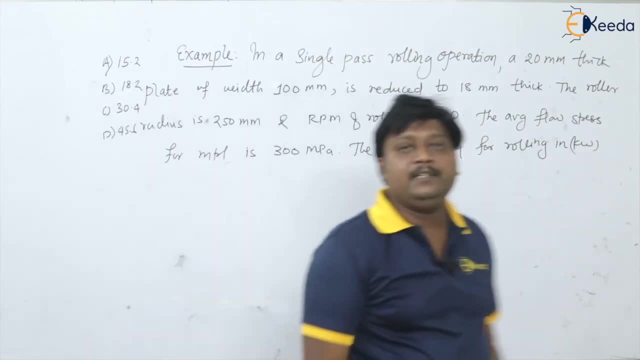 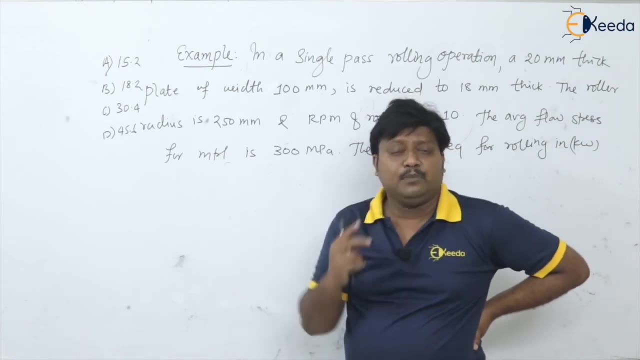 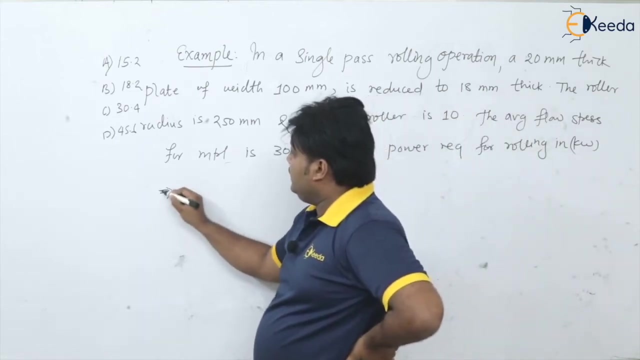 mega Pascal, the power we have to calculate in kilo watts. okay, so this is actually question from ISC Bangalore, the gate paper 2008, mechanical engineering. so see here. so I will write the data. original thickness: 20 millimeter. final thickness as 18 millimeter roller radius. 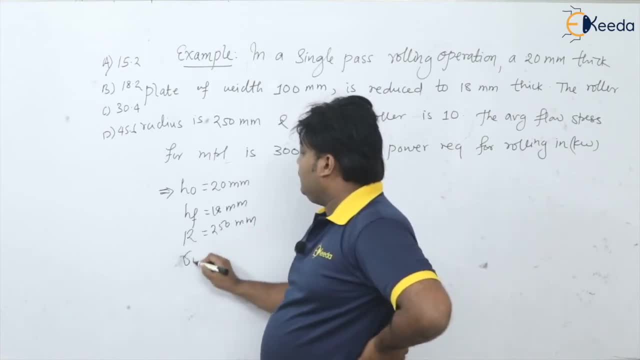 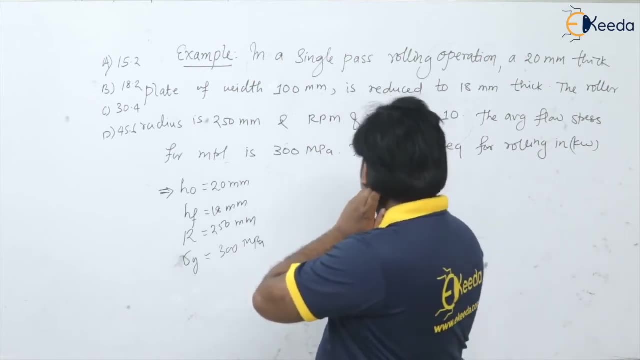 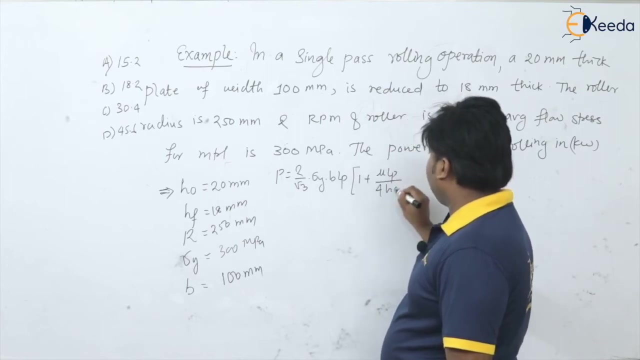 250 millimeter and Sigma Y or Sigma flow stress is 300 mega Pascal, okay, and width of the plate is 100 millimeter. so power, you know, power power is equal to 2 by root, 3 times Sigma, y, times V LP into bracket 1, plus mieux lka 4h average into lambda times. 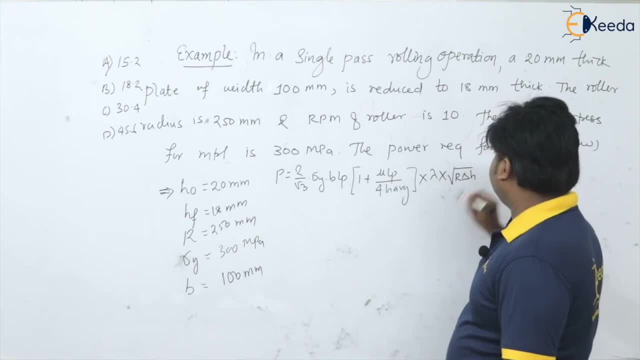 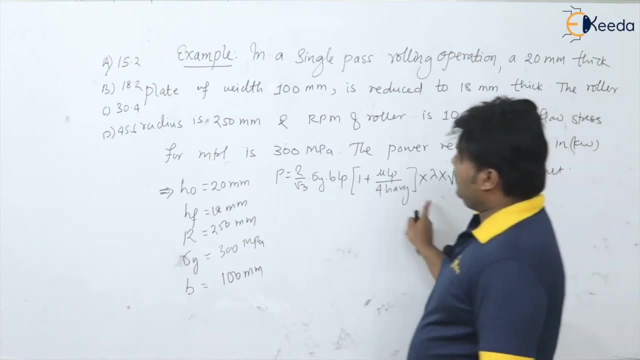 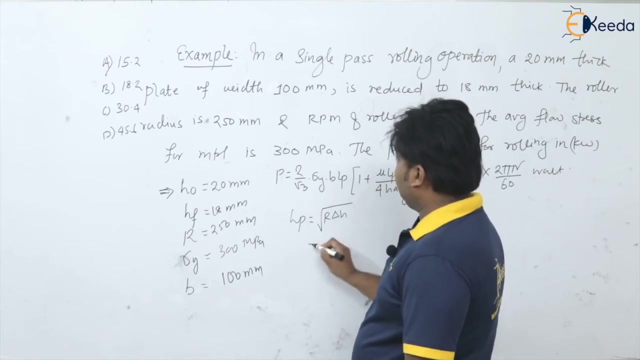 under root of r Delta H into 2 pi n by 60 watts, and this is power per ruler. if I multiply by 2, this is this. we get the total power. of course total power is gas, not power per follower. so first of all, calculate this lp value as under root of r delta h, what is 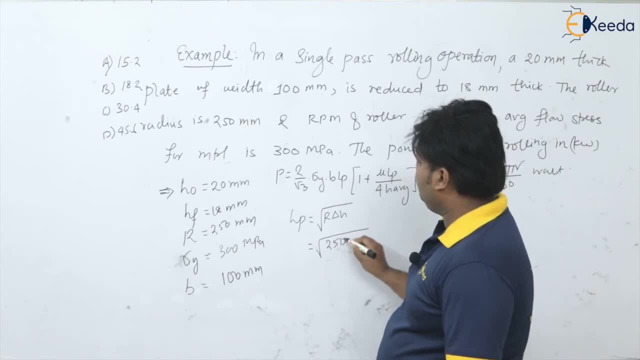 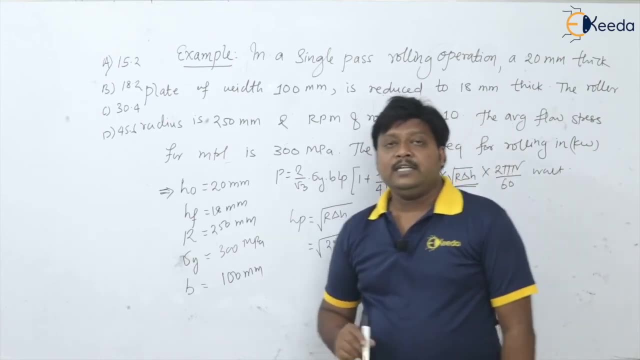 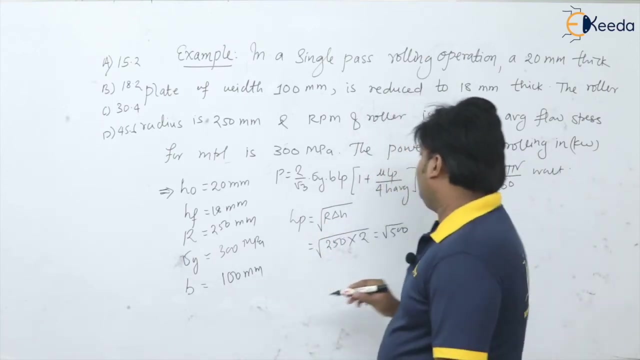 r 250 into delta h, 20 minus 18, 2, so under root of 500. okay, so here lambda value. unless and otherwise stated, we will consider that this rolling is hot rolling, so lambda will be 0.4. okay, so to get this use of this entire formula for roll separating force, let us calculate the. 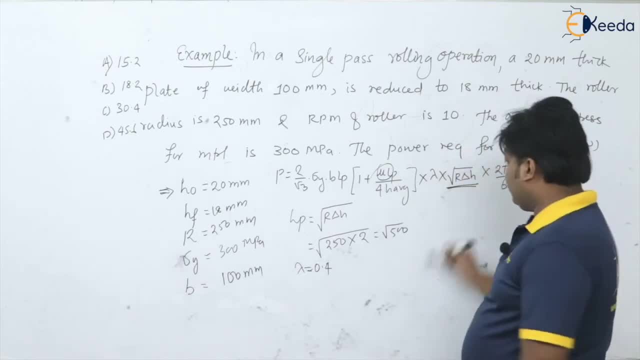 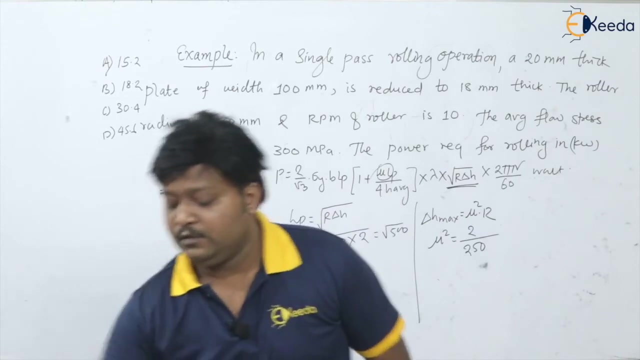 value of mu. okay, mu is not given, so calculate here. so we know that delta h max is equal to what mu square times r. so what is mu square? and delta h max is 2 millimeter divided by roller radius of 250. so 2 divided by 250 root. 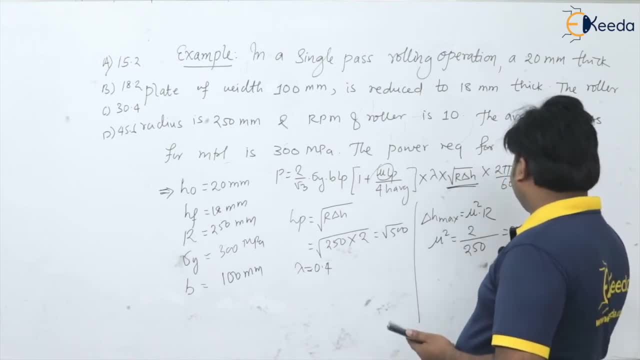 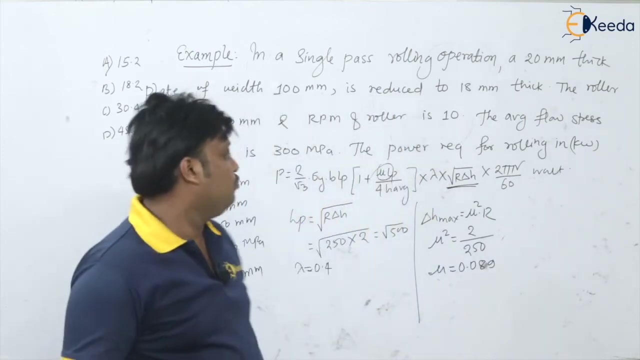 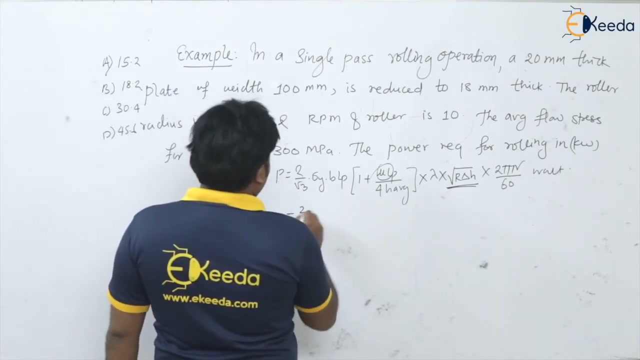 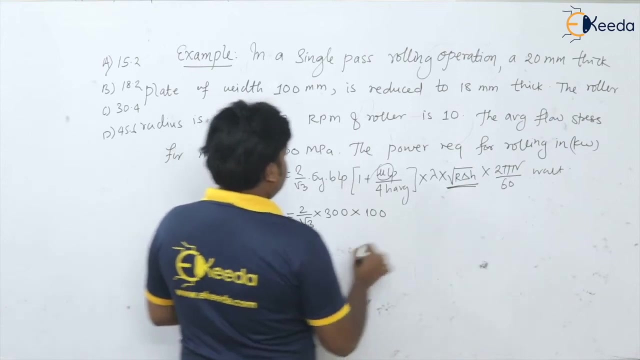 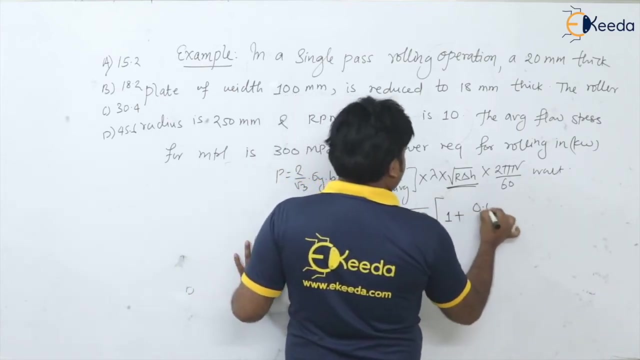 of the answer will get 0.09 as the value of coefficient of friction. you got here 0.089, actually here. okay, so let us try to put the values into the equation. so this is 2 by root, 3 times 300 times 100. isn't it into root of 500, into 1 plus 0.089, into root of 500? 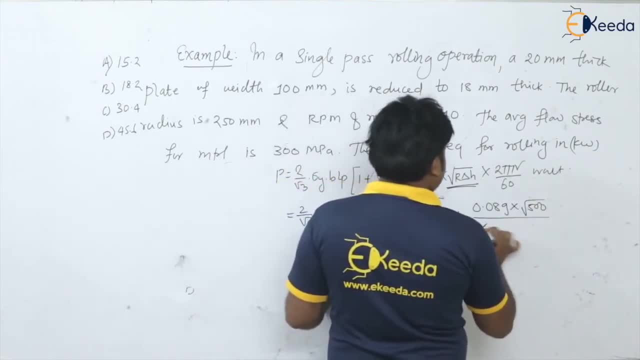 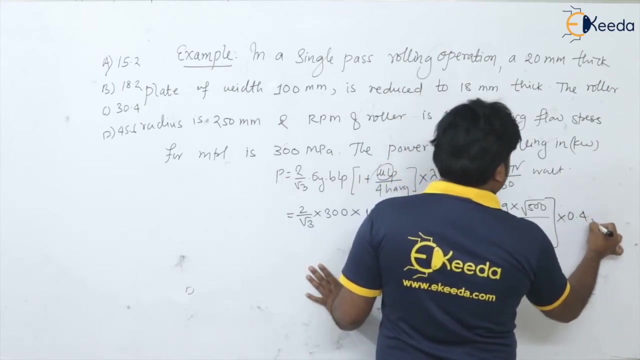 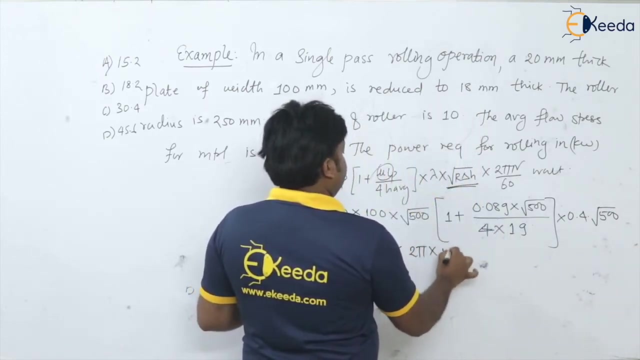 divided by 4 times, what is h average? 20 plus 18, 38 divided by 2, it is 19. okay, into 0.4 times. under root of 500 is our lp into 2 pi rpm 10 divided by 60. so let us calculate and tell me. 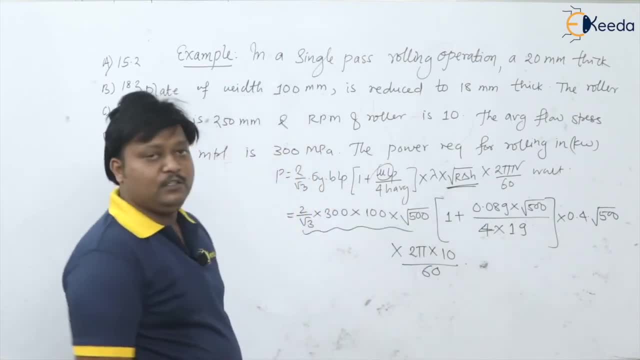 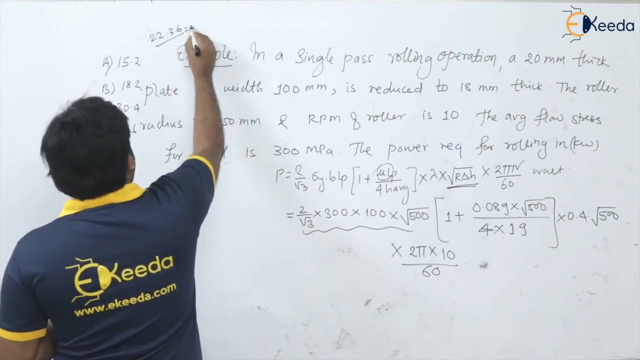 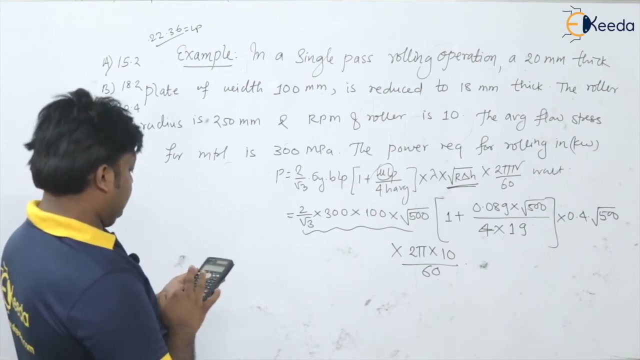 the answer. this is the power per roll. i have not multiplied by the two to get the total power. so root of 500 is 22.36. i will write here: this is our lp value. so 22.36 multiply by 300 into 100, into 2, divided by 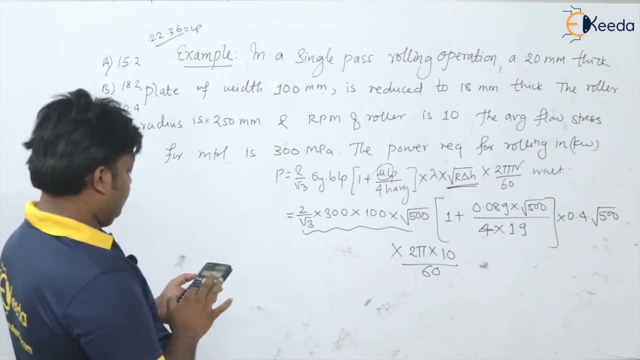 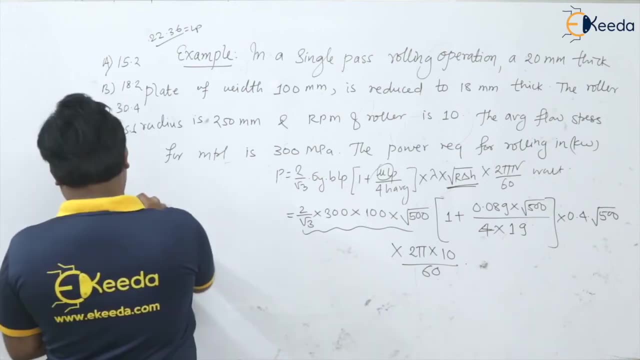 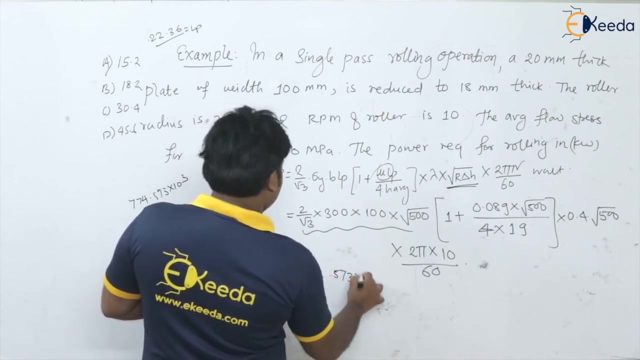 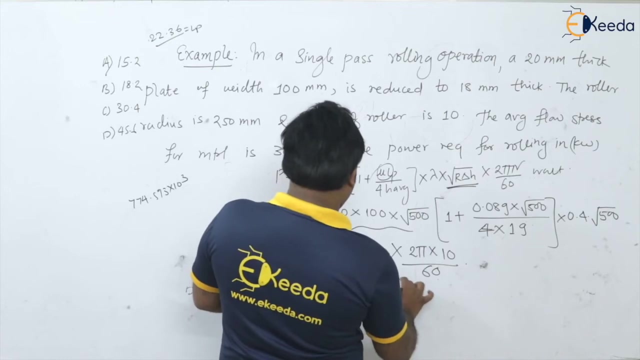 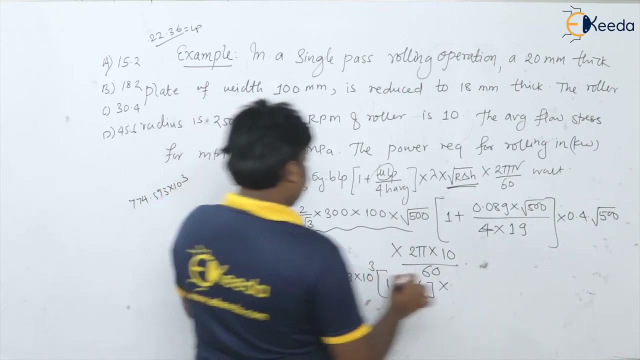 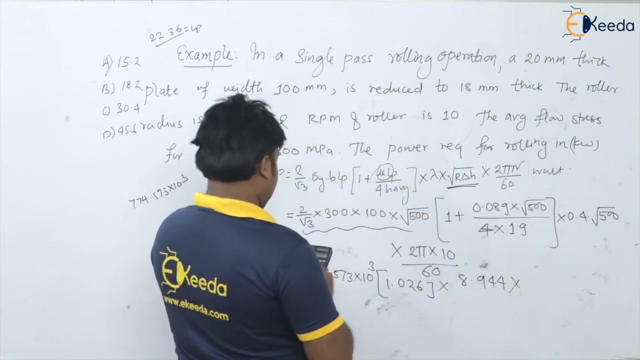 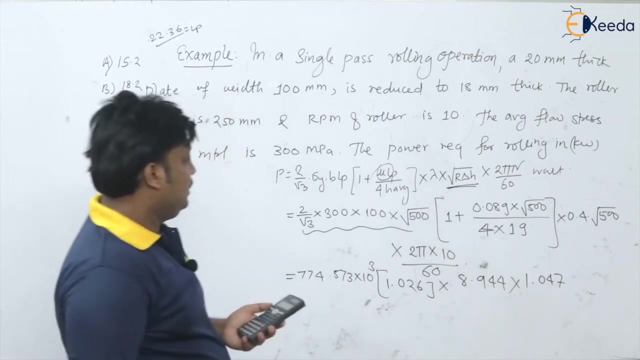 one double root of 3. okay, then you get this much value as 774.573 into E, to the power three in to bracket. so this is the value into one point zero two. six into eight, point nine, four, four into one point zero four seven. okay, so if you do this product of all we will get to one point. 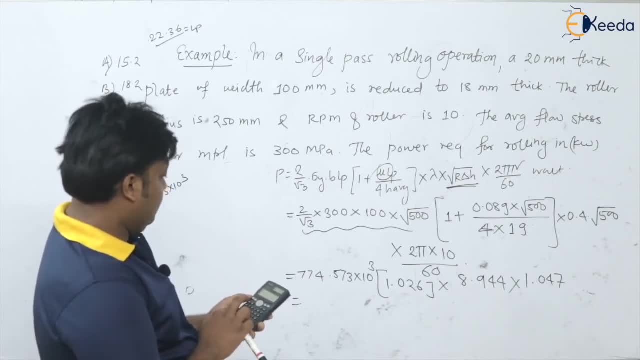 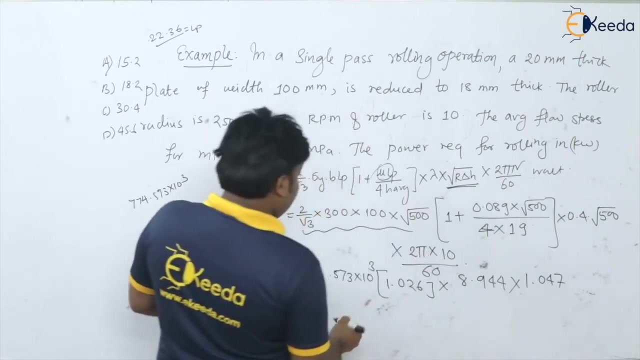 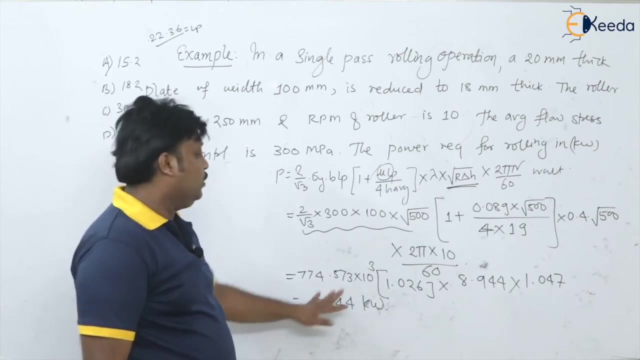 zero two six into seven, seven four point six. so you got here the power, as of course, the seven point four, four kilowatt. okay, if you get this power, you got it here seven point four, four kilo, while now here they are asking the total power. 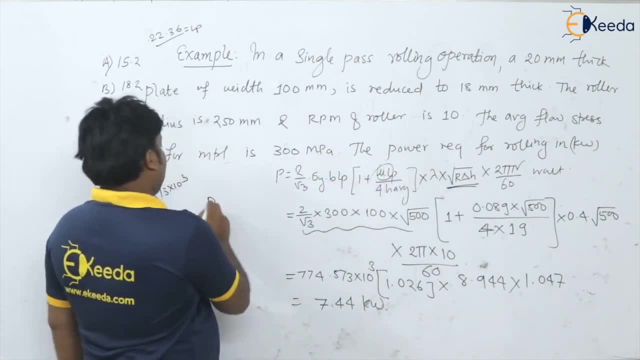 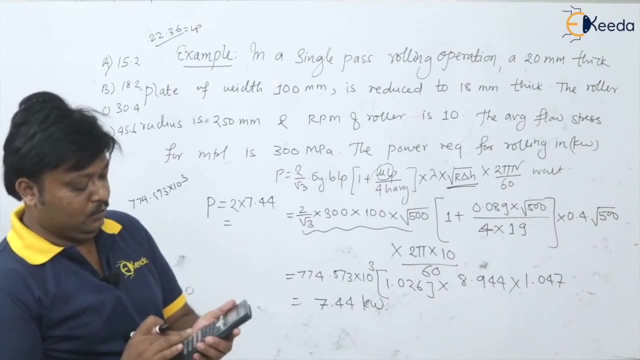 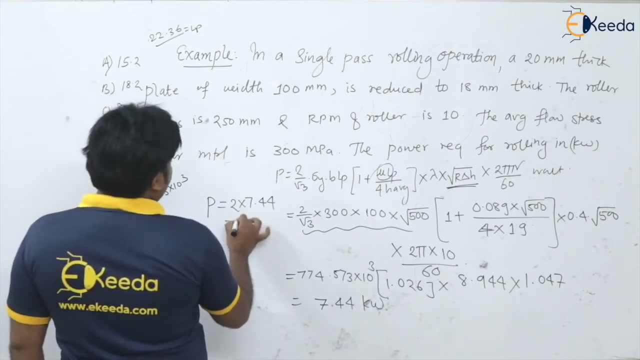 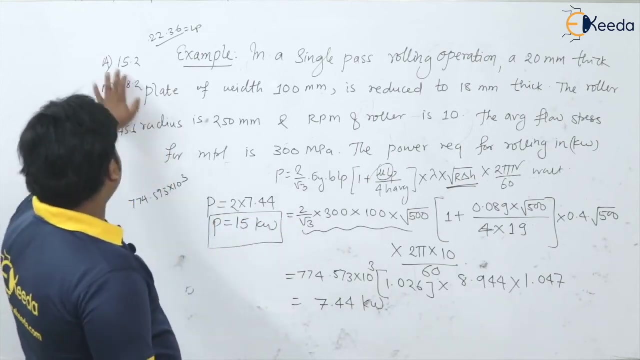 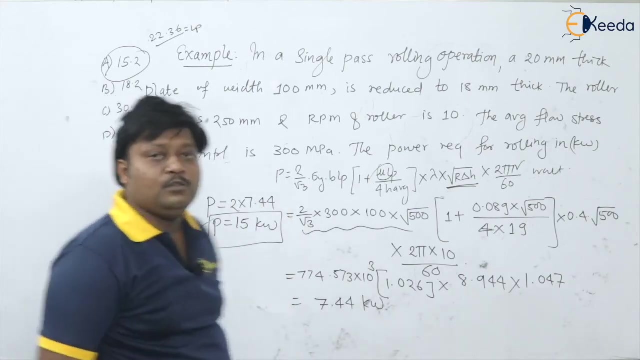 required in the rolling operation 2, so this total power will be 2 multiplied by seven point four, four. so how much it is in true? true, so it is around fourteen point eight, eight, or nearly equal to fifteen kilowatt. okay, so see here nearest answer. you are having here 15.2 kilowatt. this is the answer understood now in this video we are. 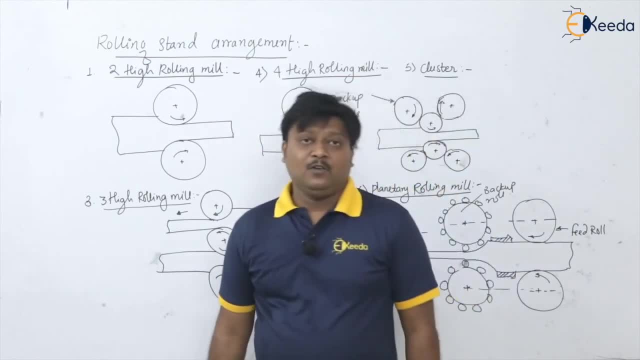 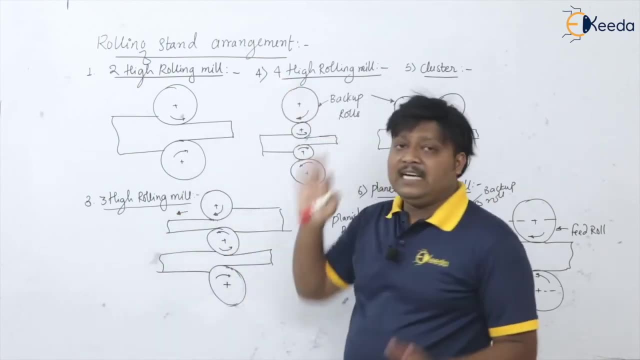 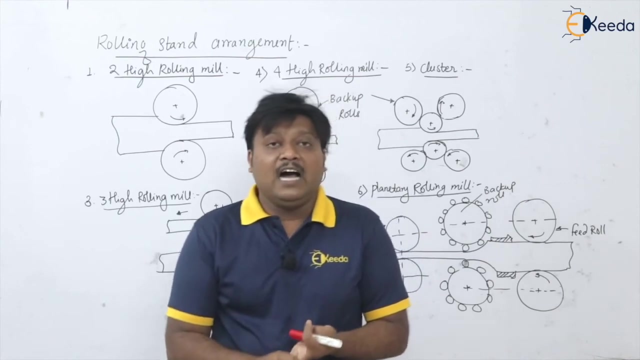 going to see the rolling stand arrangements. okay, the how the rollers are arranged in the rolling mill is called as the rolling stand arrangement. so you can see, here there is two high mill, there is two high reversible mill, three high mill, four high mill. right then there is a cluster mill. you 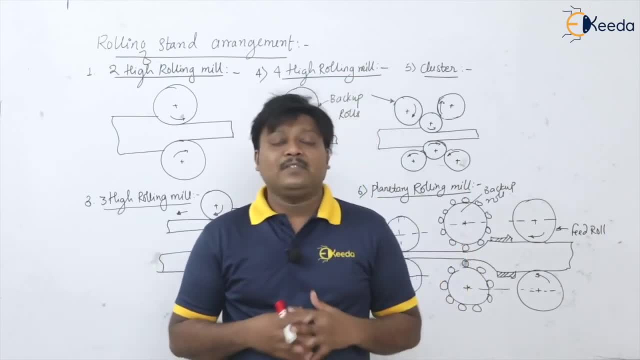 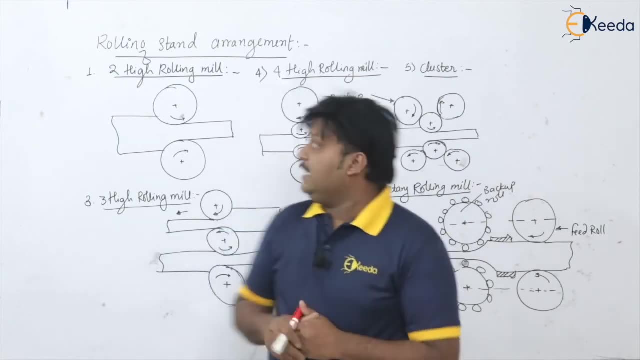 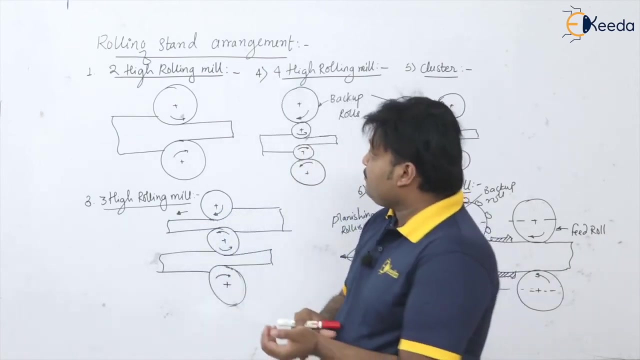 are again having the planetary mill. so these are the arrangements in the rolling mill for the rollers, which is nothing but the rolling stand arrangement. or simply you can say: these are the rolling mills, various types of rolling mills that we are going to see. so let us look here i have 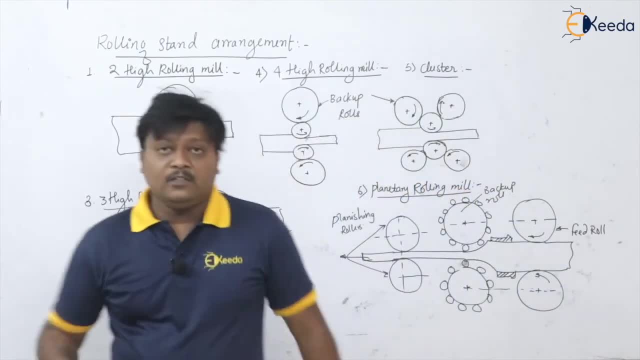 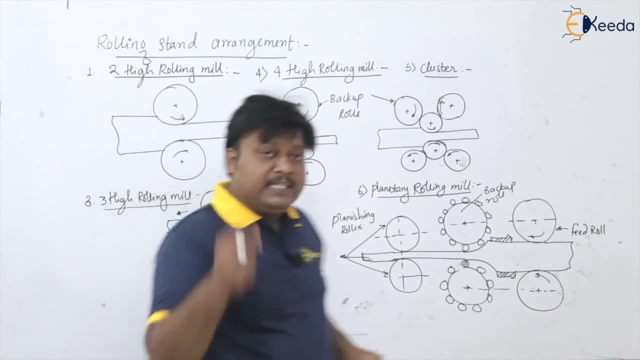 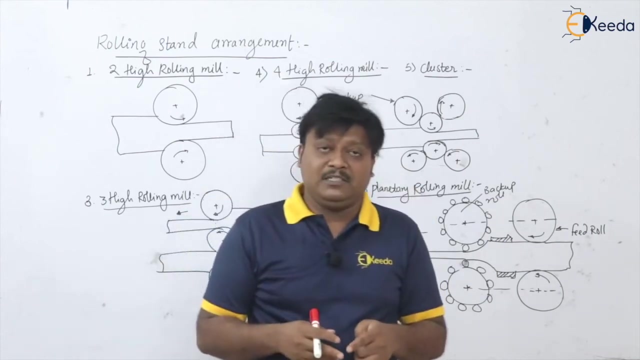 put the diagrams on the board, okay, so that we can get it quickly. see, this is the two high reversible mill. so basically, see the name for this. every arrangement is given from the how many number of rollers are there into the arrangement. that is the thing. see here, two rollers are there. that's why the name is to high. 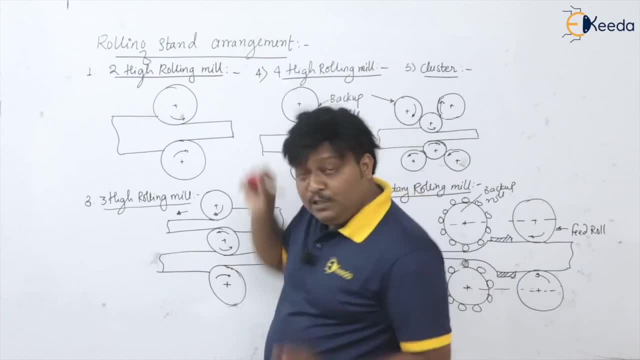 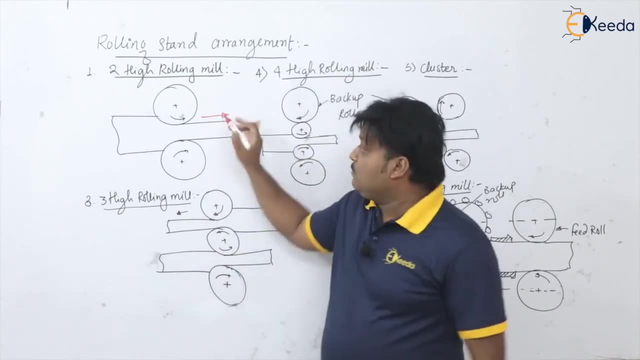 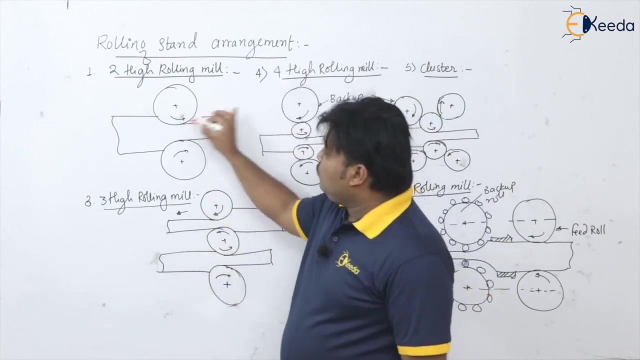 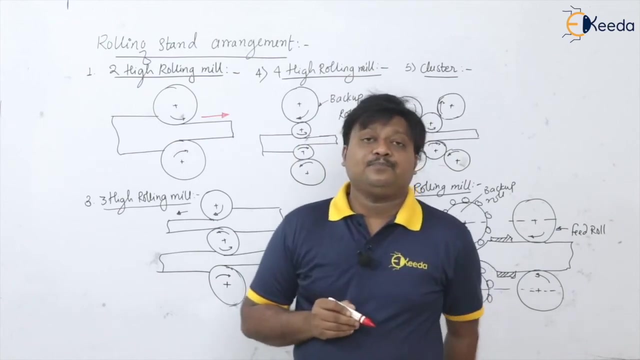 rolling mill. now, why only two high rolling mill? there are two rollers and it is moving only in one direction, and this is most commonly used rolling wheel that is too high rolling wheel. okay, the roller will move only in the one direction, so that this strip or this slot or the plate will also move into the one direction. 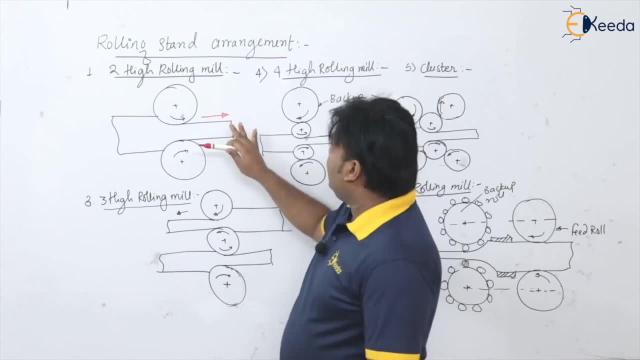 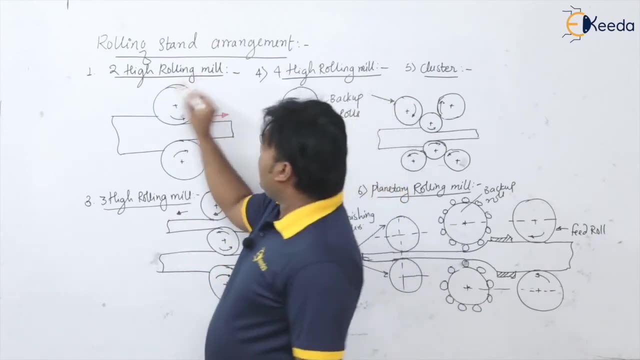 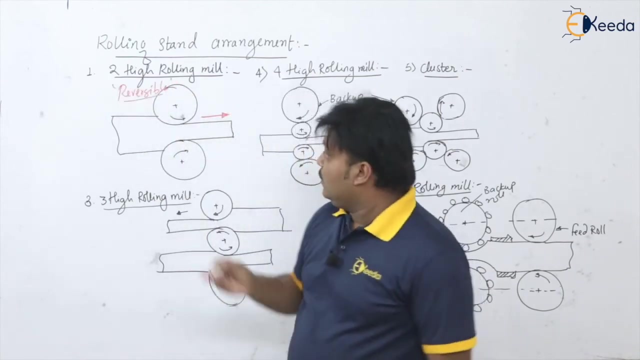 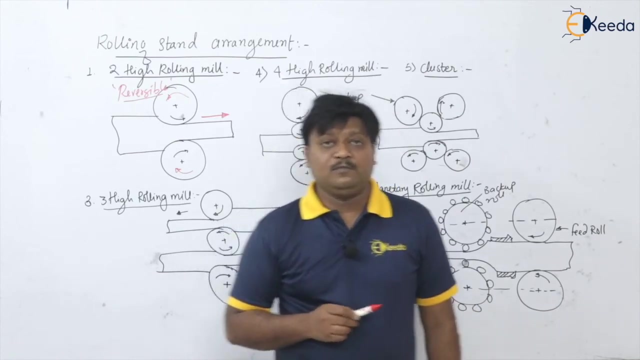 so this is the too high rolling wheel if you look at the too high reversible wheel, okay. so next category in that, if i say this is too high reversible, okay. so what is mean by this? so here we can change the direction of rotation of the rolls. okay, once you have completed this pass. 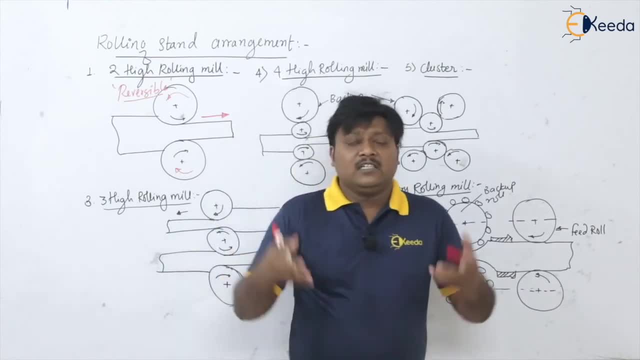 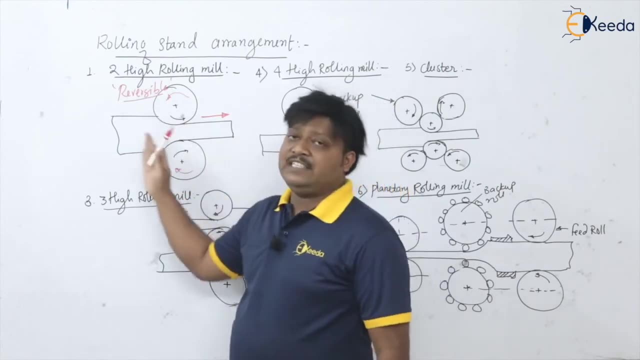 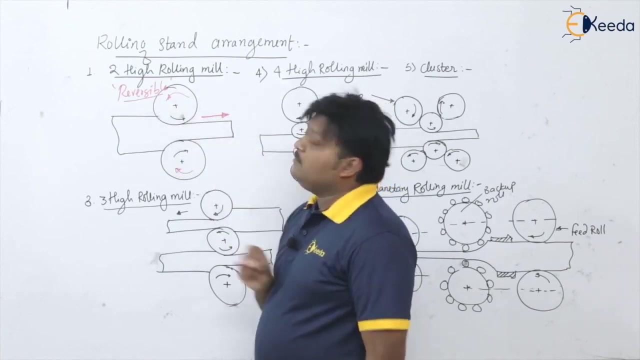 so the in between the handling of this hot slabs, we are doing this arrangement, that is, you can rotate the roller now in reverse direction also. that is the name of this stand, rolling stand is what the too high reversible rolling wheel? okay, too high reversible, we are having the. 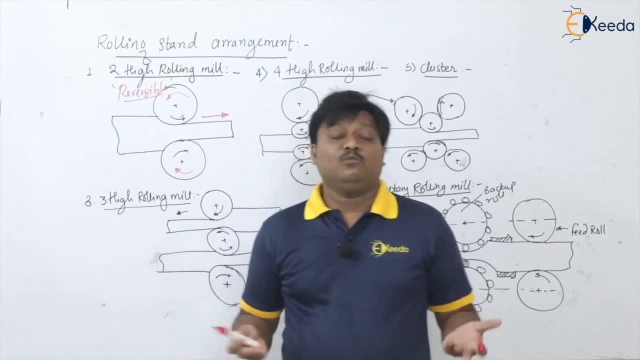 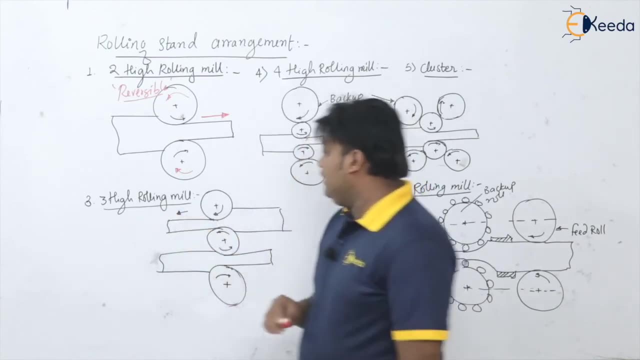 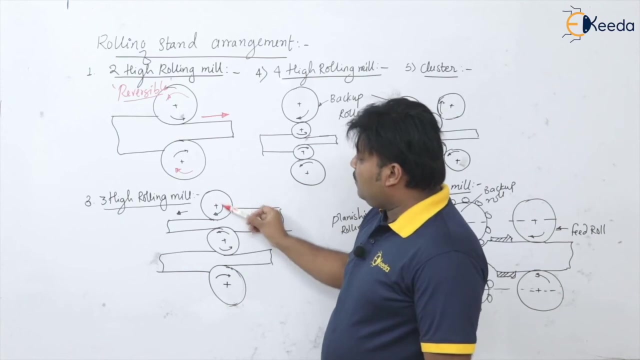 arrangement to reverse the direction of rotation of the roll. that is why this is the too high reversible. now let us see the three high rolling wheel. so of course, by the name is how the name is given, based on how many number of rollers in the rolling stand. so here see three high reversible mean so here. 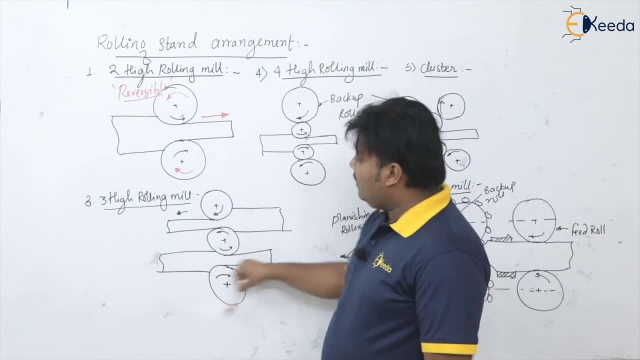 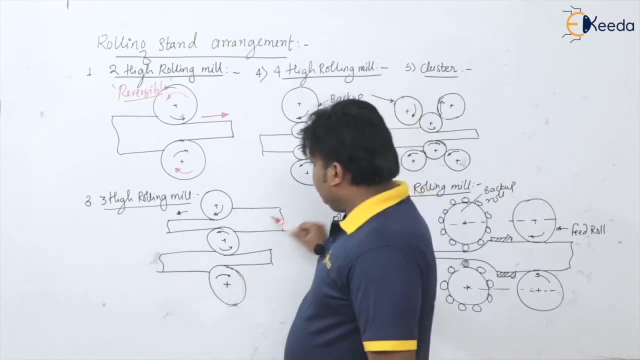 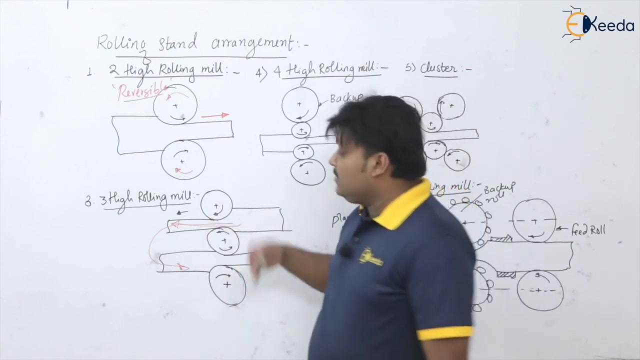 basically, this three high reversible mean is used for getting the continuous reductions by having the number of passes. so once see if this pass is completed. okay, now the this plate is given for the next pass. without unloading from the arrangement, you can see how the number of second pass. so this is the three high rolling mill. now let us come to the 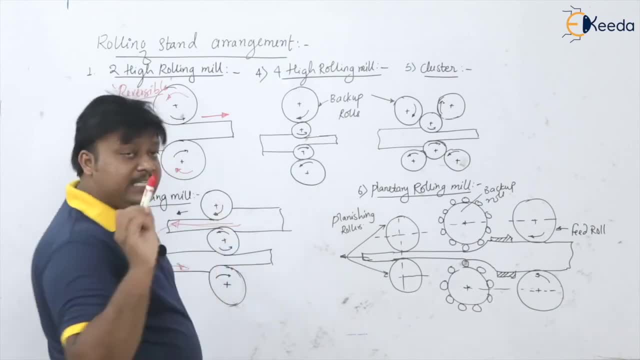 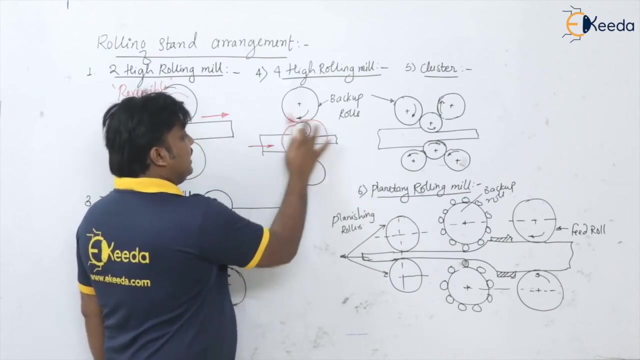 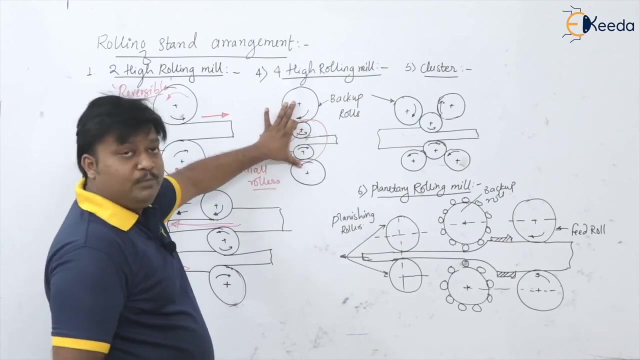 four high rolling wheel. of course, four rollers are there, but you can see, here there are basically these two rollers which are reducing the thickness of this given plate, isn't it so, whatever the deformation or thickness change is obtained by this two small rollers and these two rollers, these two big rollers, are simply backup rollers to increase the rigidity of 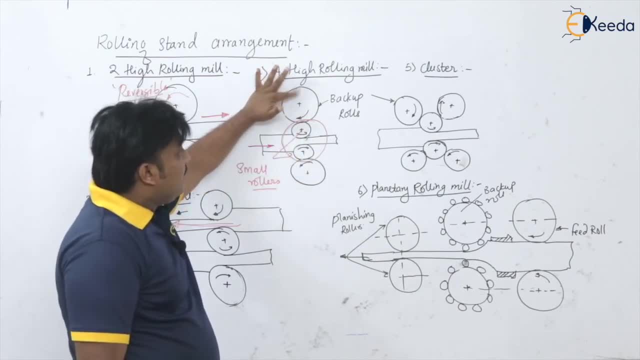 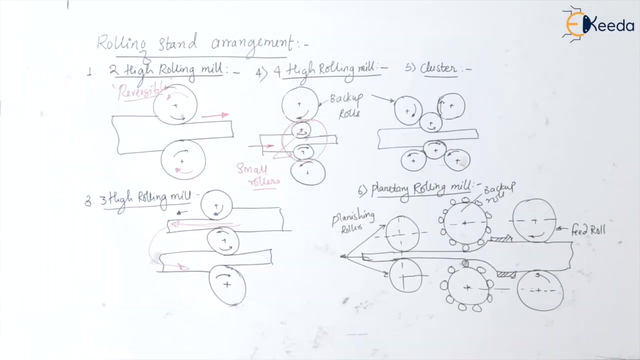 these small rollers. that's why this backup rollers are used only. and one important thing is that these axis, if you draw the axis from the centers of this, all the rollers vertically, it should coincide. okay, these axis should get coincide, otherwise definitely the chances of failure will be more there. 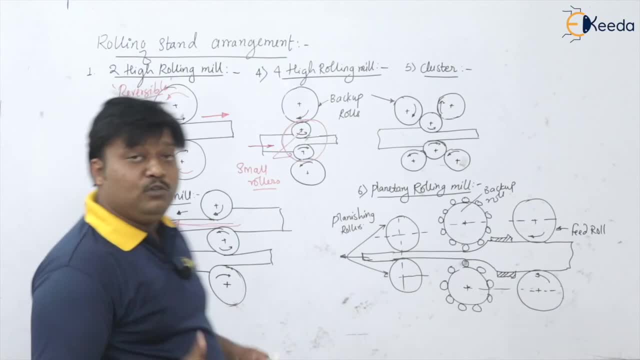 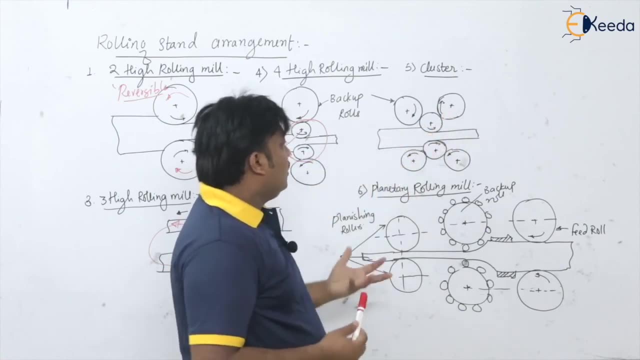 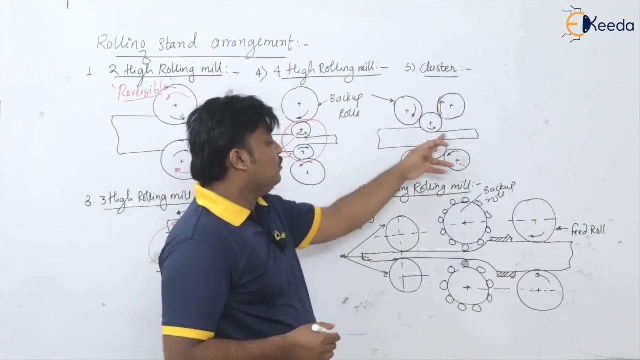 again, if you want to have even very good rigidity for this rolling stand, so again you can have the number of uh rollers you can use as a backup rolls. so again, see here, this is the small rollers which are doing this reduction operation in the thickness. but you can again increase this. 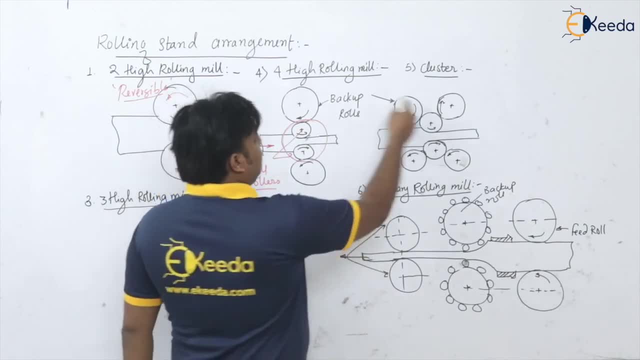 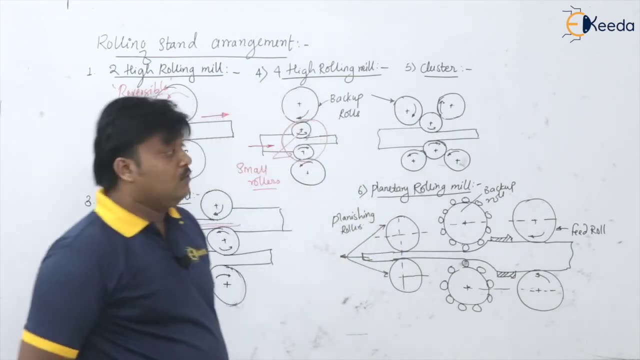 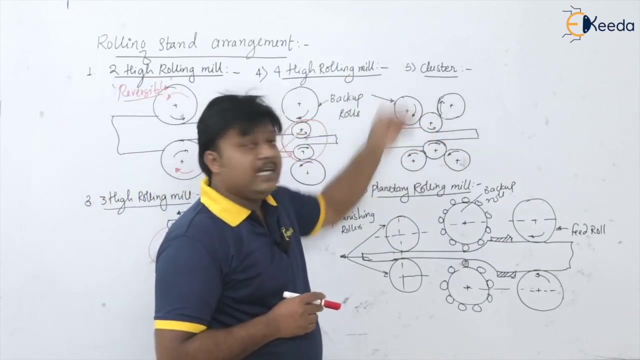 rigidity of small rollers by having this. instead of one, we are having this two for both the rollers and this one for the back up rolls. okay, so this is about the four high rolling mills, and more than four. we can call it as a cluster mill. okay, this is a cluster. and the last.